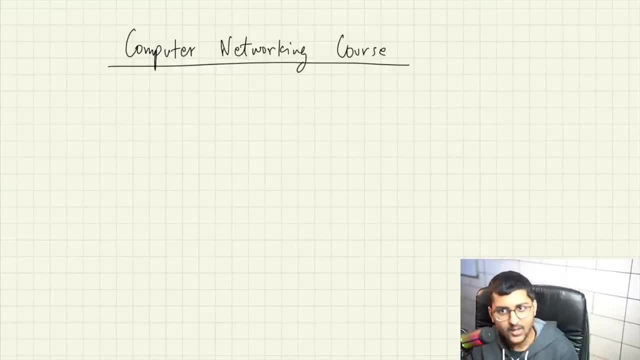 about how internet works so we look at like what is internet basic stuff how it started right what were the early days like how it has evolved over the years and then technical deep types so what happens when you enter a url what is a url how it gets resolved what is a server what is a client what is the you know protocol what are the protocols the osi model and how actually how things are working you know in a story format because even though we're learning about the textual textbook stuff obviously but that is something everyone can teach that is something you can find everywhere one thing I'll try to put it in a way is make learning fun as I always do in every single of my one of my videos storytelling format right so that you have fun while learning so we're starting with the internet and this is the complete DevOps boot camp as we are currently going on so you can check out the links in the description. We also have a complete data structure algorithms boot camp. So you'll be learning about the textual textbook stuff obviously but that is something everyone can check out. 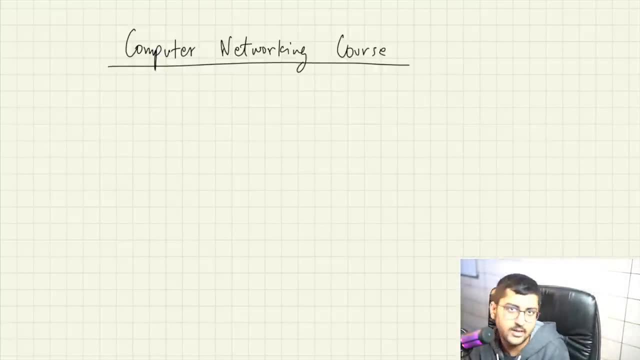 So for that you can also find the links in the description and then you can clear any fang interview with that preparation it's free everything is free so make sure you check it out. 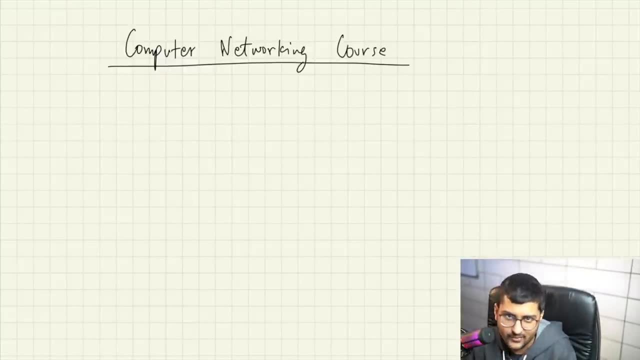 All right so we talk about like computer networks right what does it mean what do we mean by computer network in the in simple terms it's just computers connected together right that's it someone in my college also if they ask me some technical definition or whatever right oh no you know that movie three idiots it's a movie Bollywood movie. That's it. 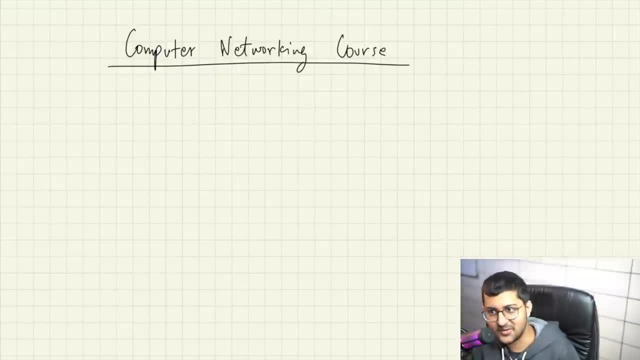 They ask what is a machine and that guy literally like says a lot of things. I have never been that guy I could not care less about the big big definitions okay what is computer so there's a computers computer also has a full form if you didn't know commonly oriented machine particularly used for training education and research that's the full form 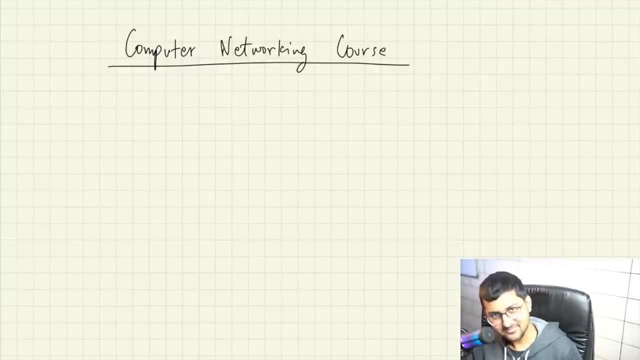 of computer I memorized it because in my high school my teacher they used to ask us this thing every day. So. 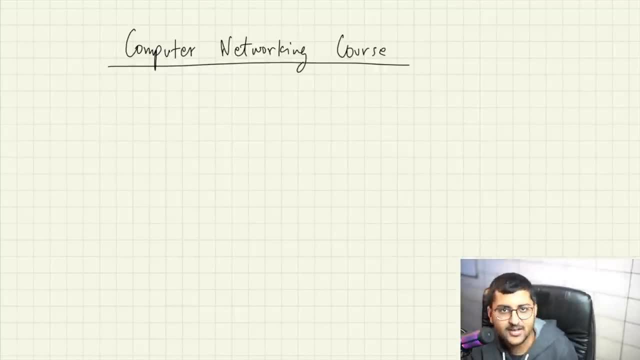 Anyway what is a network computers connected together that is a network no problem that is a network right then what is the internet so internet is basically a collection of these computer networks okay so my computer is connected to my sister's computer her computer is connected to someone else's computer and our computers are connected to like you know the wi-fi or whatever and that is connected to other people's computers and sort of like this these this connection of computers connecting with computers this connection is basically spread across like. 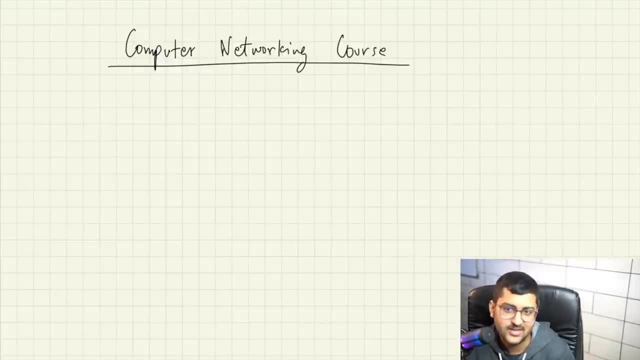 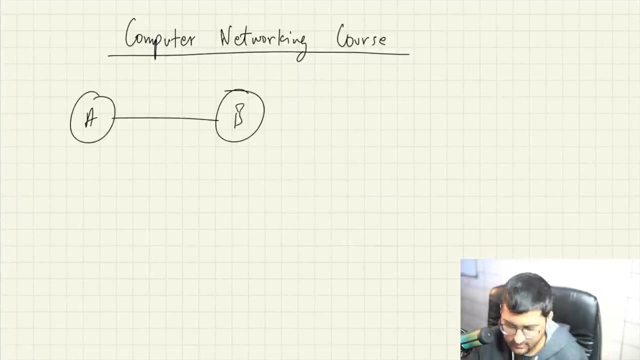 Houses cities countries so on and so forth so this entire connection on a global scale it's known as the internet okay so I don't think I have to draw anything about it but this is a network computer a connected to computer b okay if this is like spread across a large region or country or whatever you know everyone connected to each and every one of these. Whether like whatever like this is the internet okay so internet is a complete collection of computer networks let's look at like we all know this right we all know what computer is we all know these basic basic definitions and everything but let's look at what do we actually mean like how did it start and how are they actually connected that is what we are going to be focusing on this course let's look at how it all started so let's talk about how the internet started. 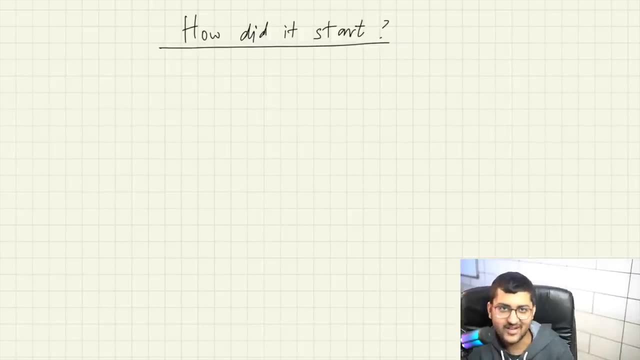 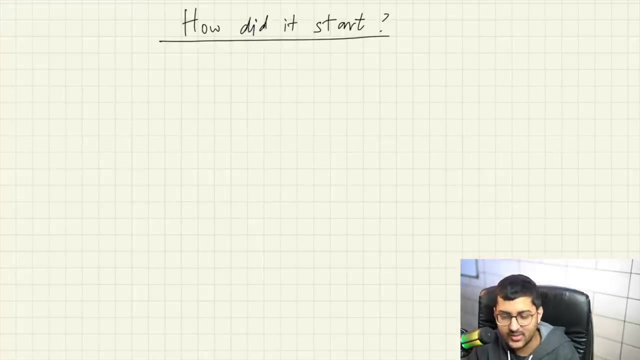 Let's go to you know the very beginning of of this era so what happened was that the cold war was going on and there was the united states and the the soviet soviet union and they they were like battling with one another like who is going to be the very first okay so when it came to you know launching the world's first satellite so the united states and you know the soviet union you know the russia they were like hey who is going to launch the very first satellite. We want our names to be written in history for example so russia won the soviet union won they launched sputnik in around 1950s somewhere 1957 to be precise so that was the very first satellite but now the u.s were like okay this is not cool we wanted to be the first how so what do we do how do we not miss out on further opportunities like for example we want to be the first to you know step on the moon we want to be the first on this or that or whatever right. 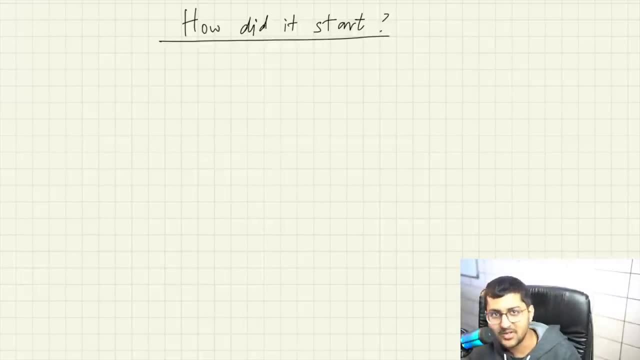 So u.s was like okay this is not cool this is not working we wanted to be the first so the u.s government they created a a program ARPA so ARPA is known as advance research projects agency okay so they were like hey you are supposed to you know do all the scientific discoveries and keep our country number one. Okay so what happened was that ARPA you know they they wanted to like have some sort of a way. To communicate with each other okay so ARPA had like facilities they had their buildings or whatever okay so they had their buildings in various parts of the united states okay but they were like hey how do we communicate with them it's becoming very difficult you know buildings are so much far far away from each other so they developed something called the ARPANET okay so ARPANET was basically there were like four four places where these computers you can say were. 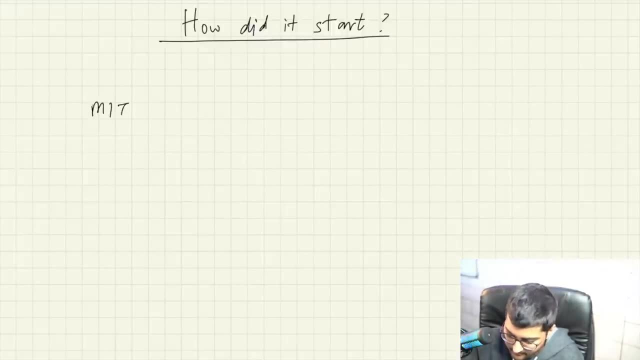 First was ARPANET. First was at like MIT okay second was at like Stanford third was at I believe UCLA and there was one more University of Utah okay they were like connected to each other or whatever okay something like that so now basically this is what they had so they were like hey we can now communicate. 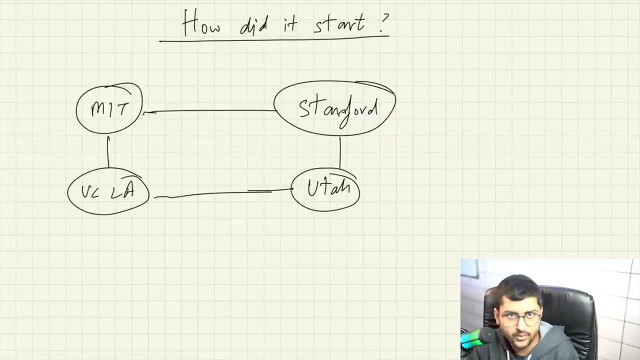 With one another you want to send some files or whatever you know whatever you want to do you can do it. 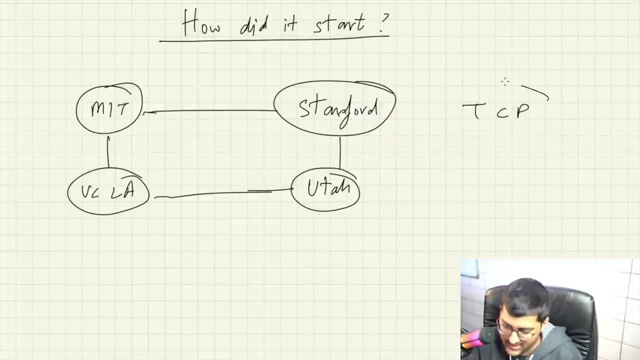 They were using TCP for this transmission control protocol what is TCP it's a very important topic TCP IP IP addresses UDP and you know file file the how simple mail transfer protocol all these things we'll be covering in detail okay so don't worry TCP. 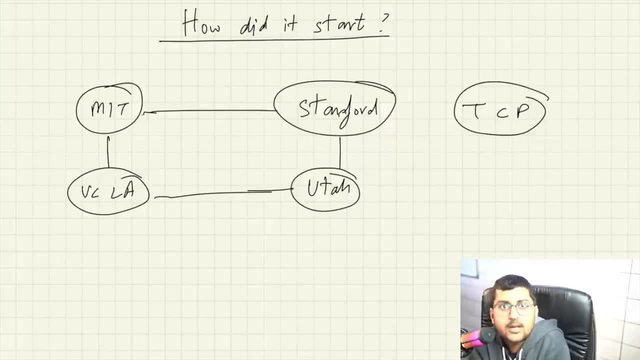 Forget about what TCP is let me tell you what it like what what do we mean by these protocols and stuff. 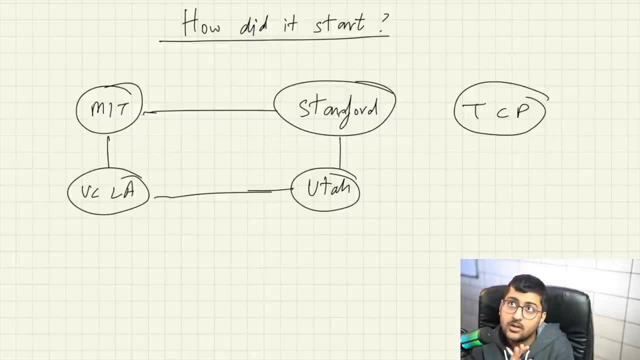 So basically in simple terms you are sending an email to someone okay they that may require some steps obviously I'm sending an email to someone it will require some steps like hey first send this email over here then send this email to that person they will then download it from the server and then they will read that email or whatever that will happen okay 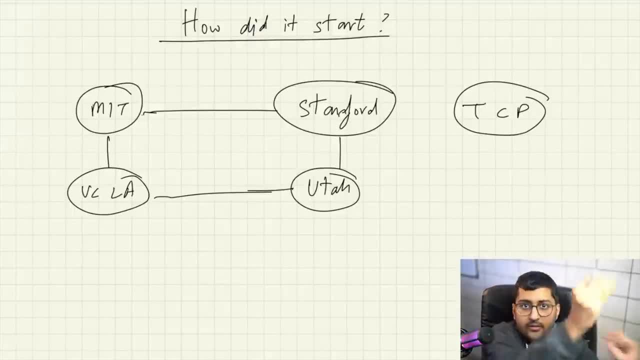 you want to talk to your friend okay so you're talking to a friend hey you connect with a friend. 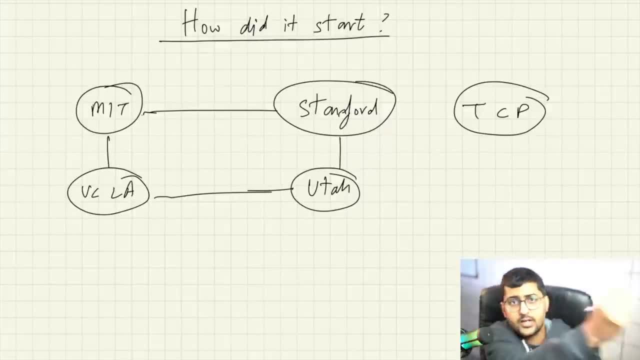 Then you take a establish a connection then you send your video they receive your video they send your they send their video you see the video and you're talking on video conferences 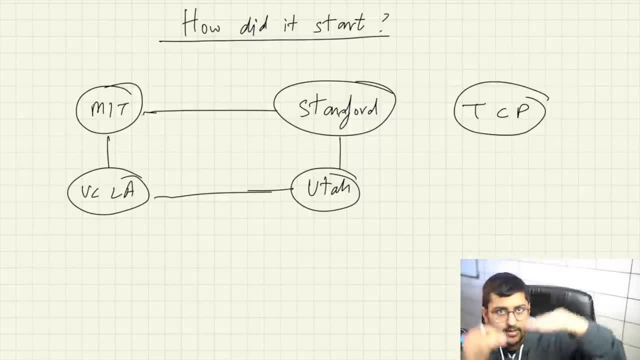 and some of the frame rates drop or whatever happens when the network is not stable right you want to send a file that is very important and you don't want anything to be removed from that file while it's being transferred okay you're like hey I want to send these special secret documents and obviously all the data has to be sent no data should be lost. 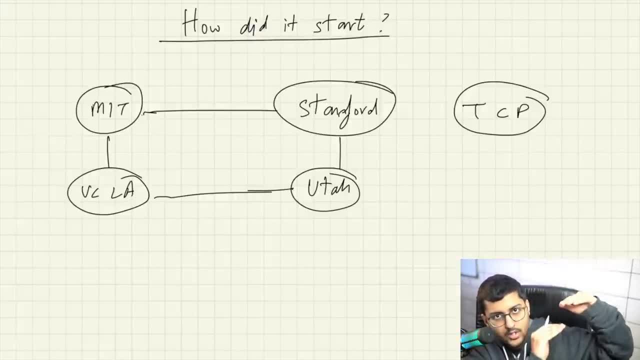 Okay. So this is what you can see different type of things I am trying to send over the internet make sense email video secure files so many things different types of things I'm trying to send over the internet so different types of rules will be required okay there might be some rules set by someone hey if you're sending a secure file the internet should make sure that hundred percent of the data that you have sent to your friend will be delivered if you're video conferencing with your friend then the internet can drop a few pictures or frame rates because it does not matter that much okay so these rules that are set up by people how a particular data is being sent these are known as protocols similar there's this TCP protocol IP protocol UDP so many other things okay now you know what TCP IP UDP and stuff the category is individually what it is we'll look into later on. 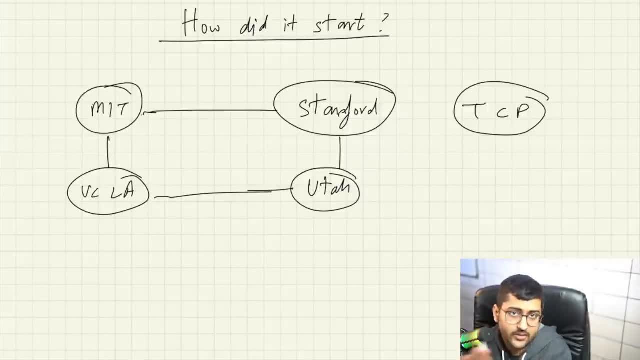 What is the difference between TCP UDP how email works and everything else okay sound good so this was like the very first computer sorry internet stuff okay cool this organization 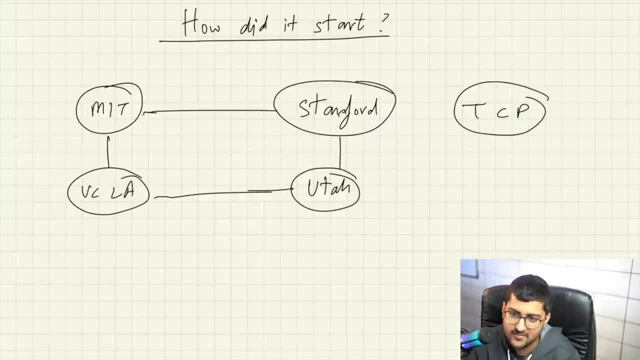 is still available like they're still like they have been renamed but they are still in practice okay so that's basically about it and after that you know as years years progressed more and more in more and more computers were added more and more computers were added more and more locations were added to the ARPANET and that's it yeah started falling like TCP IP just write IP over here as well that's it okay as simple as that so right now we are in the very early stage of the internet it does not have like really with like consumers or what it's more like research focused okay you're only able to talk to one another like this okay via some protocols we still use like TCP IP. 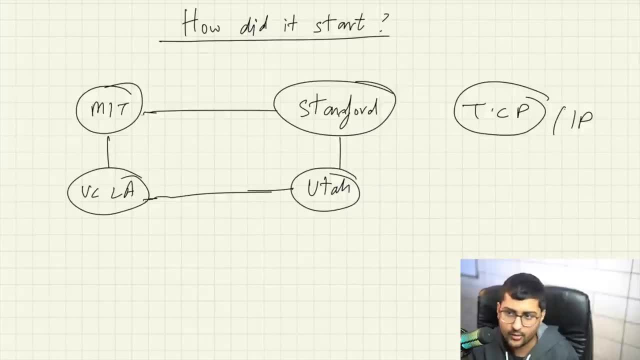 Okay. But how it has changed quite a lot let's look into that okay cool so one problem happened was that as this was a research project many people wanted to share their like research papers and stuff which was not really working in this particular domain okay so basically 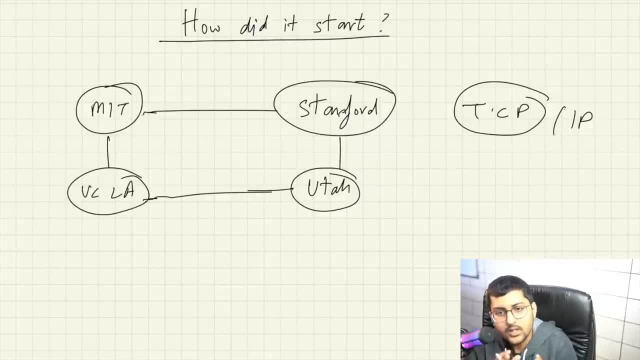 the idea was that I want to be able to share. Okay. 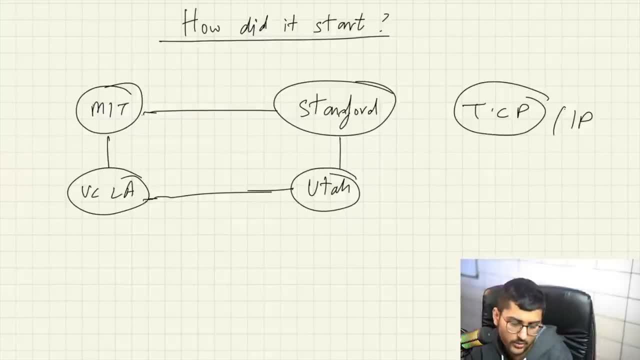 Some documents that reference like some other documents or whatever okay so what happens is that I want to send a research paper from MIT to Stanford for example this is a research paper it has a link in it this link is linking to another research paper okay so this automated sharing this was missing previously. Okay. 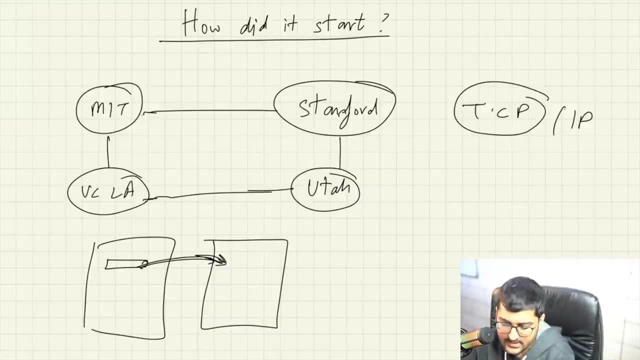 So if someone is like hey MIT has sent me a document on about something like you know apples or something and there's some other information about apples in another document I need some sort of a way that I just click this link and it will point me towards that document then that research paper or whatever comes into picture www the world wide web you must have heard of it. Okay. You must have heard about Tim Berners right so Tim Berners you know developed the world wide web okay so world wide web is a project that basically stores these documents okay okay you can store and you can access these documents via the world wide web all right you can actually check out the very first website that was created as well let me show you. Okay. 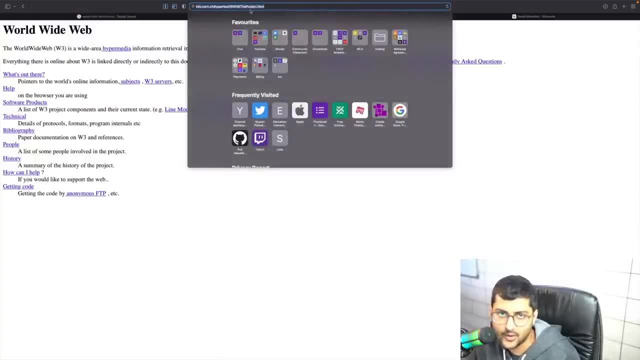 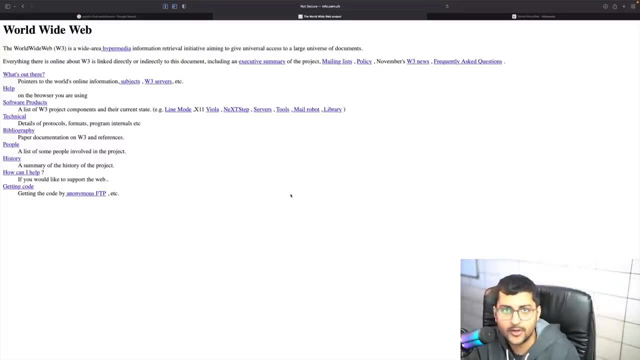 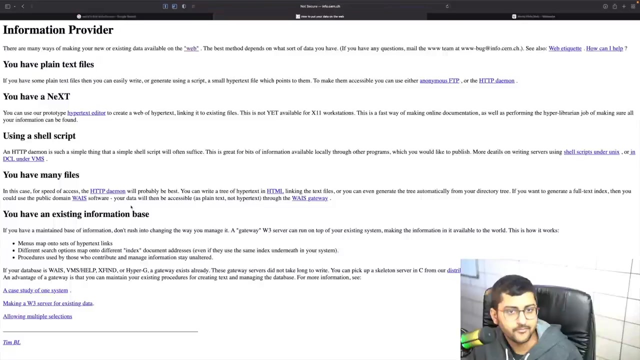 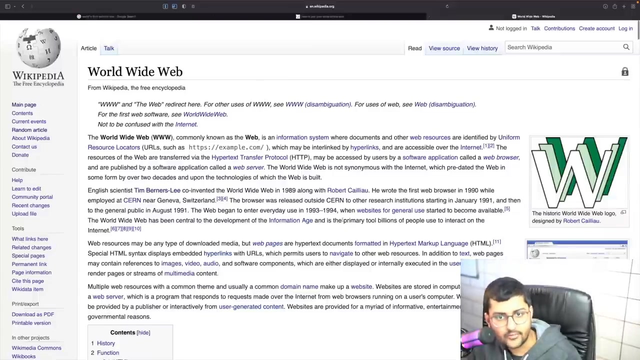 So the first website is info.cern.ch slash hypertext slash www dot project dot html so don't confuse yourself with world wide web Kunal what is world wide web where is it stored okay whatever no it's just a universal like it's it's allowing you access to all these documents and it has all these links okay but click on technical how to provide data okay you have plain text files you have initial scripts and things like that. Okay. You have to make a server we all know we'll learn how to make servers and everything world wide web you can see on Wikipedia as well it's where documents and other web resources are identified by a URL a URL like this you know we all know about what a URL is which may be interlinked by hyperlinks there are so many links that are interlinked in this web page and they are accessible over the internet that's it that is the world wide web it's a collection of all these pages and everything. 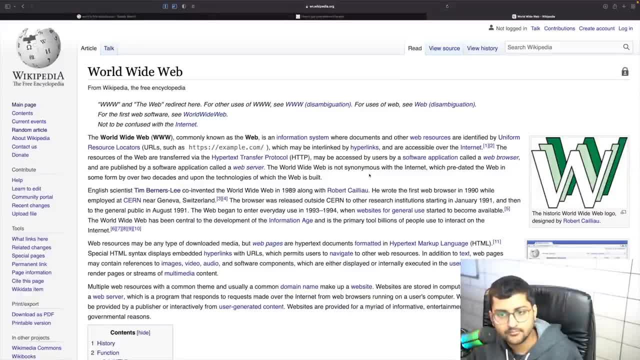 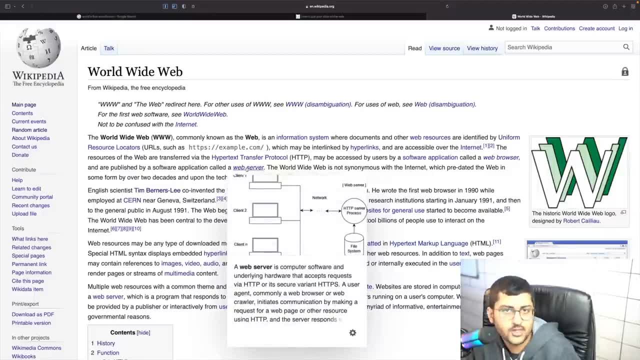 Okay. And it's published by web servers you can host your own server okay so now you know where this all these things stored on web servers how servers work we'll cover later 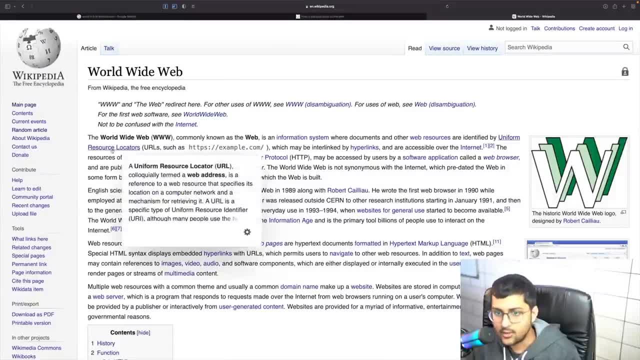 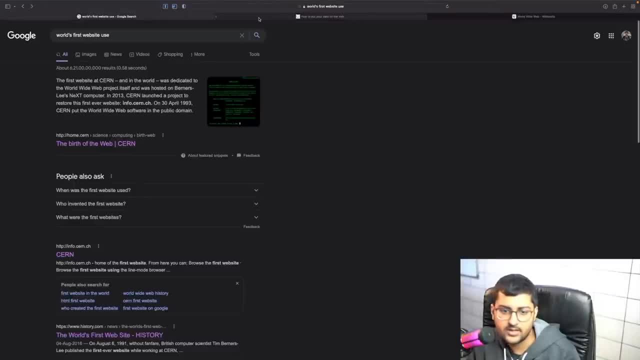 on okay so URLs and everything URL and everything we'll talk more about more about later but this is basically about it this was the world's first website. Okay. Okay. Okay. Let me just do one more thing. 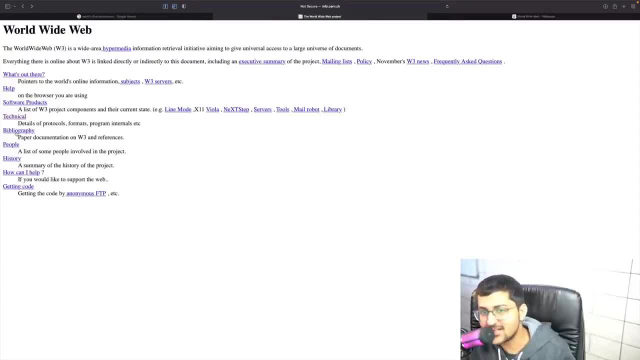 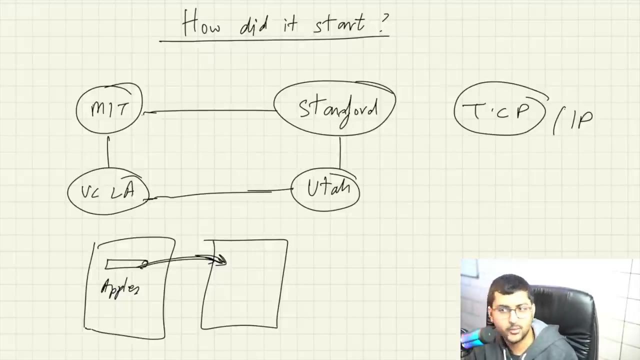 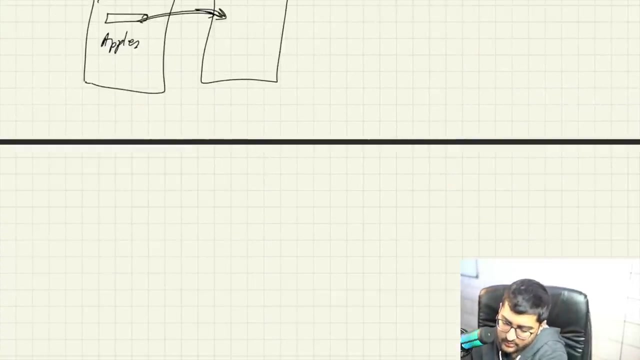 Here in this one here you can search for a website yeah. This is it but you will be like Kunal there's a problem here there's no search engine like how do I search for something if I want to search for something how do I search for it you can't you can't search for anything in this so this option was not available okay so to answer your question Kunal how did we search for things then you couldn't okay you just go to hyperlinks from hyperlinks you can you could save it in like some indices but it could not scale to like you know when there were like so many web pages here you coming up and things like that so in the end they had to develop search engines yahoo i believe was the very first one um but you can check out more about it like in the history of search engines you can go to wikipedia and you can check it out then we had search engines and now that's it that we are now you know in the history of internet now now a lot lot more things are coming up you know like web 3 and things like that and so so on so forth like i'm not sure like uh you know where we'll where we'll head up but uh but you know where we're going so yeah that's the modern internet now we have search engines and everything but that's like the brief history okay now let's learn about you know the protocols thing that i was mentioning so you might have a question 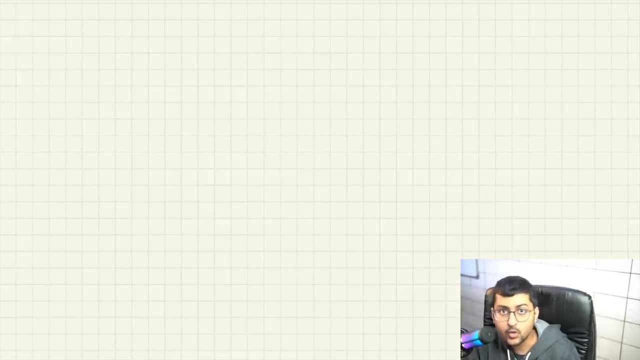 why even we want protocols why do we need these rules you know so imagine you are making an application okay and someone else in some other country is making an application you have some different rules about how your 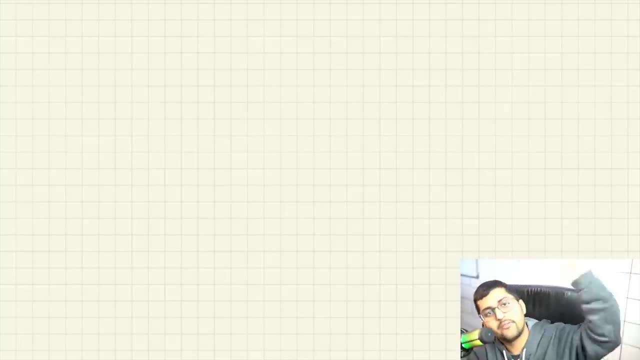 application can communicate with some other one's application they have a different rule like i will connect connect communicate with another applications in a different way so can you really communicate with each other no no you can't that is why it is extremely important to have like a set of rules and regulations okay so these rules and regulations 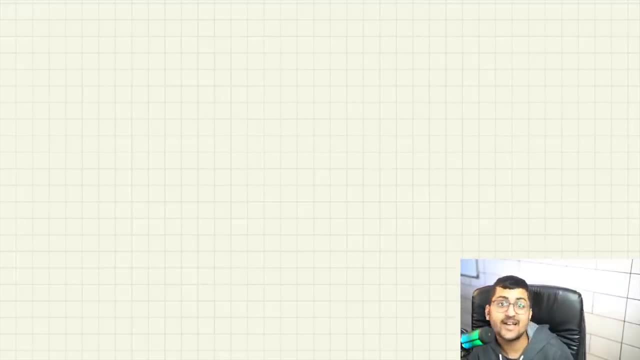 who writes these i'm talking about i want to send an email okay so every single person who sends an email to another person across the world you know have their have a that email is being sent using a set of rules and regulations 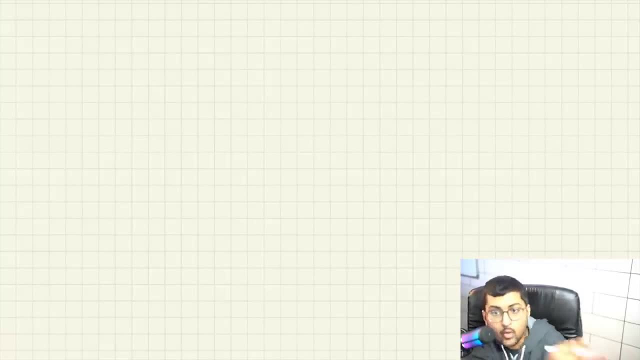 okay first this will happen then this will happen then this will happen but who made these rules who controls these rules who creates the new rules the internet society right now i'm just telling you all the cool stuff but uh how it works how the every step happens that we'll cover later on okay so the internet society as you can see over here uh this is the internet society and they are the ones who are responsible for all these things 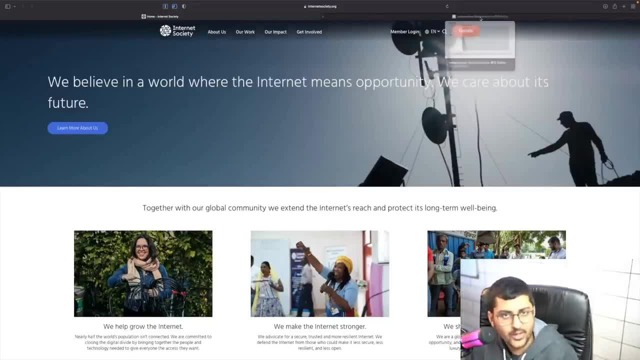 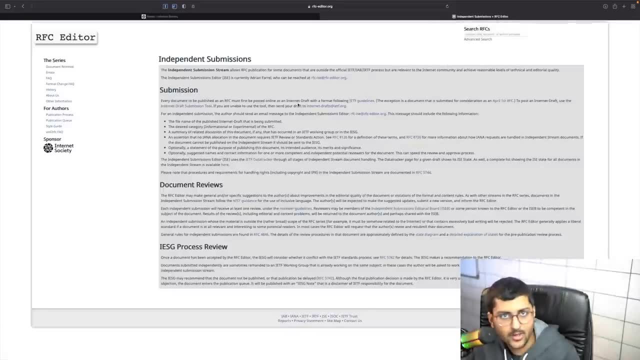 okay so how do we actually make submissions we can do that by a rfc rsv means i believe request for comments okay so you can set a document like hey i have this idea about some feature of the internet or whatever you can please you know check it out so you can submit it on on this page it's usually submitted by you know you know very high professionals or whatever but anyone can submit and submit until there is 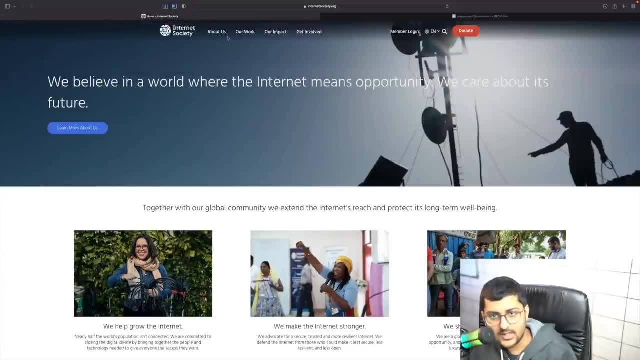 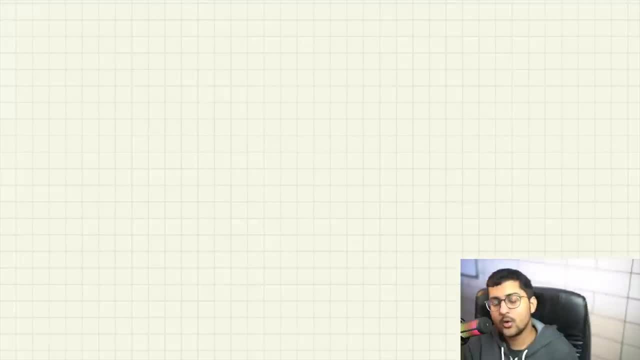 or they have like you know like till they have an idea okay so the internet society comes up with all these rules and stuff you can learn more about them over here internetsociety.org 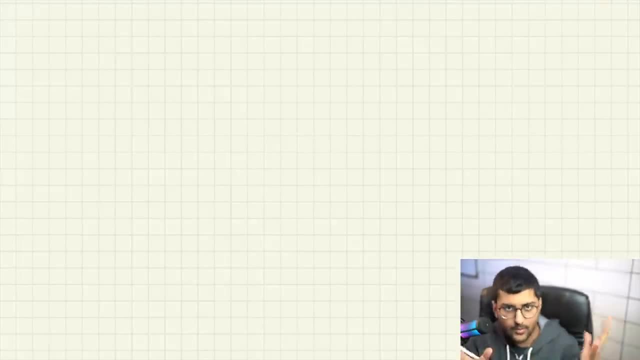 okay so now let's talk a little bit more about some technical terms we know like how internet started now and everything but now i'm mentioning about these protocols right the protocols and how the like we know what is happening but we don't know how it's happening like i know what the internet is how it started but we still don't know what the internet is 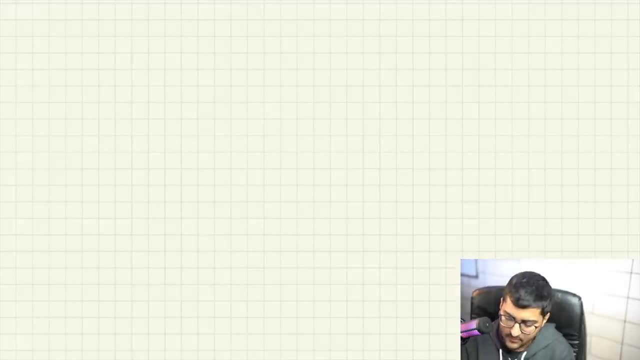 we still don't know how it works so before that let's you know cover a few terms and stuff so you may have heard about servers okay what is a server you may have may have heard about a client so what is a client so example you have your computer right this is you you have your computer and you write here google.com okay you click enter it sends a request to the google server and google 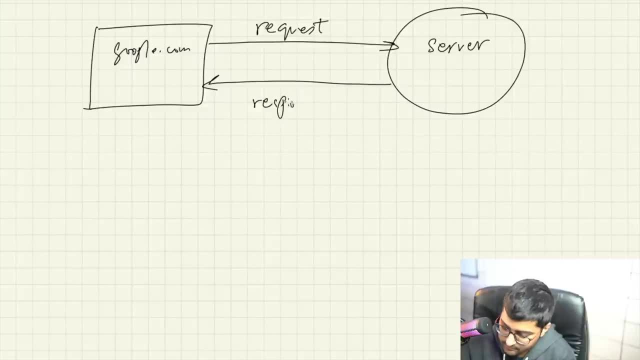 sends back a response to your computer client server 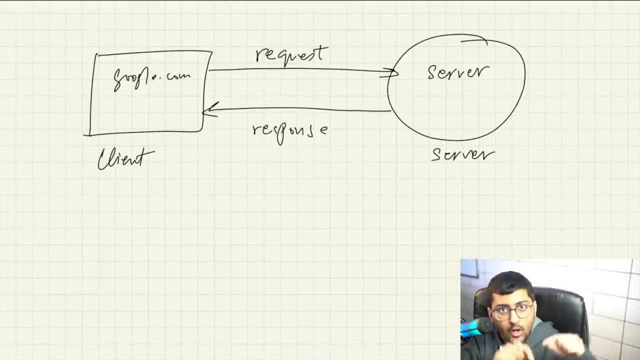 okay you write google.com again this is a very broad explanation every single deconstruction of it like a deep dive of how this is happening internally what are the actual steps that are being taken and i will actually make the picture clear in your mind how the internet works okay 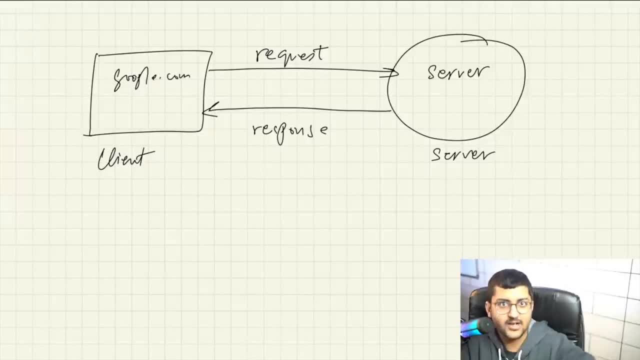 a little bit of a spoiler alert you know these various countries and various continents across the world we are connected via wires these wires are laid underground yeah under the ocean that's how we are literally connected so internet is not like in the cloud it's actually under the sea i'll tell you more how these things work internally later on but the simple idea is right now let's focus on what we are doing okay then i'll talk to you talk you 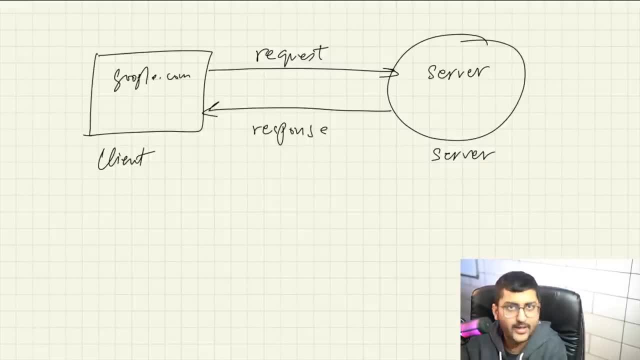 talk to you about how we are doing it so basically you write google.com okay google it it this basically your computer sends a request to the server google server okay and the server gets that response server is like okay i got your response uh i got your request here's what you wanted there you go take all these uh take all these 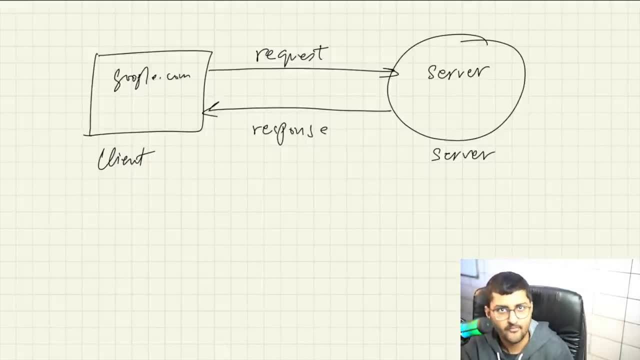 things it sends back a web page and a bunch of other things a response is sent back to you 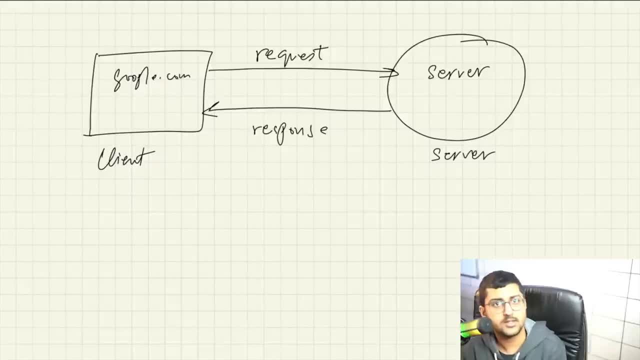 okay so does this mean that you cannot be the server yourself when you're like your 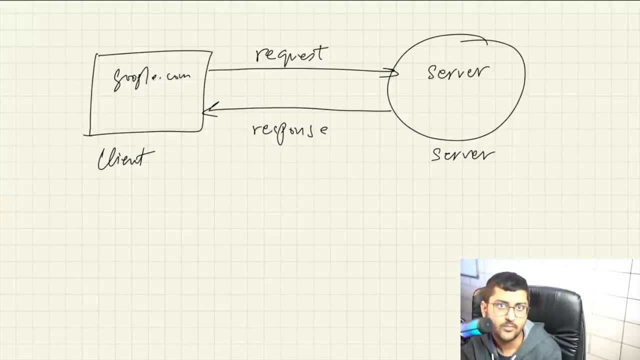 own computer cannot be a server it definitely can be okay that's known as when you work on local host and stuff 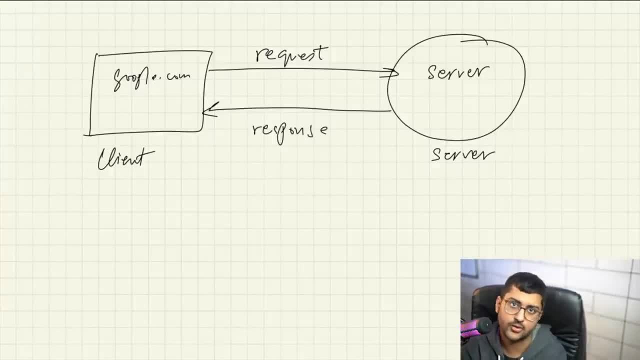 okay so your same computer can act as a server also and a client also okay let's just give you an example of this okay here let me write google.com 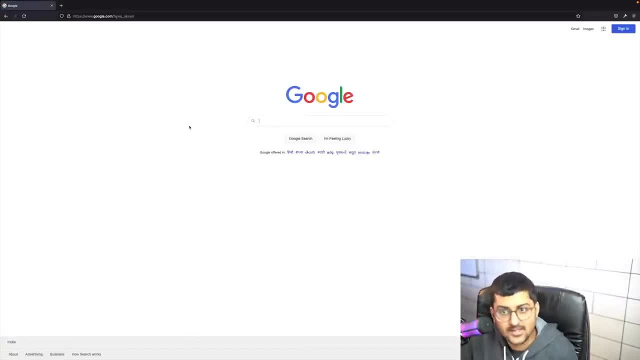 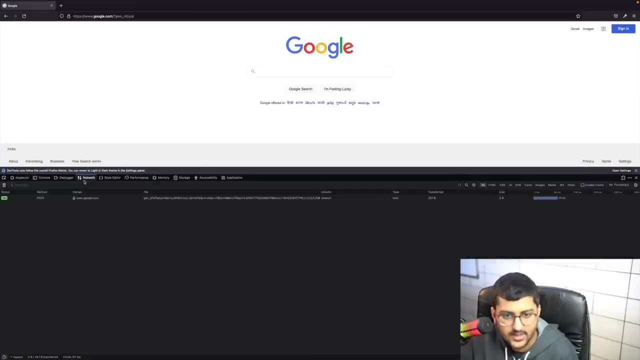 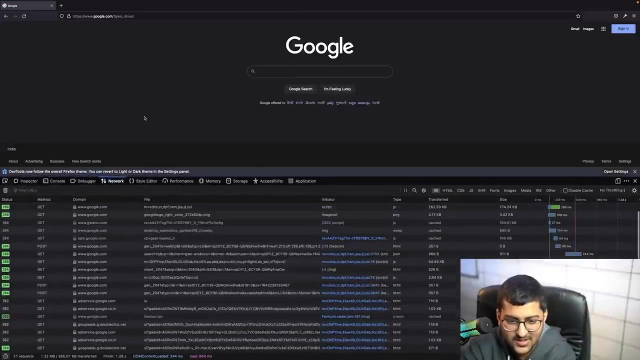 web page loaded how what happened so there's a bunch of things inspect tell him inspect so inspect basically shows me all the things network and refresh so many things happened okay in this one request these many things happened 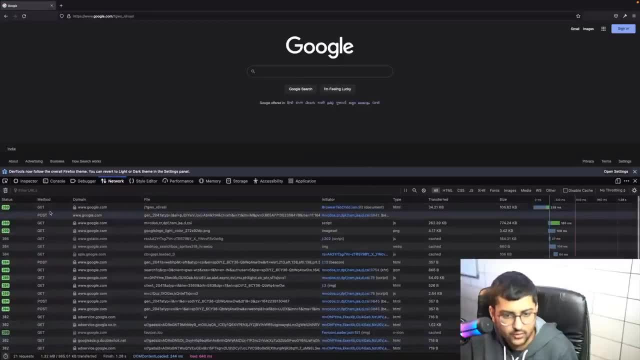 okay a get request was made and get request was made and so on and so forth and these are all the things you know like status 200 means everything is okay and everything so you got like html uh and uh you got like j some javascript and png and html json files and so on so forth so 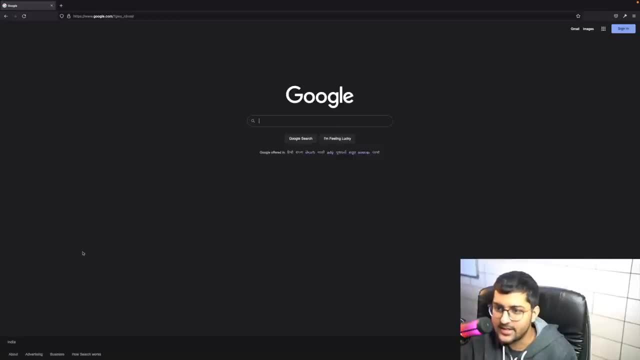 all these things we got back from google and it created this web page okay let's do a deep dive into this like how this thing is working and how google.com gets resolved to ip addresses 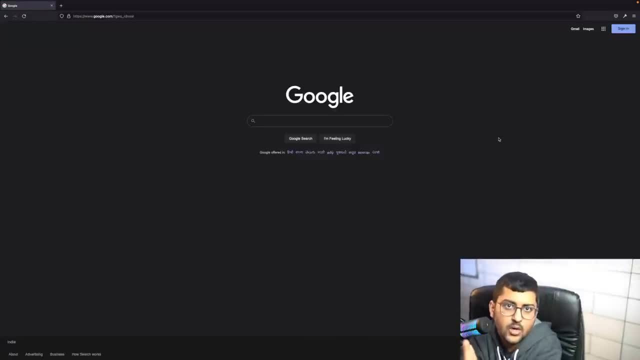 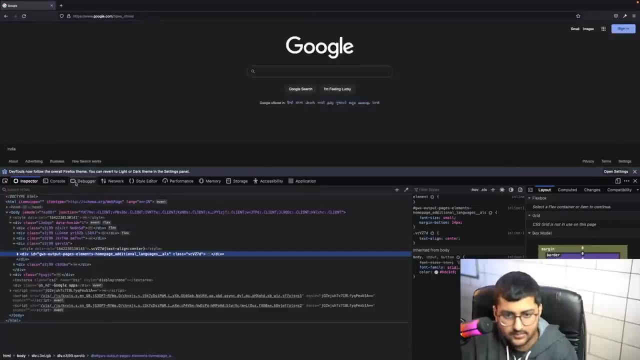 or forget about ip addresses let's talk about what are ip addresses okay what are these protocols and everything let's and what is this like status code what is this get what is this um you know post and get like if i refresh it you can see there's get there's post what is this method 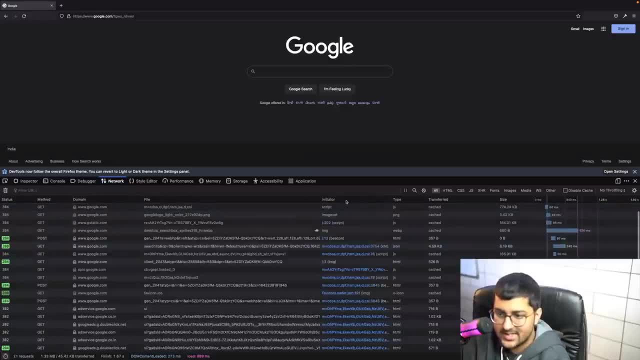 what is this get do is get here what is this and it's the rest of the gas printing states these are you what is this domain, what is this status code, what is this indicator, initiator, what is this type, and what does this mean by like this transferred, what is this B and KB, what is this size, what is this thing, what are these milliseconds, everything will cover. 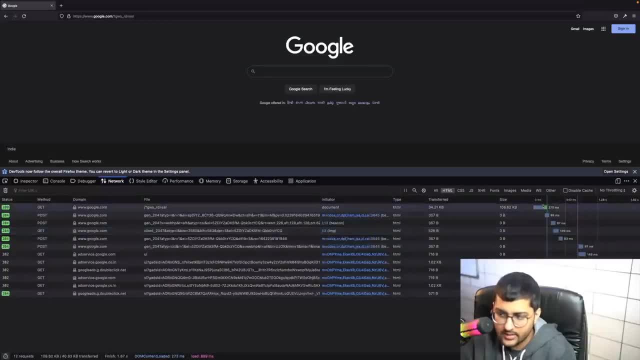 Okay, so if you wanna see all the HTML that we got and everything, and you can see like what is this thing, everything will cover right now, okay, so let's do it. 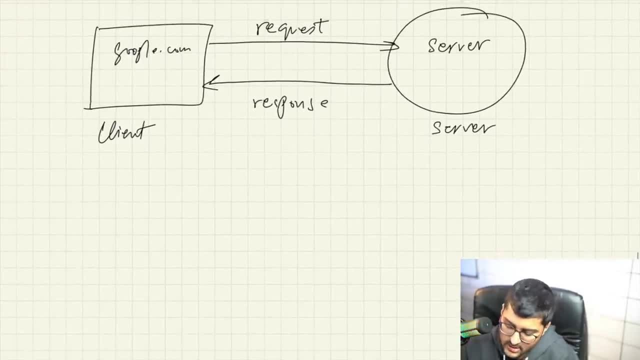 Okay, so before that, let's talk a little bit about protocols that I mentioned previously. 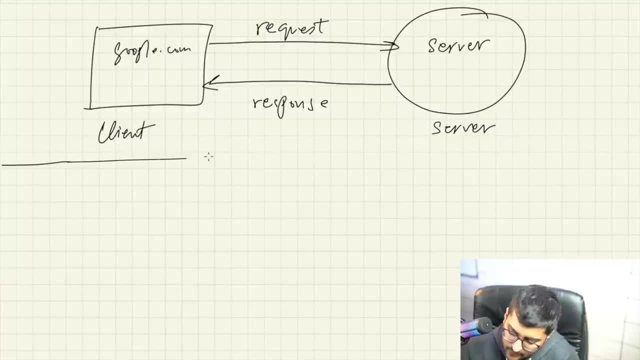 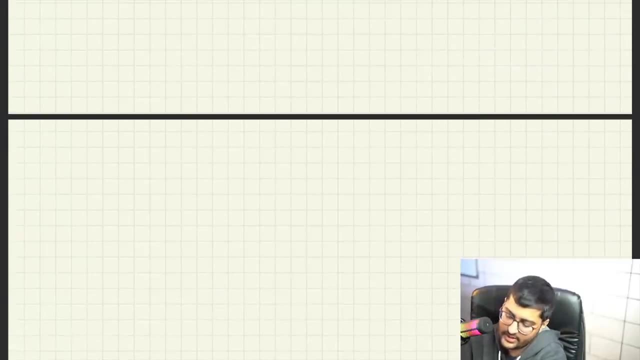 So what are protocols? Protocols are just rules that are defined by the internet society, okay. They're like, hey, these are the rules, this is how data is transferred and everything, okay. 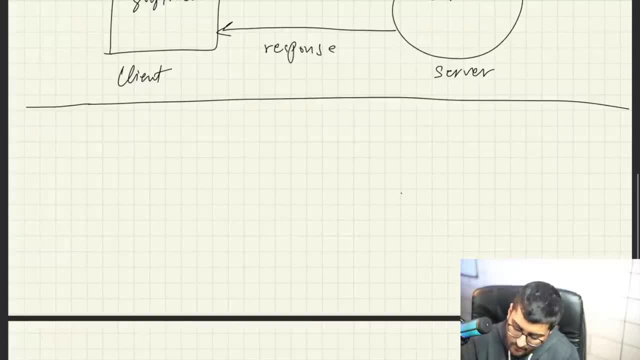 So there are some like basic protocols. There's like TCP, which we'll look into details, okay. 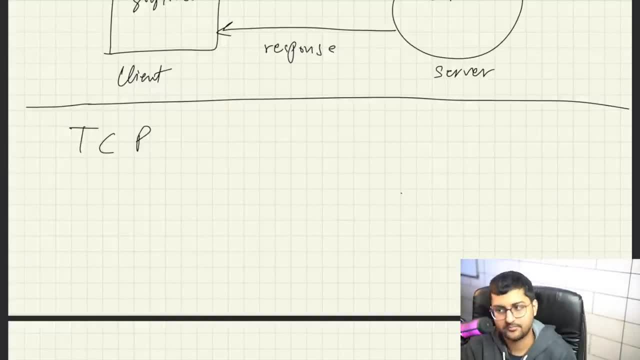 So TCP is known as transmission control protocol, okay. So the idea is that it will ensure that the data will reach its destination and it will not be like corrupted on the way, okay. 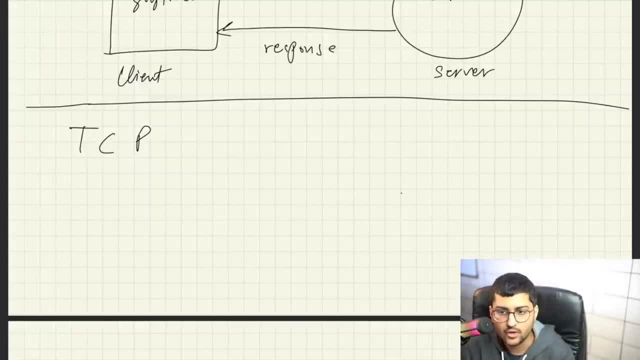 So there's something you definitely want the person to get completely, you should use, it will be using TCP in your applications, okay. 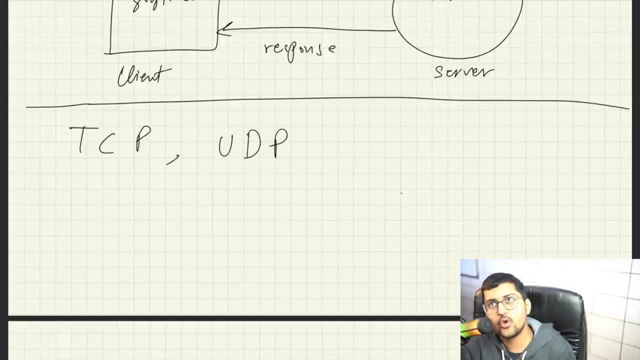 There might be another examples like UDP. So when you do not care about if 100% of the data is reaching your friend or not, whomever you want to send the data. 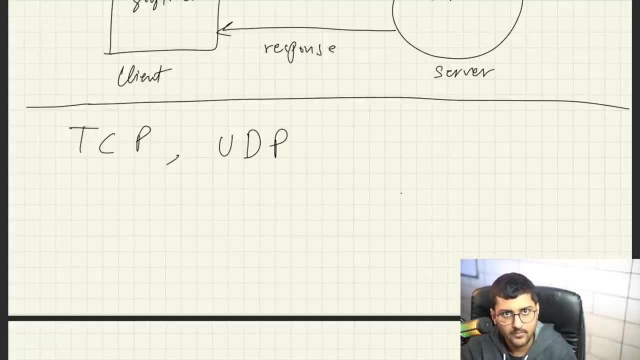 For example, video conferencing. Okay, so not all data may be reaching and that is totally fine by us. Another one is HTTP. 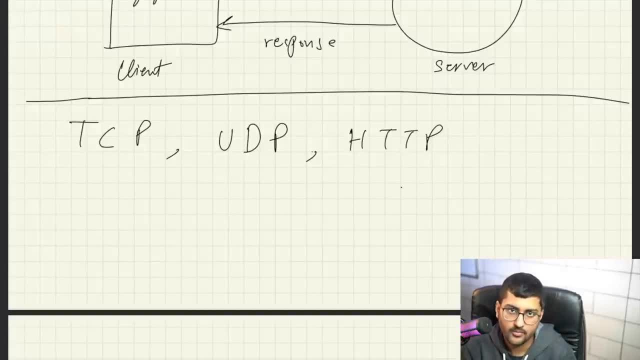 UDP means user datagram protocol. The next protocol is hypertext transfer protocol, okay. 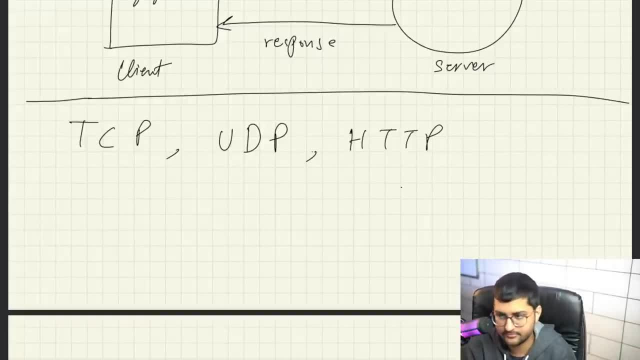 This is being used by web browsers, the worldwide web, okay. So it basically defines the format, okay, of the, you know, the data that is being transferred between your, like, when we talk about WWW over web clients, basically and web servers, okay. 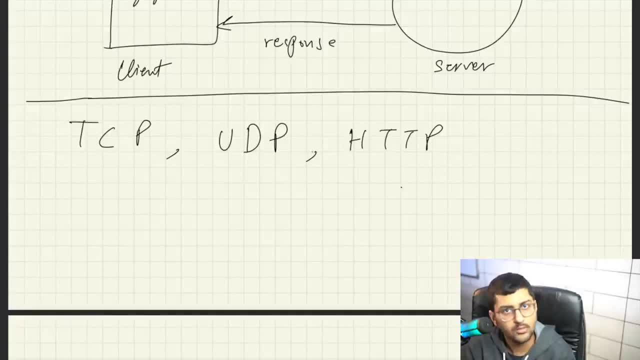 Clients and servers. Okay. Cool. 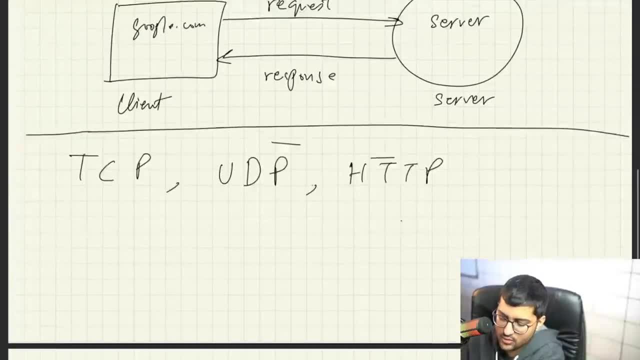 So when a client over here in this you can see, sends a request to a server. 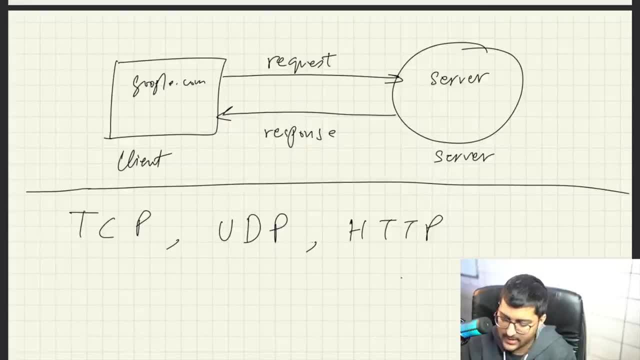 So, these particular things like clients send a request to a server. Server will send something back. server will send something back. 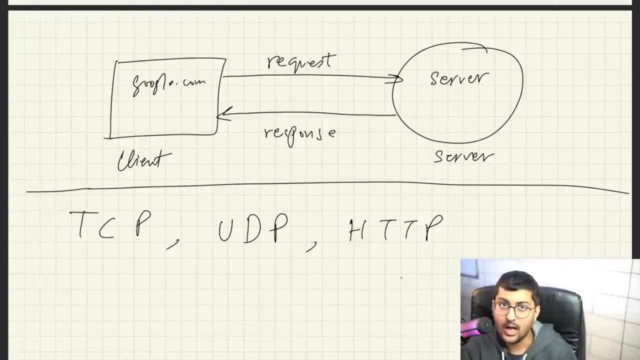 things are given inside http how the server will send back the data that is also a rule that is given in http okay we'll talk more about that later http https and everything okay cool so 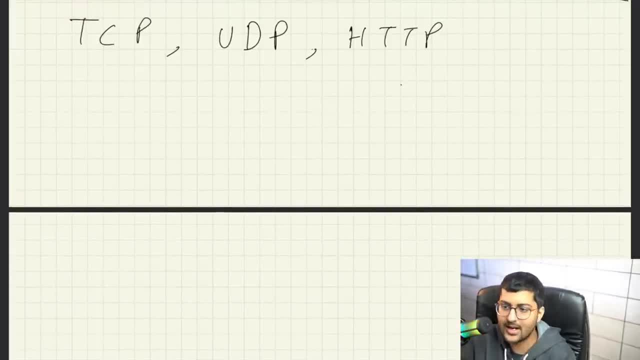 it's basically about it but don't worry we'll go into details of it as well like how it works and everything okay okay one more thing that we'll cover later on and i'm just giving you a brief 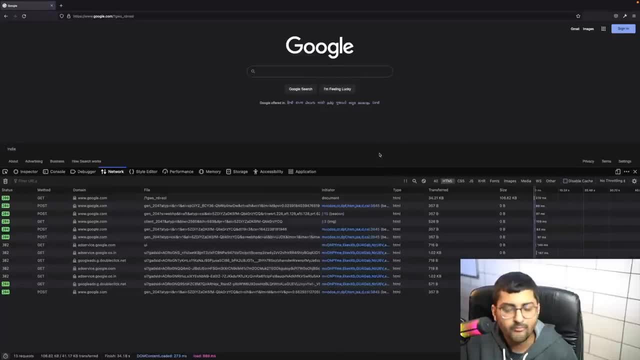 about is how data is transferred okay um you know everything in online is like uh in computers everything is zero and one okay so it's it doesn't make sense to send the entire data at once 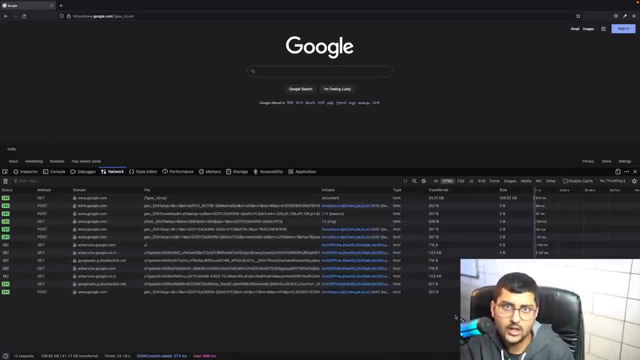 suppose you want to send a large file over the internet do you send the entire file in just one single go no it comes in chunks isn't that correct same things happen with these sorts of things like when you're loading a web page watching a movie online or whatever 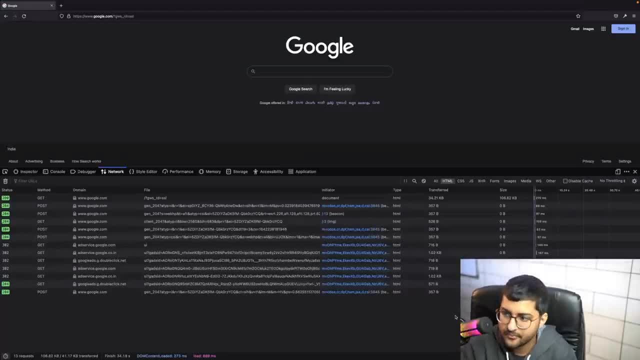 you're sending a large file over the internet and you're sending a large file over the internet data you'll be getting will be in packets okay sound good let's refresh so you can see these 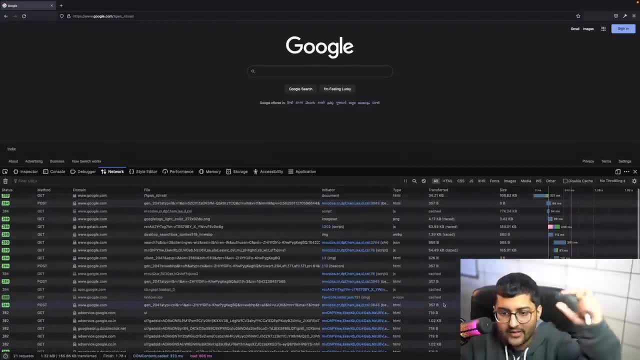 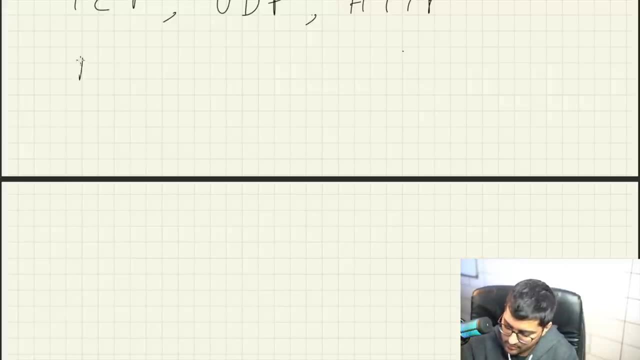 are like individual calls and you're getting different different packets of data all right okay so we have to cover about packets also packets are to be covered there's one more 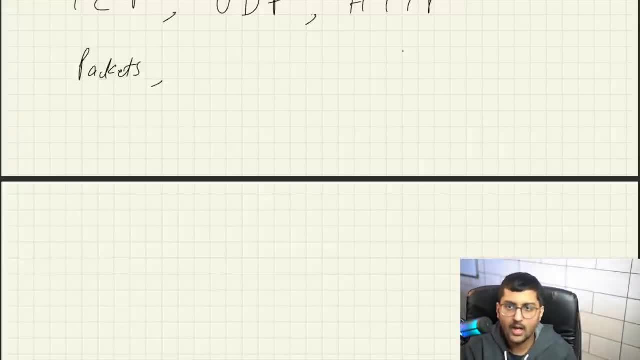 thing when you write google.com okay how does it fine which server to connect to or whatever okay so basically these computers and servers they are 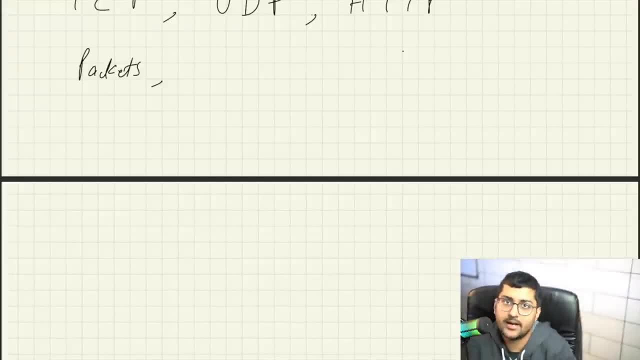 all identified via something known as an ip address so you can think of it as your uh phone book okay so in computers what happens is that uh sorry in like phone numbers what happens is you have your so many friends right you have let's say 200 contacts and uh when you call i want to call someone you just dial their name and then you have like 200 contacts and uh when you call i want to call someone you just dial their name 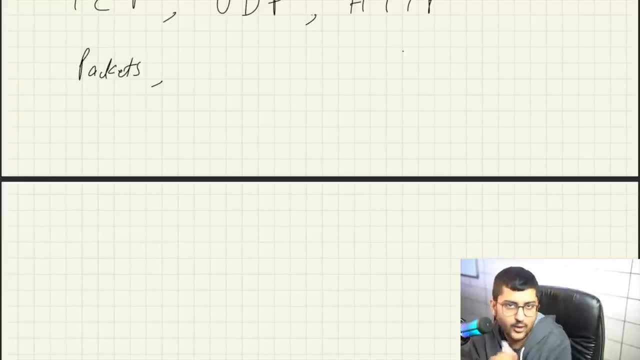 okay just like hey call mummy and it will call your mom okay or call sachin or someone okay anyone 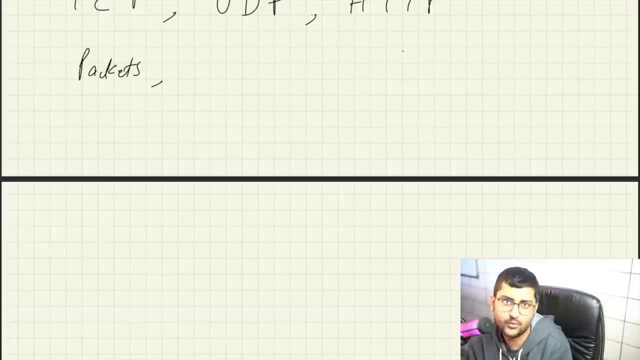 you want to call do you type their number all the time no so what is happening actual value is some number nine nine nine one one one nine something like that this is being linked to a name okay name 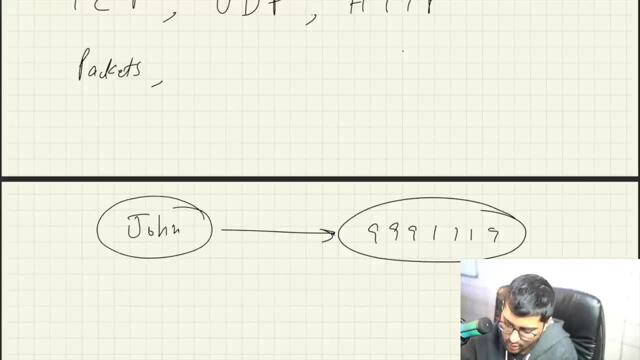 like john or something you want to call john you just call john and it will directly dial this number 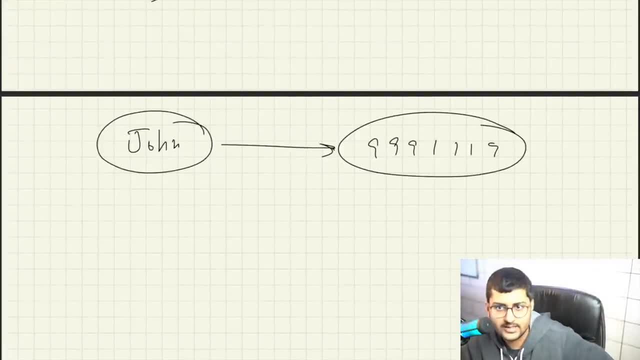 this is the same thing for ip addresses and stuff okay all the devices that are connected together you are watching me right now okay you are connected to youtube right now okay so youtube server okay you are interacting with the youtube server so every single device on the internet that can talk to each other they have something known as an ip address okay ip address for example 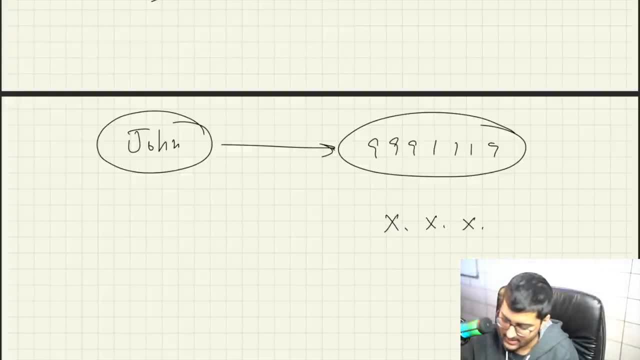 um x x x x this is a format and every single x can have the numbers from 0 to 255 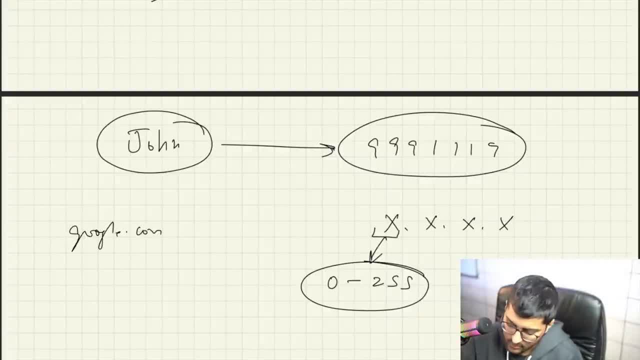 okay you write google.com it will be resolved to a particular ip address i hope it makes sense what is an ip address okay sound good 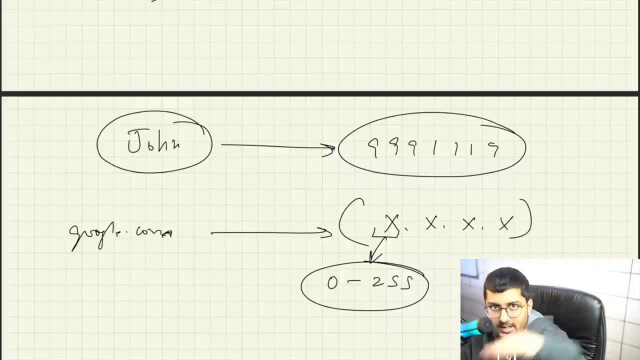 so we'll talk in detail about ip address they are like classes of ip address some are that are reserved for example okay that no one can use or whatever okay and how it actually like works cool 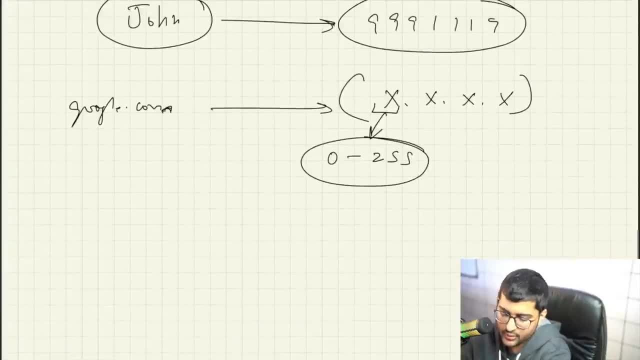 sound good if you want to check ip addresses of your own computer you can you can do that as well you can use the curl command and you can use like the command 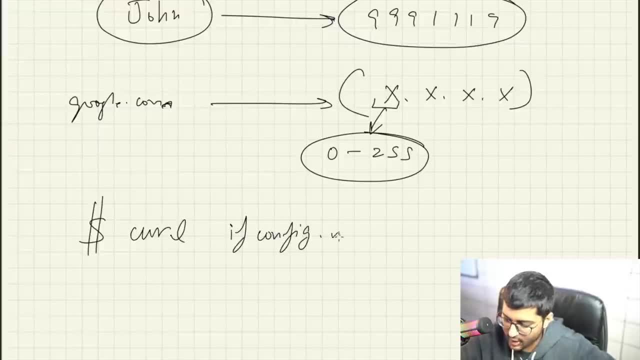 curl ifconfig.me dashes you can use this command it will give you your ip address of your um 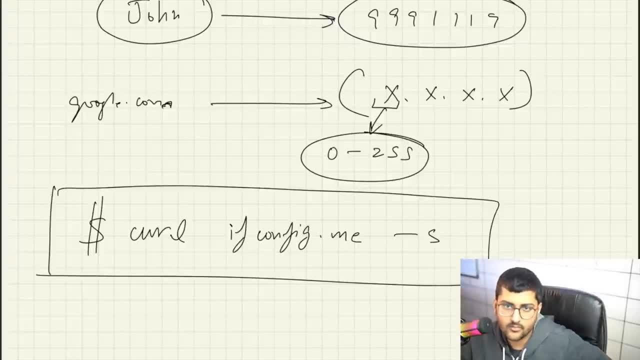 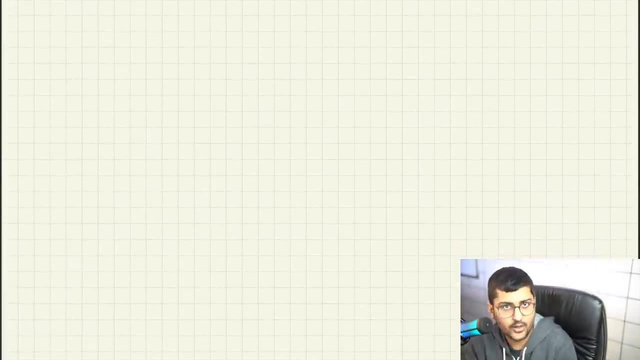 the internet internet provider okay so how does this work now do everyone have the same ip address or what is the ip address of my devices if my device is connected to uh if let's say you are at your house you have a router like a modem and a router and uh um you you you have like four devices connected to your wi-fi so all these four devices are they going to have the same ip address or different ip address or how is it going to work okay let's think about this this is how it 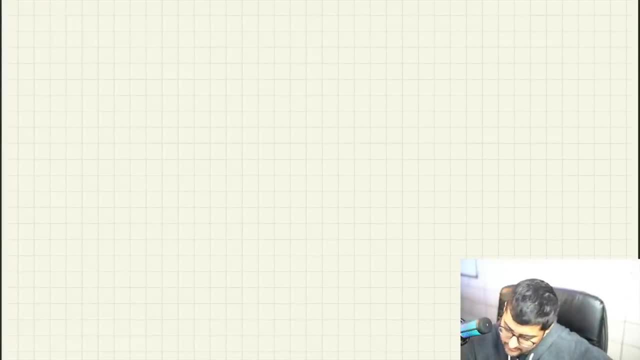 actually works this is your internet service provider okay mine is atl for example okay internet service provider okay your internet service provider gives you a modem or something okay your modem and router or whatever 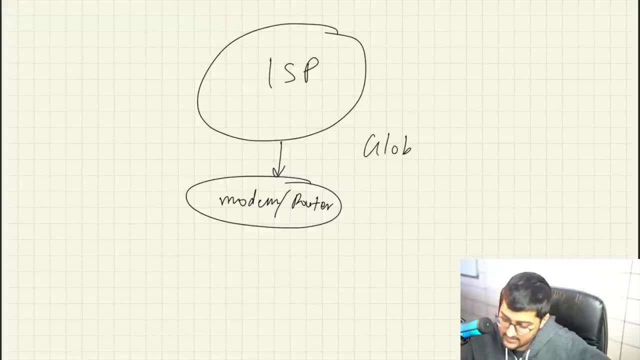 okay this is going to have a global ip address all the devices connected to this wi-fi modem are going to have the same ip address for everyone around the world 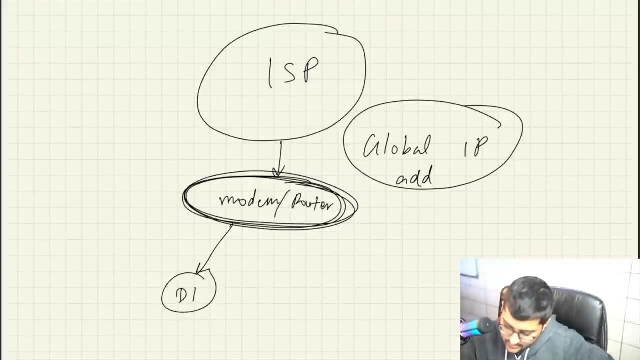 okay inside this modem device 1 may be connected device 2 may be connected and device 3 may be connected 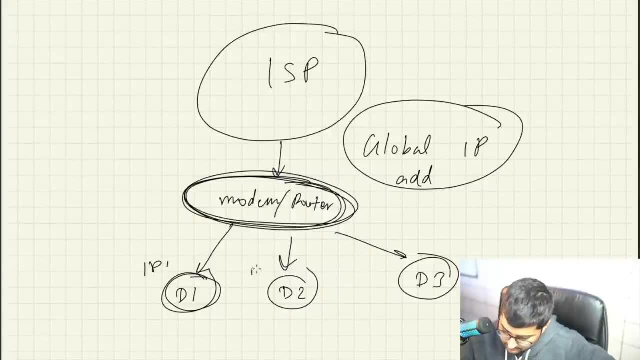 as well now i'll show you how you can give ip addresses to these as well 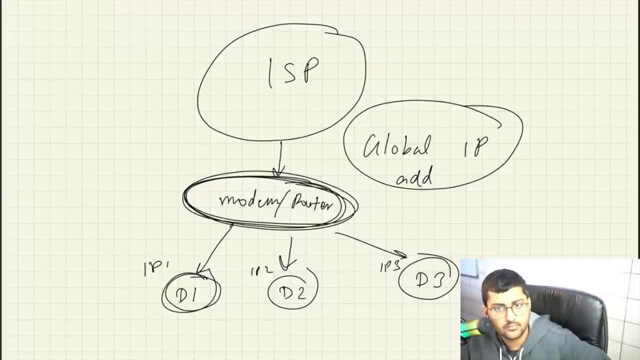 okay these are known as local ip addresses okay these are known as local ip addresses 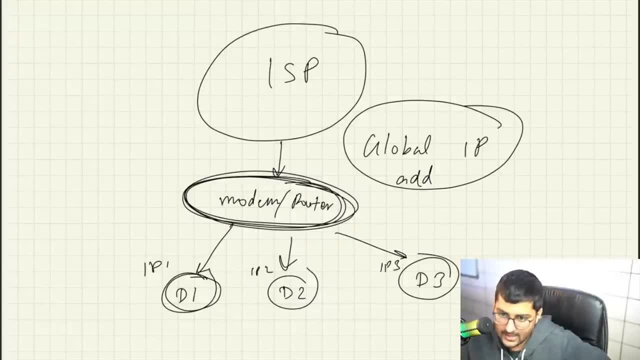 how does it do it dhcp dynamic host configuration protocol this is also a set of rules and regulations only i will talk to you about dhcp as well in like in the later of this course right 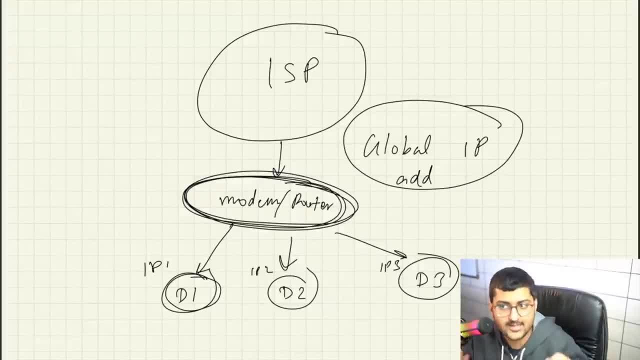 now i'm just setting the stage taking my time and just setting the stage we'll cover it in detail so modem and it allow it assigns these ip addresses using dhcp protocol 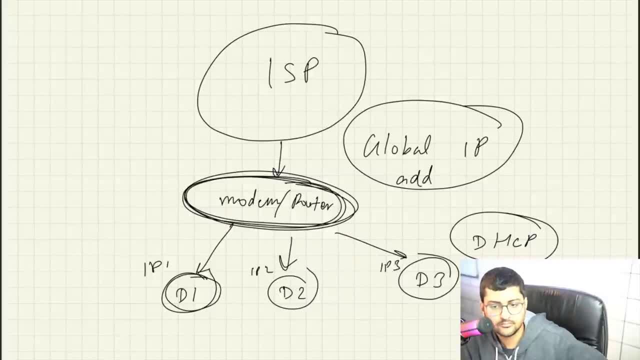 okay that's basically about it okay so this is a global ip address so if anyone wants to if you make a request to google.com google will actually see this global ip address 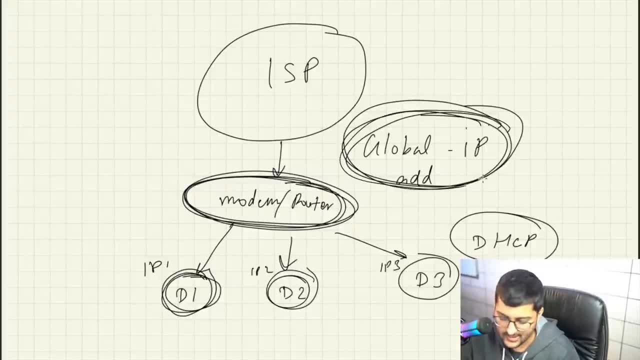 for google it will only be like okay this one single device is making a request okay cool 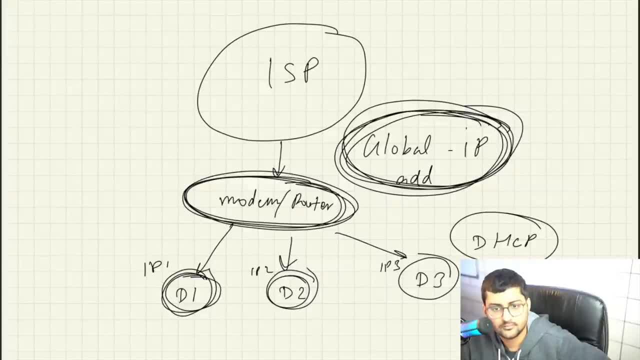 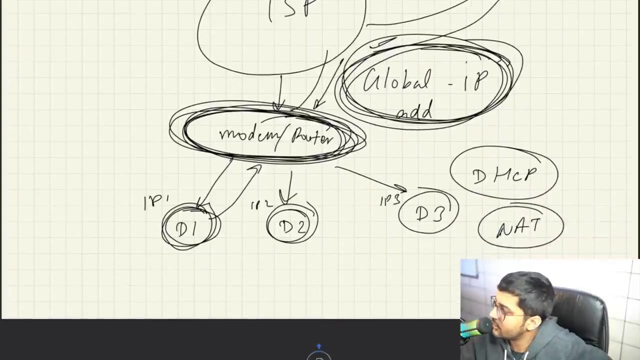 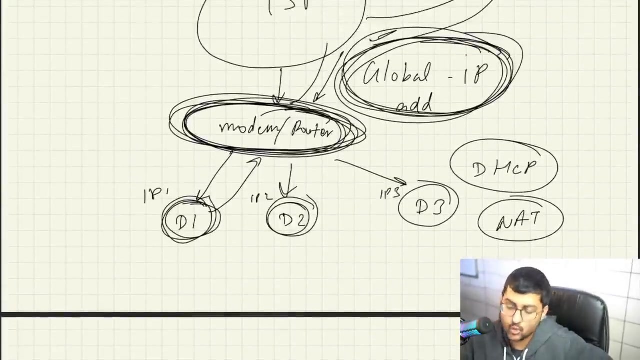 okay and when the request comes back from google so this is connected to the internet i'll talk about how isps work and everything later on so you send a request to google.com your isp will send a request to google.com okay it will return back the request okay now this modem is set up to be able to send a request to google.com okay now this modem is set up to be able to send a request to google.com modem will decide the router will decide who was the one who had the request was it device one device two device three it does that using NAT okay network access translator I wrote it down over here somewhere here okay so like a device one had a Google Chrome open on its tab and that is the something that requested 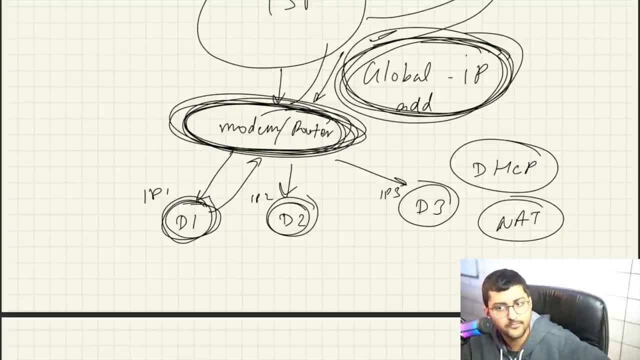 this okay sound good cool okay but now modem and router is like okay I know device one was the one that made a request but which application in device one made the request how do we figure that out you're running let's say Mongo DB you make some requests and you want data to be connected to the device and you want data to be connected to the device 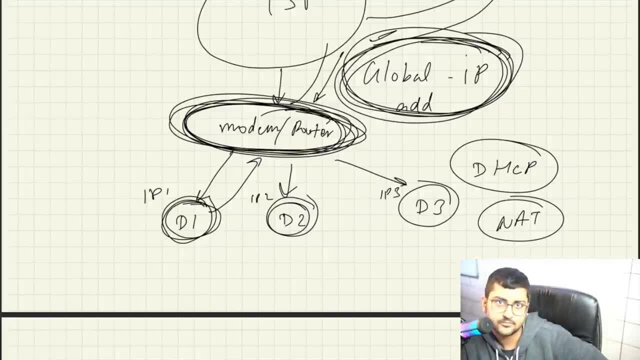 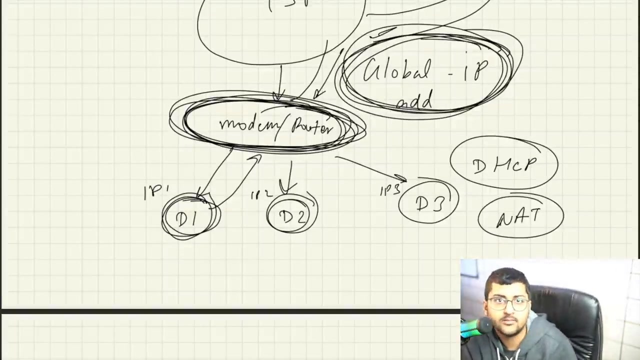 get got you want the data to be back in Mongo DB or you're running or your own server on your system you make a request to the Internet and the data when it comes you want it to come to your own server or application whatever you're running you are gaming some for example you're gaming you're chatting to someone in an online game that is installed on your computer you send a request to the Internet the Internet gives back the message of your friend and now your router is like okay I know it's it needs to be sent to Kunal's device but how do I know where do I need to send this message present to the game or the browser or whatever where do I send it so IP address is a very important point IP address decides which device to send the data but how do we do decide which application to send the data in that device we that we do that using ports okay because one single computer can be running many success micrograms you don't need to have senior computers to do that you can just install 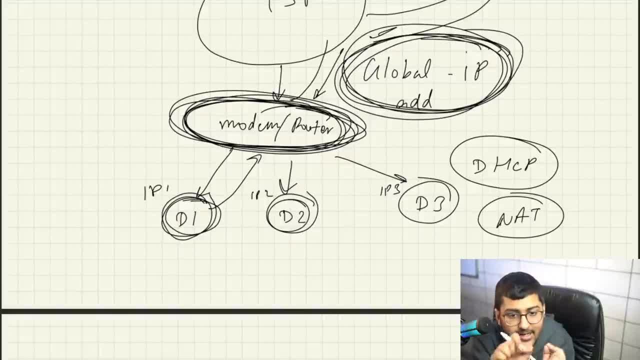 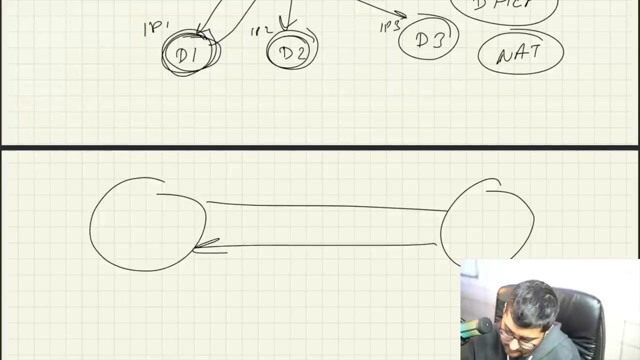 internet applications and when the internet sends the data to that computer the computer has to decide okay fine I have gotten the data but which application requested this data you do you make a you make the you know all the all these will be having obviously the same IP address because they are on the same device okay but how do these applications differ using port numbers okay that is basically what a port number is so if you attack if you're talking to your friend using you know some some application some chat application or something so you will be having an IP address you you and your friend you and your friend are talking to each other okay you will have an IP address and you will have a port number your friend will also have an IP address and a port number IP address and port number will determine where your computers are located port number will be denoting which application you are using to communicate okay so IP address will identify the computer but port will be identifying the application okay cool 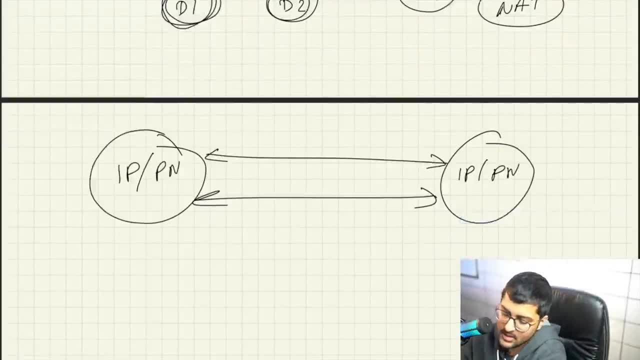 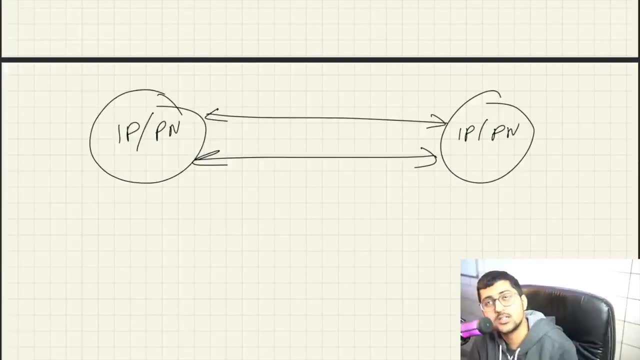 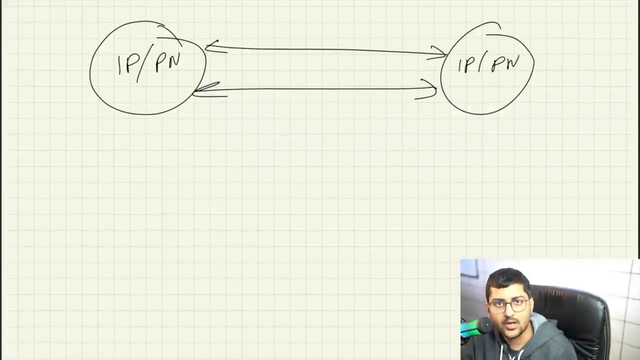 let's talk a little bit about about ports okay so ports are basically 16-bit numbers okay if you don't know what bits are check out the mathematics video I did in the data algorithms bootcamp there I have covered in detail number theory and everything so 16-bit means what your port number is a 16-bit number so 16-bit basically means you can have 16 cells and each every cell can contain what 0 or 1 so how many total numbers can you create 2 raise to power 16 okay so total port numbers that are possible are two raise to power 16 just something around 65,000 okay something around 65,000 port numbers are available okay sound good we know that web pages are using which particular protocol HTTP and our protocol is http and we can use that in many cases we can use that in many cases don't worry how it's using it i'm just telling you i'm asking what is it using how it's working everything i'll cover later on okay so we know web pages are using http okay so there should be some sort of port number defined for it if you're browsing on the web you say google.com request is sent to google google sends the request back now your request is on your device but it does not know where to send it do i send it to the web browser do i send it to the email do i send it 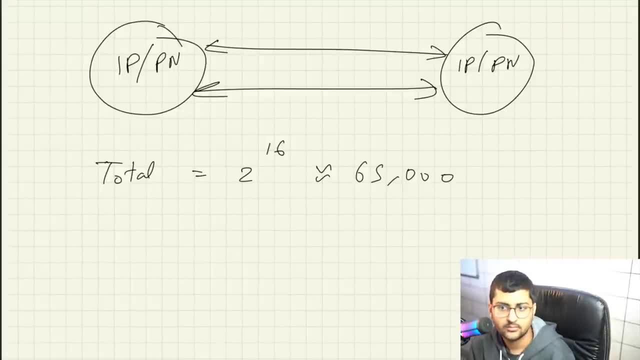 to some game you're playing where do i send it for that a port is defined so all the http stuff that you do that will happen on port 80 it's well defined these are well-known ports okay it's defined by people all right 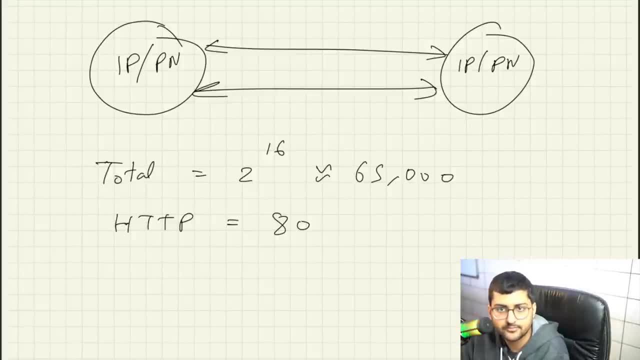 sound good if you're running mongodate mongodb okay mongodb i believe the port for this is 27017 correct me if i'm wrong i'm not sure 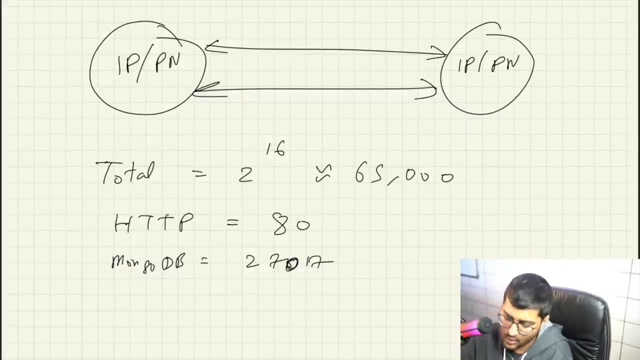 okay so ports that are from 0 till 1023 these are reserved ports now what do we mean by reserved ports reserved port means that if you have your own application created you created your own application and you're like hey i will host my application 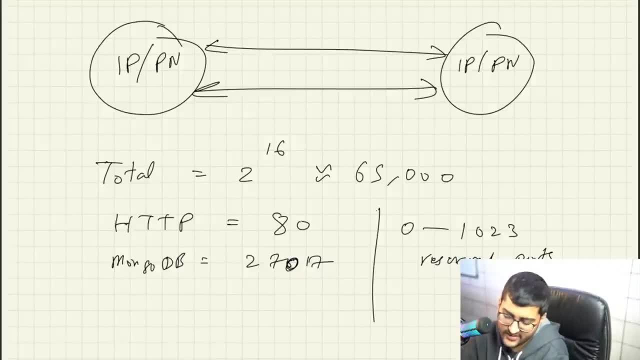 on port 80 you can't do that it's already reserved for http stuff okay sound good ports number 1024 till 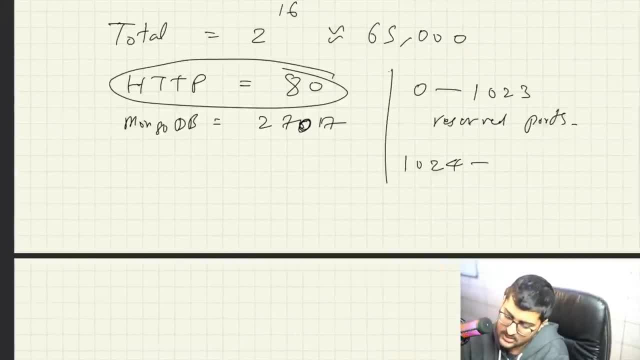 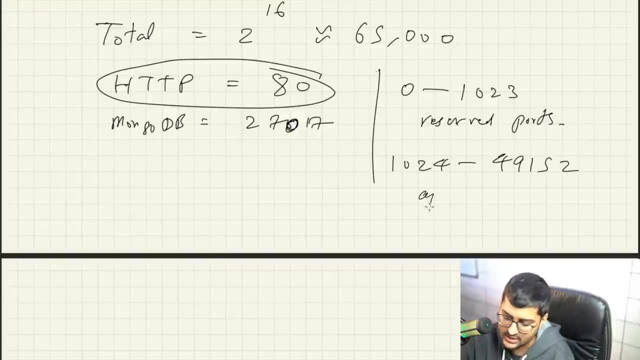 something like 49152 they are also registered but they are registered for applications some specific applications like mongodb mysql okay so sql has every sql server that you run on your application on your system 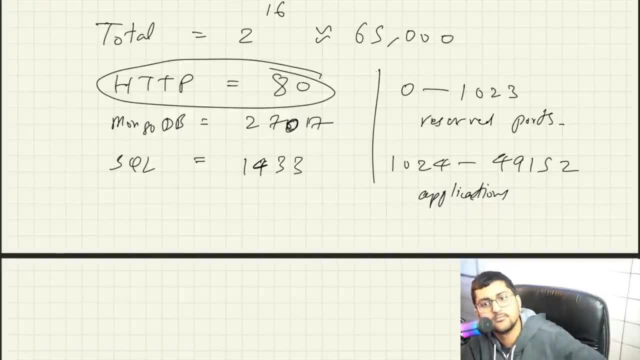 it has a port of 1433 port number okay the remaining ones you can use 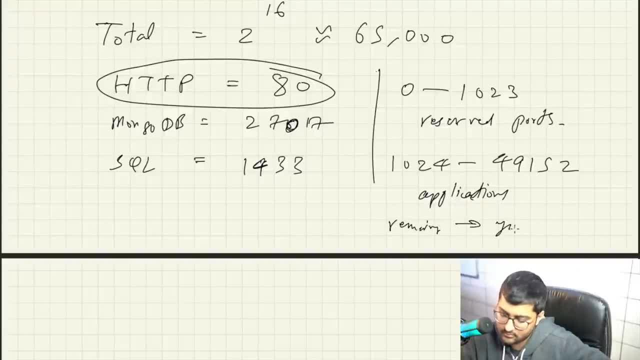 okay okay sound good remaining you can use okay that's basically about it but we'll dive deep into it as well so this was just basic stuff right now we'll obviously dive deep into everything okay so when 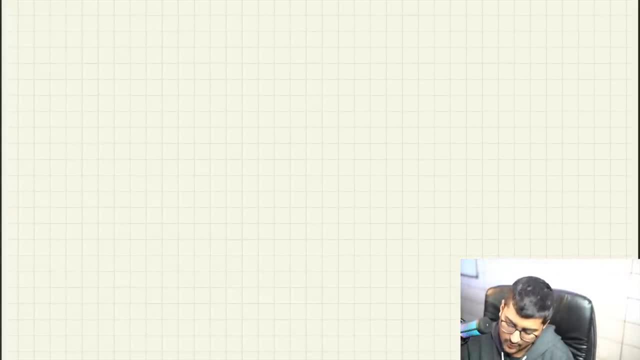 we talk about like the internet you you have your own like computer over here let's say 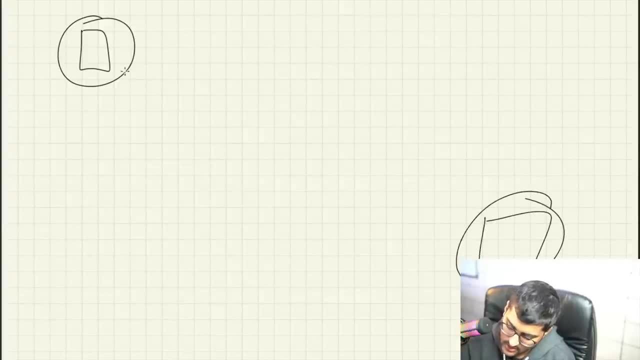 okay your friend has a computer in some other other country and you're connected somehow okay say internet this is a cloud 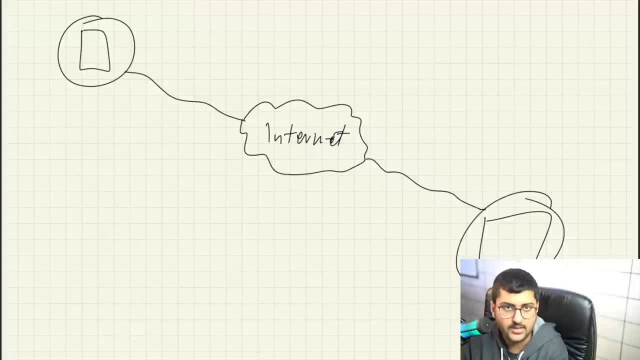 okay so you all are connected like these you know big big things on the initial scale you're connected with your internet service provider isp so an isp is a person that connects you with the entire of the internet a company or whatever like i'm using air 10 okay but before we dive into it 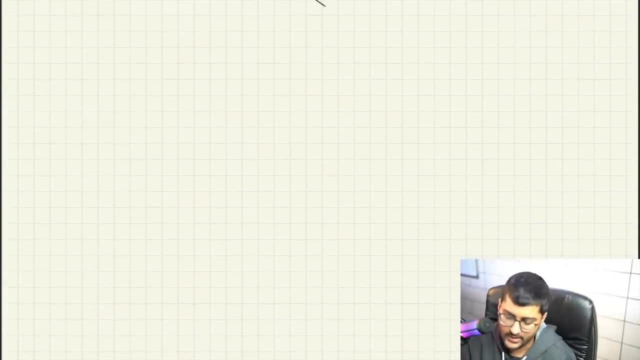 let's talk a little bit more about like how do we measure it right so when we say that what is the speed of your internet service provider like i am like 350 mbps or whatever like that okay so what do we mean by this what do you mean by if your speed is let's say 1 mbps mbps what is it what does it mean it's very simple what what is the full form of mbps 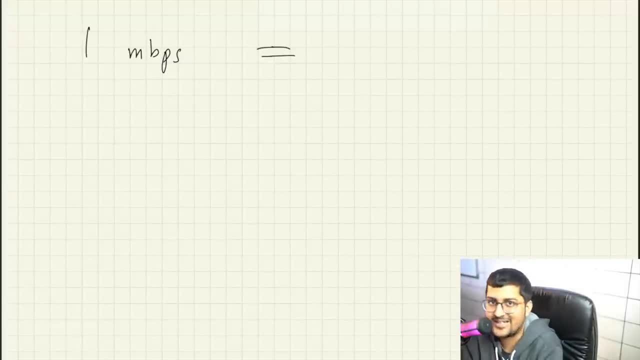 is it megabytes per second no it's mega bits per second bits bit one single bit is zero 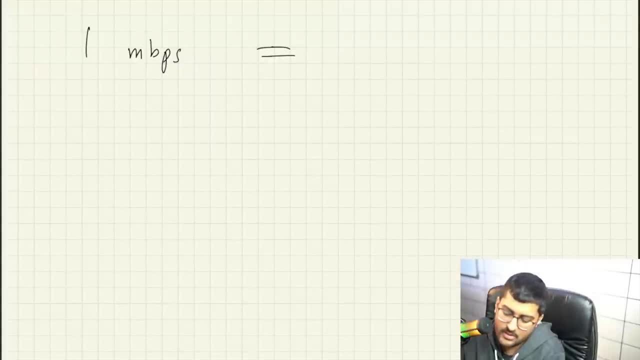 or one okay so one mbps means one mega bits you can transfer per second mega means one with six zeros so one one two three four five six bits per second can be transferred one gbps is what nine bits ten raised to power nine bits per second one kbps is what 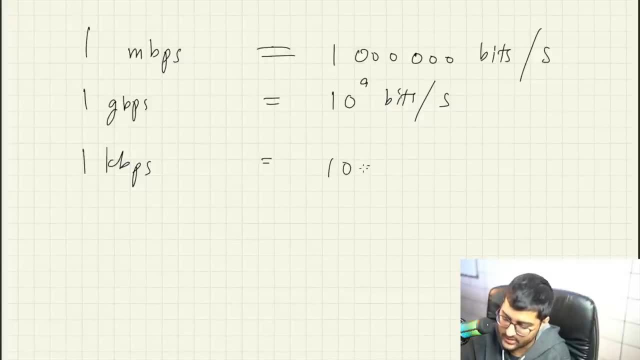 ten raised power what kb means thousand yeah one thousand bits per second very small very slow 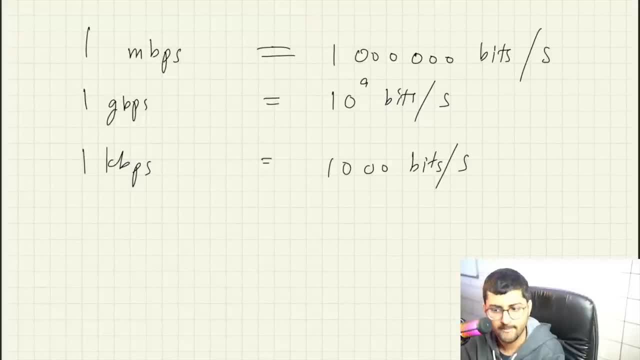 okay cool so when you when you send the data okay so you send the data back you send the data from one computer to another computer let's talk about you you are sending data from one competitor to another computer that is known as upload when someone sends data to you and you're downloading that it's called download okay the download speed upload speed that's basically what it's about 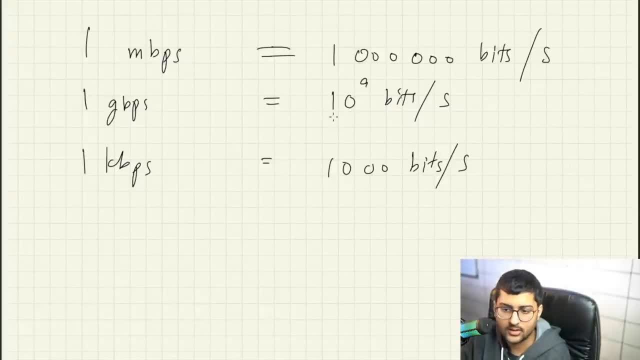 okay so check it out uh you can check out the link in the description box you can check out uh ucla speed test or whatever random speed tests and you can check out your internet speed okay so now let's talk about let's start talking about because it's such a complex topic i don't want to rush into it because people are like you know i don't understand osi model or whatever and how it's actually linking towards one another so that's why i'm 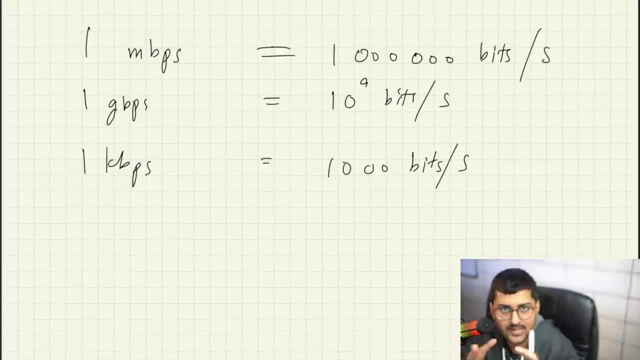 building it up okay now let's talk about how does this thing happens how does the communication between two computers and things like this happen there are two ways via which it happens okay 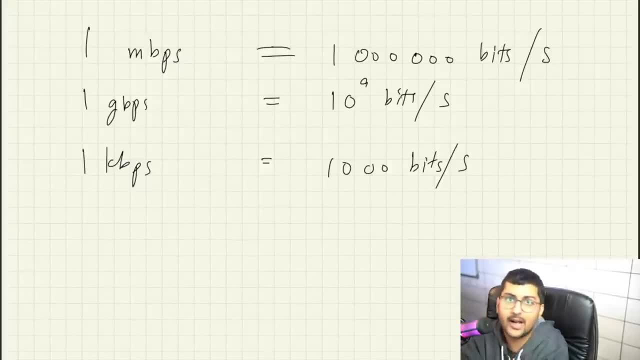 one is the guided way and one another one is the unguided way guided way means what guided way means like uh there's a set of path already defined for example so for example two computers are connected with a wire that's the guided way what is the unguided way uh communication 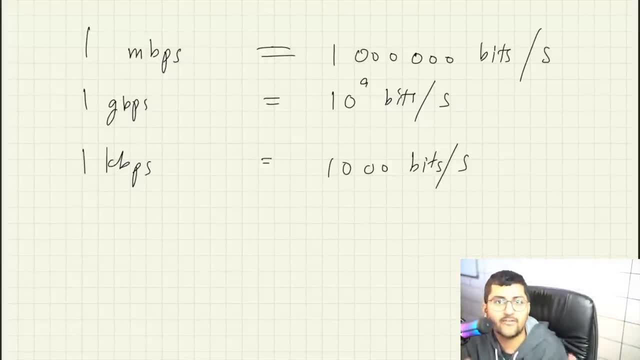 is happening but there is no like one single path for example wi-fi bluetooth okay internet 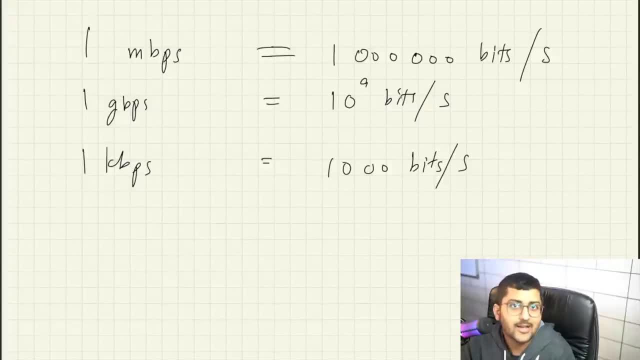 is connected with one another okay so what's the unguided way okay so when i am talking to someone from the uk okay i send the request to like my isp isp sends it to uk uk gives it back 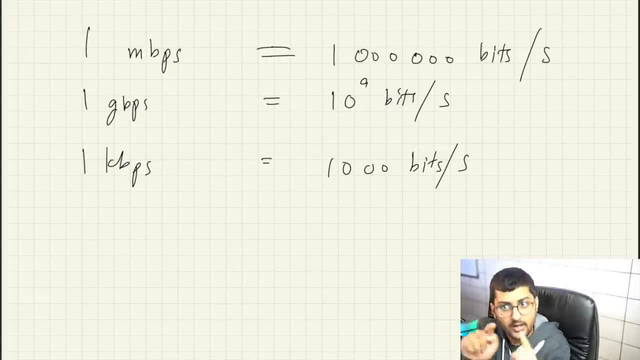 okay how are our countries connected so on the minute details how it happens i look into later on now let's look into how the bigger picture happens how are countries connected with one another 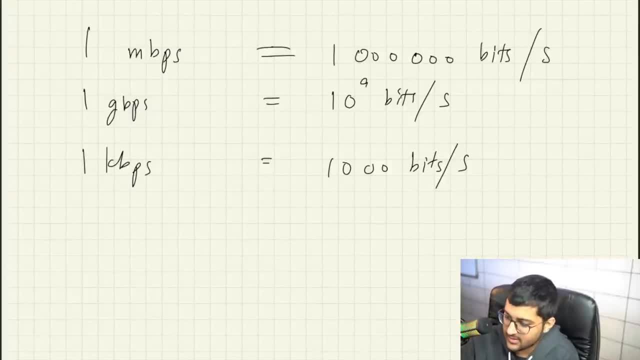 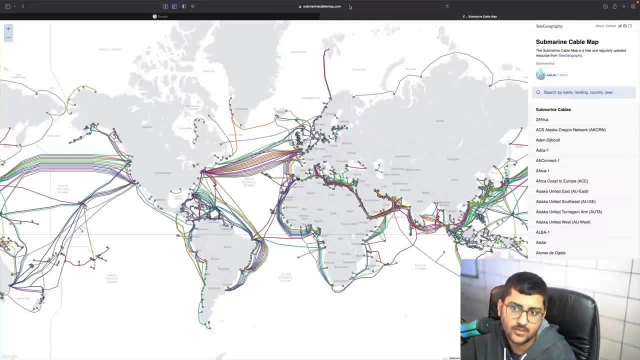 okay because it's super fast this transmission and everything that happens it's super fast how is how it's actually a website that you can go to submarinecable.com so literally they have 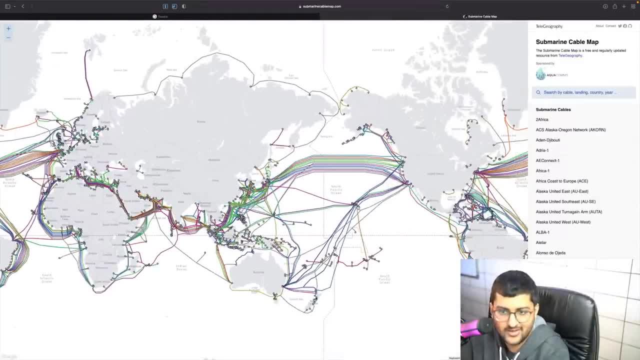 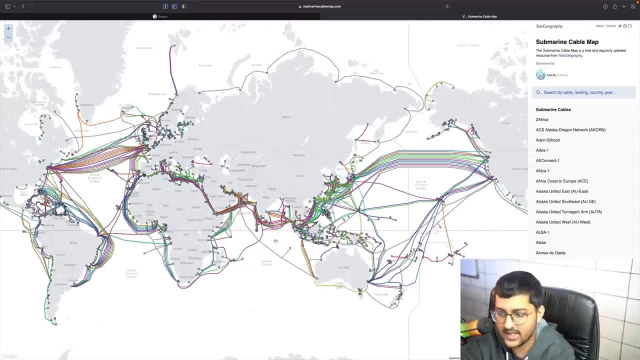 they have wires running across the ocean from one country to another wires are running down the ocean so you can see in india 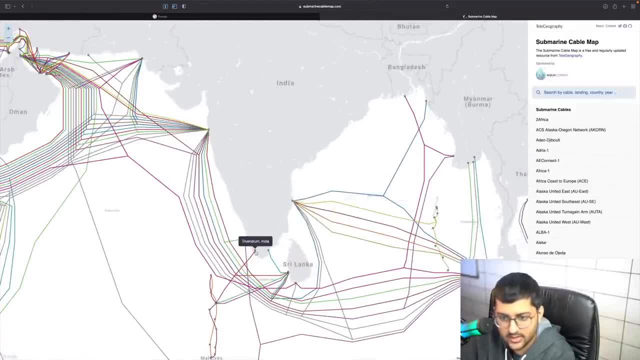 india from where from chennai cochin and uh yeah somewhere from the south you can see we 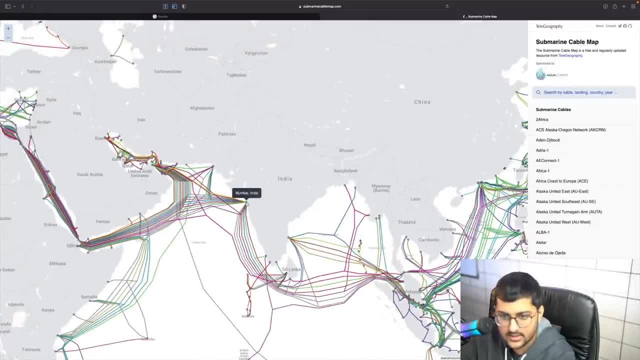 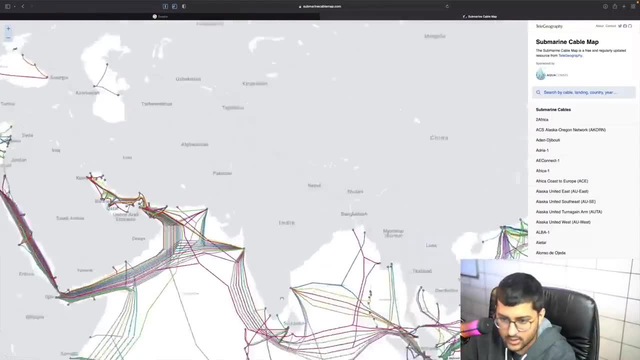 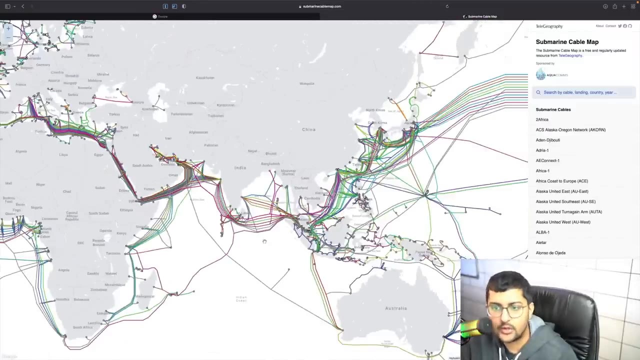 are connected to sri lanka and uh this is uh mumbai so from mumbai we are connected to like dubai oman uae and we're also connected to i believe somewhere in singapore so we're connected to malaysia and stuff and that's how it sort of like works okay so there's like a big um 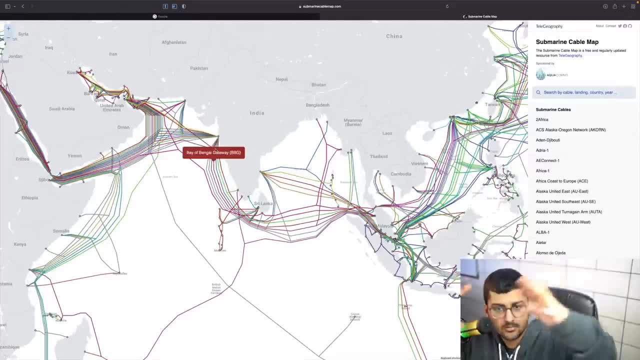 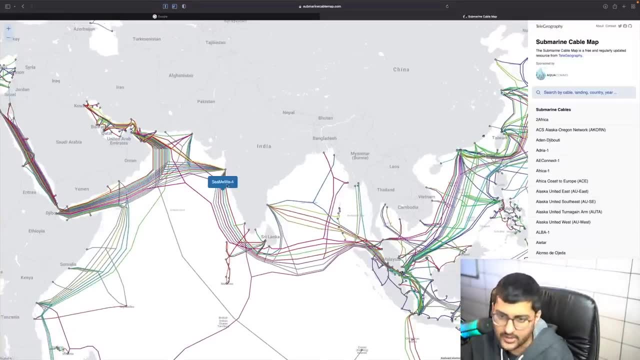 you know entity in like countries that controls this big stuff in india i believe it's startup i could be wrong but you can this is something this information you can find online who controls it from india and then they the bigger entity they give it to like smaller entities and then they give it to internet service providers and internet service providers give the control to us that's 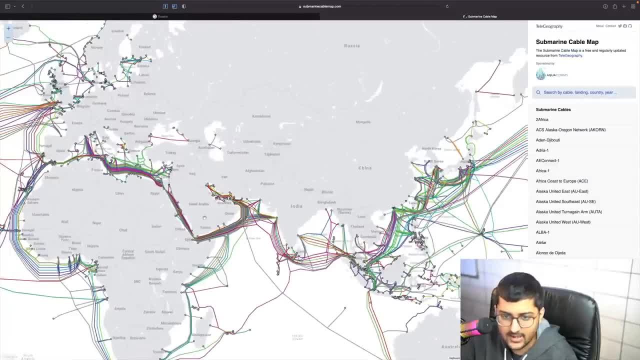 how it works on a larger scale so this is literally inside like uh inside the ocean here you can see submarine cables are inside the ocean 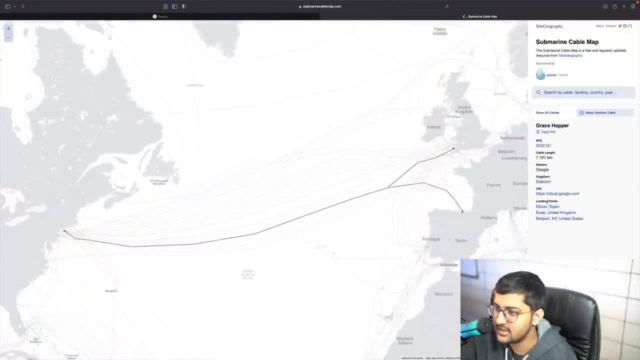 this is one of the cable it's from spain uk and the united states 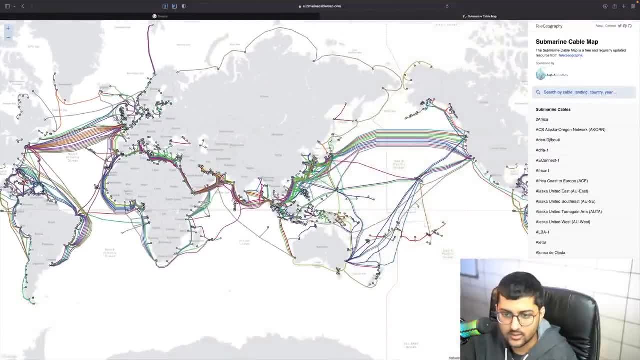 cool easy swirls look one in india over here let's check this one 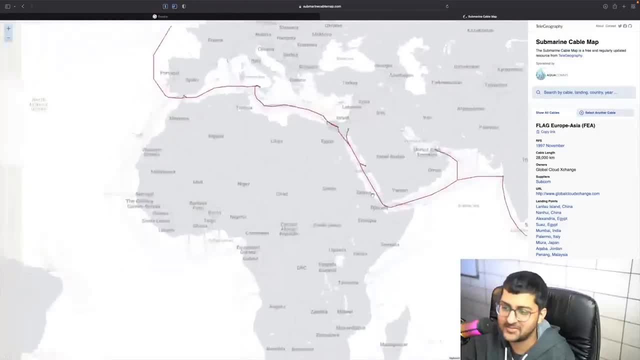 okay 28 000 kilometer is the length of this cable 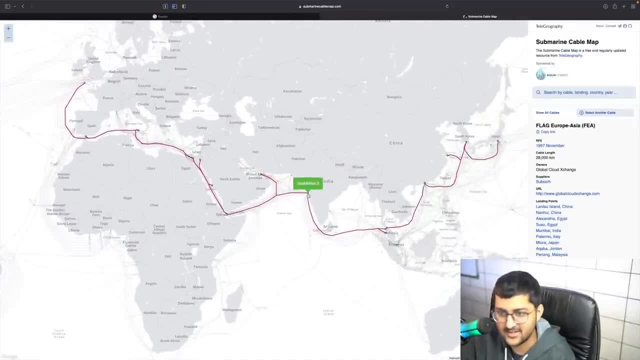 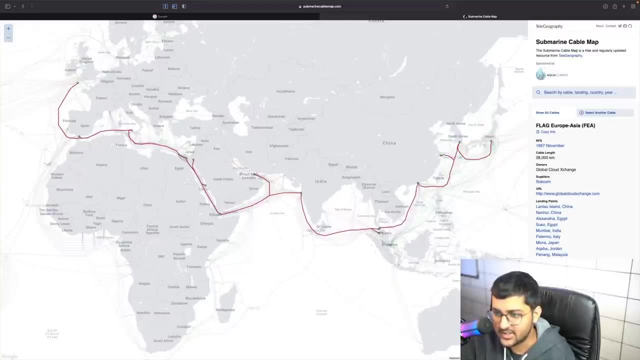 it's running from a lot of places wow japan south korea and china and malaysia india uae israel 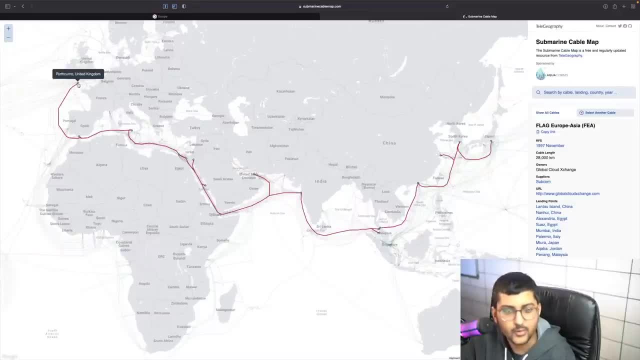 italy and uk one single wire spread across continents how fascinating is this you can see this as well submarine cables 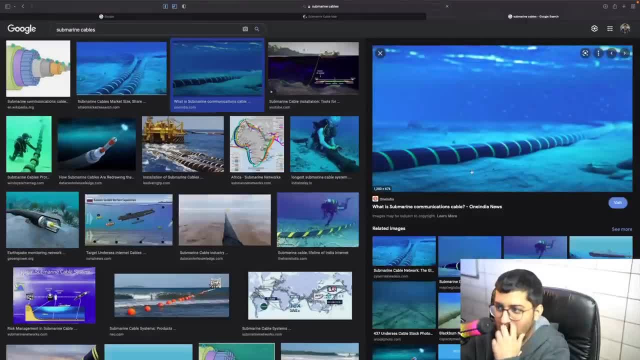 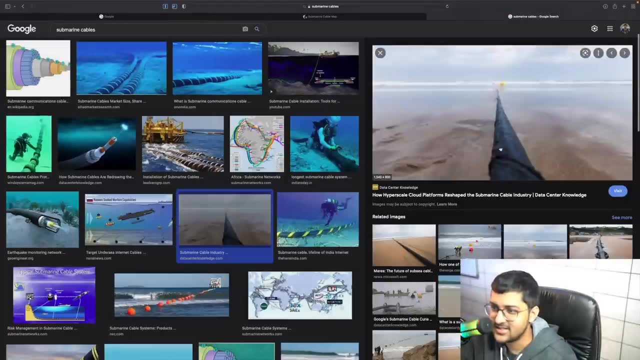 this is how it's inside the water so internet is not like above us it's actually under the ocean this is basically the submarine 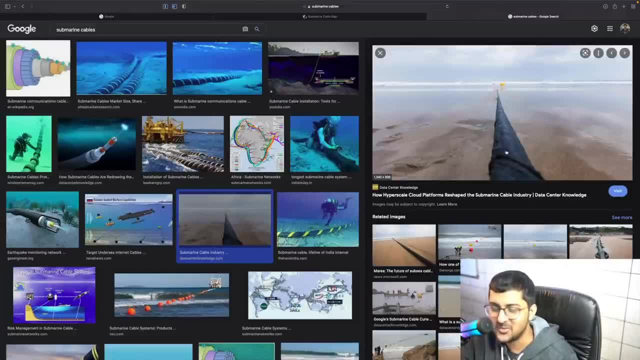 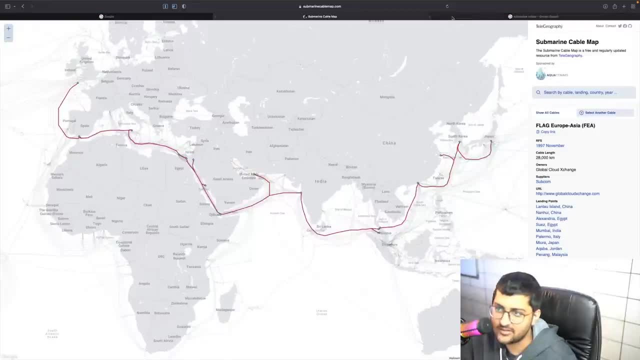 cable google also owns a lot of this right uh google has its own like search engine and whatever they own a lot of such cables right so google is like also pretty pretty famous in this they have like a lot of cables underground some people ask when i don't sharks or something you know they cut 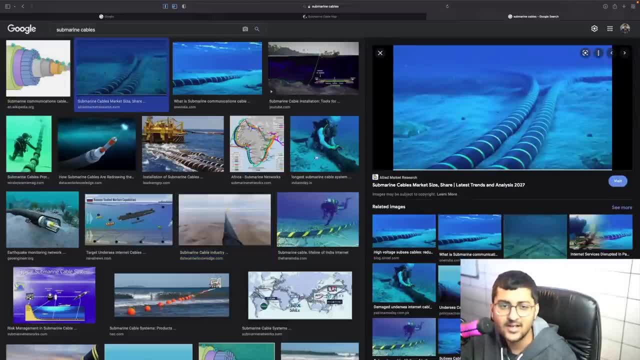 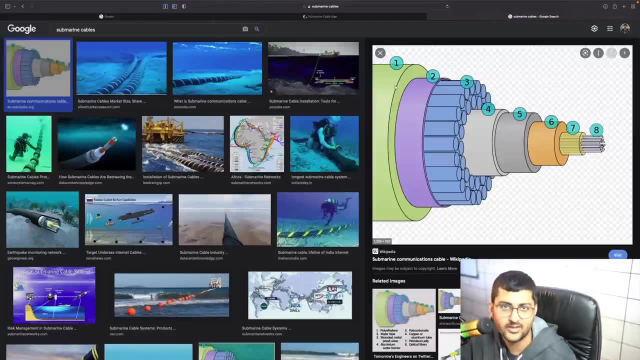 this cable or fish fishes don't they cut these cables um no they don't because it's actually very heavily guarded okay and it's actually heavily buried on the ocean floor so animals can't get 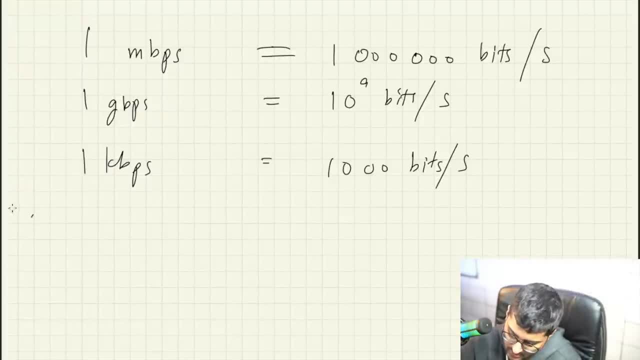 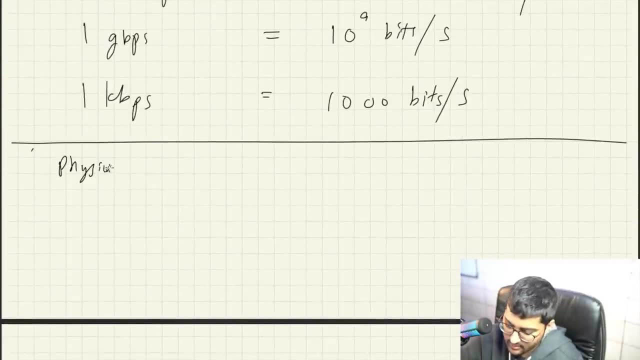 to it okay so if you want to learn more about it you can um how the you know data is uh like how computers get connected so physically they get connected in this way you know you can look at like your optical fiber cables for example optical fiber cables okay how these things work 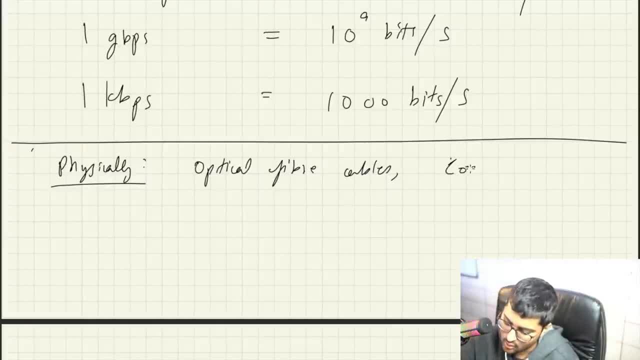 and all these other things coaxial cable coaxial cables or whatever okay you can take a look into 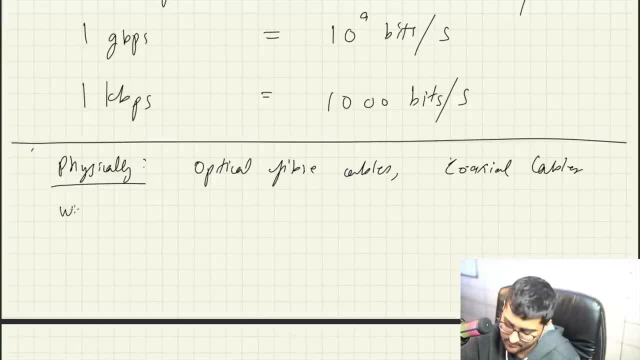 this other than that this is the wireless one so in the wireless we are already familiar with it 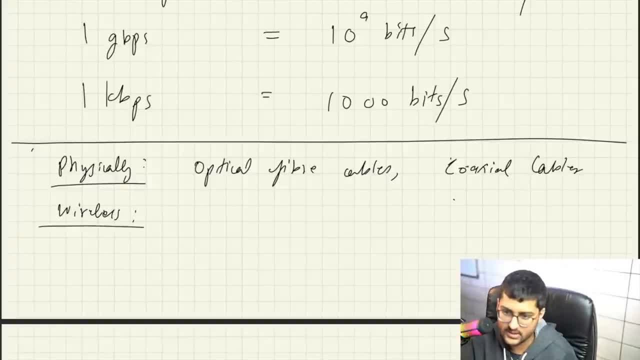 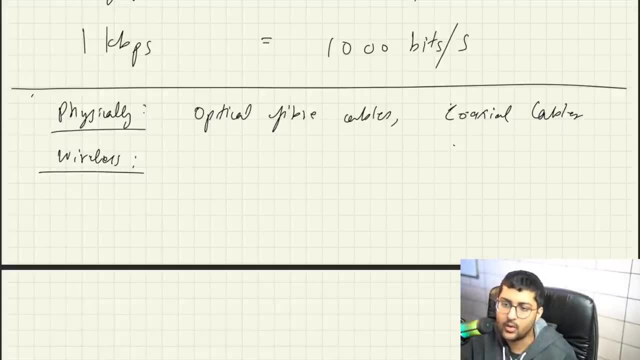 what is the wireless stuff wireless stuff consists of um like radio channels for example right so we're talking about uh example bluetooth which is for short range bluetooth is there then we have wi-fi 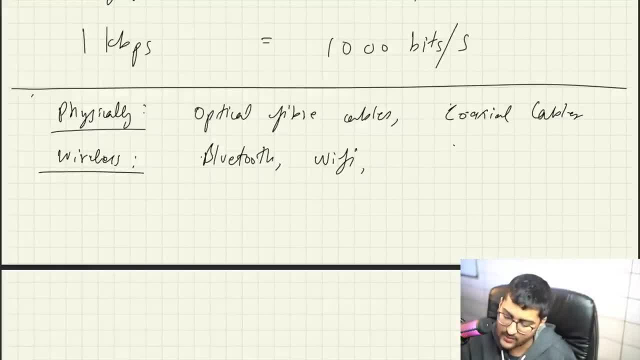 okay and if you're going to talk about like longer ranges for that we have like 3g 4g like lte now we don't have a lot of time to talk about that but if you're going to talk about something like that 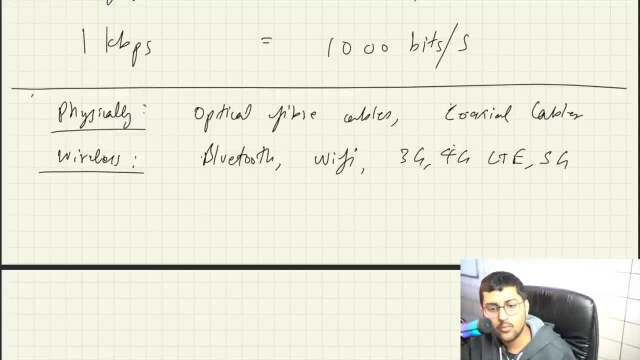 okay so that's basically about it now you'll be like why do you have why do we have these you know why can't we just use satellites why do we have to put cables under the ocean so many long long 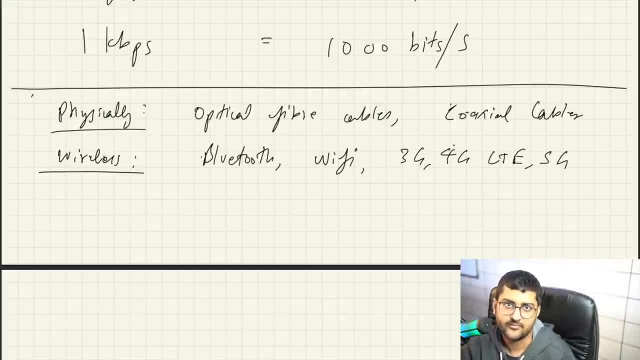 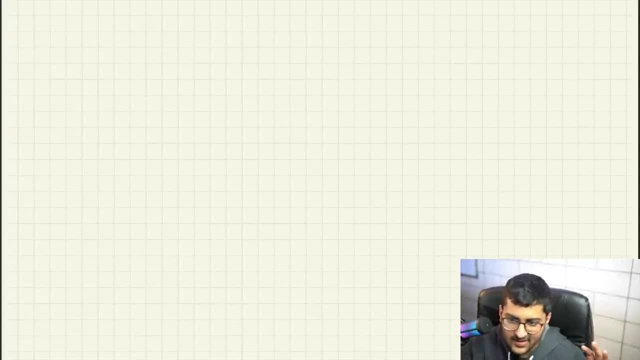 cables across the world because it's faster than satellite okay currently also there isn't like i haven't given you the actual feeling of how the internet thing you know actually works how how the protocols happen and what are the 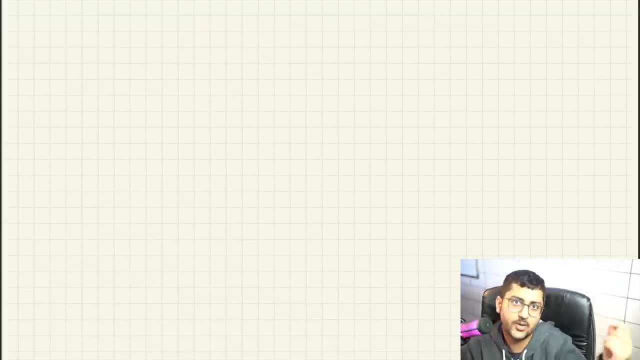 various stages and the all the things that i mentioned like you will have your global ip and you know you will get the request and it will transfer it to your local computer and then it will transfer it to your application or whatever so how these things happen internally we haven't covered it yet we will cover it later on in this video itself when we talk about the osi model okay so there are some layers in the osi model and we'll cover every single layer in detail before that i 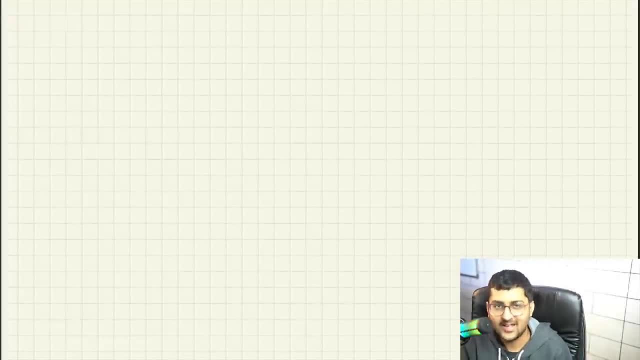 want to give you a refresher on what we learned in high school okay in high school we learned a 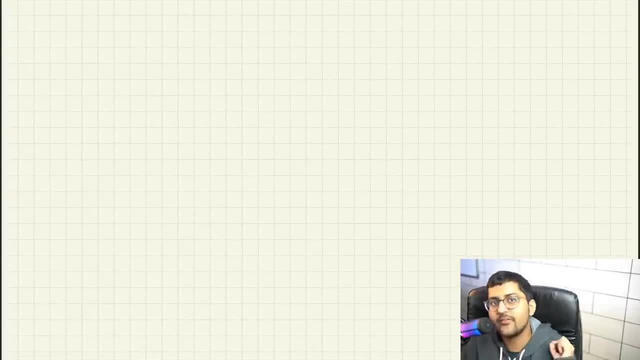 okay so i just told you how countries are connected let's do a little bit of a refresher of how various things are connected okay so we know there's something known as a 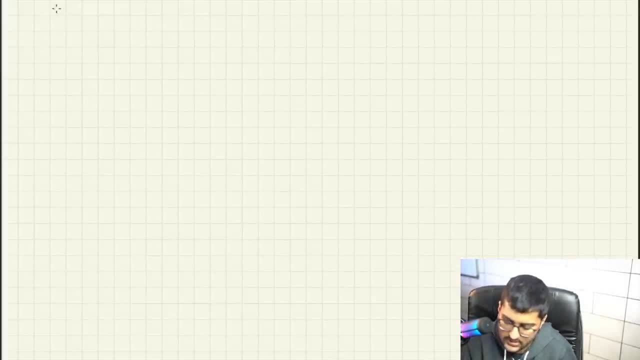 local area network lan okay so we know there's a local area network i'm just writing down pointers you can google it like like yourself what is this small house for a small house or office if you have like some devices connected that is known as local area network 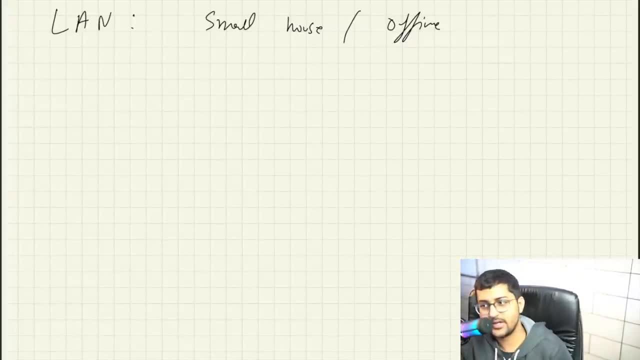 okay small here does not mean that there's only five computers you can connect or 10 computers you can connect okay you can even come out you can even connect 10 000 computers if you want okay but it just basically means it's like in an area 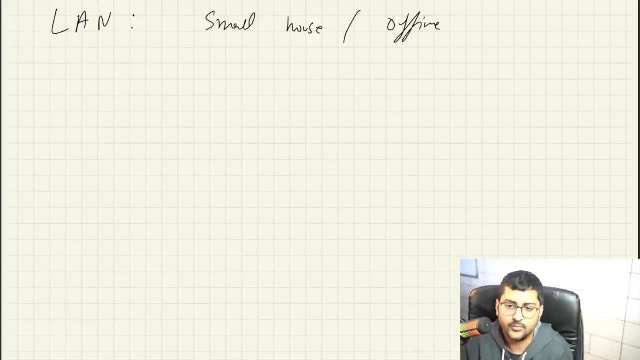 okay okay cool so that's basically it and uh let's also look at some of the concepts of uh like lan or how how these computers let's say connected it's very general knowledge we have worked with this before 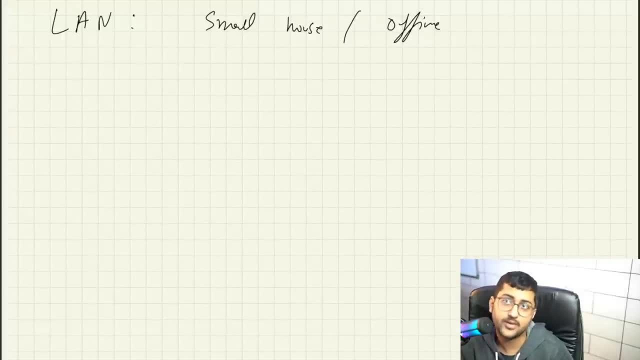 um you have uh if you have game you know game with your people like folks before you can connect it via ethernet okay so how via ethernet ethernet cable 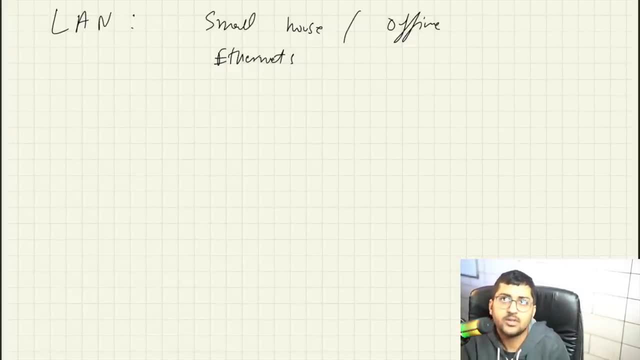 right they're like network adapters and ethernet switches because there are so many ways to connect to the outside world uh via wi-fi via like bluetooth via ethernet or whatever there needs 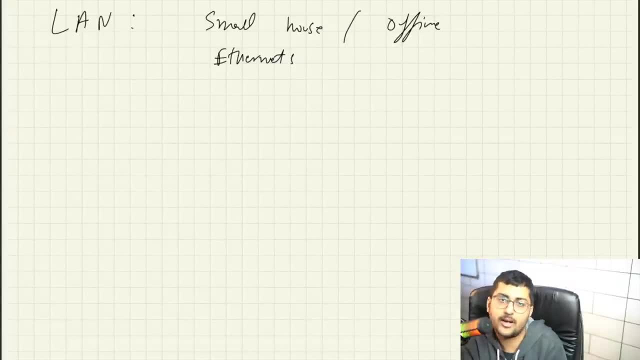 to be some sort of a device to manage this that's known as a like a network adapter like network for example okay or how we can connect on a local area wi-fi also yeah wi-fi works you can connect via wi-fi also 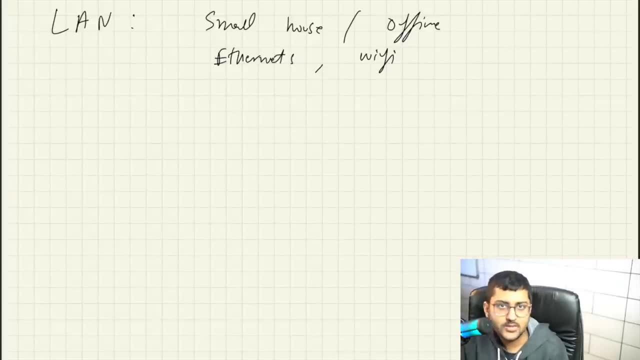 okay now in high school we also learned about man metropolitan area network which is across a city it's very simple stuff 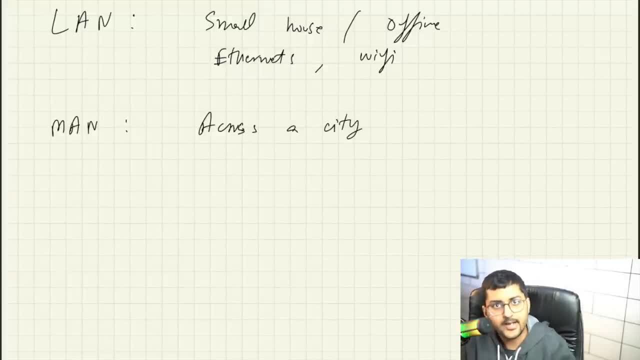 across a city okay i'll cover in detail how isp helps us in you know connecting us to the internet service providers okay then there's a wide area network okay across countries for example 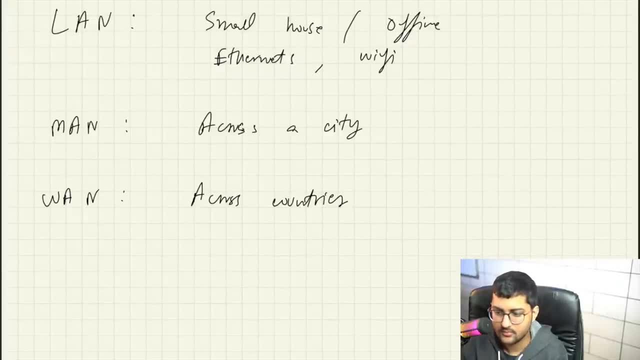 okay cool all right so wide area network basically allows you know for you to connect over countries okay typically using optical fiber cables optical fiber cables 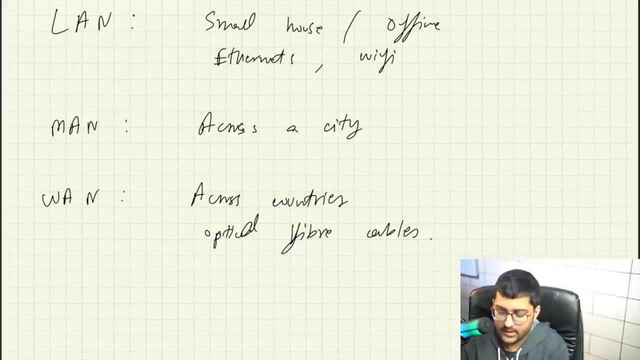 okay so we all learned about this in the in high school but how does it relate to the internet so internet is actually a collection of all these three a lot of local area networks that are connected to each other using metropolitan area networks or local area networks or local networks networks that are connected to each other using wide area network okay so this wide 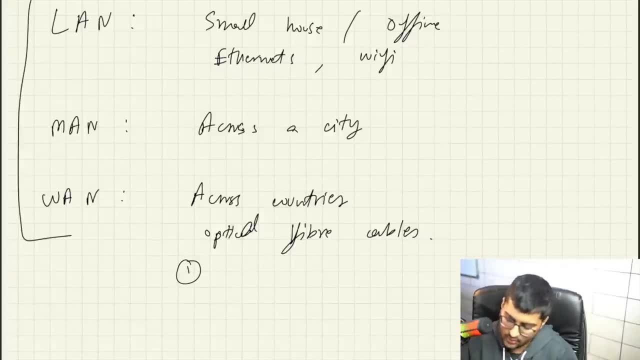 area network there are two more things I want to mention over here one is known as SONET okay SONET basically means synchro synchronous optical networking okay so it basically carries the data using optical fiber cables hence it can cover larger distances second one is frame relay okay 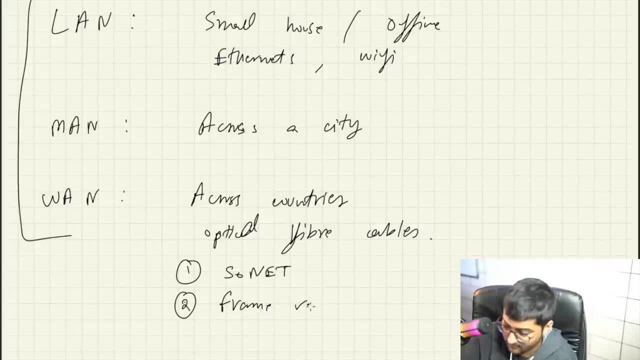 so SONET basically means SYNCHRONOUS OPTICAL NETWORKING okay so it basically carries the data using optical fiber cables hence it can cover larger distances second one is frame relay now what is frame relay it's basically a way for you to 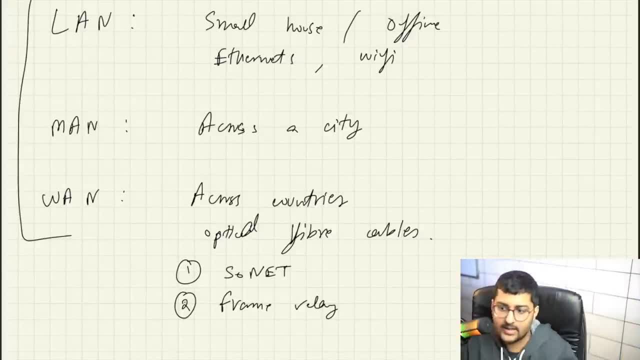 connect your local area network to the wider area like the internet 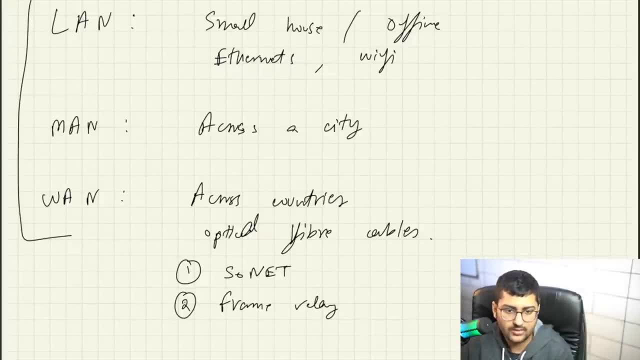 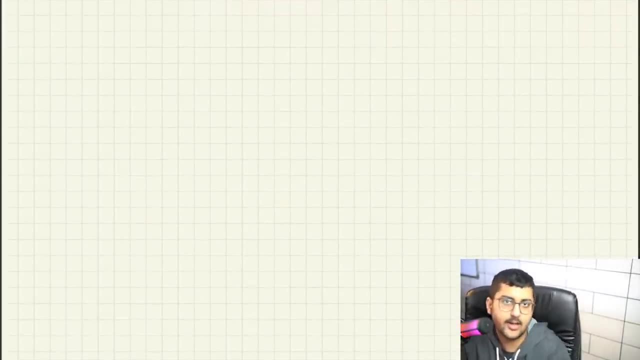 okay so that was about it okay let's talk a little bit more about this thing in detail a little bit more terms before we move forward to how the internal implementation and everything is done okay right now also we have learned a lot of terms and i'm writing it down over here the video is recorded i'll be adding timestamps so 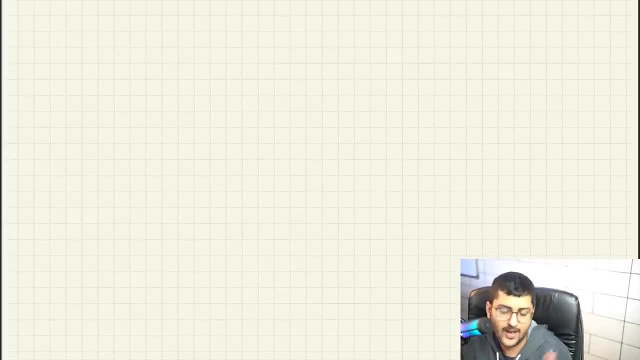 you can add on it add on to it like come back revisit and whatever so when i talk about modems and stuff okay what is a modem i'm going to talk about router what is a router so a modem is 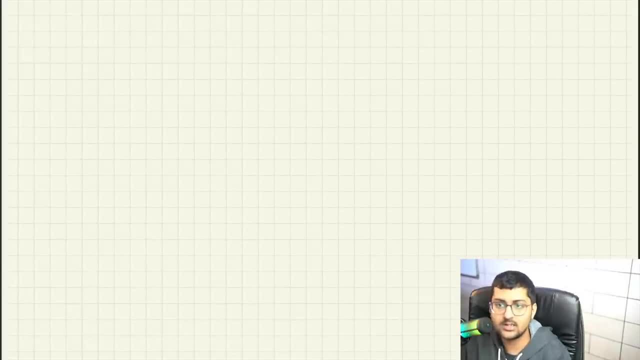 basically used to convert digital signals into analog signals and vice versa 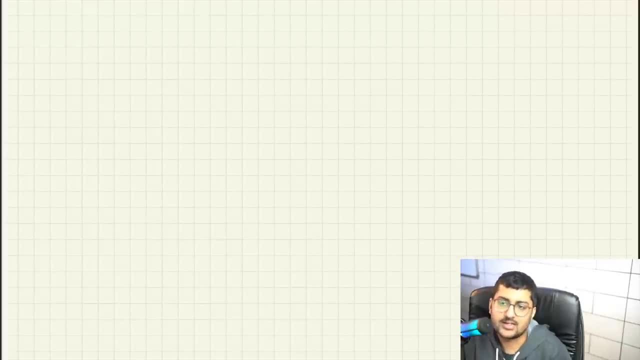 okay so for example the digital data that you have on your computer a modem can convert that into an electrical signal so that you can transfer it over let's say some telephone lines 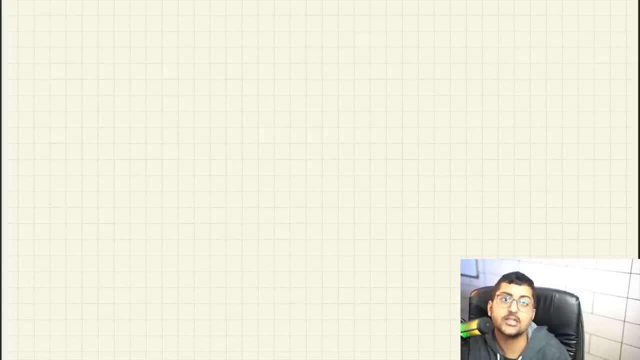 or some other you know other modem at the receiving side for example and that will recover 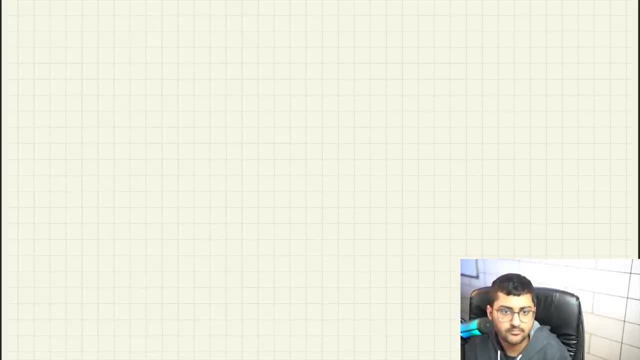 the digital data like an image okay sound good or and a router is basically a device that routes 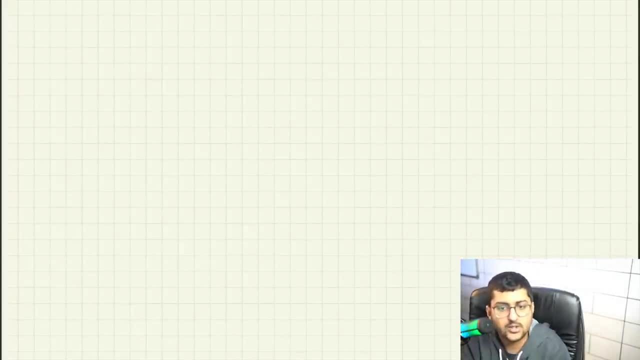 the data packets the packet thing we talked about right based on their ip addresses okay 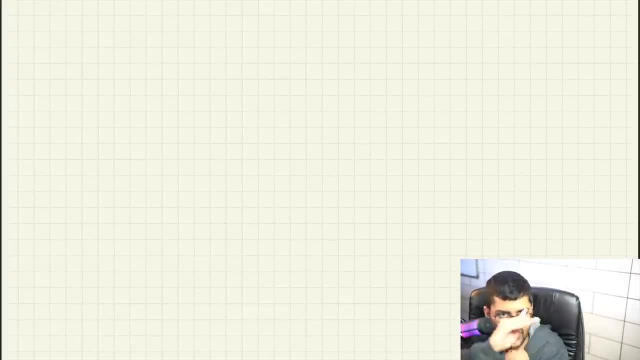 when we talk about osi model we'll know that it works on the network layer and they are connected to 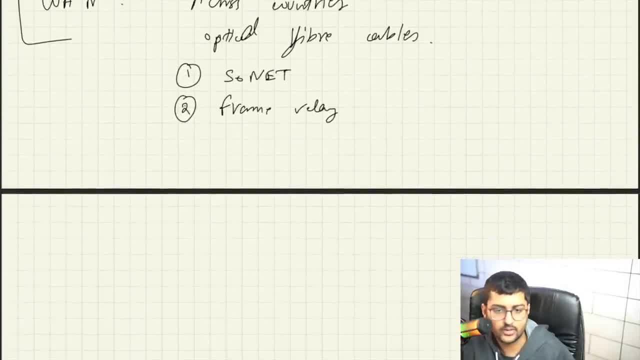 like the the LANs that we just talked about and the wide area networks okay so how this data is 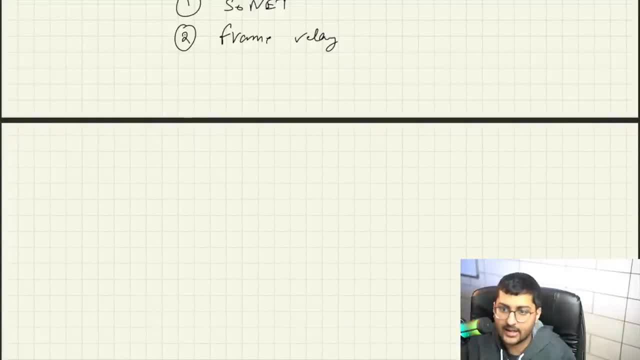 routed and everything what is a packet what is consisted inside a packet and everything i'll cover shortly okay but what we're trying to say over here is that like for now that is what you 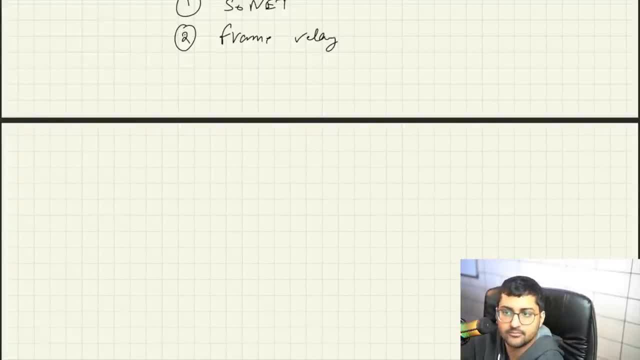 need to take into consideration we talk about modem okay 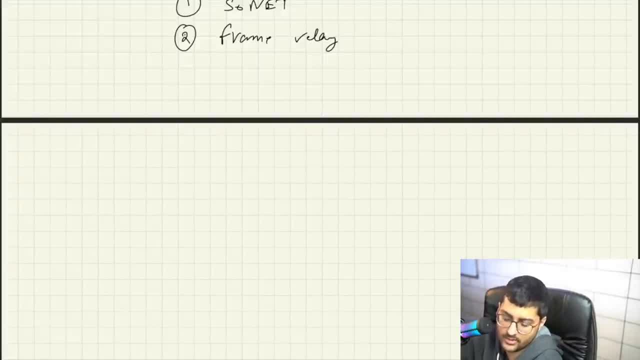 cool we already talked about like how the client and server model works and everything so we talked about like what modems and routers and these all devices and stuff we'll cover later when we talk 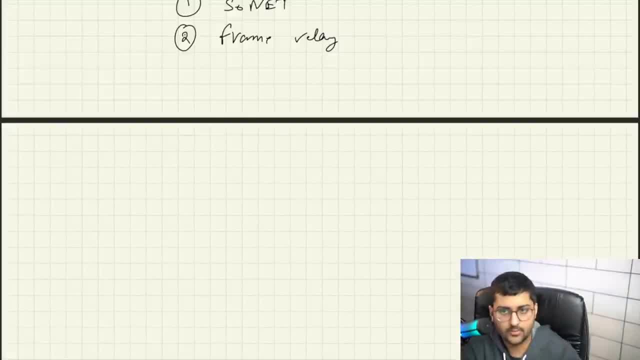 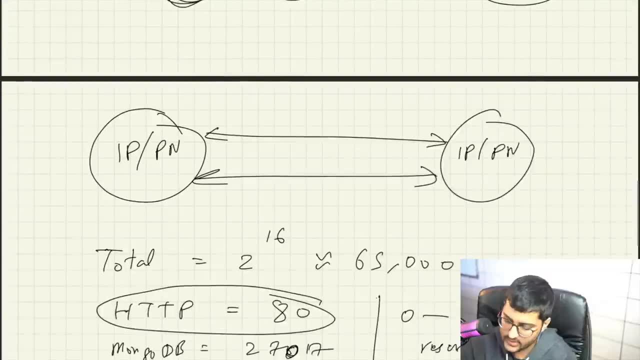 about osi model and everything okay so the client server model we know uh client makes a request server will send a response we had a you know uh we had it written over here somewhere right okay 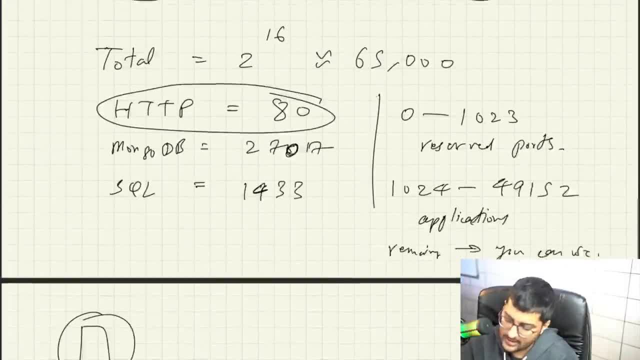 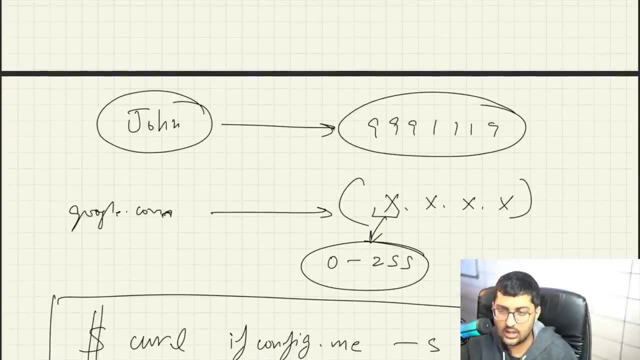 cool um we talked about ip addresses a little bit right we talked about uh what are an ip what is an ip address and it sort of like resolves you know uh it's like a phone book 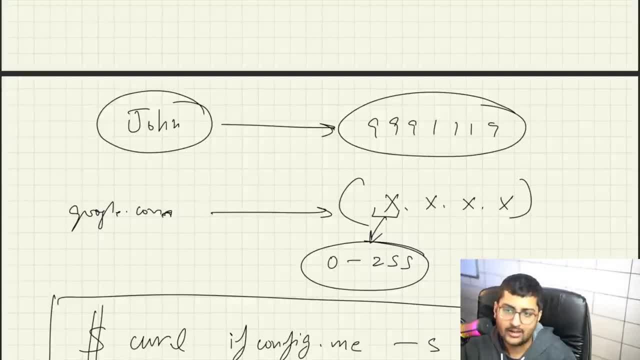 phone book of the internet if you will okay and um we can basically remember the domain name and it will uh point to the computer or a server of that ip address okay one more thing i talked to you 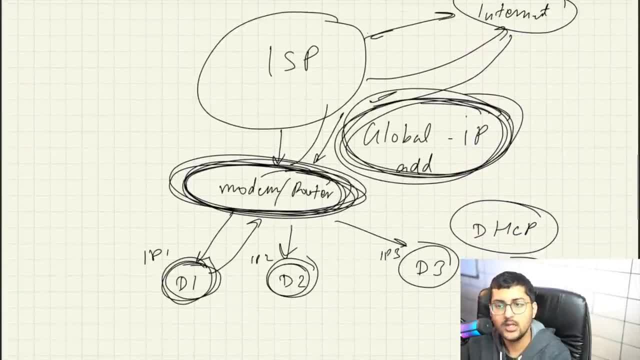 about was internet service provider okay so internet service providers are companies that 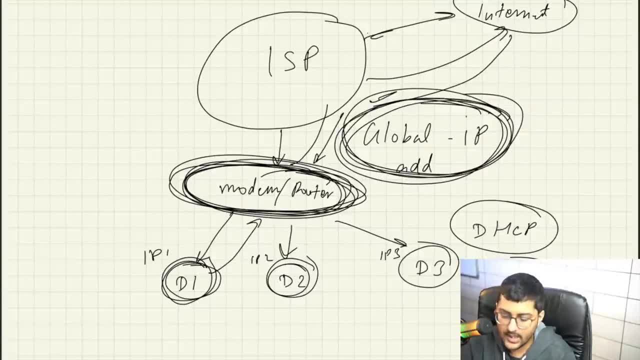 provide us access to the internet okay so internet service providers are basically connected to larger internet service providers that provide service to them like i mentioned previously okay so in india the the top level you know uh they are like top level is internet service providers in the world and there are only a few these are known as tier one or tier one 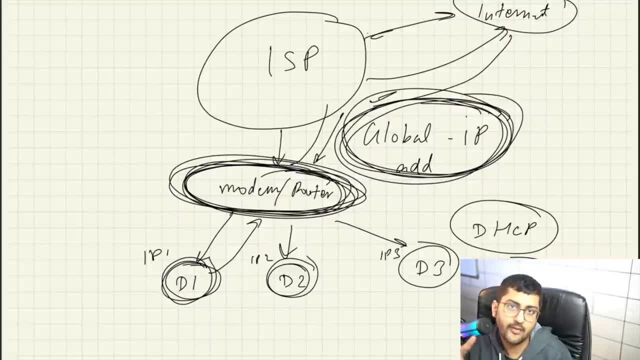 um internet service providers in india we have the tier one service provider tata okay tier two internet service provider can be like airtel or whatever 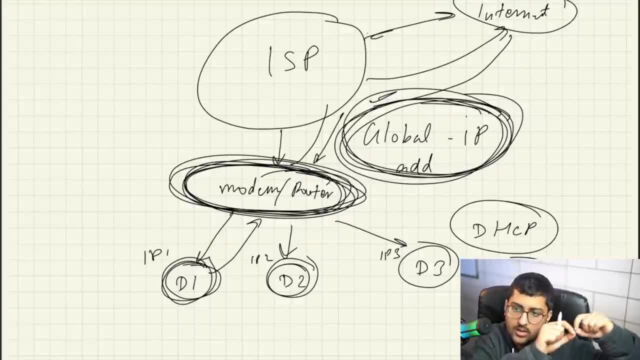 okay so there's a long cable from chennai uh for tata in like chennai to singapore and stuff okay so repeated it multiple times hence you should not get uh not get confused 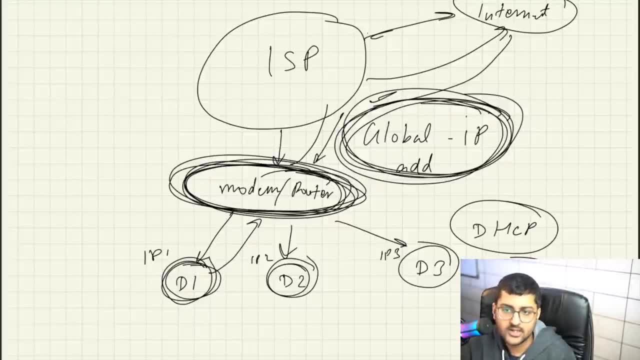 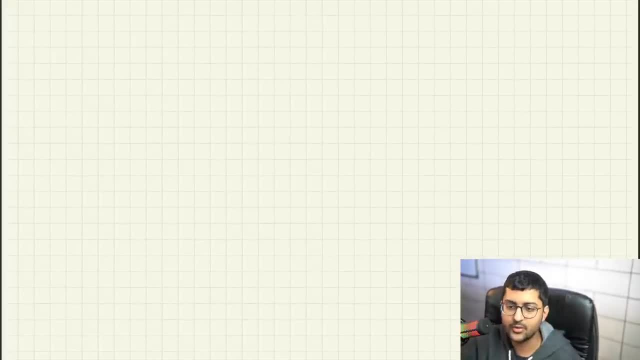 and um yeah on a bigger picture that's basically about it cool let's move forward okay now one more thing we studied in uh in high school which is also very basic stuff which is 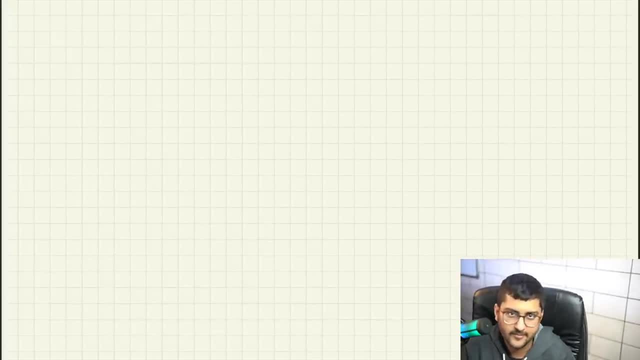 uh how computers are connected various ways they are connected right so topologies you have studied this in high school as well topologies just a little bit of revision don't leave out anything kunal you left out this thing you left out that thing or whatever okay so the number one topology very simple one everyone knows this bus topology okay so every system in the bus topology it's like connected to one like 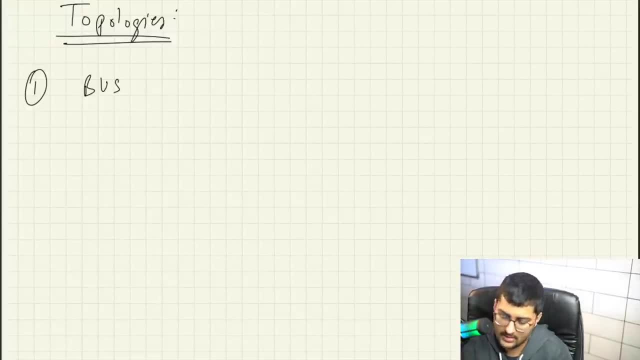 a code or like a backbone okay for example so here we can have let's say a backbone is like this and computers are connected to it like this computers are connected this is bus topology 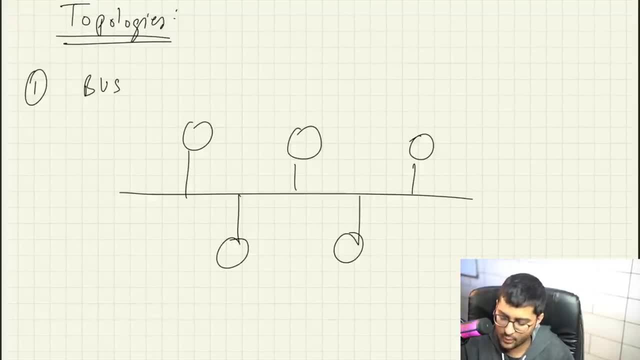 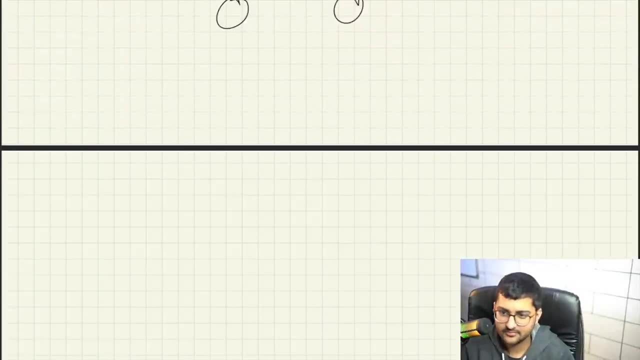 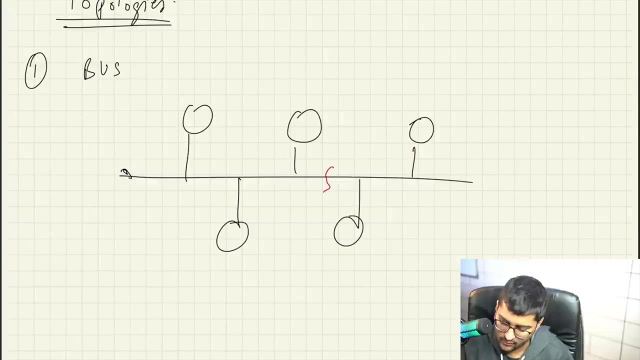 okay but what is the problem here it's very simple if the if this gets broken this link gets broken then it will like spoil the entire network okay and also since everything is being transmitted via this cable this one over here um only one person can send data at a particular time okay so this is the bus topology this is sometimes how computers are connected okay 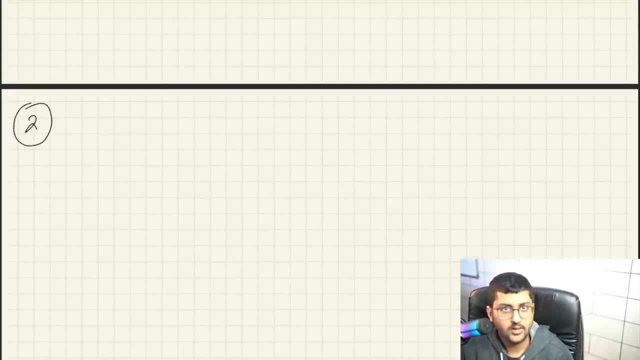 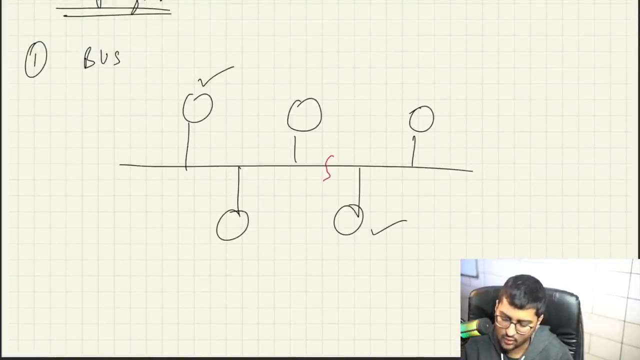 second one is also pretty simple which is known as a ring topology ring so as the name suggests computers are connected in a ring with one another okay so in this for example you want to send data from here to here it's pretty simple it will go via this wire okay but in ring topology what is happening is that every system communicates with 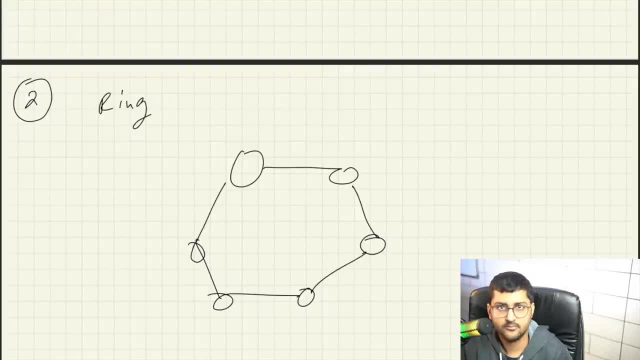 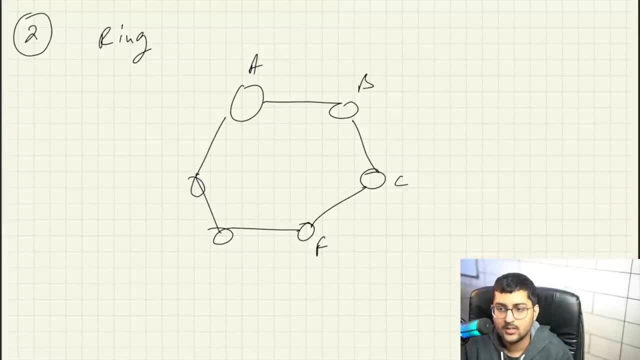 but what are the limitations here now one more limitation here is if one of the cables break then that's it you won't be able to transfer data what is the second limitation 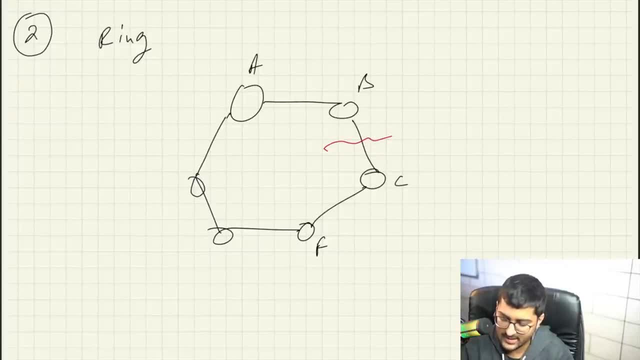 a lot of unnecessary like you know um calls are being made so if you want to send data from a to f it's making calls to b and c also so that's also not good right so that's that's a limitation 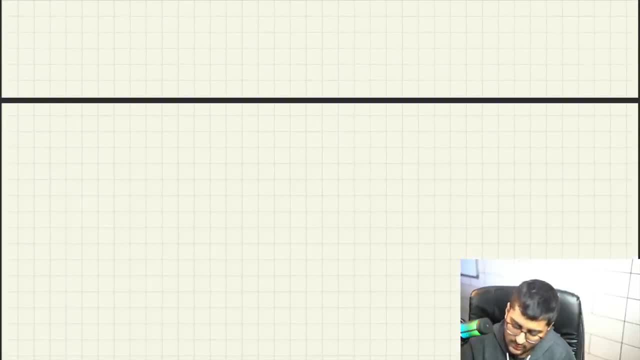 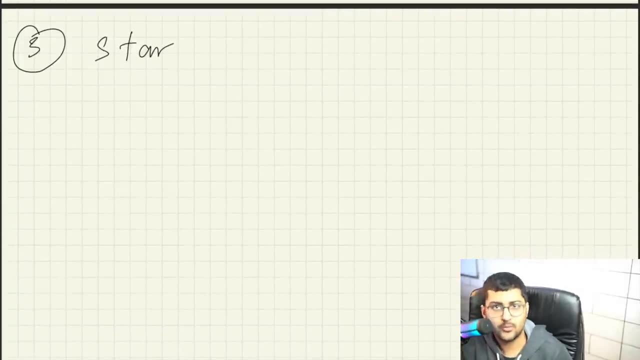 all right cool let's talk about another one another topology how other computers are connected star topology okay so what is the star topology there there's one controlling device one central device that is connected to all the computers all computers are connected to that only if computer a wants to send something to computer B then it will just communicate via this device over here this is a centralized 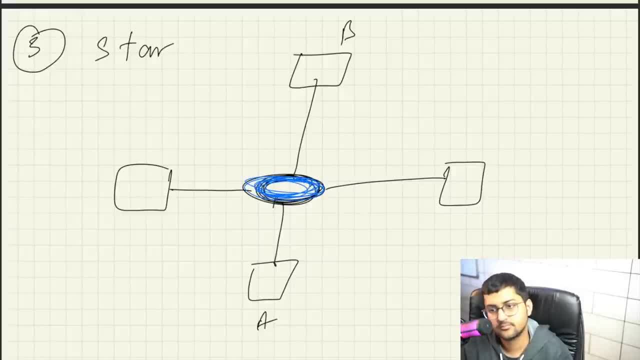 device cool what are some of the limitations if the central device fails then computer 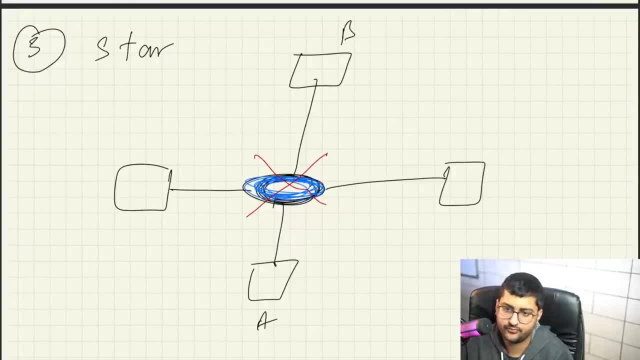 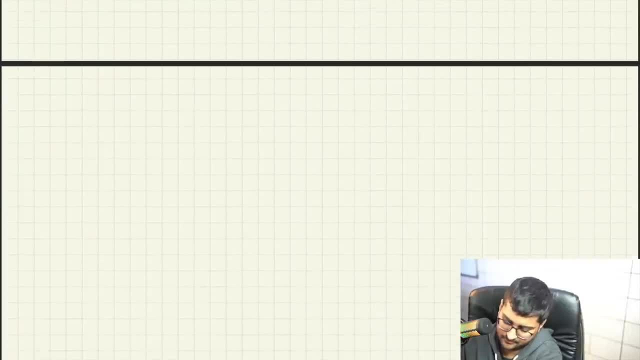 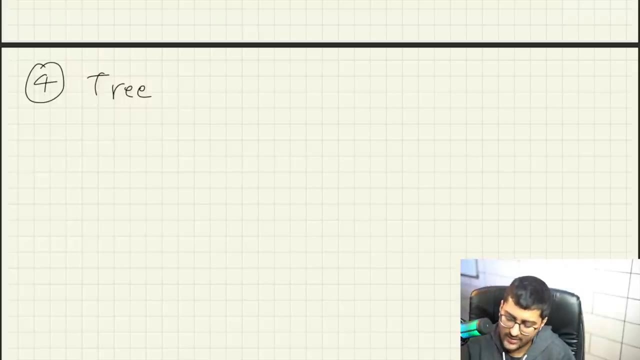 system will go down your network will go down okay there's another one fourth one what is the fourth one tree topology it's sort of like a combination of bus and star topology 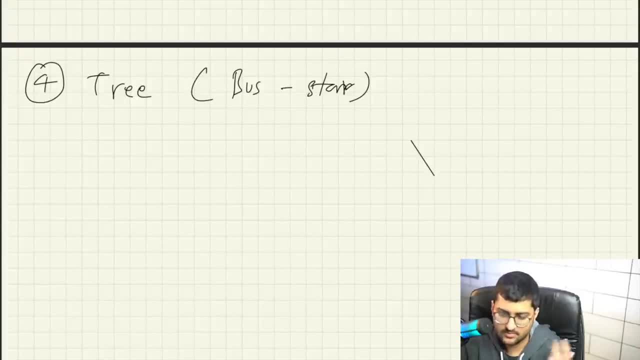 okay so some some some star networks connected like a bus so bus basically contains one single one like this and every single one can have like itself a star topology computer computer computer centralized device computer computer 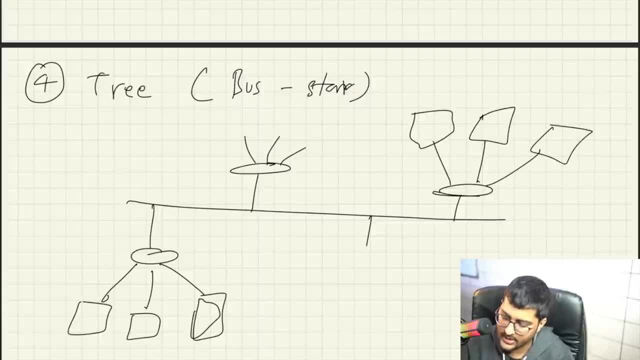 computer so many many stars are connected in a bus sort of a way so little bit has a little bit more fault tolerance and everything number mesh 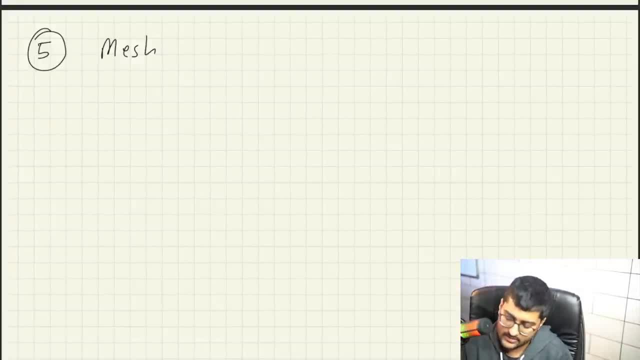 okay so mesh is basically something that every single computer will be connected to every single computer okay 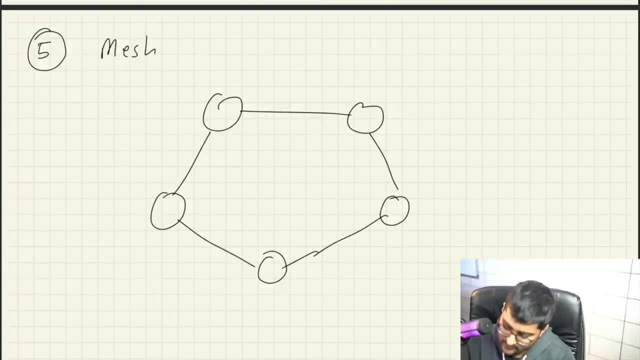 you so every single computer is connected to every single computer what are the 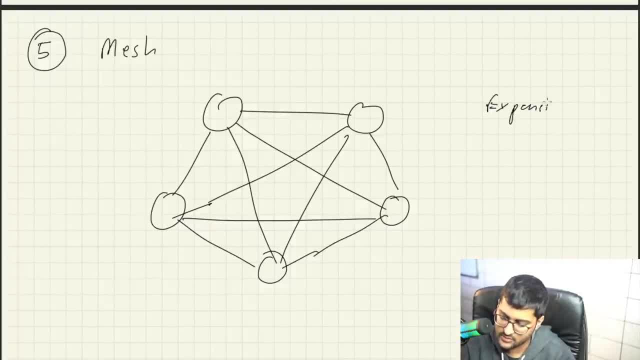 limitations it's expensive so much wire being used okay if you want to add one more computer then you'd have to connect that computer with every single computer 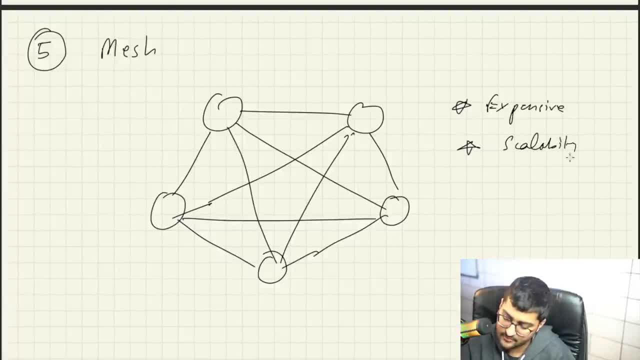 so scalability issues right that's it yeah okay so this was about topologies 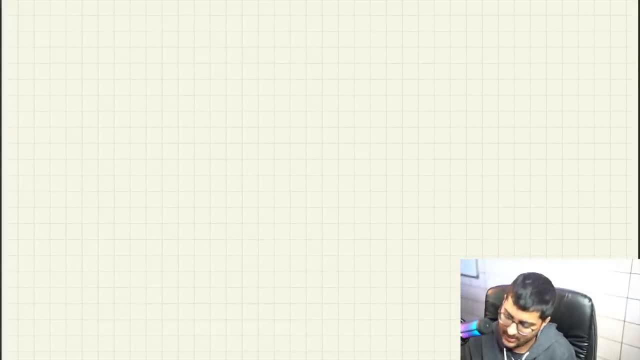 okay now basic stuff are done and now let's talk about the main stuff which is also extremely important a lot of terms I'll be sharing over here that are going to be useful during the you know development of the software and the development of the software and the 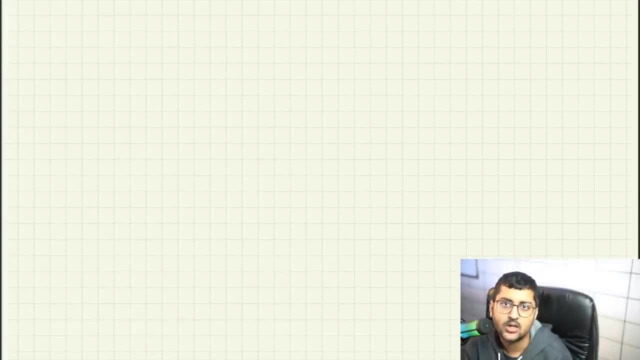 DevOps bootcamp like you know like DNS IP addresses cookies OSI model and all these other things okay now this is a new new like segment of this course now 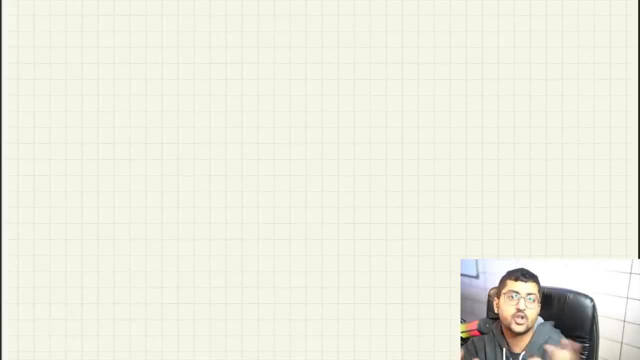 we're talking about the network in like the structure of the network basically okay so structure of network will talk about the OSI model let's talk about the structure of network how things work internally what are all the processes involved 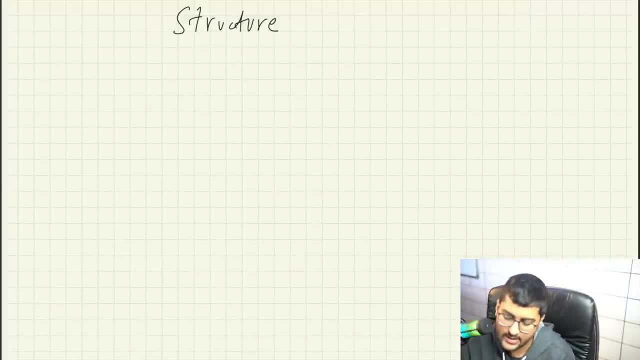 and so many other things like protocols how everything works internally what does it look like we'll see that as well structure of the network let's imagine it 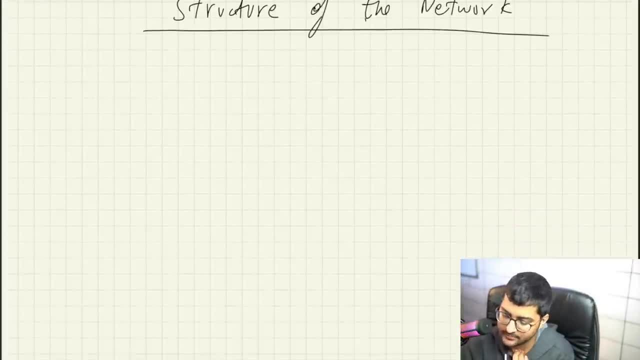 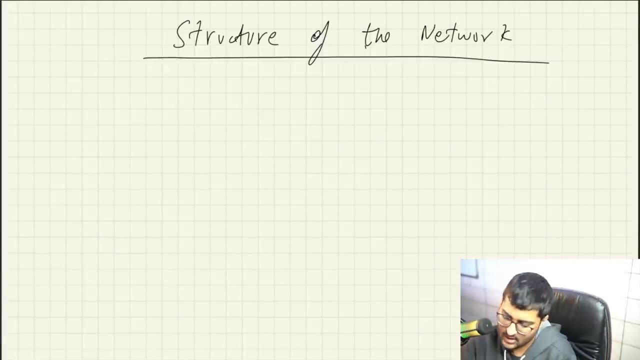 with a real-world scenario because I mentioned initially I'll do that internet is very complex okay we all know that so it would make sense to break it down into smaller pieces okay so how can we break it down into smaller 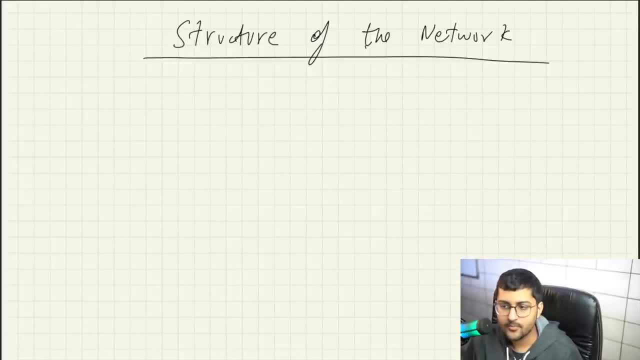 pieces let's see you you order some food okay you order something you order food okay to the restaurant you call the restaurant or you order it on your app and the restaurant gets your order very simple right now you given the order to the 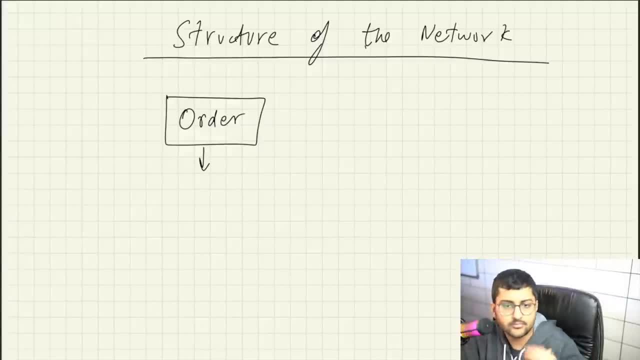 restaurant the restaurant will they will like you know take your order and prepare your order okay so restaurant will take your order and they will then prepare your order for example okay and then they will sort of like let's say you know send it to the delivery agent okay a restaurant example is actually a bit 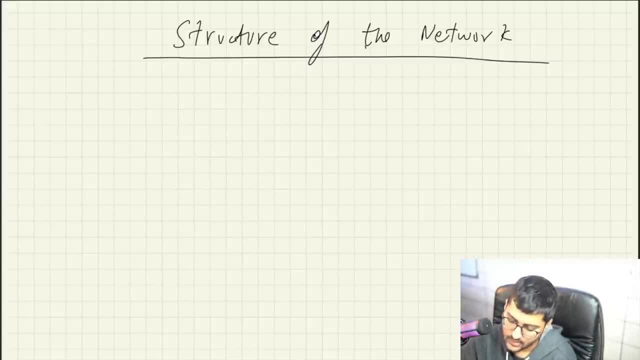 complicated let's say we talk about Amazon okay so you order something online okay you order something online make sense you give it to Amazon and Amazon will be like okay we got it and Amazon will take care of it okay then Amazon is like okay we have got your order and now Amazon 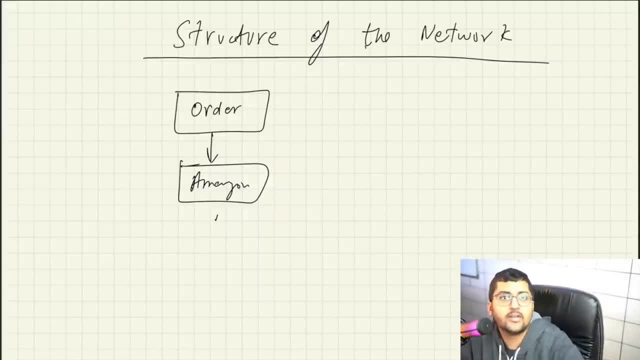 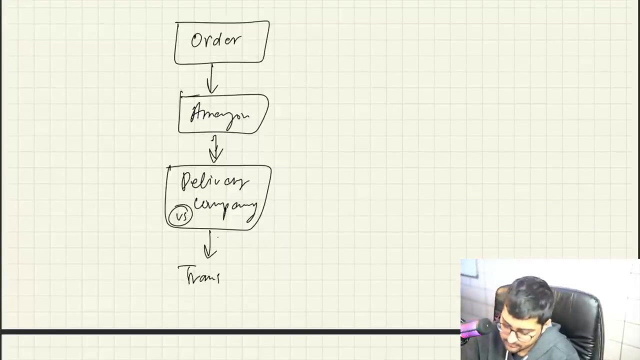 will ship your order to your local delivery agent okay your delivery company is coming from the United States so it will be having delivery company from the United States from their your order will be sent out then your order will be transported transported okay now your order has arrived in India your order has arrived in India it will again be transported into your lives so を 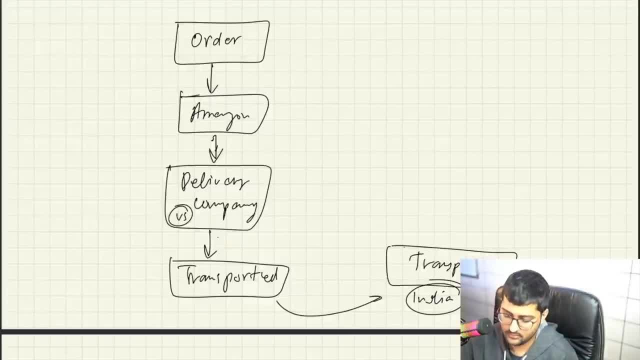 to the delivery company responsible right to the delivery company that is responsible over here delivery company or whatever okay that delivery company in turns will then provide it to amazon like hey amazon um the package is going to be delivered or whatever you can deliver it so let's let's imagine amazon is like directly delivering it and this company is only for 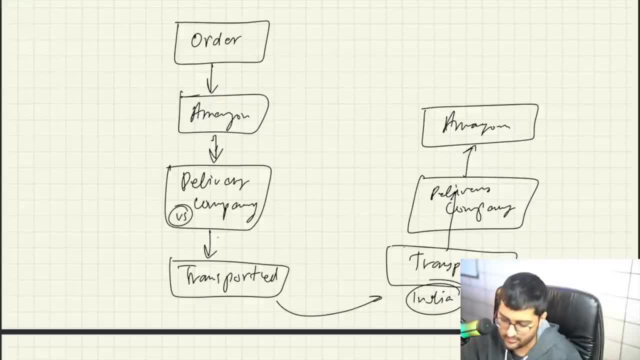 country-wise country-wise distribution okay then you get your amazon from order received okay this is the internet this is how we can imagine the internet 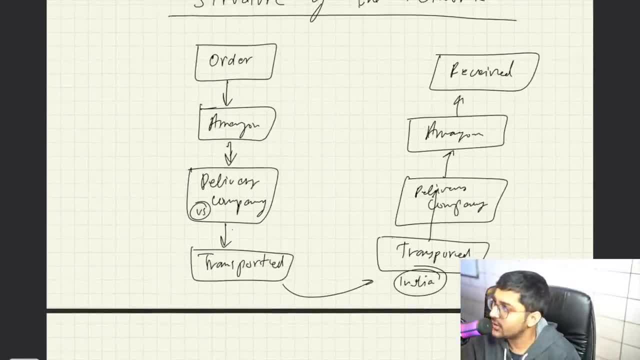 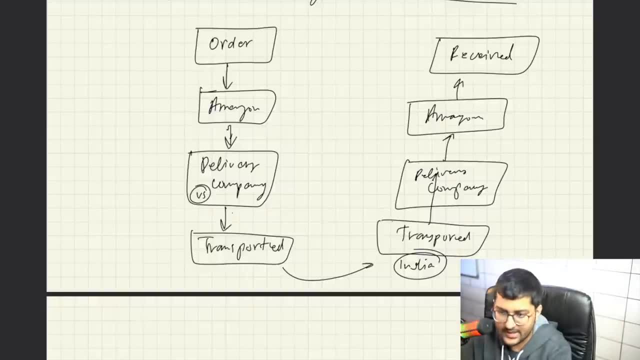 so basically you request some files you request let's say a video from youtube a movie or something right you can you can do that and youtube will take care of it youtube is going to be like okay this is what you want let me see how we can do it it is going to prepare 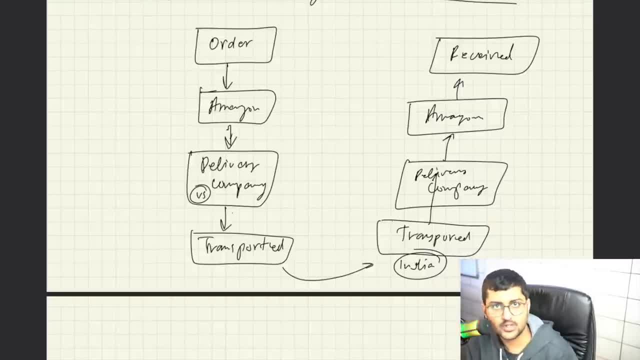 all the data and it will give it to you in terms of transportation from its server then it will reach the server in your country it will be like okay this is all everything and now it's received to you okay so this is basically what we are trying to do this layer where you get the 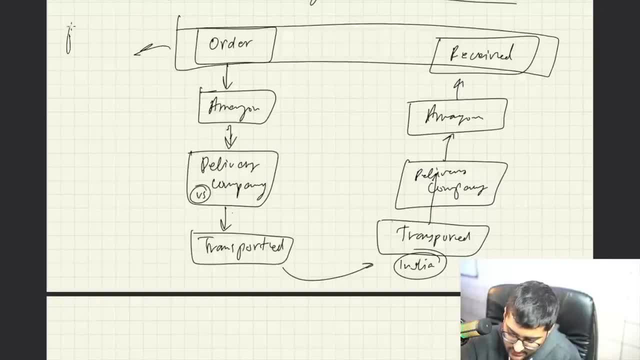 order and everything this is the application layer from which you are able to interacting the very first so application layer can be like your whatsapp messenger 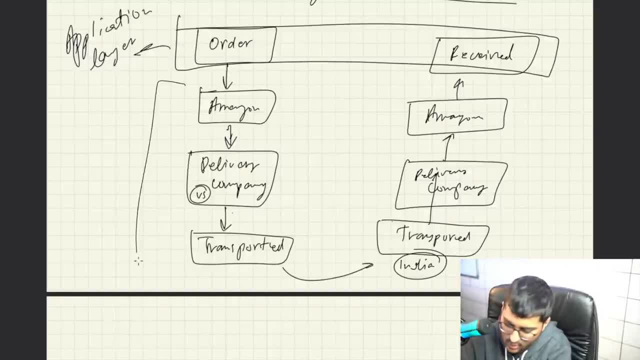 it's an application internally how this complex thing is working do you really know no we don't know all we know is how to use the application whatsapp okay so this was a general analogy 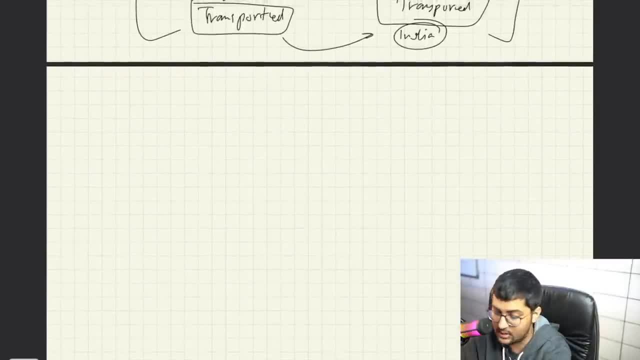 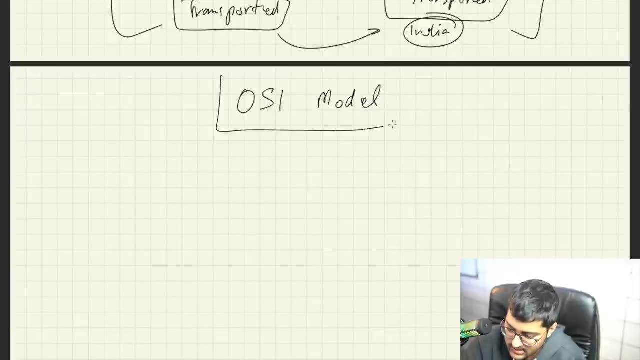 now let's look into the details of it let's look into how this thing works how the internet works is the main part osi model very important part this is how the internet works main part this transportation of data 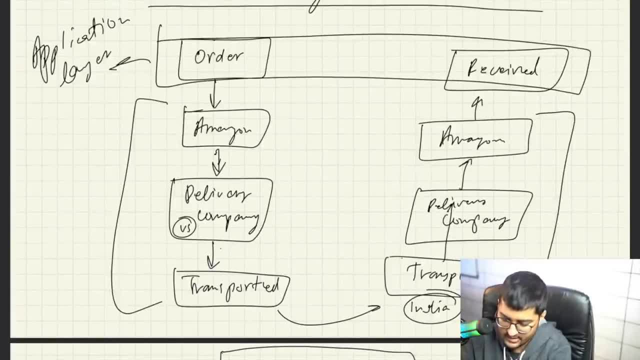 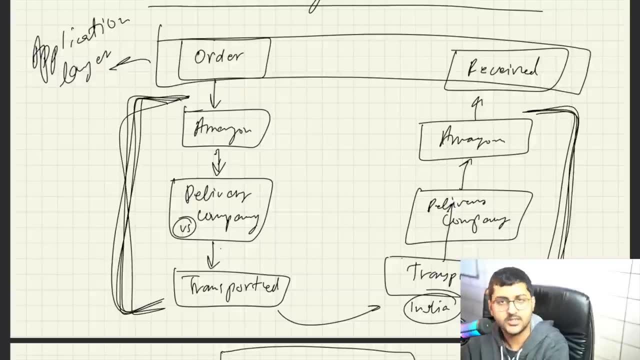 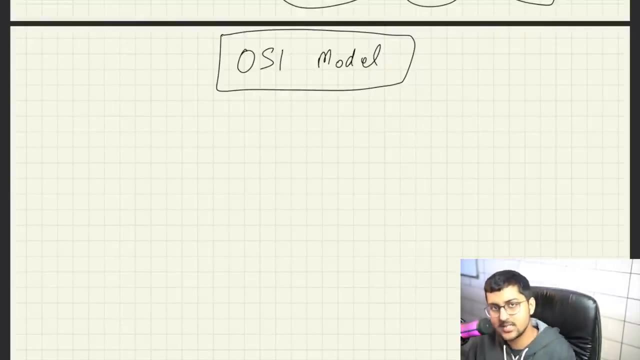 you send a message and the message is received to your friend this this part is the internet okay let's see how it happens okay so let's talk about how it works how the internet works okay so the osi model stands for open systems interconnection model okay so the idea is that uh 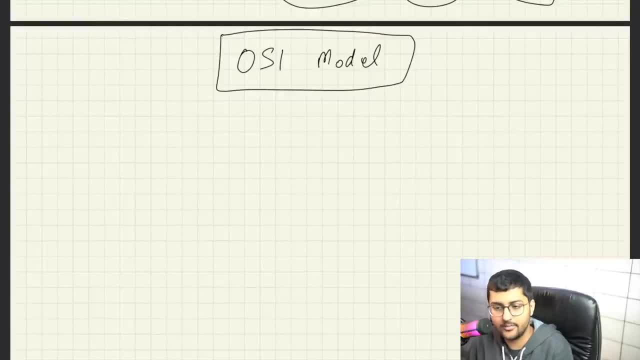 it was developed so that you know uh there was like a standard way 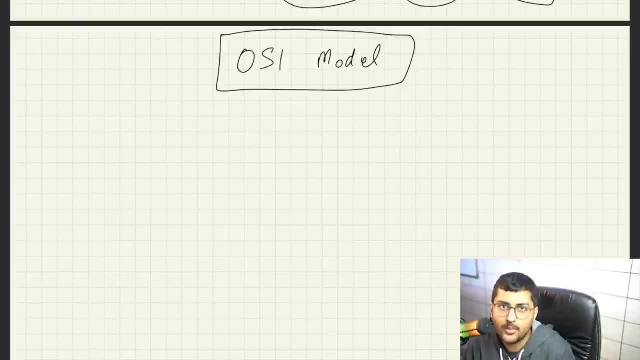 about how to come let's say two or more computers communicate with each other 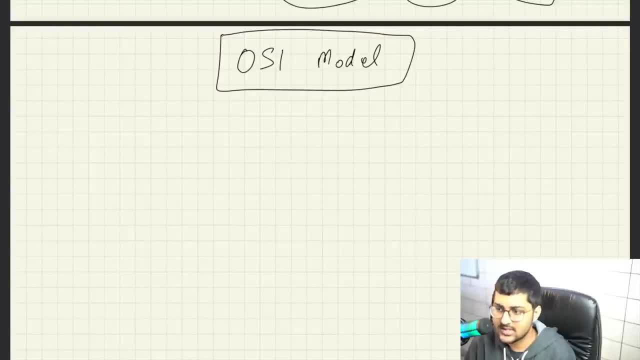 okay sound good so it's just like it's a it's a standard for how people and how servers or whatever communicate with each other okay so there are a few layers in this osi model internet is very complex a lot of things 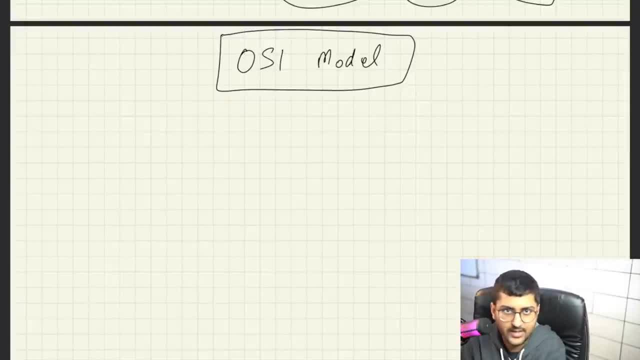 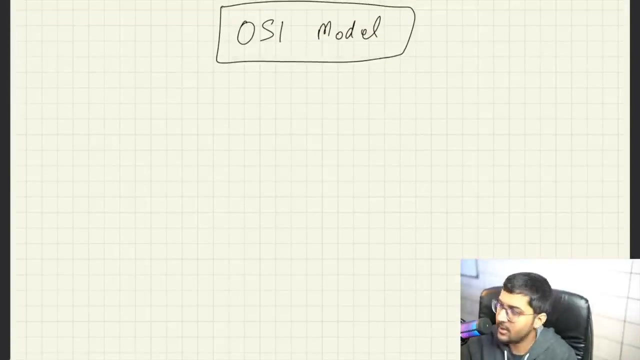 things happen okay so right from checking out an application and a messenger sending an application sending a message that that message will be you know sent to your ISPs or whatever and then it will be sent to your friend in another country and then you will determine which where your friend is which device which application very complex let's divide it into steps okay so there are seven layers in the OSI model how many layers seven layers first is the application layer I'll go into details of every single layer but right now let's look at the overview then we will check it check out every single layer independently okay application layer presentation layer third one is session layer transport layer network layer data layer data link layer and then add the last physical layer OSI model is the most important topic for interviews they ask you ask you in many many interviews my friend was asked about it in the 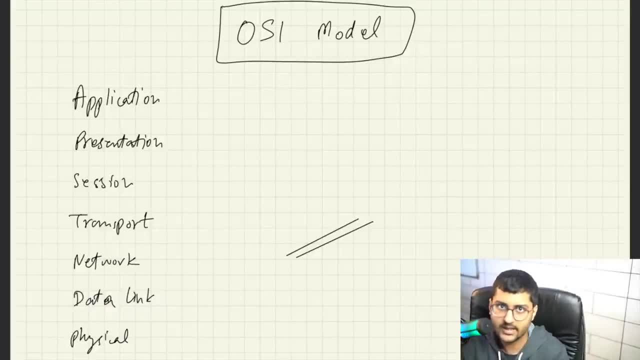 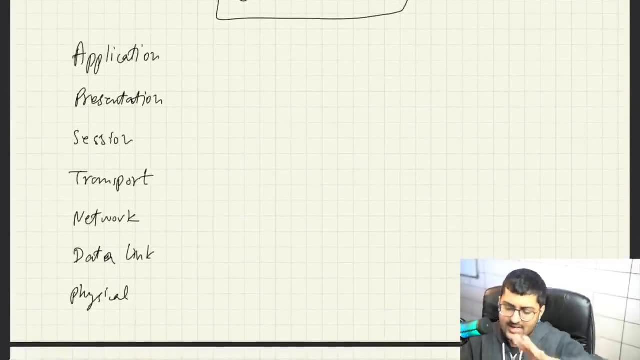 in his facebook interview so OSI model is extremely important please take care of it okay so here are seven layers of OSI model every single layer will have like different like you know protocols and 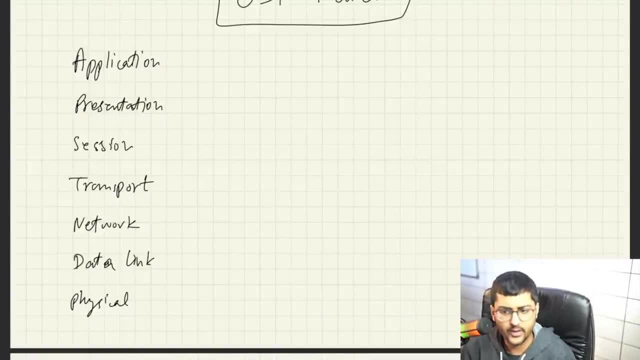 things and devices and everything being used which we'll cover into in details okay so in detail we're 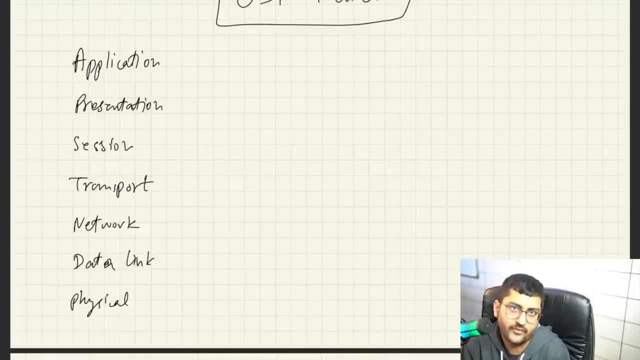 going to cover this thing let's look into the abstract of it first just like in simple terms let's look into it okay then we'll look at every layer in detail first one is the application layer 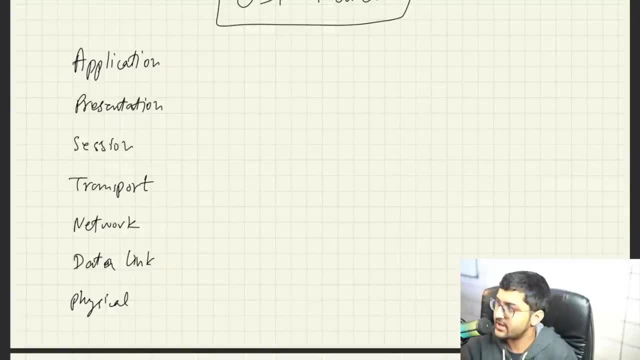 okay let's talk about the application layer what is the application I don't feel like writing I'm just dictating you can write the notes on your own okay so application layer basically 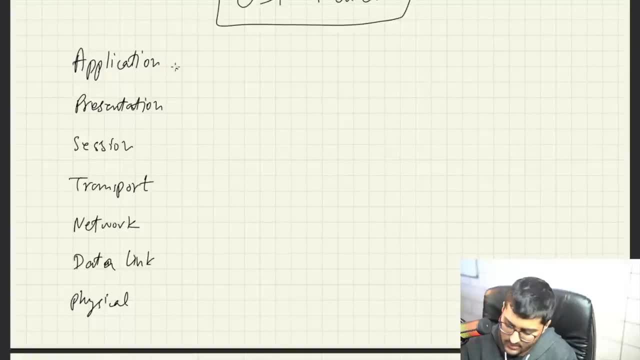 it's implemented in what software it's implemented in software the name suggests it's an application so the folks who are the users they will interact with their application send messages files or emails or whatever application layer contains the 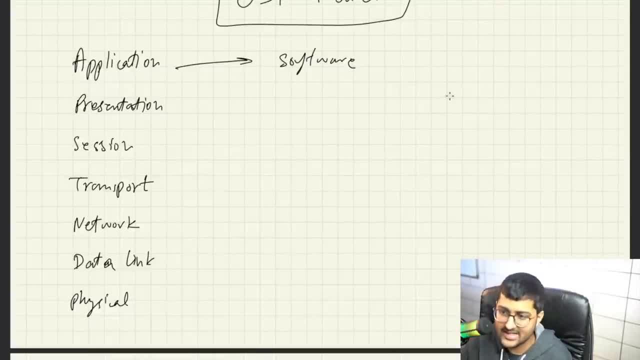 applications okay like browsers and messaging applications and so on and so forth okay so you send your data over from application layer to presentation layer you sent a message 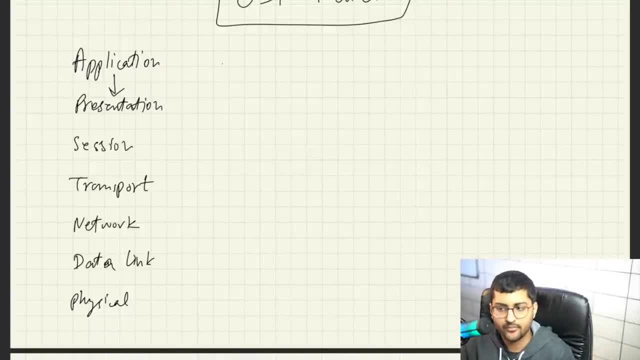 that message was sent to presentation layer now okay now what is the idea of presentation layer so the the presentation layer basically 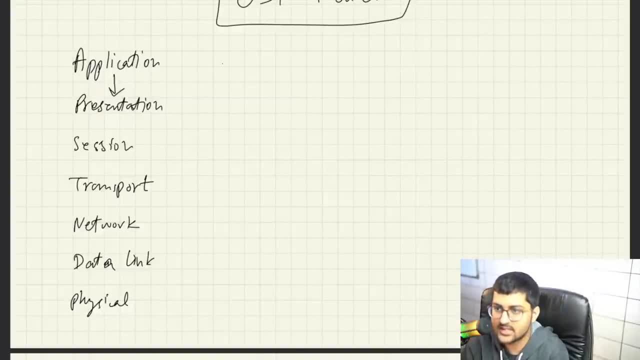 uh so in the application layer when I talk about like having software systems or you know like 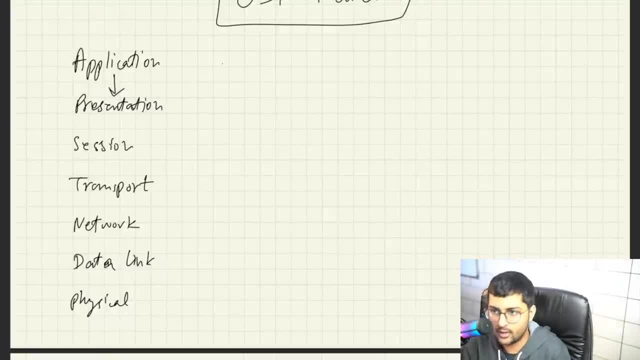 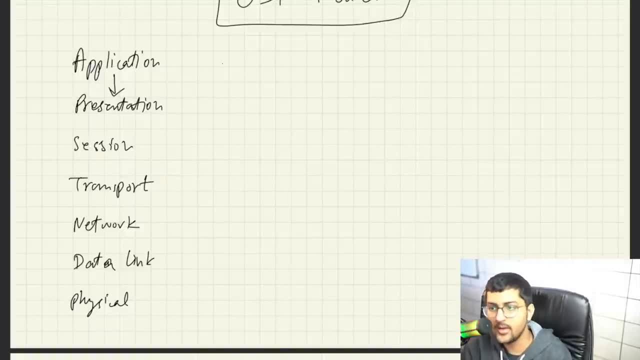 I'll talk more about these protocols later on okay in detail okay and DNS and everything we will talk more about that later for now just focus on the above thing so it will have 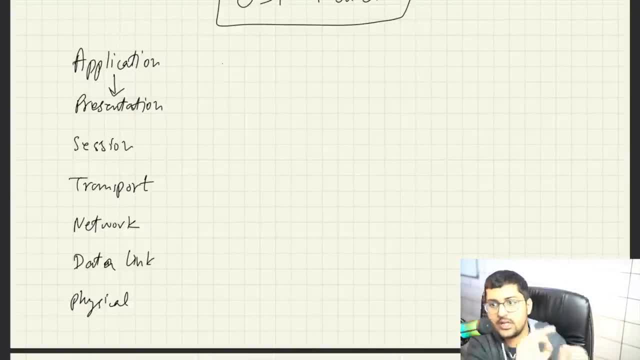 your data it will give the data to presentation layer okay presentation layer take this data presentation there will take the data whatever your message you're trying to send to your friend in another country it will get the data from the getting from the application layer and this data will be in form of what like words and characters and letters and numbers and so on and so forth right so the presentation layer is going to convert these characters and stuff into machine representable binary format okay from ascii to something like ebcdic okay this is known as translation okay a few more things happen so for example before the data is transmitted further it goes 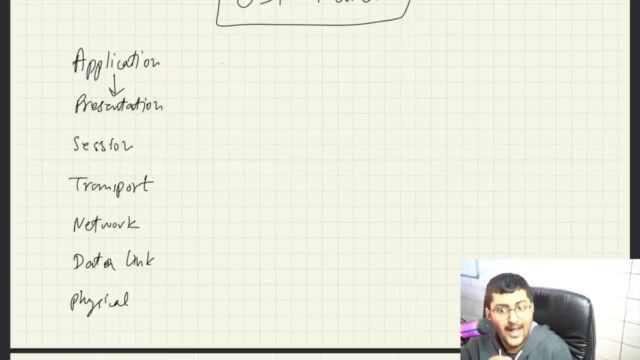 under like encoding like i mentioned i just mentioned encoding encryption okay so changing 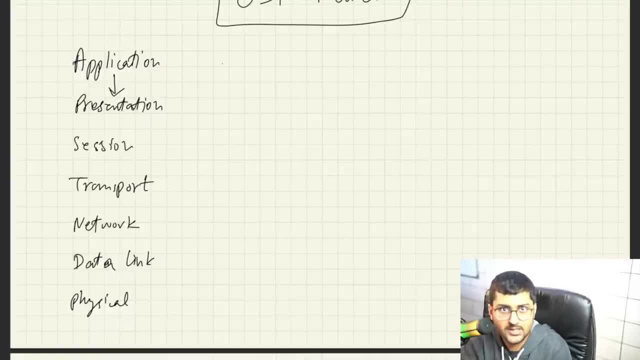 the data so that it's only readable to the person that the data was sent to okay that thing is happening over here how this happens internally you're not like okay you're saying data is 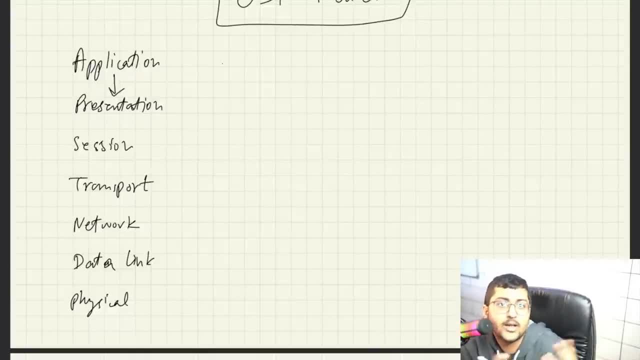 encrypted then how does my friend know how to encrypt or decrypt it or whatever no don't worry 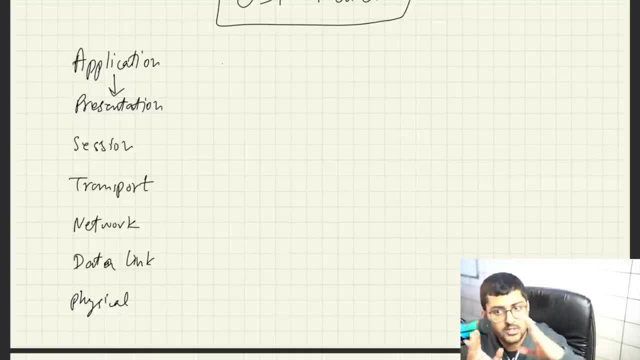 about that i'll cover that later on when we directly just talk about presentation layer right now in this module 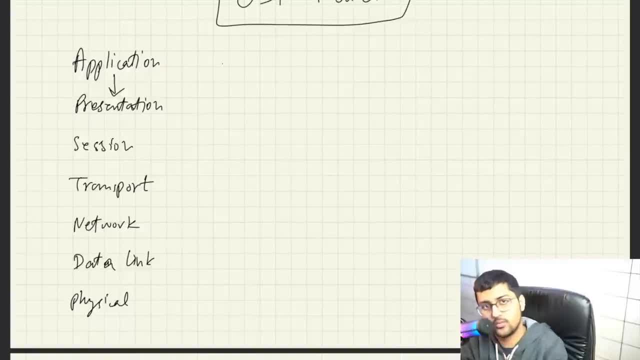 we are learning what every layer does how it does it i'll check out i'll share with you later on okay so it encrypts the data it also provides abstraction okay it also 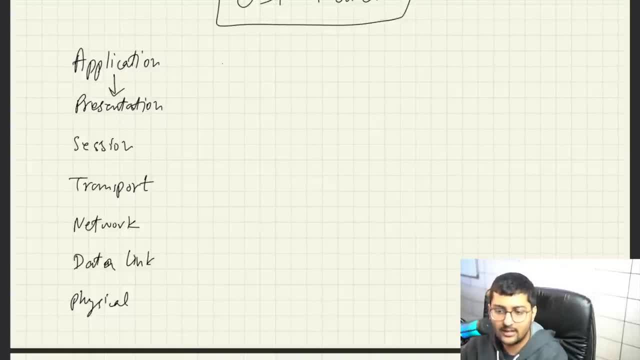 provides abstraction so basically it abstraction i've converted in object-oriented programming but this presentation layer is basically going to assume that if i send the data downwards okay then it will take care of it 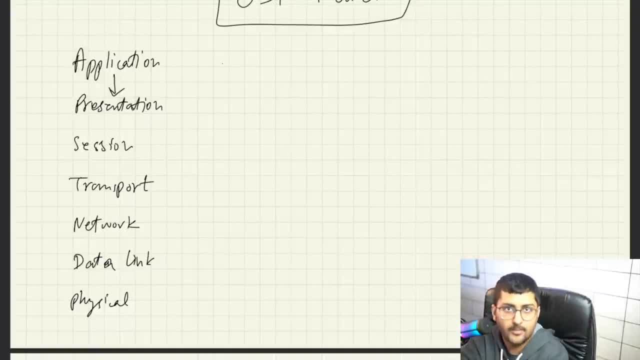 okay the data over here is also compressed so that it's easier to transport over like large distance and like reduce the traffic and everything so data is also compressed this can be lossy or lossless it depends um but like uh yeah so we talked about encryption compression translation right good sound good here ssl protocol is used ssl we talked more 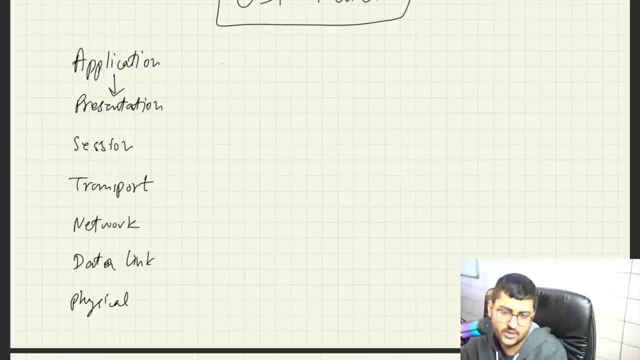 about like later secure sockets layer for encryption and description decryption okay so ssl what is it 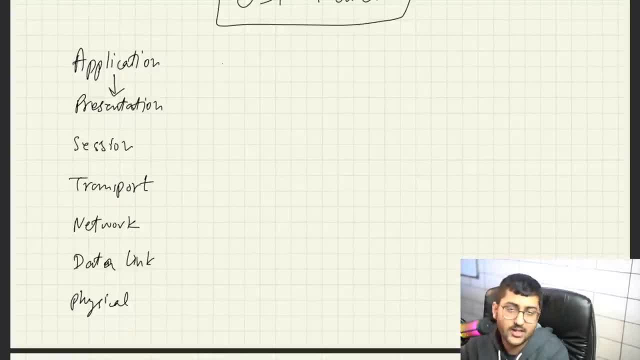 what are these http telnet organelles how many terms you mentioned what are these protocols right now just think of it as protocol right now just focus on what these layers are doing 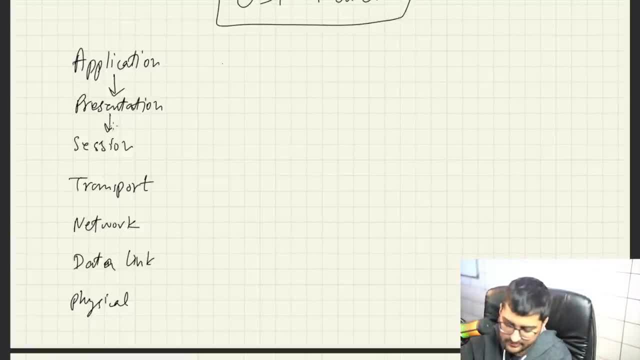 okay then your data is sent to session layer okay okay so then your data is sent to session layer now the session layer protocol basically helps in setting up and managing the connections and it enables you know like the sending and receiving of data 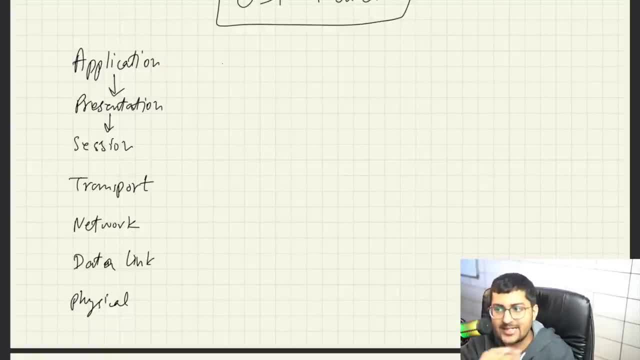 followed by termination of the connected sessions okay so before a session is established it will do some sort of authentication and stuff server you know many times it asks for username and password that happens quite a lot of times 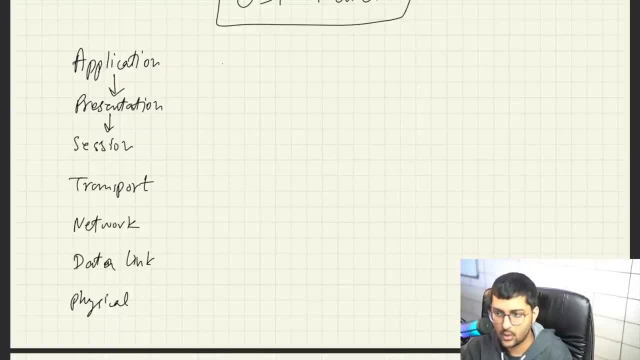 that is known as like authentication okay and then authorization takes place so whether you have permission to access the file on a server or not that depends okay 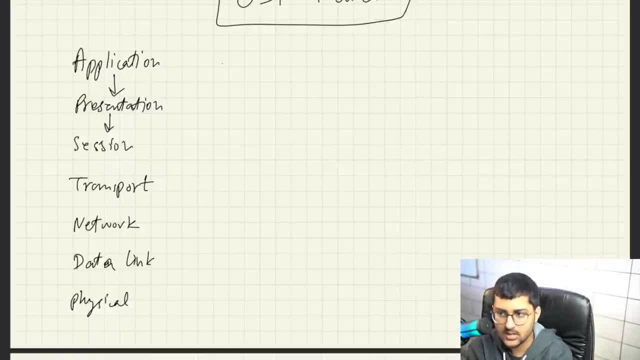 okay sound good okay so with the session layer also this is like the similar stuff session layer assumes that the layers below it will do their work session layer assumes that 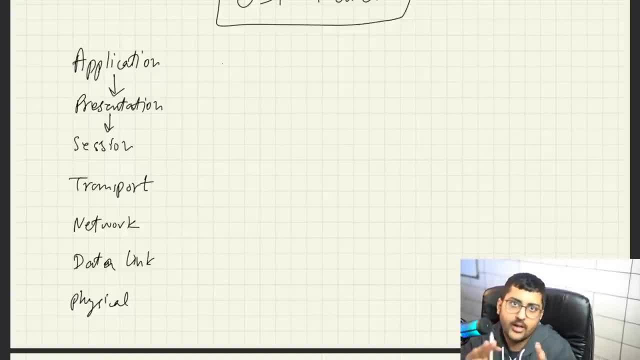 there's a layer let's say transport layer below it and it will be like okay if i just establish a session the data transport station will be done by the transport layer it assumes it so session layers work is this thing okay maintaining so one more example can be when you're 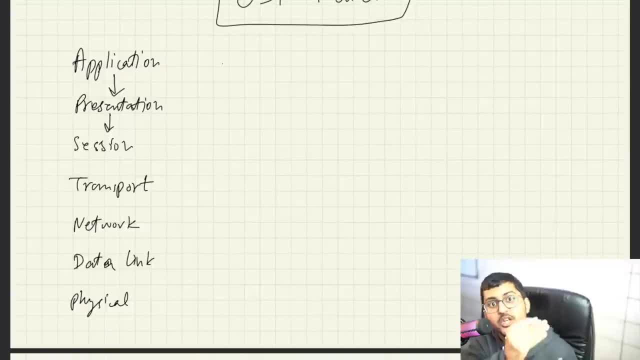 getting from flipkart or amazon.com okay there's a session being created for your computer and the flipkart server or whatever okay and when everything happens it logs you out and payment is done that's basically the idea of session layer okay how it works internally 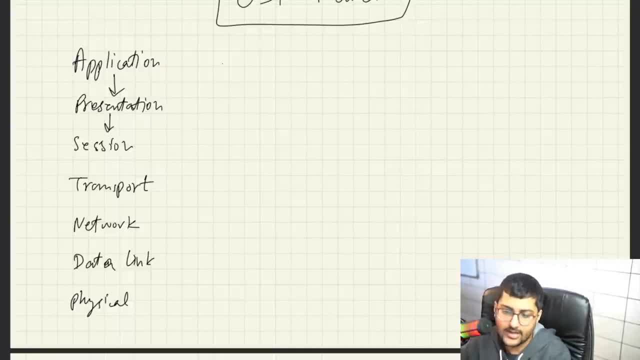 we'll we'll obviously look uh look into like later on the data packets are used and everything is used so on and so forth okay cool next is the transport layer so data is transferred 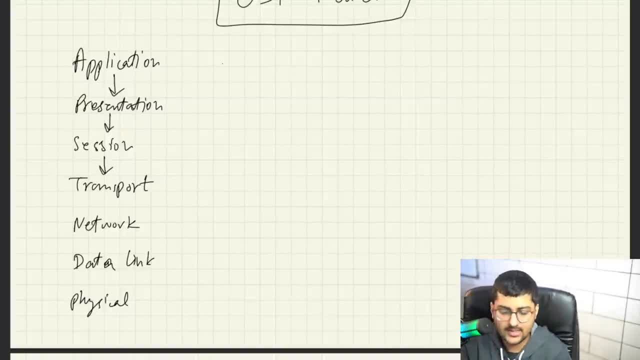 from session layer to transport layer now transport layer basically it's like okay transport is going to be application layer got some data and then it presented that data then the session was established and now it's my part to work with this data and make sure it's transported to the friend easily okay so it has its own like protocol of how data 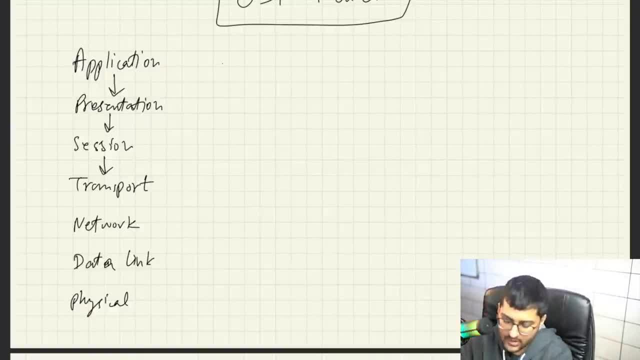 will be transferred like udp and tcp after this overview i'll tell you a little bit more about protocols okay so protocols are nothing but how data is transferred okay so it does it in three way there's one part known as segmentation so data that is 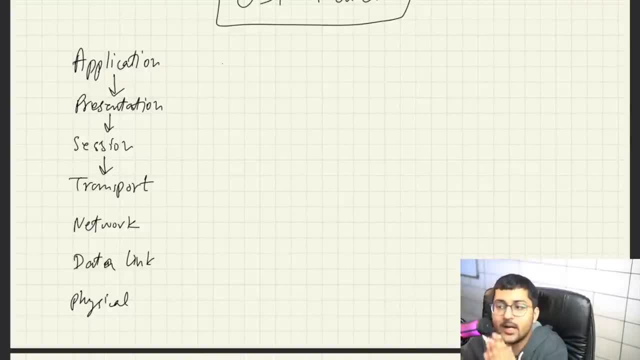 received from the session layer it will be divided into small data units called segments okay and we talked about port numbers right so every segment will contain the source and the destination's port number and a sequence number port number we already know what it is right so correct application the data will be received to the correct application like whatsapp or google chrome or whatever sequence number basically helps to reassemble the segments in the correct order we all know that all the data will not be transferred as once it will be transferred into chunks for that it has a sequence number i'll actually show you this sequence number also we'll have some commands lined up okay the next thing is flow control flow control basically transport layer controls the amount of data that is being transferred so the server is you know having 40 mbpns but the client has server is sending at 40 mbps but the client is really receiving at 20 mbps so then that's not correct so the data is not going to work okay it will be like hey slow down also one more thing it works on is error control some data packets got lost or corrupted data or whatever so how it works with that this is also something we'll see in detail okay when we learn about transport layer in detail right now i'm just telling you the overview okay and it adds 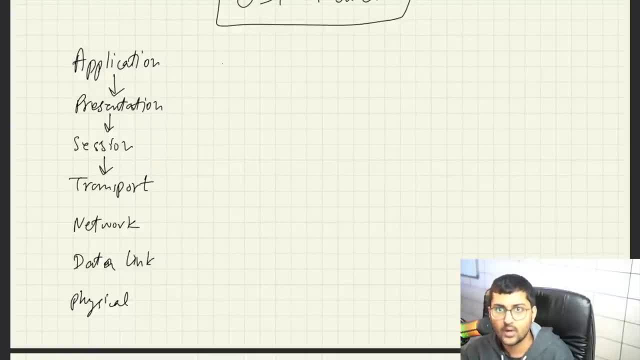 something known as a checksum to every data segment okay that way it can figure out whether the data that was received by a friend was good or not okay 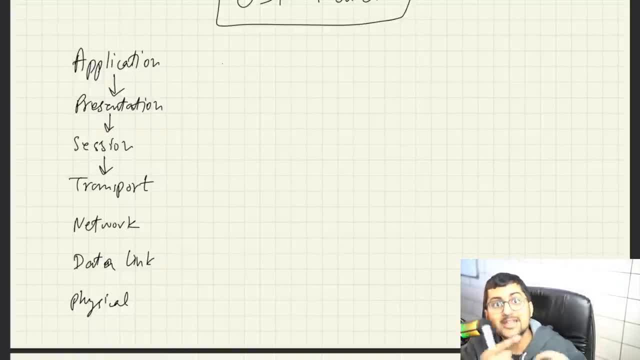 so there's like a connection oriented transmission like tcp and there's a collection connection less oriented transmission called udp udp is faster because it it does not provide any 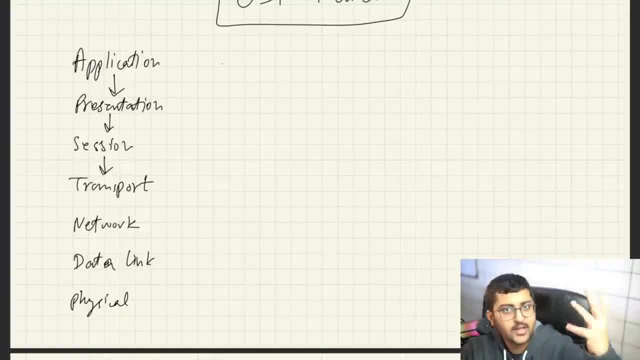 feedback if data is lost or not it's like okay whatever data you're sending keep sending that is why some data packets get lost in udp 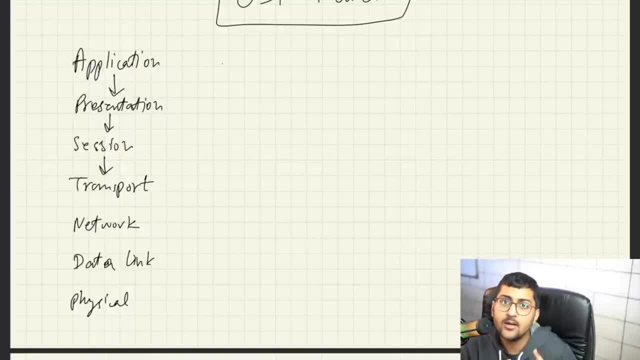 for example video conferencing or gaming but in tcp it's like when your friend receives the data your friend will send an acknowledgement hey kunal uh internet i've got the data you're 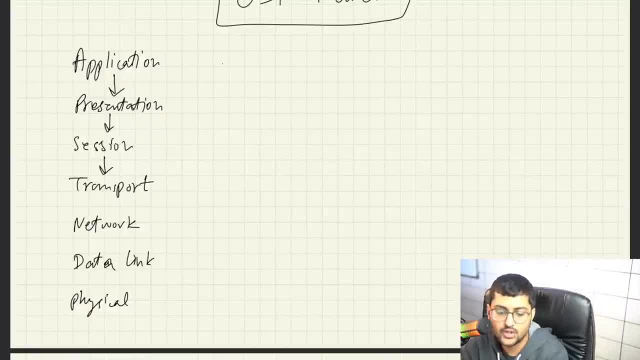 it means 100% data transferred don't worry so uses of TCP like email and file transfer protocol so 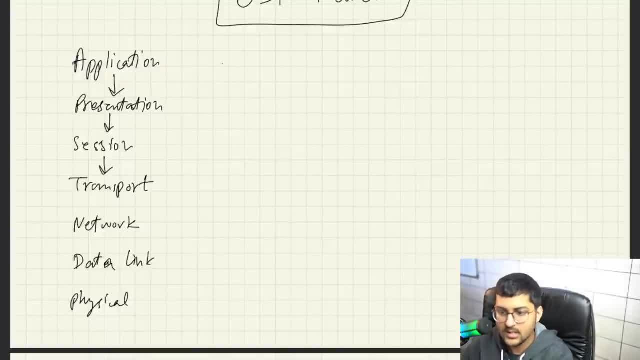 on and so forth okay so that's basically about you learn more about like checksum and like segments and all these other things later on after that what happens is it gets transferred so in here 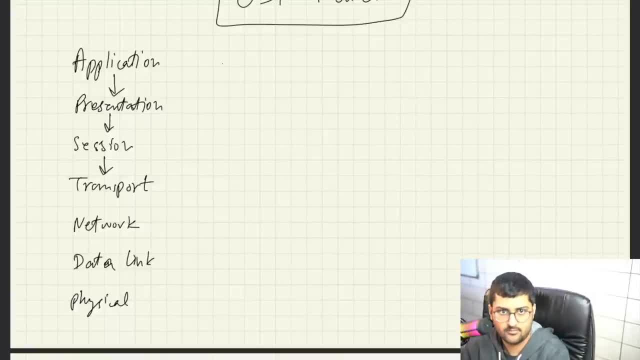 we'll be learning about UDP and TCP okay please make notes yourself okay I can like in I don't wanna like ruin it but please make like notes yourself and I have sharing everything so you can make like make make notes yourself okay so now we come at network layer so network layer is 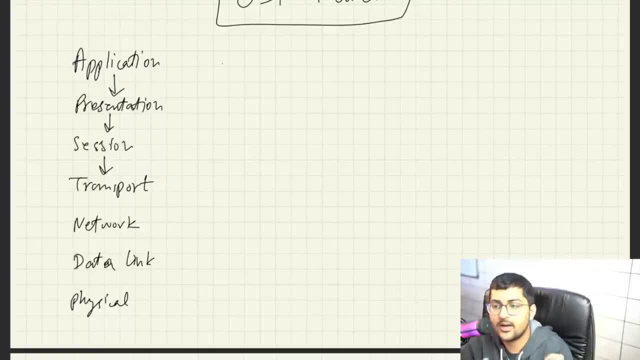 pretty simple so network layer basically works for the transmission of the received data segments 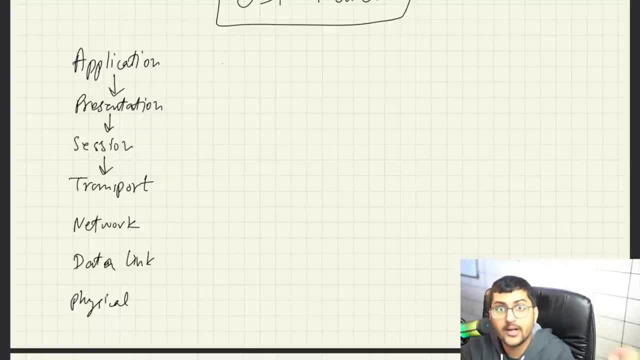 from one computer to another that is located in a different network okay so basically here till now here we are talking about the network layer and the network layer is basically the network layer 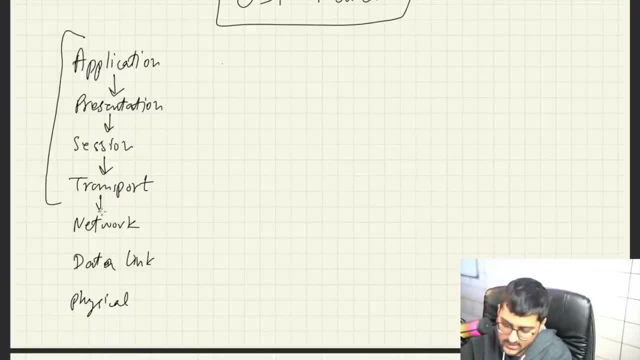 right now but now when you're talking about sending this to the network layer now this is communicating communicating with other computers outside this is where the router lives router lives over here router lives over here okay make your own notes from video 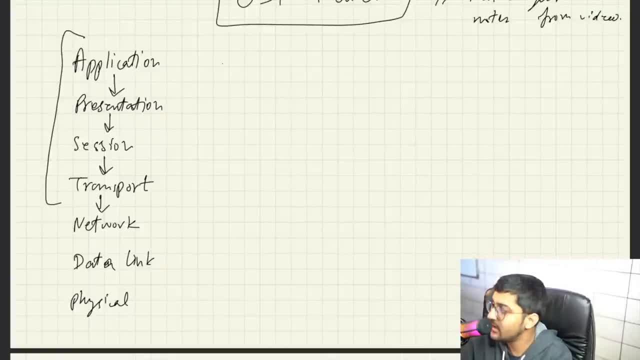 okay so this thing like router lives over here and stuff things like that you can make your own notes okay what is the function of network layer logical addressing so IP addressing done in the 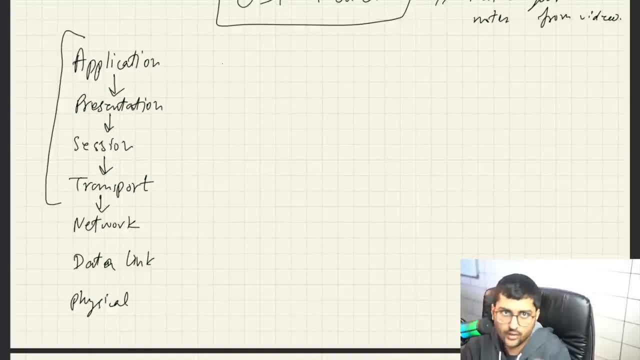 network layer is known as logical addressing because you all know every computer has their own IP address network layer assigns the senders and receivers IP address to every segment and it assigns the senders and receivers IP address to the packet the data packets that it's receiving so that every data packet can reach the correct destination okay sound good and also it performs 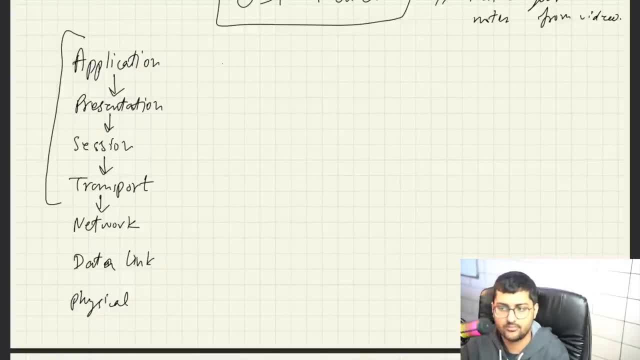 routing so moving one data packet from source to destination okay it's based on like IP like IP addresses and things like that okay 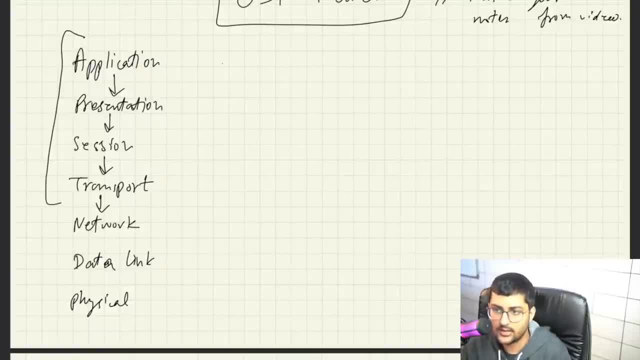 cool so it performs some sort of a you know like logical addressing and then it will transport the data okay we'll learn about how it does it in detail like subnet masking and routing from packet 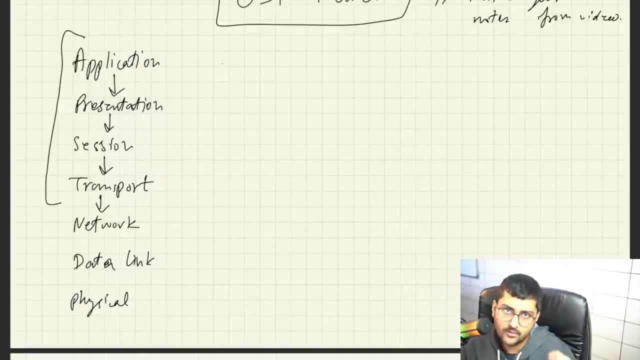 1 to packet B how it happens internally everything will cover later on okay okay so it determines like okay Kunal you know you have your own network computer and there's your friend's computer or 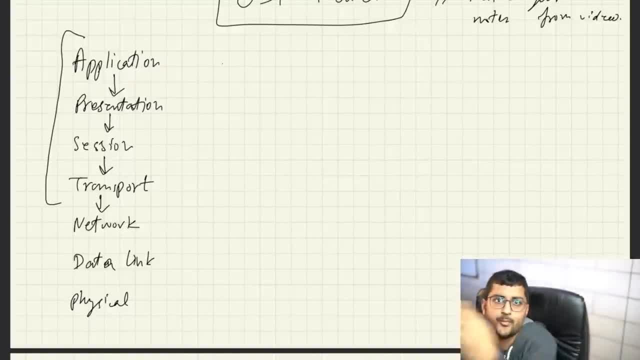 what is the best path to take to send from data from your computer to your friend's computer what is the greatest path like I can take some routing protocols and stuff this is a distrust algorithm that it may be using which we'll learn more about later so all these routing protocols and like transportation of packets and everything happens at the network layer load balancing also happens over here right to make sure that this it's not overloading okay cool after that the data is transported to data link layer 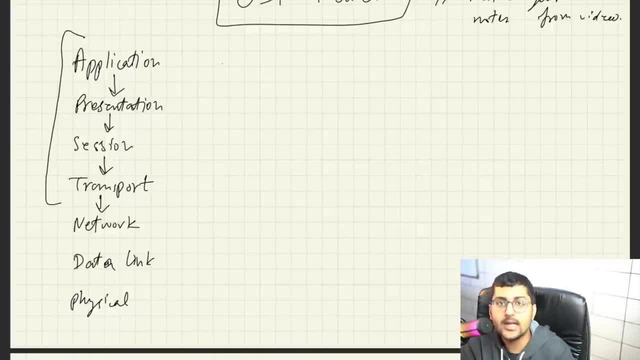 basically allows like you to directly communicate with the computers and hosts okay okay so data link layer will receive the data packet from the network layer and this data packet contains the ip addresses of both the sender and the receiver which we already talked about now the data link layer it's actually doing two kinds of addressing logical addressing that is done at you know like the uh like the at the network layer which is about ip addresses and stuff um so when the sender and receivers ip addresses are assigned to form a packet so let's let's draw this only okay no 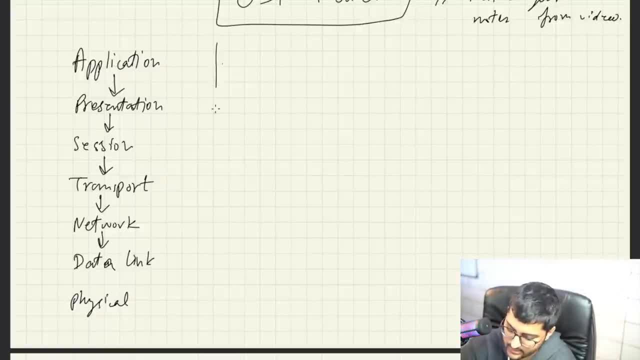 problem no problem we can draw this particular thing how it works at the network layer okay no 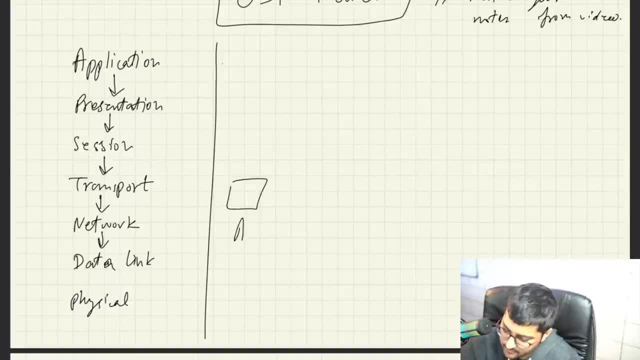 problem so we have your own computer you have your computer a okay you have your computer a it has a 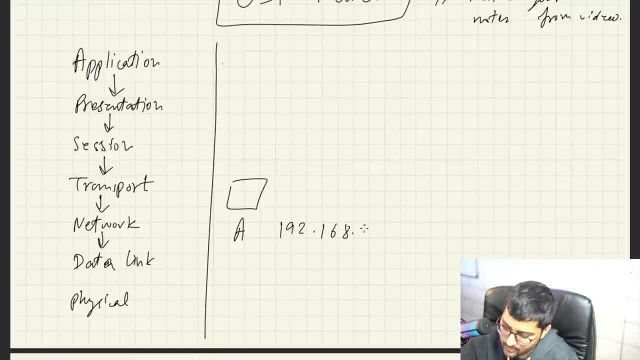 ip address of let's say something like uh 168.1.1 okay it is connected to your network like this network number 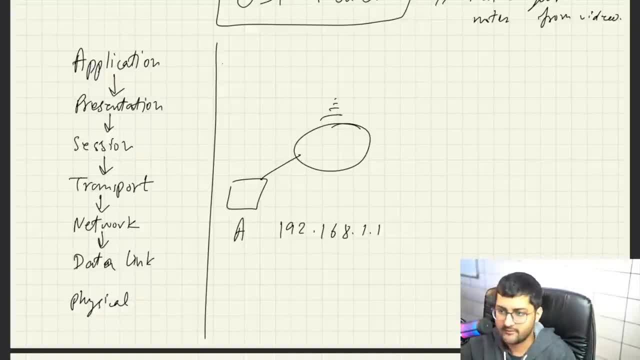 one your wi-fi okay it's connected to your wi-fi now here it's sending a message to let's say facebook okay the data packet okay so a data facebook will have its own server like 192.168.3.1 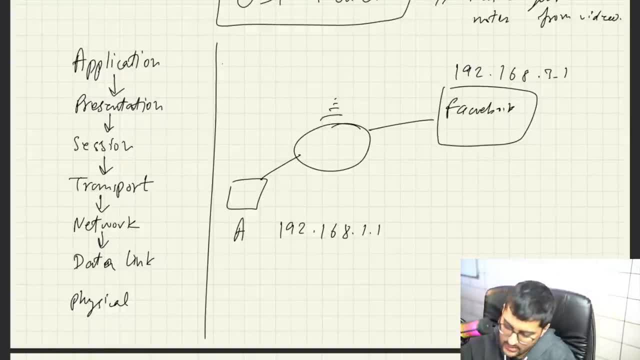 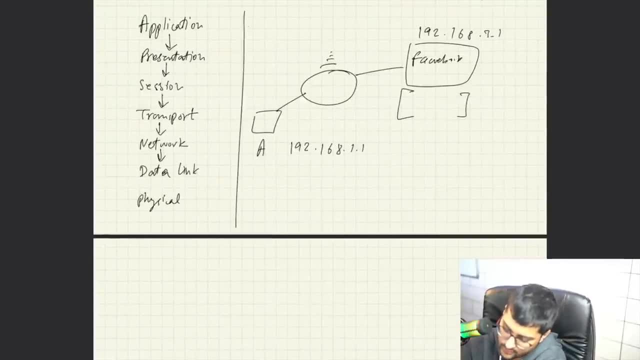 for example it's the ip address of the facebook server every packet will contain three things it will contain the sender and receivers if this is a receiver i have to draw it somewhere over here 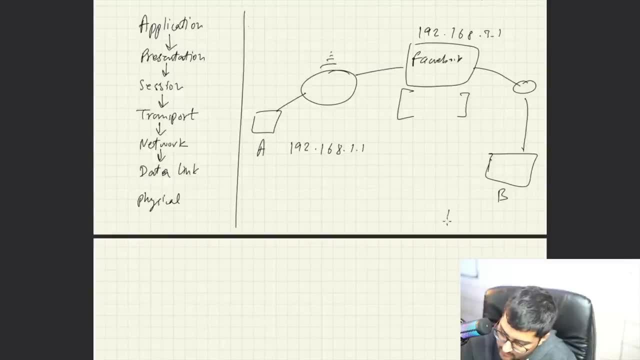 if this is a receiver okay computer b 192.160.2.1 okay so this ip address 192.168.1.1 192.168.2.1 and a subnet mask which i'll talk more about later subnet 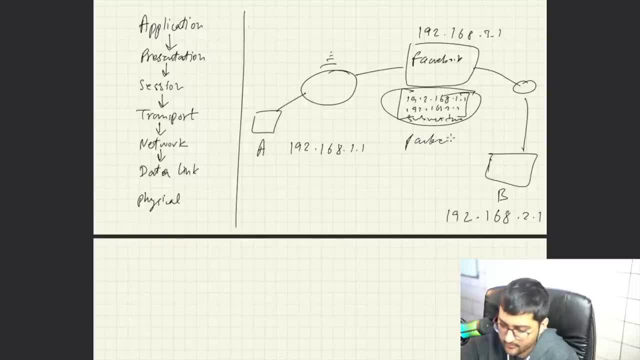 mask this thing is known as a packet so as you can see whenever a packet is transported like this it it will be like having the IP address of sender and receiver okay now it will be transported to next person that is basically how it works so in data link layer what happens is when you receive the data over here this will obviously be at the network layer once you have received the data and whenever you are working with routers or whatever that's network layer but 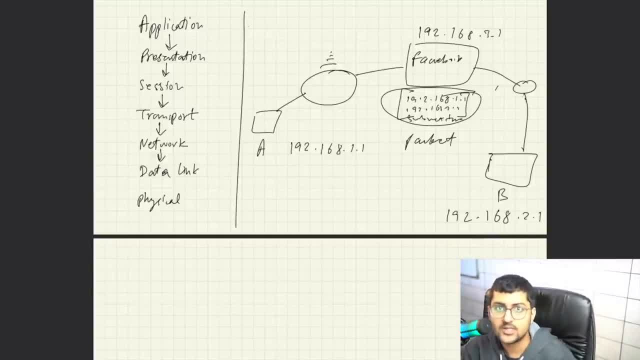 now the idea is which application to send this data to there is not a physical addressing 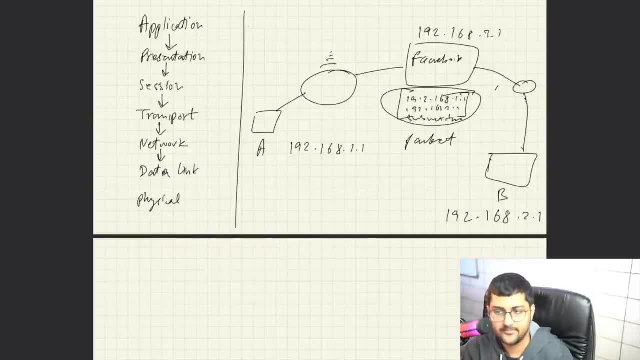 this is done as done at data link layer the physical addressing not the logical networking addressing no the physical addressing and what are the physical addresses you may have heard about those MAC addresses okay now MAC addresses of sender and receiver are assigned to the data packet MAC addresses okay to form a frame so frame is basically a data unit of the 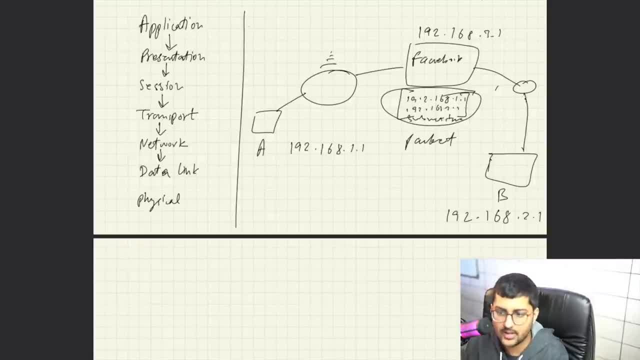 data link layer what is a MAC address you may ask MAC address is a it's a 12 digit alpha numeric number of the network interface of your computer it's not like your computer has only one MAC address no your computer's bluetooth may have some other network and a MAC address your computer's wi-fi may have another MAC address so on and so forth okay 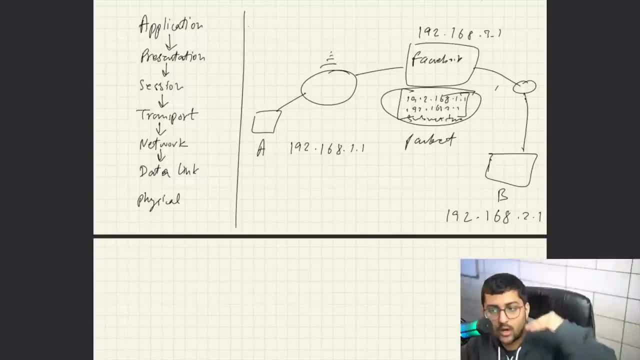 so data link layer performs two functions it will allow the all the upper layers of the OSI model to access the the these frames and stuff like it will pass on these frames whatever things that I just mentioned and it also controls how the data is placed and received from the medias using such using things known as media access control so basically techniques used to get the frame on and off media and like error detection and stuff okay things like that so what does 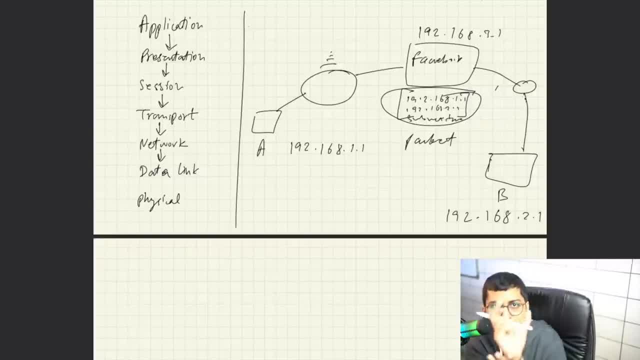 data link layer do when our data link layers adds MAC addresses in a frame and in a packet calls it like a frame and pushes that frame and like you can then transport that frame 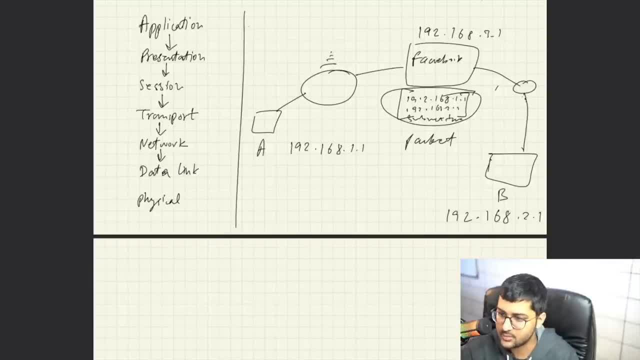 all right I'll cover this in detail later on but let's move forward okay and then in the end we have our physical layer okay physical basically contains of hardware this is the 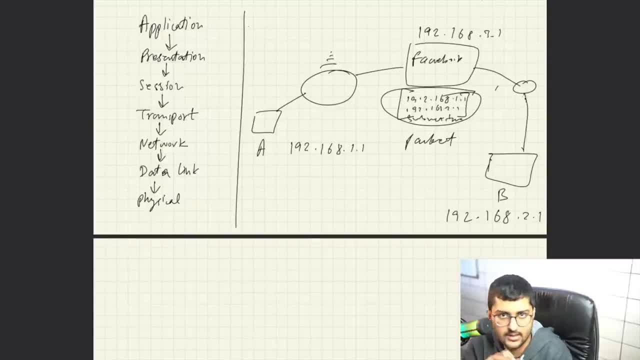 hardware section and here you actually have like you're some mechanical like wires or something mediums and here it transmits the bits from electrical signals it does not have 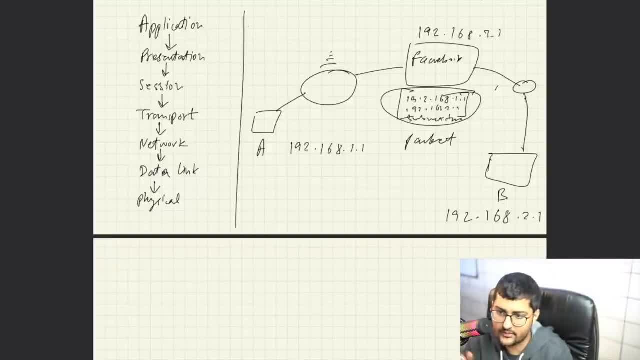 like packets or do space hazard that the model this is the如何 to convert or let's say some illegal bottels parts you can choose that and it fast forward and you'll find as many as or datagrams like segments and things like that we talked about so you work with uh cables and stuff 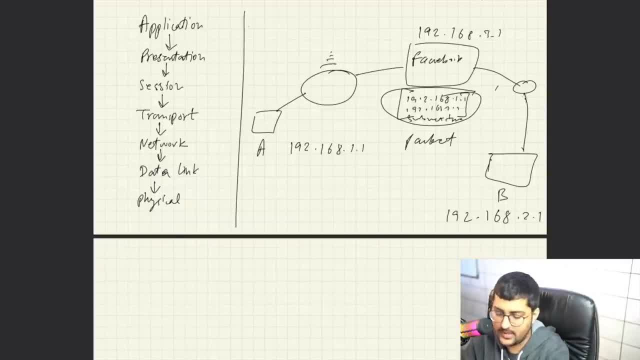 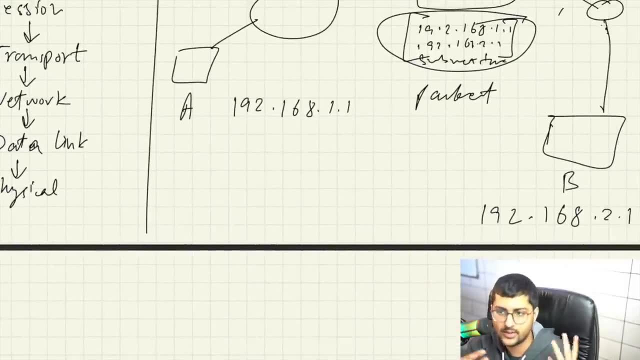 in this okay so data that you get from the above it will be like in the form of zeros and ones physical layer is going to convert this into you know and transport it over like wires and your local local media it can be like an electrical signal or something a light signal in the optical fiber cable or whatever or a radio signal in case of wi-fi or something okay so the physical signal uh the physical layer receives the signal converts it into like some at the receiver section okay so 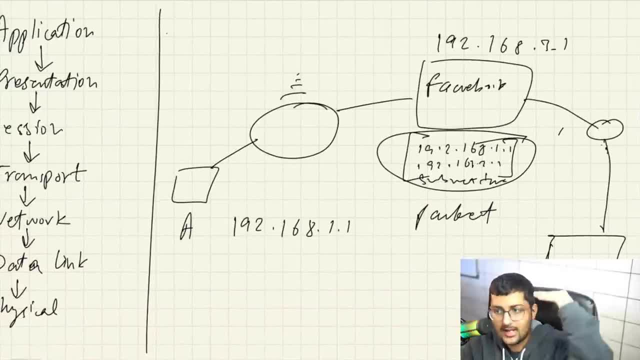 when the data is received to someone okay at that particular point of time the physical layer will 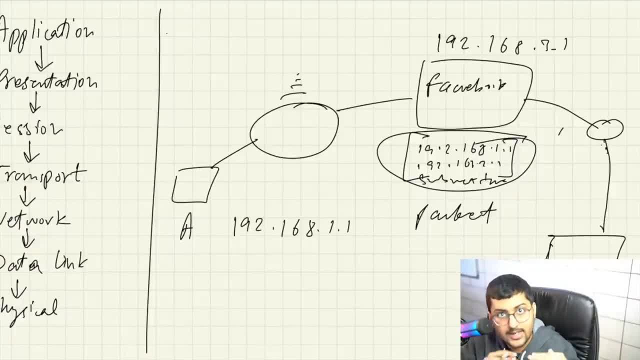 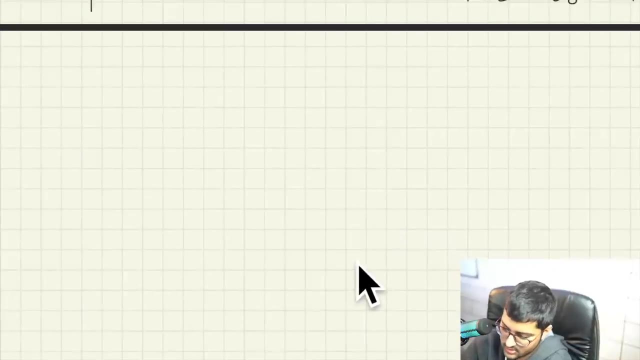 receive the signal convert it into bits pass it to the data link layer as a frame and then frame will be you know move to higher higher higher layers let's look at how it says things works like the order of execution how everything works okay let's see how this thing works a little bit easily so i'm just gonna i am going to write it over here so you send a message this is you 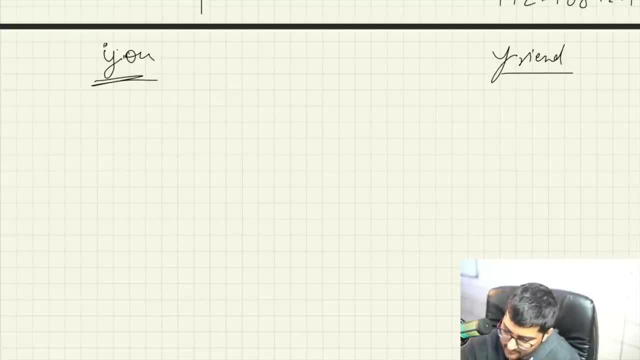 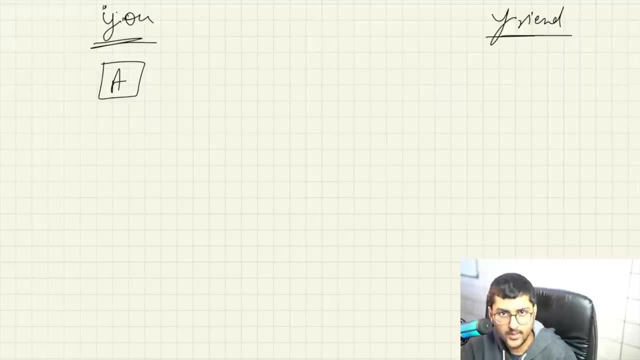 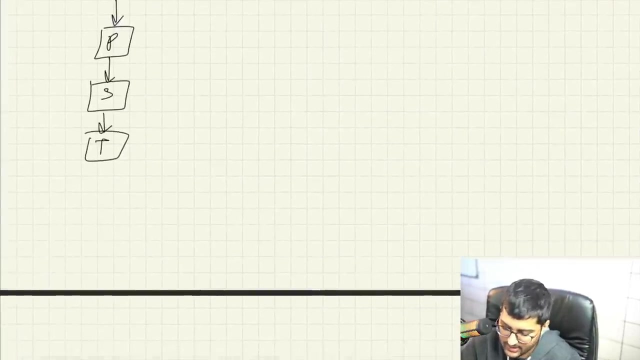 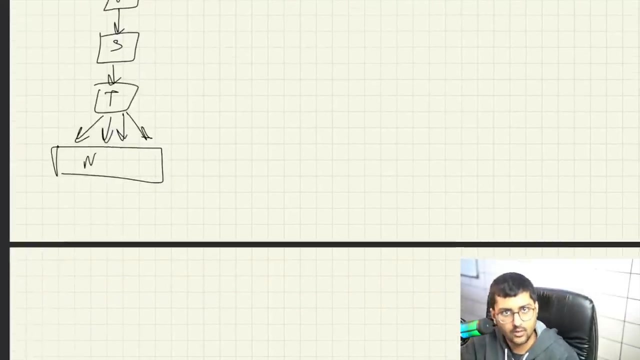 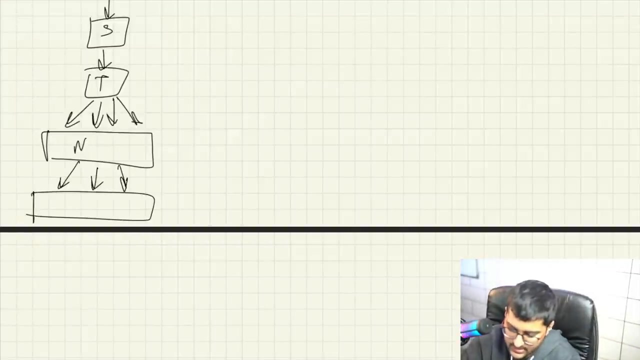 and this is your friend okay how it how this thing actually works so you have your application layer okay it will transport the message to your presentation layer okay the presentation layer will do its thing transport it into the session layer session layer will transport it into the transport layer and transport layer will make it into like packets and segments and stuff so divide it into like packets and stuff into the network layer okay network layer will also bundle it okay assign the ip addresses so network layer assigns the ip addresses sends it into the data link layer data link layer will assign the like mac addresses and stuff and send it to the physical router okay now your physical router will send it to the physical router of your friend via that okay so your physical router of your friend you can see this is not happening like directly i'll just show you right now okay so 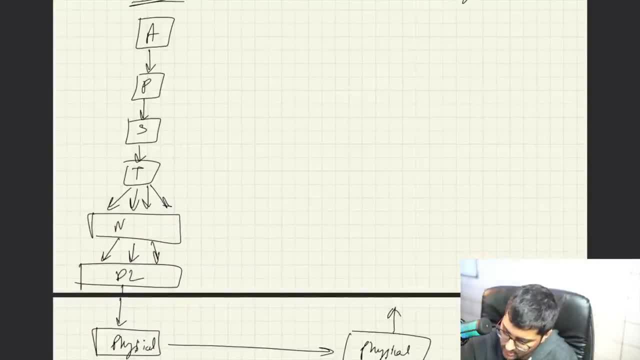 how the ip addresses are resolved and everything we'll cover later on okay so your physical layer it will be like in your data link layer now it will give it to data link layer data link layer will give it to the network layer okay network layer will give it to like the transport 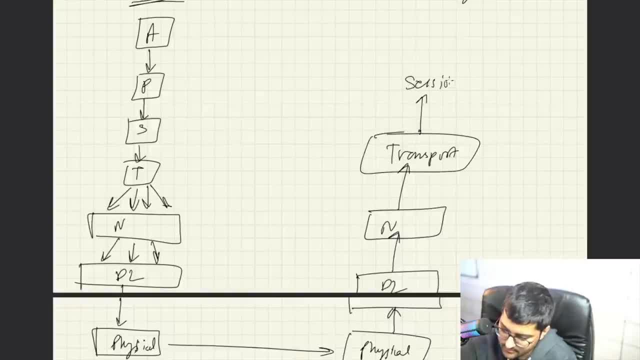 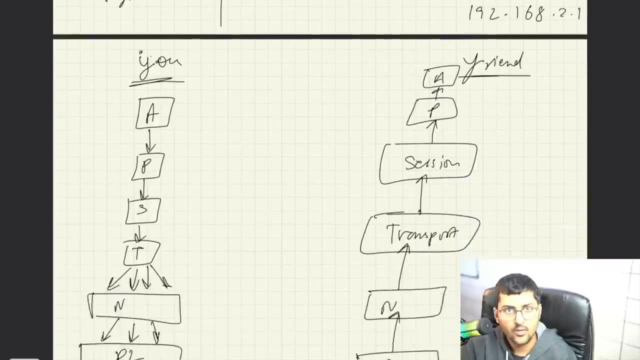 and then transport will at the session layer okay session to presentation presentation to application and your friend will receive your message presentation to application okay this is how it works each layer it will be like okay 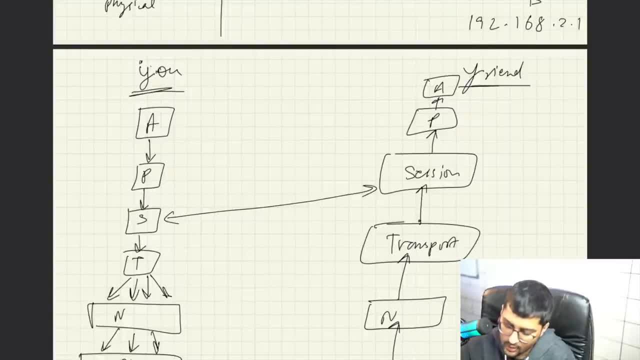 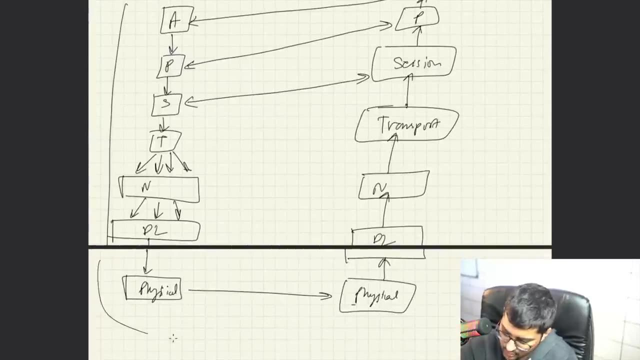 it will imagine that i am talking to the session layer of my friend or i am talking to the presentation layer of my friend or me if my friend are chatting on whatsapp so we'll be like i am talking to the my friend's whatsapp number okay but internally it's the route it takes is this thing that i just mentioned this is the route okay 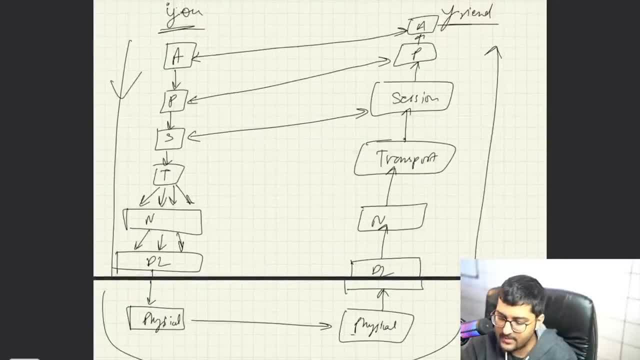 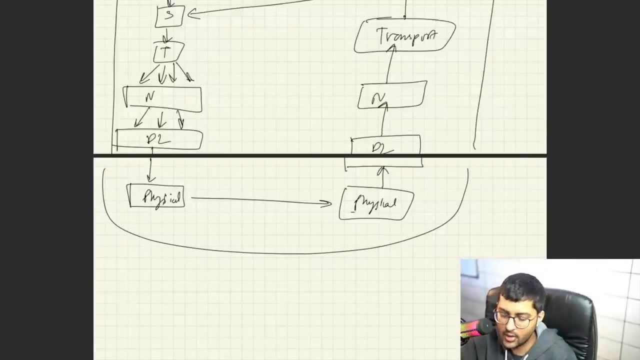 it's like a conceptual way okay so first it starts from application layer and the data is prepped and everything and then it's transferred to the physical layer now this physical router will try to find the physical router of your friend using all the routing techniques and everything 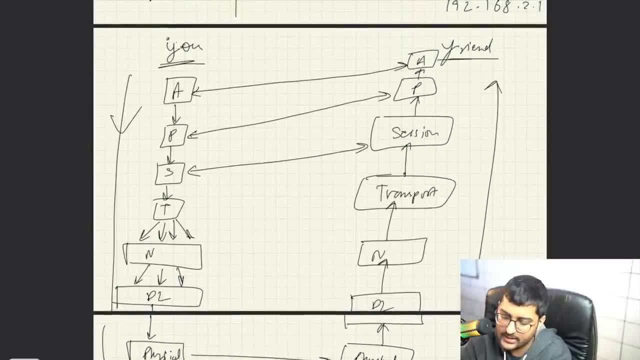 and all these other things and then it is goes back again till the application layer that's as simple as it is how it works 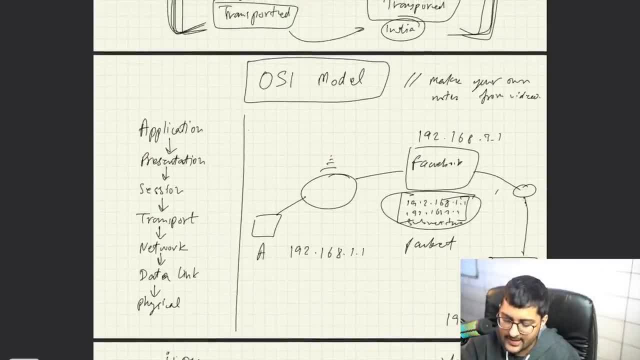 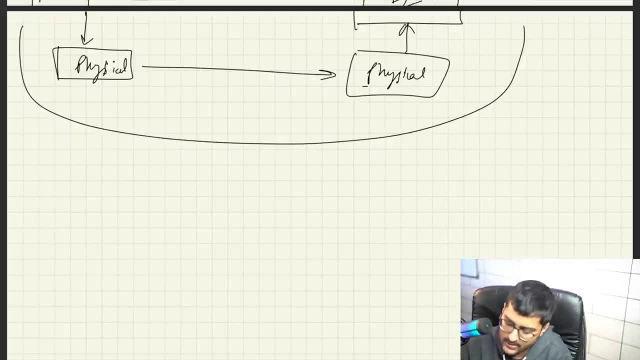 okay that is the osi model i talked in detail about every single layer and uh that's it okay so that was the osi model there's one more model another model 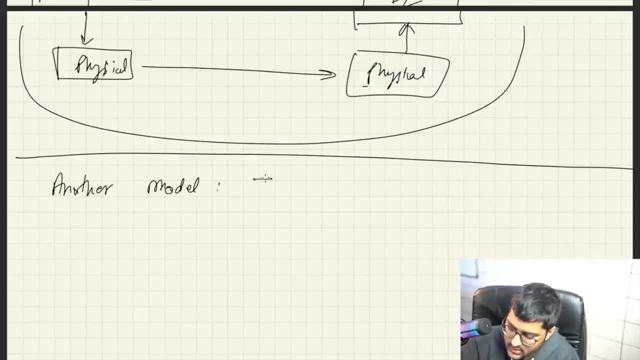 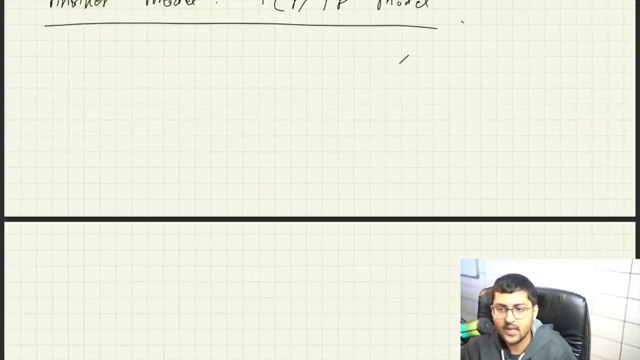 another model this is known as the tcp ip model look now what is the difference between tcp ip model and osi model okay it's mostly similar it's just a little bit of a difference in like the layers and stuff so it is 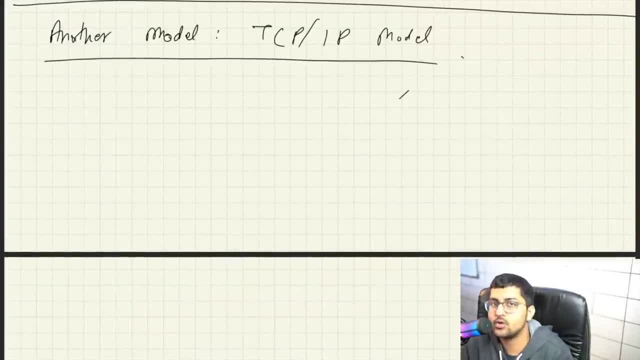 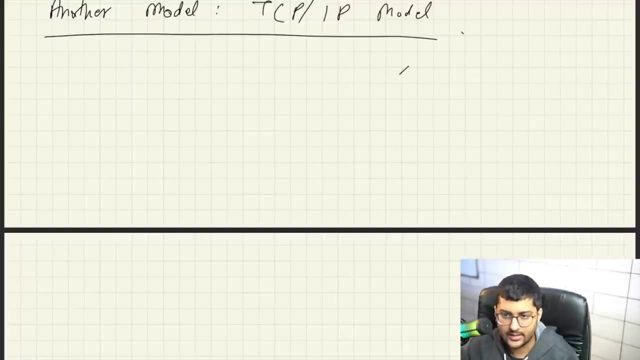 basically known as the internet protocol suit okay and it was developed by the the American like the ARPA thing that I have mentioned previously okay the idea is that it's sort of like similar to like OSI model but the layers are 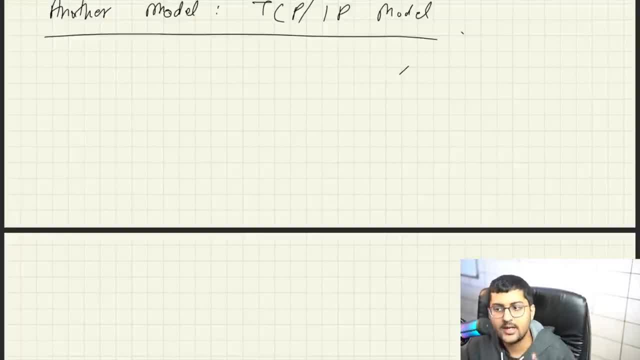 reduced not from not like they're not seven layers it's like having five layers only now okay so the layers are application layer transport layer network layer data link layer and physical layer okay so you can see that the OSI models application 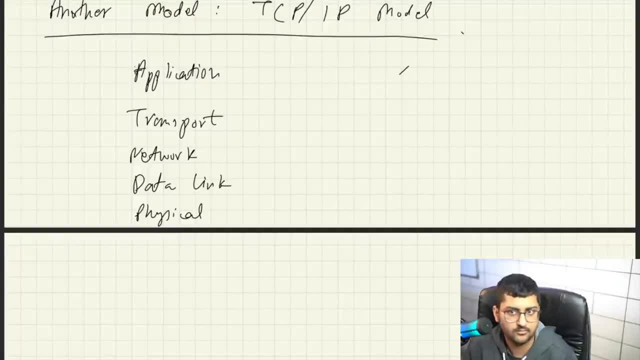 presentation and session layer in this are merged into one okay so this is more 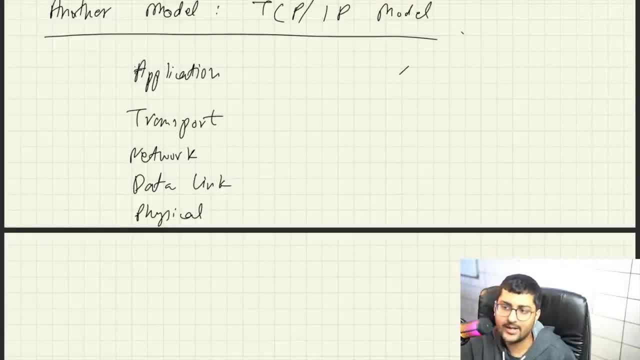 like used practically and the OSI model is more like concept based okay 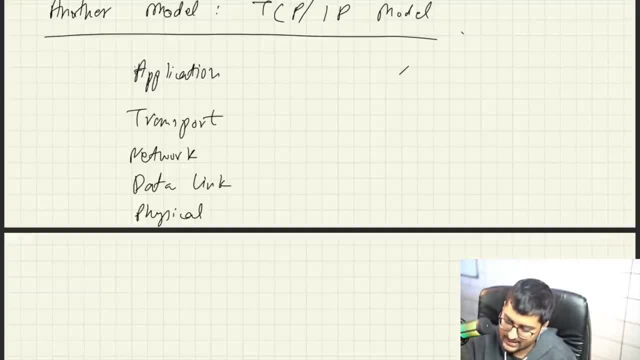 theory okay and that is it let's see now basically now we're going to do a deep dive into these layers okay so we in detail see how these things work 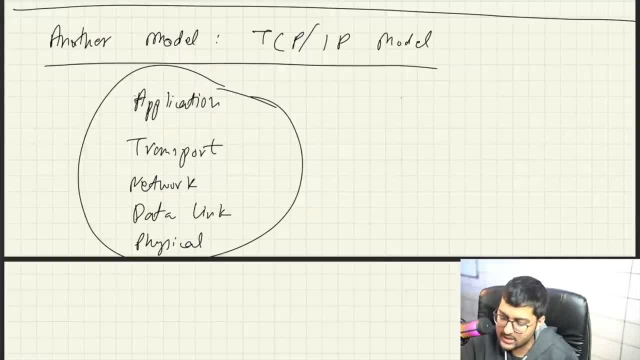 internally and like a little bit more you know hands-on approach and see how things work internally okay let's start with the very first one 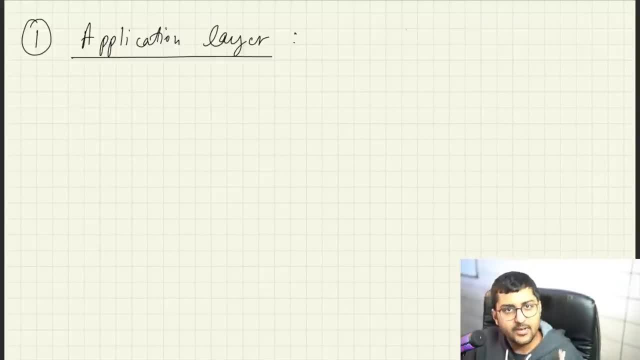 let's talk about application layer okay what is application layer we already covered okay but now it's time to get into the details of it so what is the risk what are like the responsibilities of this layer what do we do in this layer and like why why does this layer exist so simple it's like the main like layer where users interact with right these are the layers where users interact with it it consists of applications right it can discuss consists 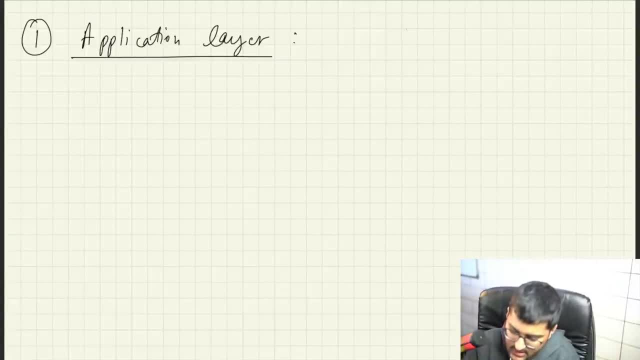 of various applications like your web browser so basically this users interact with this okay we all know whether we all it's very simple this is very simple users interact with this okay so for example if you're talking about you know whatsapp where does what supply application there whatsapp your 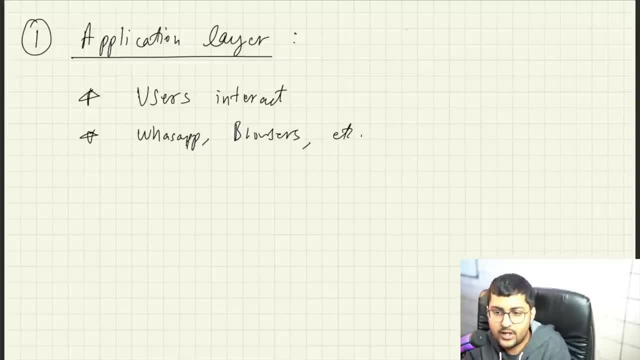 browsers etc okay so you write your message you send your data and everything it's available in the application layer 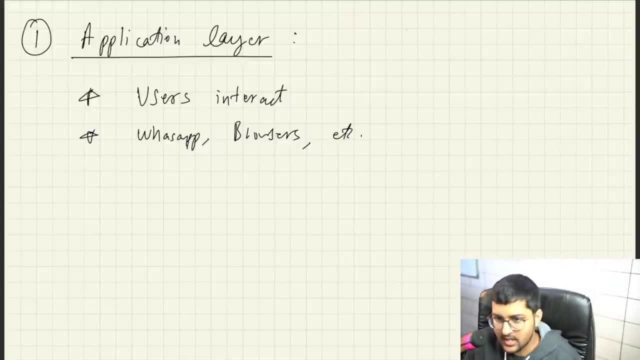 like application layer is the one that you use to interact with it okay so they are where is the application it's on like your devices okay where does it lie 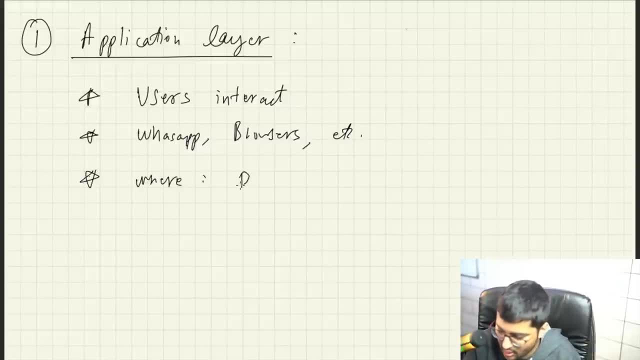 on your devices where on your devices okay so application layer has like imagine this okay how data is transferred how data is communicated 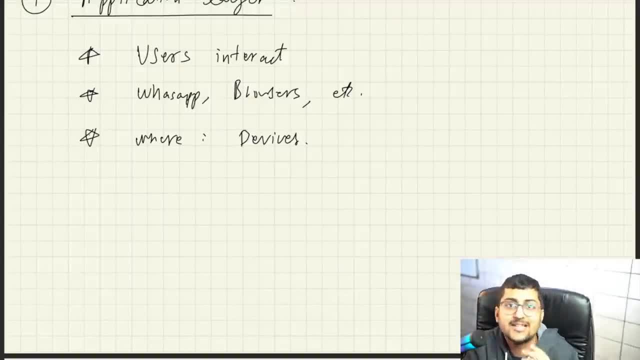 what type of data is transferred using which types of like steps and rules and regulations this is dependent on 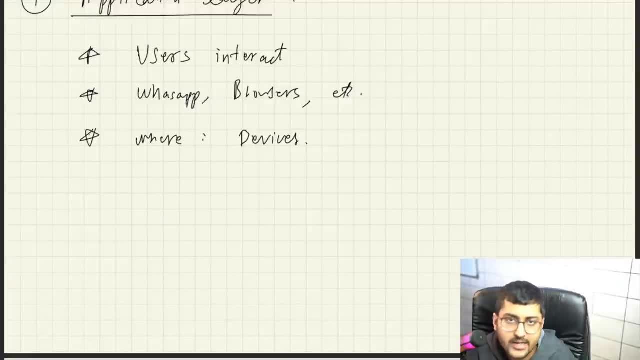 protocols we already covered this there are many protocols like HTTP like file transfer email protocol like UDP for videos and tcp or whatever right so application layer has some protocols okay let's let's will also learn about 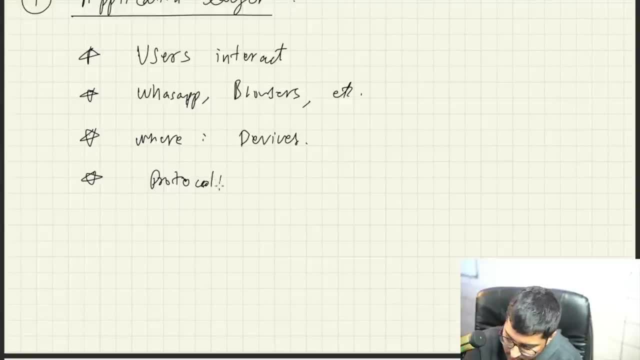 like protocols here protocols and we'll also learn about the client server in front server architecture also in this check architecture know that it's a architecture okay because the idea is that whenever you see the request to some particular server they should be knowing like how to deal with that request okay if you want to talk to 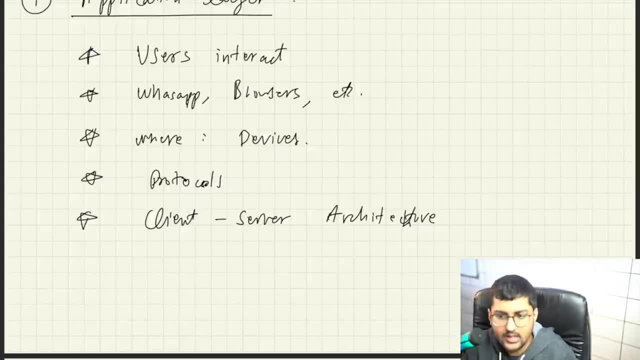 your particular server if the client wants to talk to the server the server should know what type of you know request i am getting what do i have to reply so there should be a set of rules regulate rules and regulations this is what is known as protocols let's look into it a little 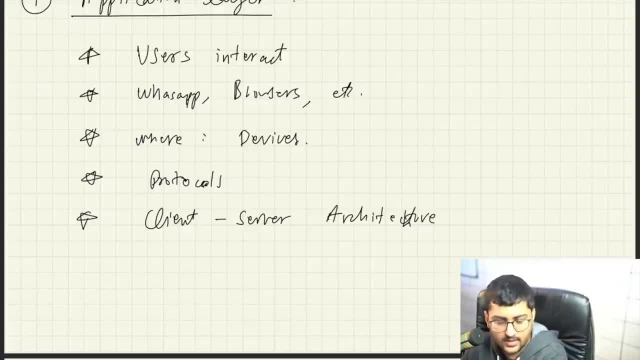 bit more detail okay so we already cover about this like in in brief we talked about there's like a client and then there's like a you know a server and something like that so you have a client 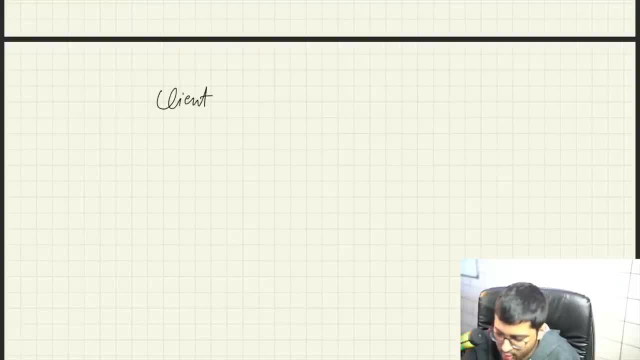 like this okay so let's see how applications like talk to each other okay um and how applications are like in the in the networking system where applications lie and how does it work so you have 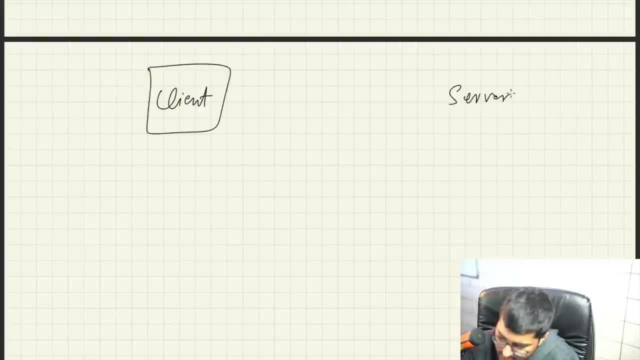 your client over here you have your server over here we already made this diagram previously client sends a request 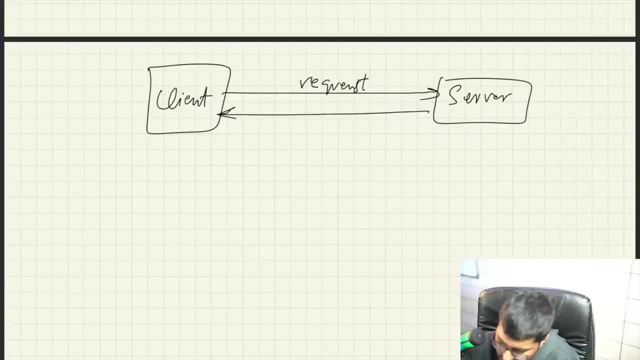 so the server sends a response back we saw this in action also in the firefox browser what is a server 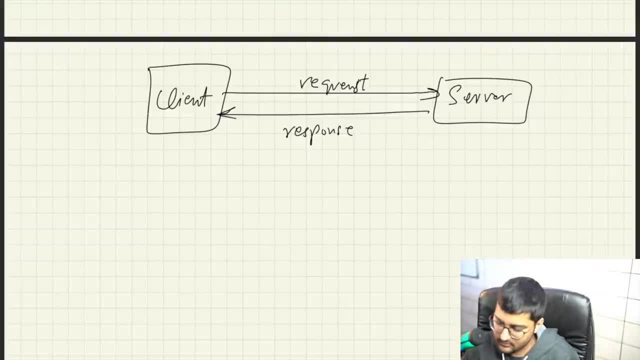 server is basically a system that uh let's say you know um controls your the website you're hosting for example okay so basically this is the client server architecture so here basically the application that we're talking about has two parts client part and a server side part 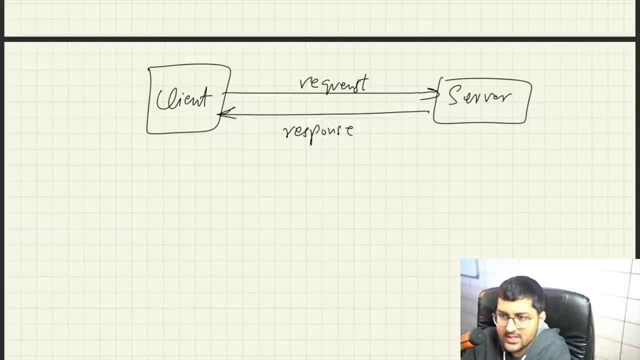 okay and these are known as processes and they communicate through each other 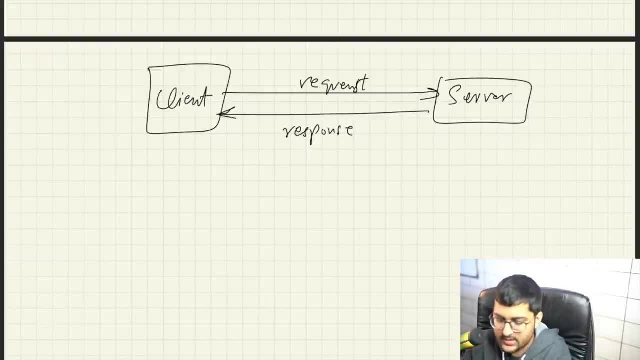 okay cool so process will be running on this application and then another process will be running on like the client and another process will be running on server these will be communicating with each other okay so if you want to host your own server okay then uh obviously like uh 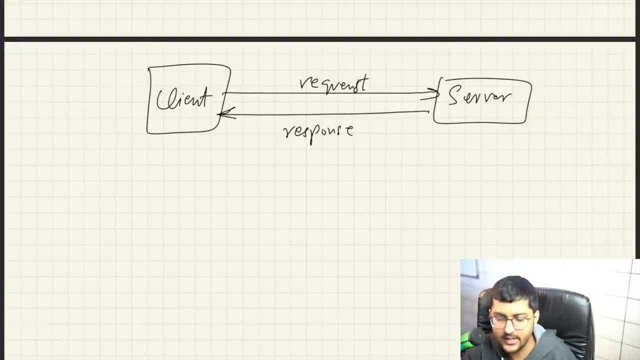 you should have like some reliable ip address right uh which can be reached via clients okay and um you should be also having uh like um you know high availability yours you don't want your servers to be down client on the other hand is uh you know folks who are using and who are consuming these resources us we are like we are making a request to google you are a client okay so that's basically about it so when you make 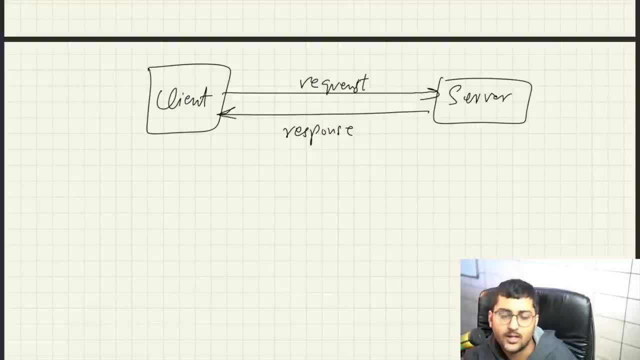 a request to like youtube.com okay hey like hey youtube uh show me show me some videos or whatever so you are the client and the youtube server is like the server and it sends you the data back so when i'm talking about servers of youtube or facebook or microsoft or cevo for example so we have a lot of servers we don't have just one server we have a lot of servers 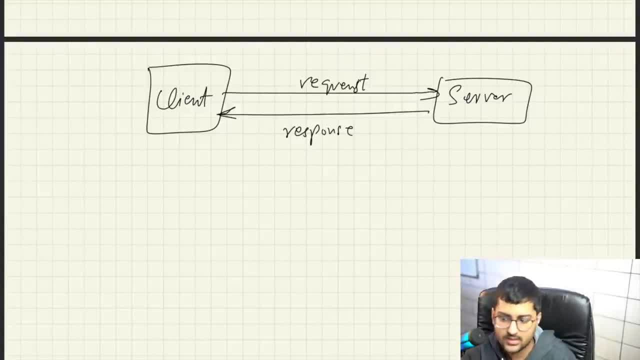 there are there are like a lot of servers because this is like such a big company right so many folks are using if all the folks are contacting just one single server the silver will go down happens many times when a result are announced so many students are trying to make request to 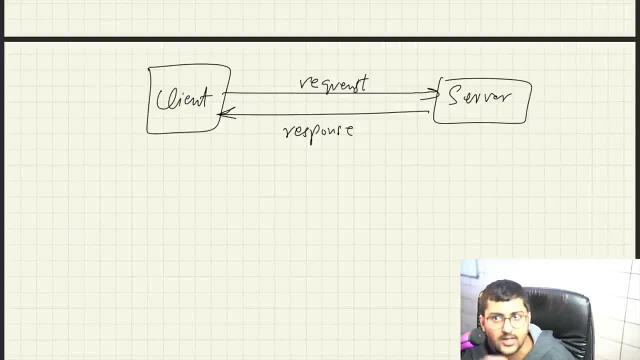 the server and the servers are not really fast or like not really enough websites crash same thing happened like you know uh so many like uh people try to buy ps5 websites crash game 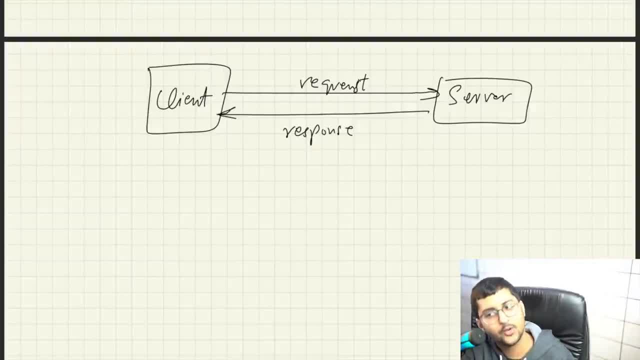 the shop was not working at vs5 pre-order launch okay so these are known as these servers the collection of servers in a big company it's known as a data center okay it's like at a really big 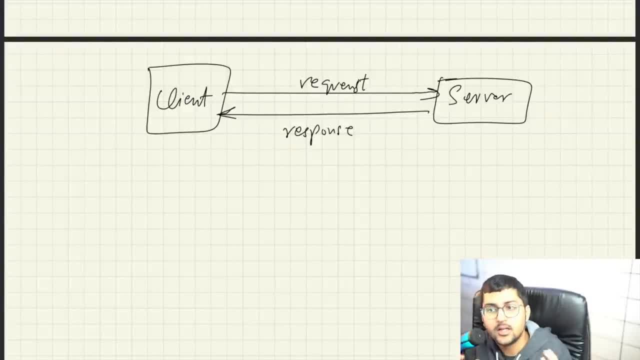 scale okay so when we talk about data centers we talk about like it's a collection of huge number of computers okay it may have like static ip addresses addresses that do not change they have like very good you know internet connection that does not go down and high upload speed 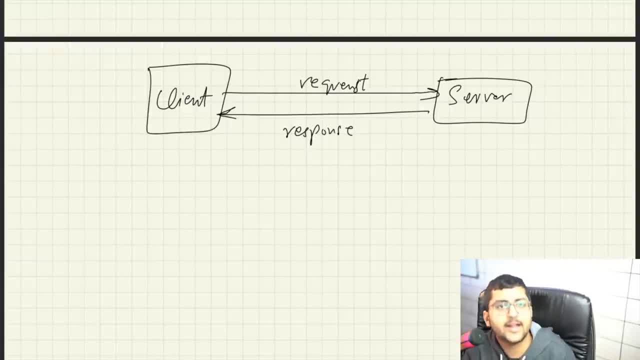 because you know uh there are also companies that are like renting their servers like cloud providers which we'll talk more about later in the future of the devops bootcamp okay you can 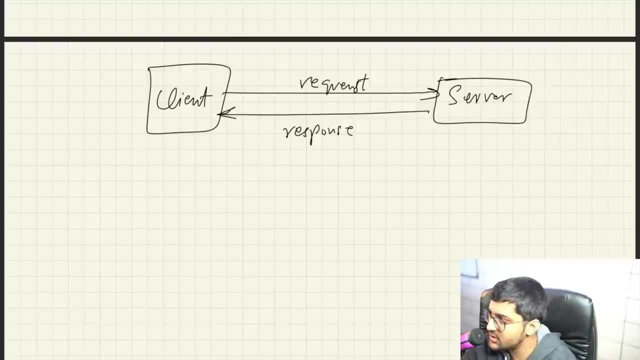 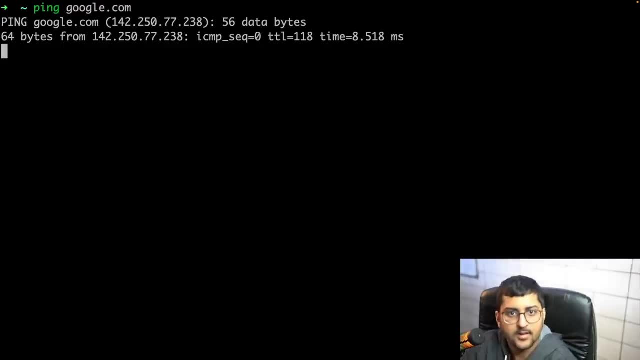 actually do this thing that you're seeing on the screen right making a request to the server even though you type google.com but if you're in your terminal you just write ping google.com or something so i can see it's taking it in chunks the packets that i talked about these are the sequences 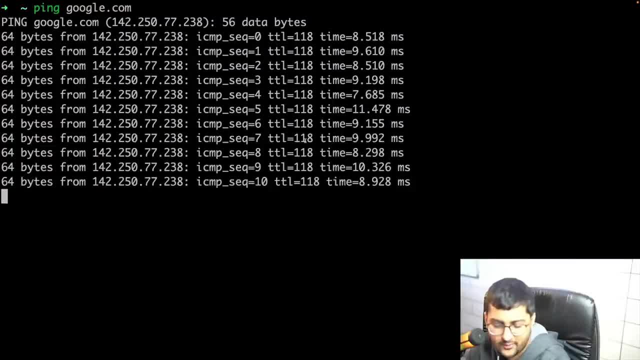 these are the time to live so something we'll cover later on 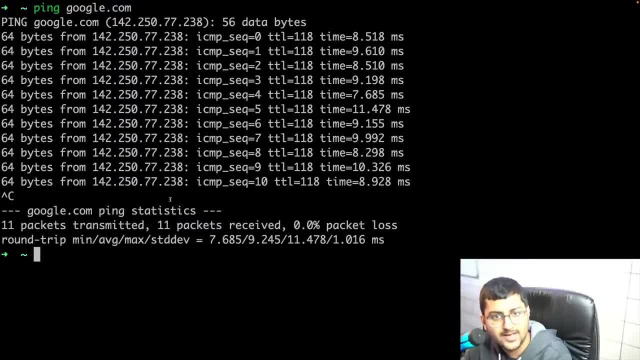 okay no packet was lost 11 packets were you see i told you about packets right these are those packets every packet is a size of 64 bytes these are the ip addresses of like google server this may be different for you because google does not have just one server they have many servers okay and there's something like the sequence so in order to make sure that data packets are in order to make sure that data packets are in order to make sure that data packets are 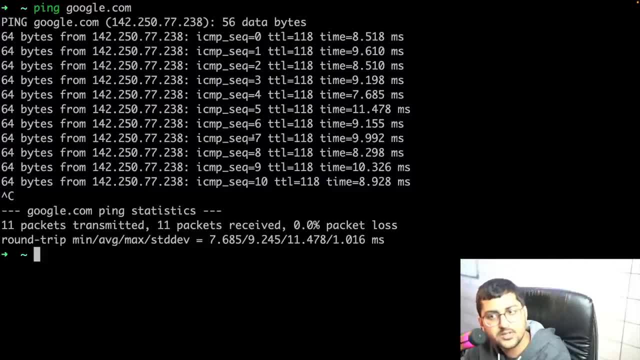 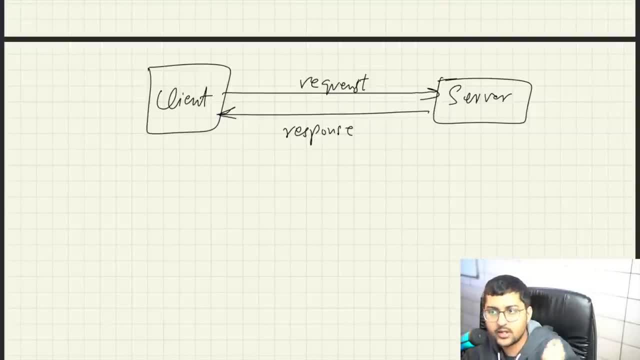 received in sequences there's a sequence number i mentioned previously time to live is something i'll let you know later on how how this thing actually works okay so that ping that basically you saw that was uh it measures the round trip time for messages sent from the originating host 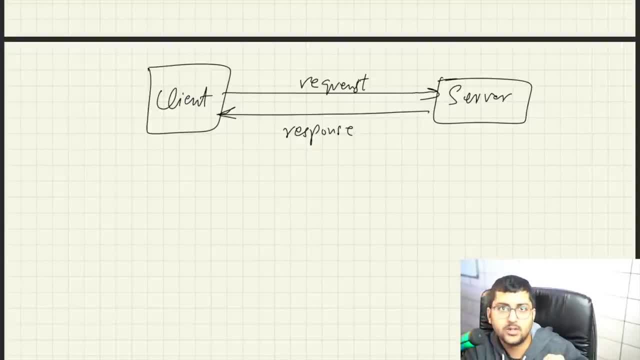 to the destination of the computer and that are echoed back this entire time is known as ping ping time okay so questions i asked i got asked once like can we reduce this ping time not really because you're getting the best possible ping time signals are traveling at 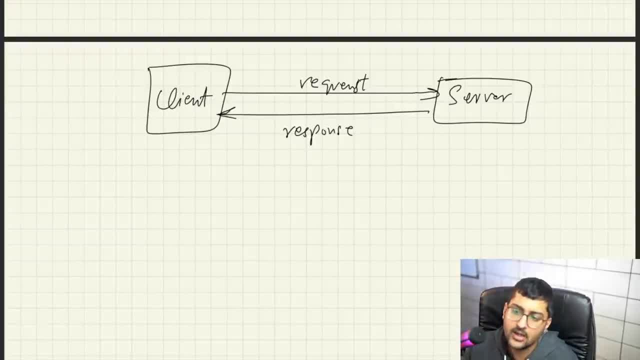 the speed of light through like cables and satellites etc so you're getting the best possible time cool all right so this was about the client server's architecture there's one more way in which uh applications are connected from end systems this is known as peer-to-peer architecture or p2p okay so first is client server second is p2p peer-to-peer 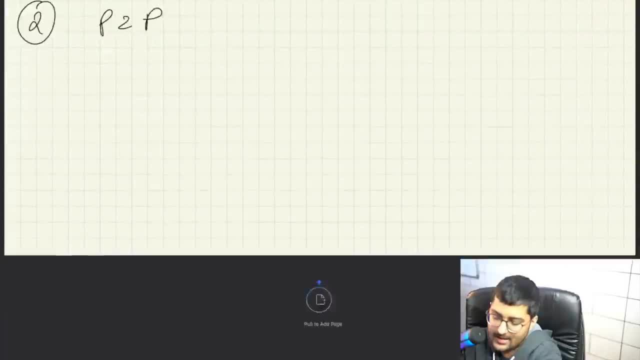 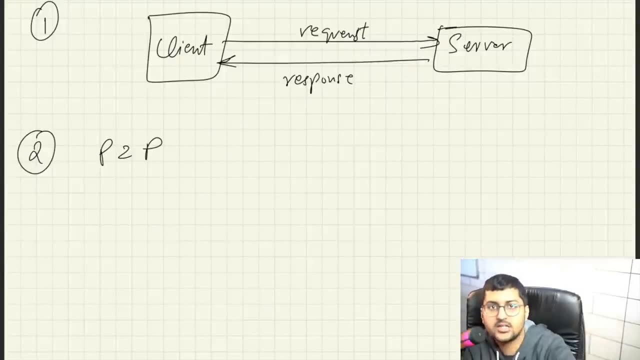 in this what happens is various devices uh applications that are running on various devices they get communicated they get connected with each other so there's no one server or a large data center or whatever okay so example in your college there may be many computers the computers will be connected to one another something like this 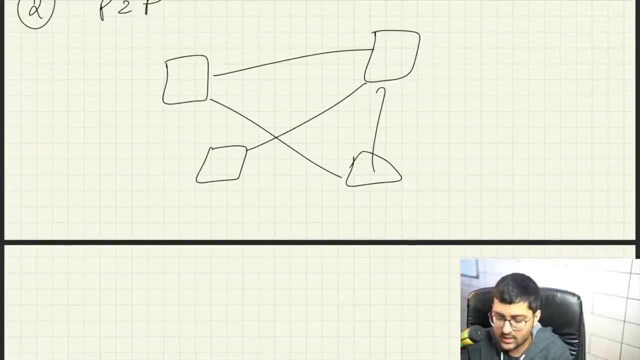 something like that this is peer-to-peer communication there is no one dedicated server 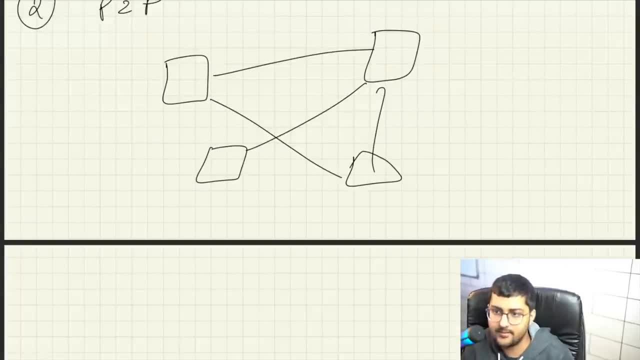 uh there's like a lot lot more the key advantage over here is that um you know you can scale it very rapidly okay and it's it's like a little bit like a decentralized network as well okay so here what is happening is what is client and what is server over here in this since this is also serving as a client and a server every single computer can be termed as a client as well and a server as well a good example for this can be bit torrent right 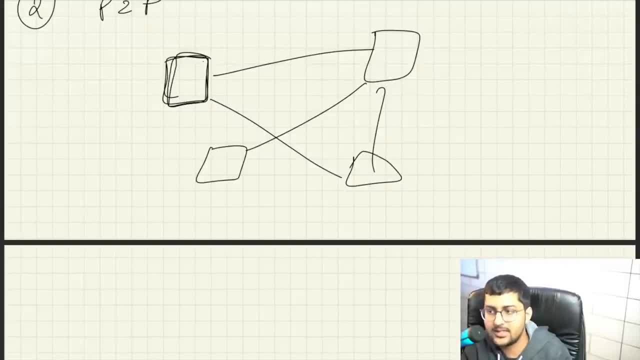 you may have heard about like uh you know in bit torrent there's like seeding and stuff so how torrent works we'll cover more about that later on like how torrent works okay but torrent is a 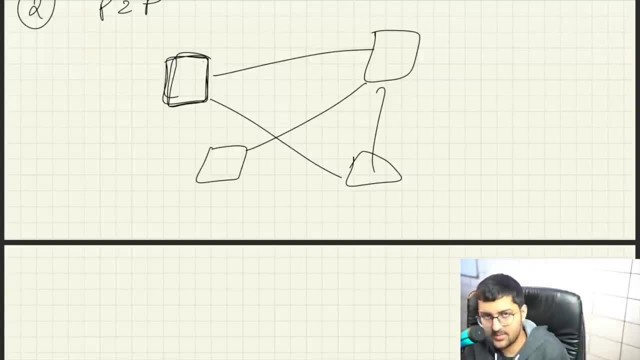 good example of this okay hybrid also exists from our peer-to-peer and also having some sort of a centralized database that is also possible cool so that was basically about peer-to-peer all right 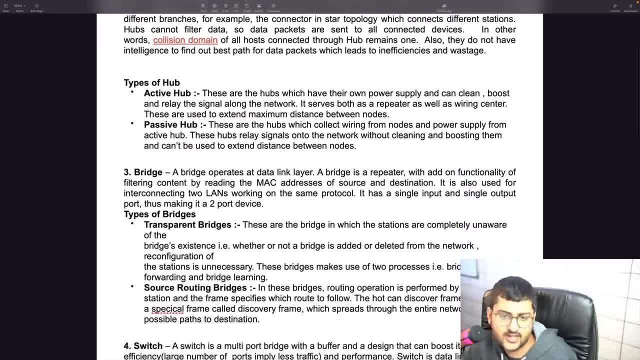 now before we move forward i just want to give you a quick overview of all these networking like 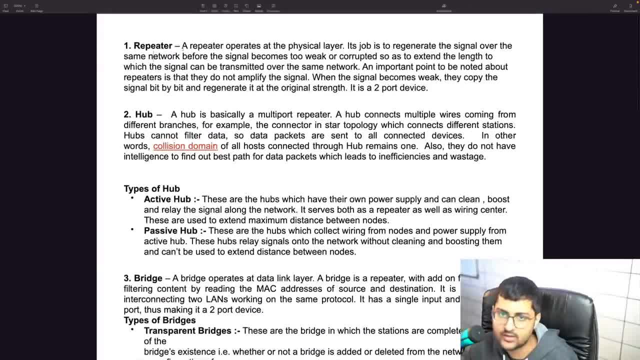 use it's a pretty straightforward you can find the definitions like online i also have like a nice little pdf open over here the first one is like repeater so a repeater basically is at the physical layer we already know what the physical layer is now and the its job is to regenerate the signal over the same network because the signal before the signal becomes too weak or corrupted okay so it can be transmitted over the same network okay um and an important point to note over here is that it does not amplify the signal so when the signal becomes weak they copy the signal bit by bit and it reach regenerate it to its original strength okay it's a two port device okay so there are like two ports available um hub basically is a multi-port repeater okay instead of just two port it has multiple ports and it connects multiple wires coming from different branches for example the connector in like the star topology that we mentioned okay so it cannot like filter the data uh so the data packets will be sent to like all connected devices um in in other words it says that the collision domain of all hosts connected to hub remains one okay and also they do not have the intelligence to find out which are the best path for the data packets so hub is like a repeater only okay and the job is the result is to regenerate the signal over the same network because it before it becomes too 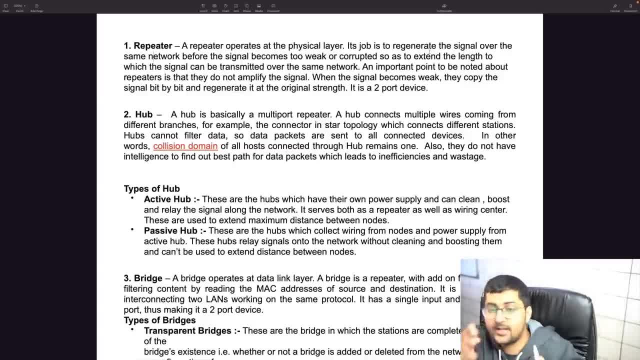 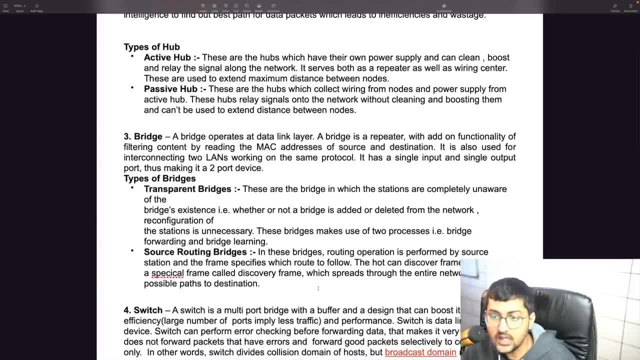 weak it will regenerate the network okay it will not amplify it or whatever but in hub it's basically a multi-port repeater okay you can learn about the types of hub or whatever bridge 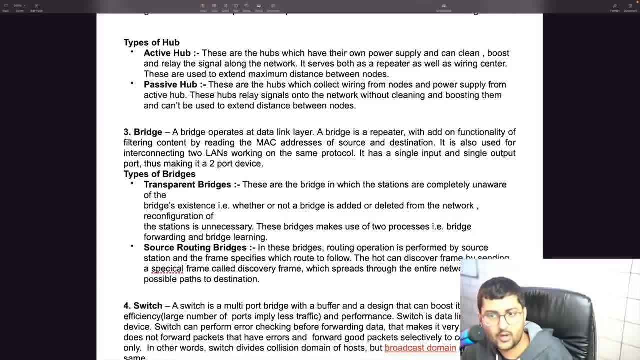 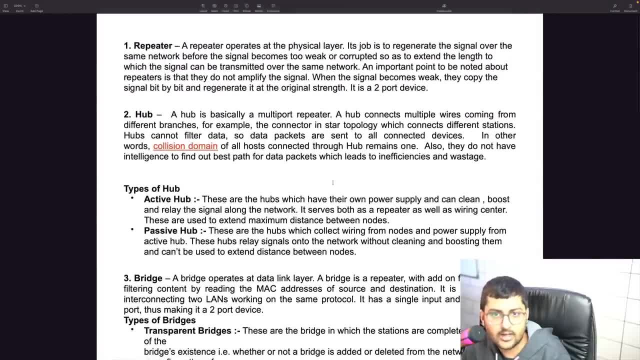 operates at the data link layer we talked about the data link layer in detail we talked about mac addresses right at the data link layer we'll obviously cover data link layer in detail but a bridge is type of a repeater we have we covered yeah repeater is over here and it has an 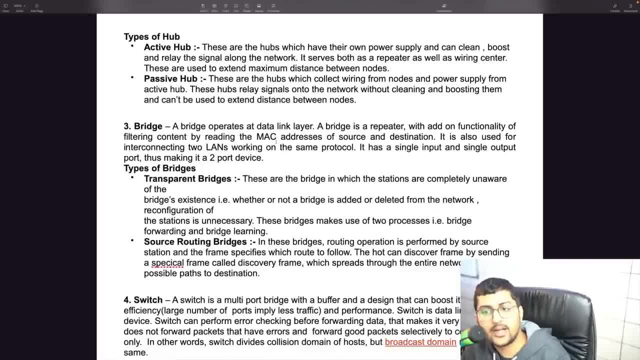 additional functionality that it can filter out content by reading the mac addresses of the source and destination we know that at the data link layer the target and packets what we have that contain the mac addresses of what sender and receiver okay so it's able to filter that out 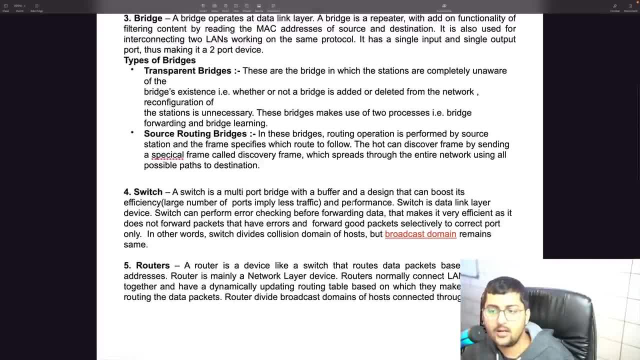 switch is a multi-port bridge okay with a that can basically boost the performance and efficiency okay so it is also at data link 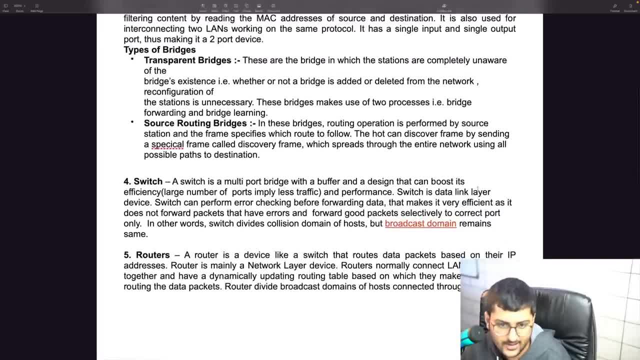 layer because it's a bridge so bridges are a data link layer so it is also at a data link layer and it can perform like error checking and before forwarding the data so it makes it very efficient 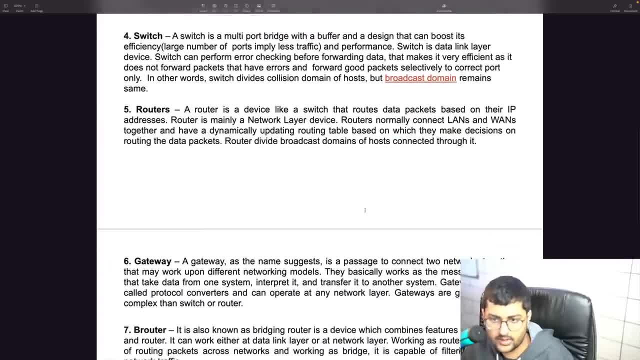 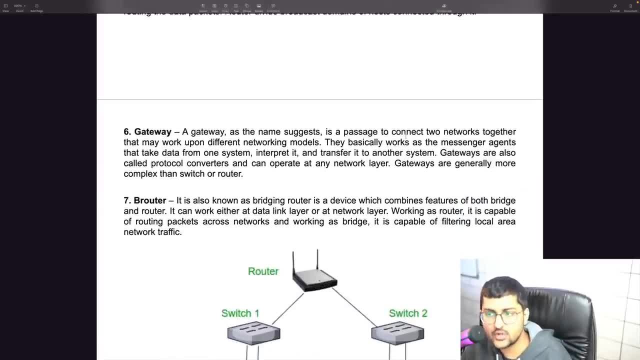 right cool router we already covered what are routers at network layer we already covered it no problem gateway gateway is as the name suggests a pass a passage to connect two networks together 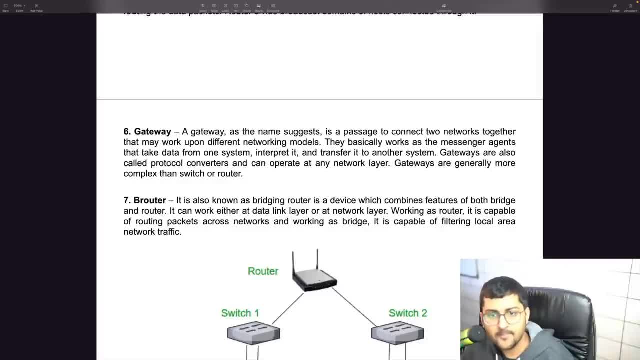 and it can work upon different networking models okay so for example uh here it's saying that uh 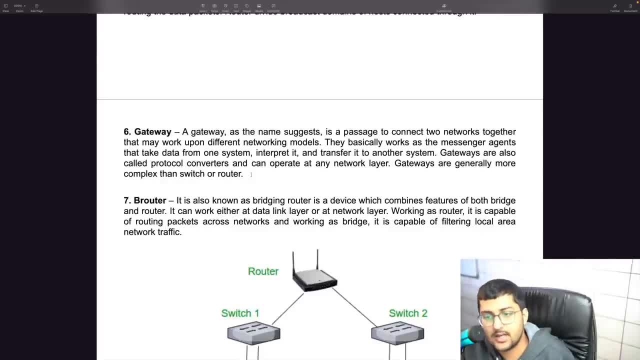 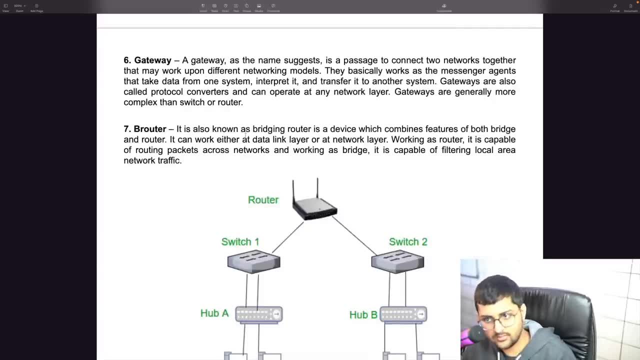 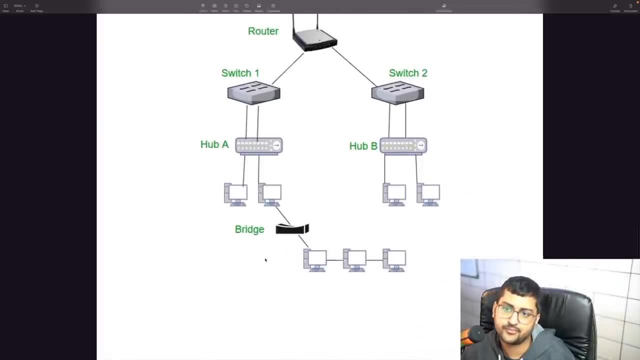 it's sort of like one network we may be working on some different protocol another network may be working on different protocol it can basically connect that okay router is basically a bridge and a router combined you can say right and it offers the functionality of both bridge and router and this is like a nice little diagram for you okay so it's very simple nothing nothing you know major in 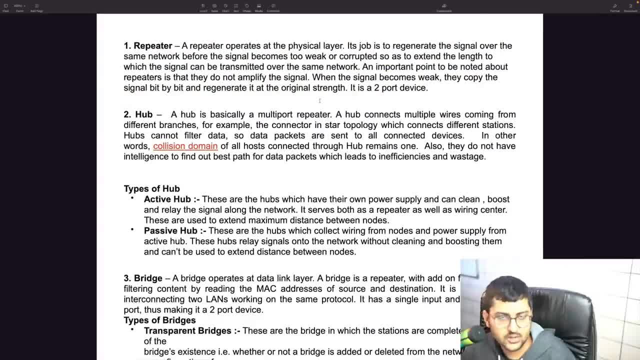 this so i just wanted to mention like the um basic use cases of these things as well you can take a screenshot of this if you want and uh yeah 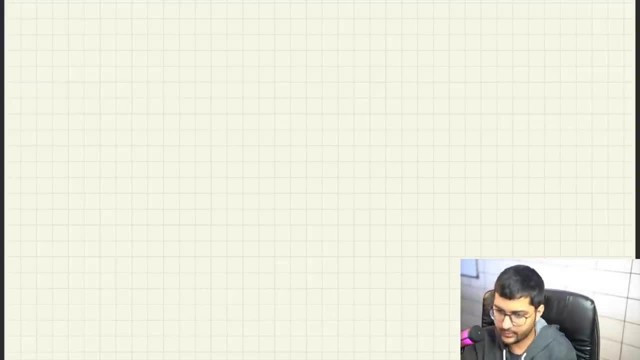 cool okay now uh one more thing that i promised i will go into details was uh protocols so we all know what protocols are network protocols let's talk about protocols 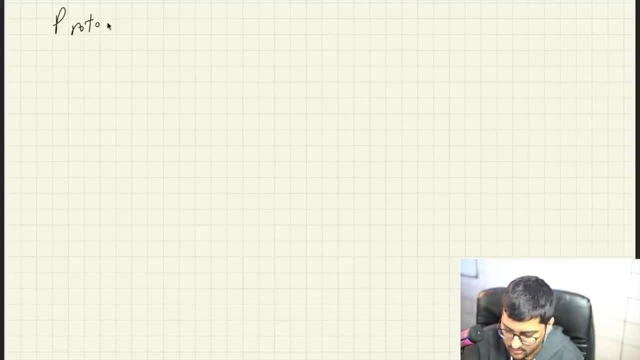 by the way we're on application layer only right now okay protocols so every application will have some sort of a protocol if you're working with web web web or something just browsing the internet you will be following like tcp ip protocol http for example 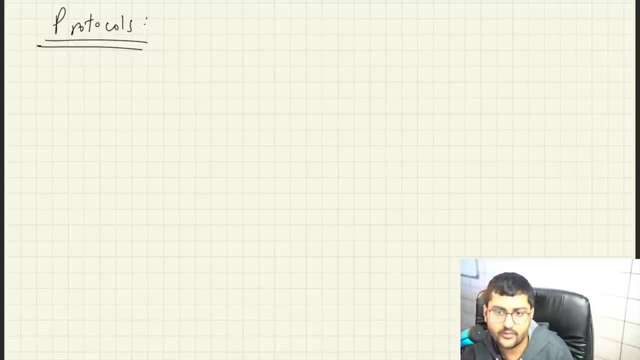 right if you're sending someone a file then there's file transfer protocol if you're sending an email then there's simple mail transfer protocol so on and so forth okay so what are some of the protocols let's divide it into like categories i have already explained what protocols are so i won't like go into you know details details of it um we talked about packets and protocols are what protocols are and stuff let's talk about like web protocols when we talk about protocols protocols okay how it works and everything 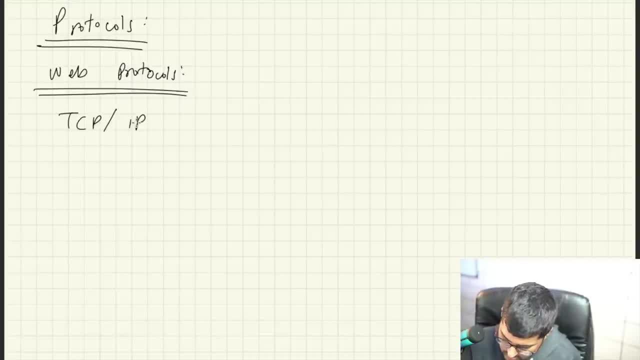 okay let's talk about tcp ip protocols for example okay so here you can have like uh http okay hypertech transfer protocol so it defines how uh you know the the html page like how data is transferred for example html pages and things like that i also mentioned briefly about dhcp 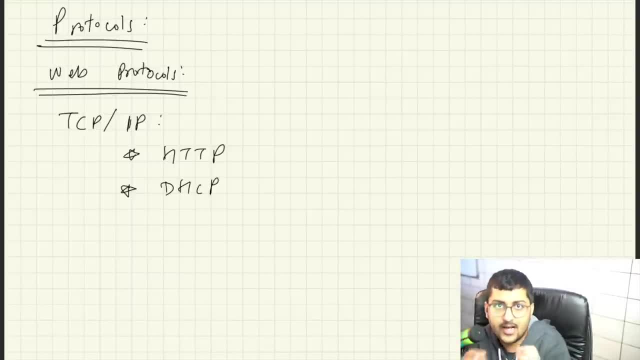 uh dynamic host control protocol it basically allocates the ip addresses to your device people and devices that are connected to your network so if you have a network uh if you have a network uh 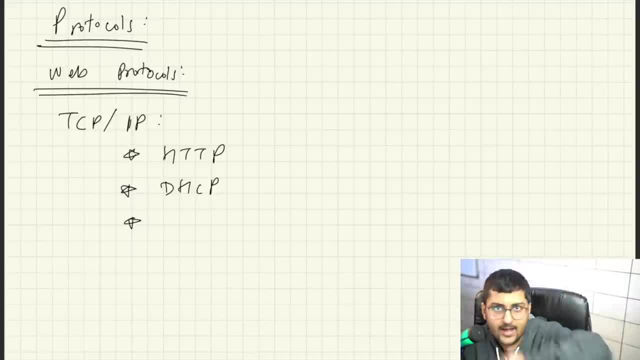 network right and i gave you a little nice diagram of that as well everything was covered 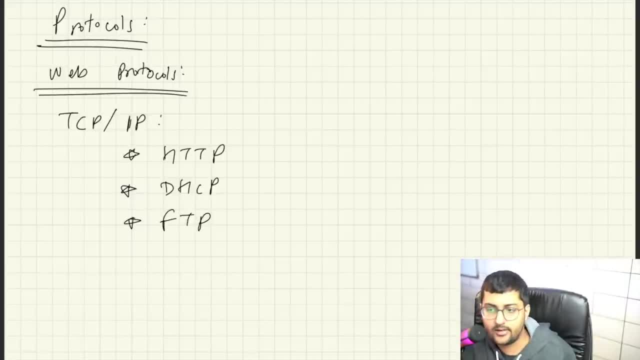 file transfer protocol okay how the files are how the files can be transferred but i don't think this is being used anymore because files can now be transferred over http right um there's one more called simple mail transfer protocol this we'll see in detail how in how emails work okay if you 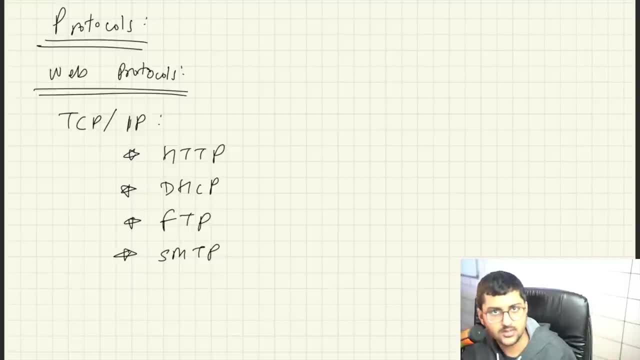 want to send an email on a receive an email how how it works using the simple mail transfer protocol okay it's used to send the emails to receive the emails you have pop3 shout out dan pop uh check out 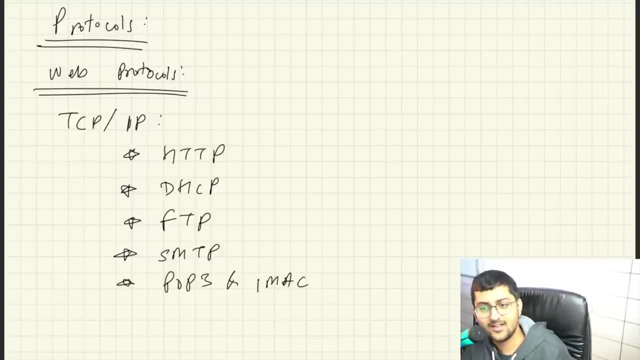 popcast pop and uh yeah and imac okay so these are used to receive emails what else what else 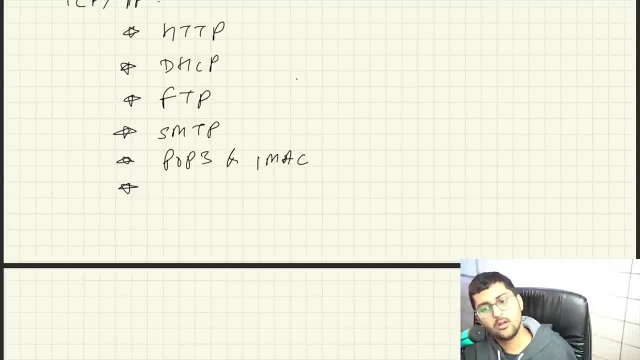 protocols are theirs um ssh secure shell okay so if you want to log into a terminal of 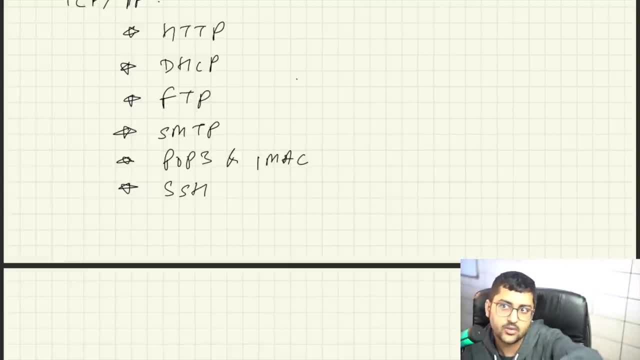 um um someone else's computer for example you can use ssh for that so we'll be using this heavily uh i'll 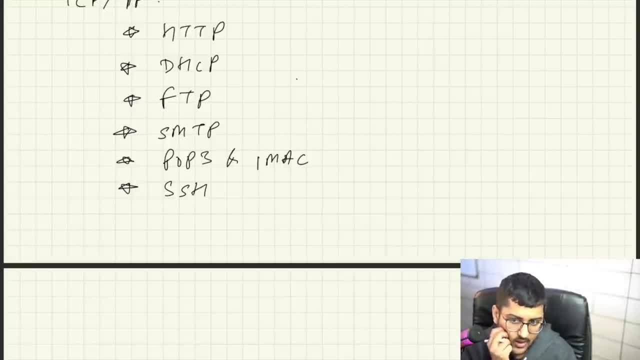 be using the ceo cloud instances and i will be using that um in order to you know um log into your computer and things like that okay um all right so that's ssh and there's one more called 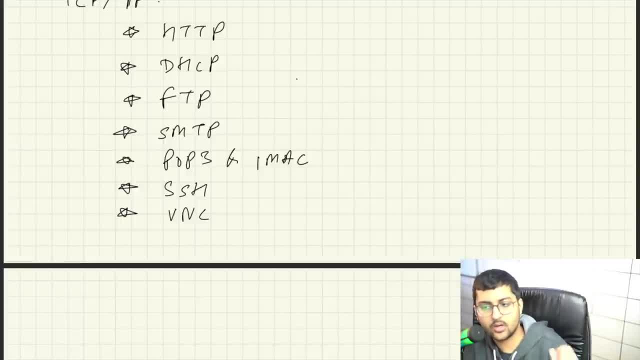 i believe there's so many so you can google it virtual network computing it's for graphical control okay that's it there's one more called telnet 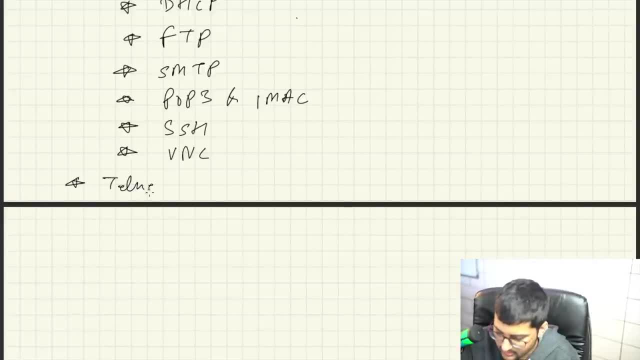 okay outside of like tcp ip there's one called telnet so telnet is basically a terminal uh emulation that enables a user to connect to a remote host or a device using the telnet client okay usually it's over port 23 or 23 let me write the port over here as well okay so for example uh typing 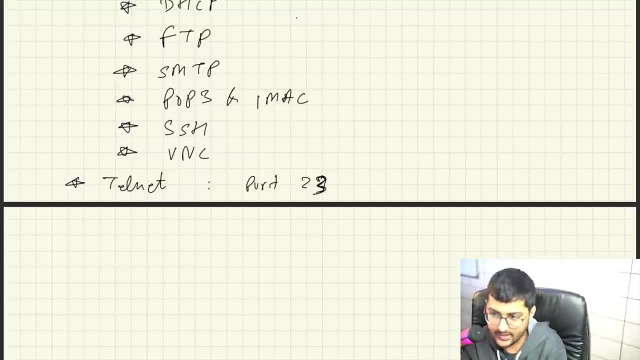 like telnet host name would connect you uh would connect like a user to a host name that is called like host name okay so if i say telnet kunal like it will connect me to a host name called kunal so it enables users to manage an account or a device remotely okay it's a very low level protocol okay all right um cool 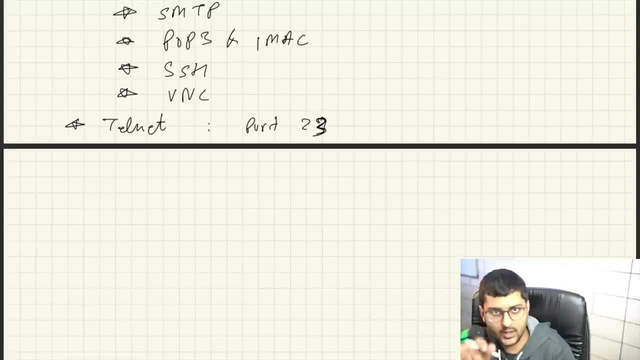 one more thing in like http and https and stuff s means secure so i'll talk more about that later 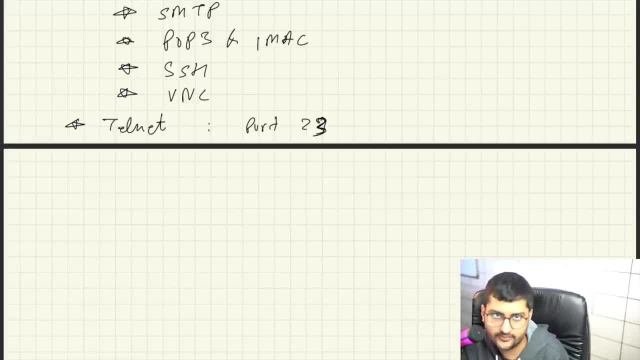 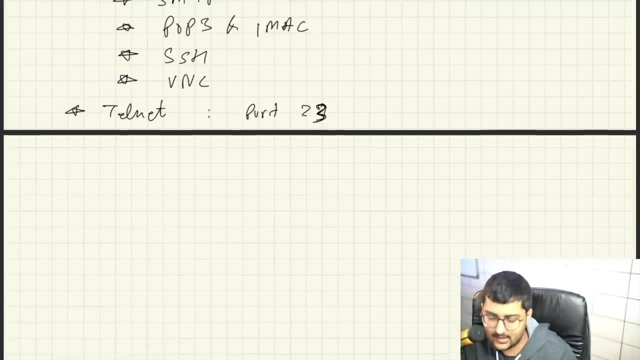 now we get data that is like encoded for example like utf-8 and stuff okay these are standards of encoding in terms of encoding we get data that is like encoded for example like utf-8 and stuff okay intel net it is like not encoded or encrypted okay so all these things are handled at the 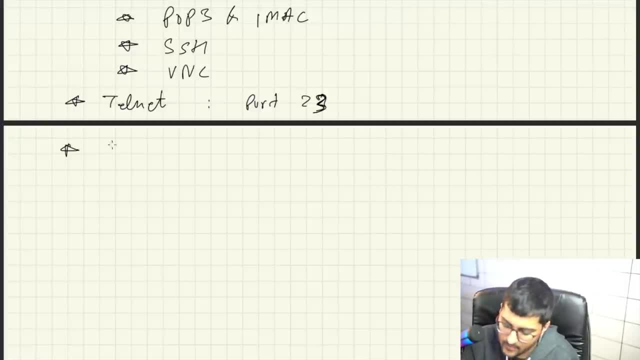 application layers is that what we're talking about right now udp already mentioned a lot of times how it works i'll cover in detail i'm just listing it out right now so it's a 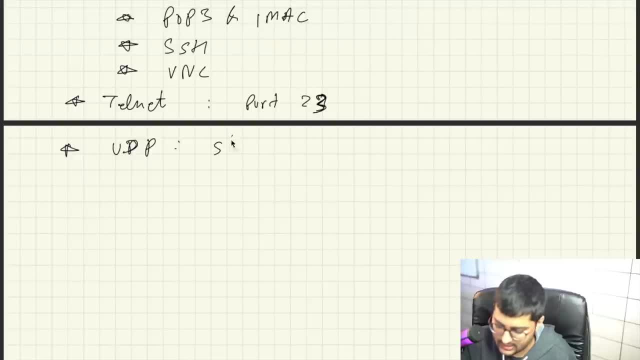 connection-less session um like a stateless collection it does not maintain the state okay data may be lost in this okay during the lifetime of the connection cool uh let's look into the connection-less session okay let's look into the connection okay data may be lost in this okay during the lifetime of the connection 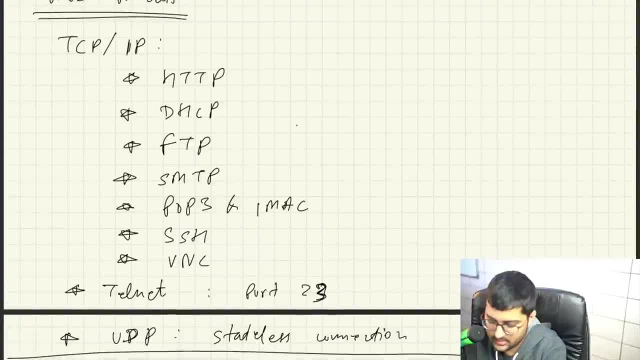 cool uh let's look into the data collection okay data is probably only for right so take a look here uh let's look into like a little bit more detail of like some of these protocols okay so now we 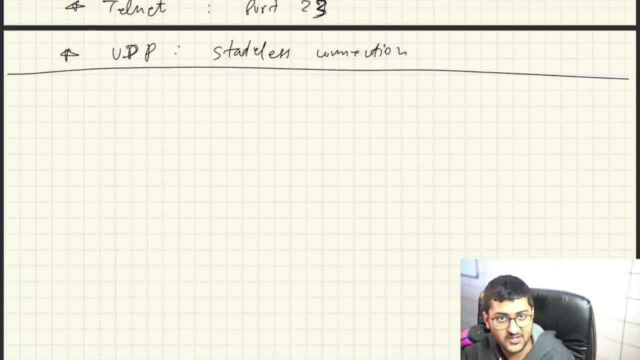 have let's say applications okay and we're still on the application layer so obviously we're talking about applications so one thing we have to cover over here is uh how do these applications 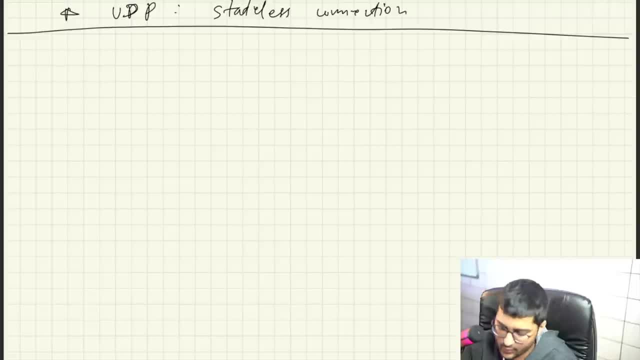 like talk to each other okay so there are like a few terms when we talk about like applications so basically let's talk about uh let's say we talk about um 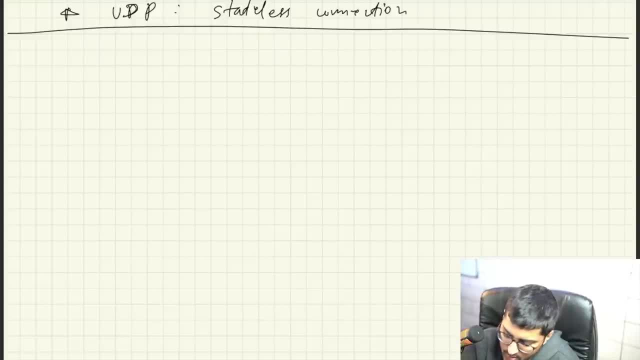 whatsapp okay so when we talk about whatsapp this is known as our program like our application so our program is whatsapp 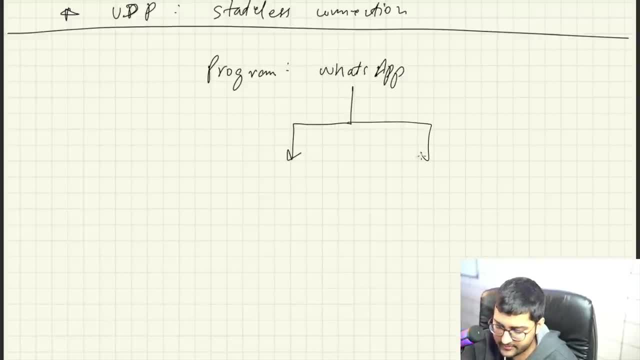 okay now this program whatsapp will have some processes in it okay so for example you are sending a message okay or record a video these are known as processes of my program 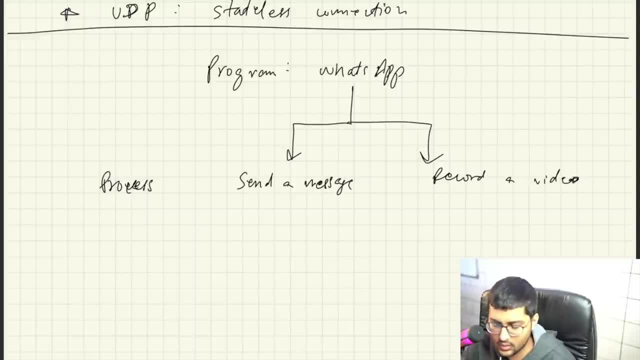 okay so what is a program a program is just like your application okay so for example whatsapp and you know amazon or flipkart or email surveys or whatever okay that's a program an application 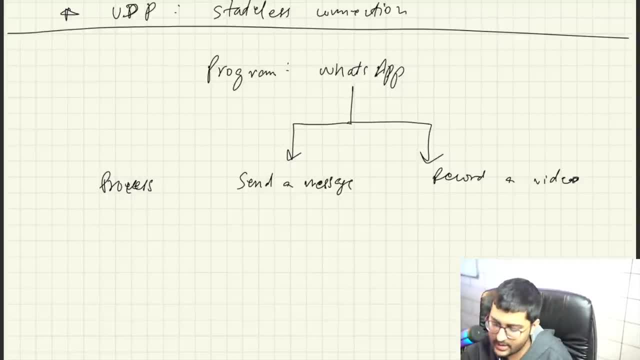 process is what a process is like um you know like one of the features of the program for example right or a running instance of a program okay so one program can have like many many processes running at once 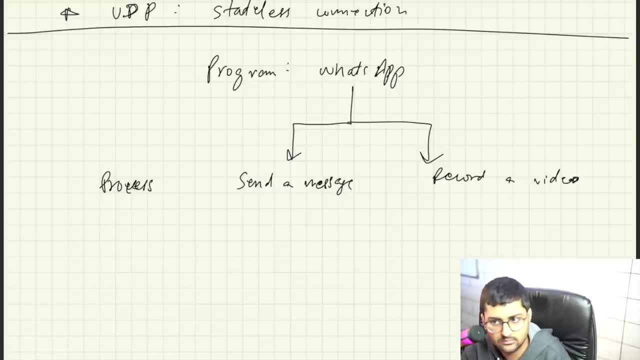 okay recording a video while sending a message for example okay and uh there's one more thing called um a thread you may have heard about thread so thread is a lighter version of a process 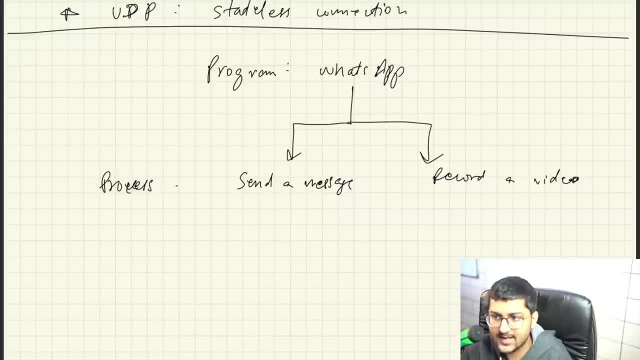 okay so when we talk about like uh one process it can have like multiple running threads okay so what is the difference between like here i can say this has like some thread sending a message 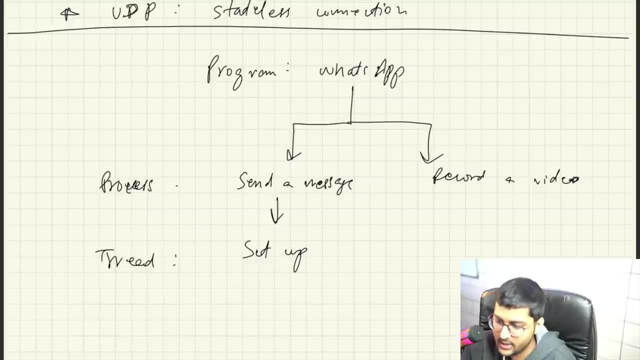 can have like set up um you know the uh page or something recording a video open camera 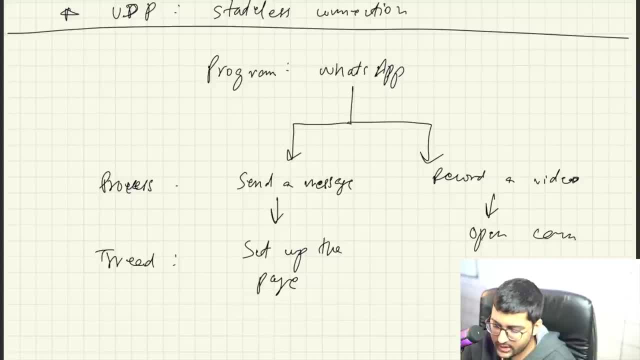 open camera or something so the only difference between a thread and a process is that the thread is only doing one single job okay so you know i have multi-level multi-threading uh you know multi-threaded programs where multiple threads are working simultaneously that's basically what the idea of a thread is okay so what is a thread so a thread is basically what the idea of a thread is 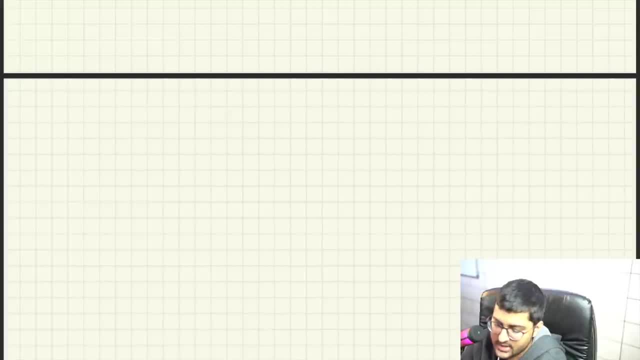 okay now now how do these uh things communicate with each other so we know that you have your application running on your phone and then there are so many billions and billions of phones in the world how does the internet determine you know which message is being sent from you want to send a message from your whatsapp to someone else's whatsapp how would it communicate over the internet okay so here we are talking about addresses so ip addresses and port numbers we already talked about ip addresses we'll talk about port numbers in a in a single single second there's one more thing known as sockets okay so sockets are basically like uh you know um when you need to send messages from one system to like another system okay um we can use sockets for that so it's not like you're continuously like you know it's not like the client server stuff but it's more like um it's a software process it's not like you have some 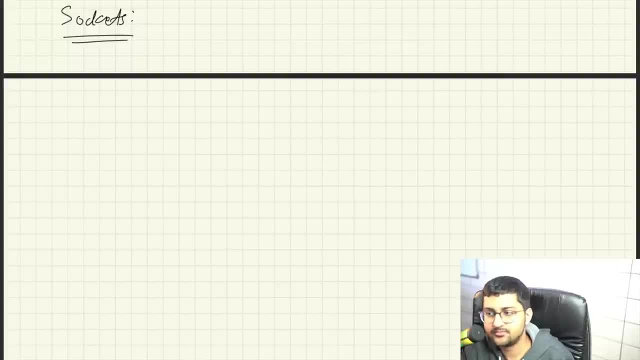 something like like a hardware socket or whatever okay so uh it's basically like uh the interface that is there between like the processes that i mentioned 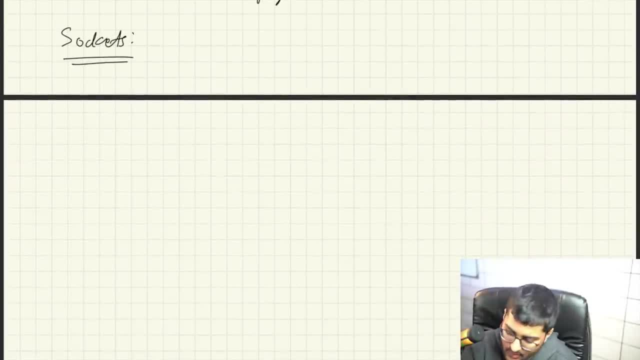 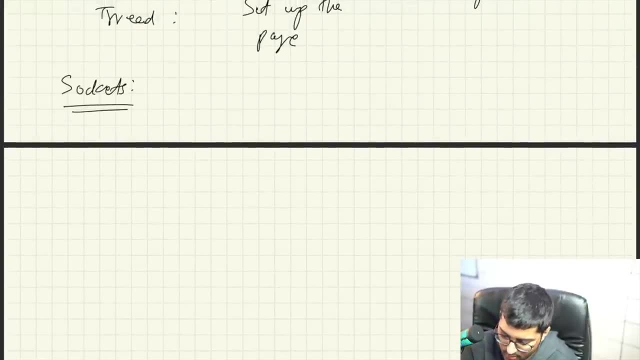 and the internet for example that's known as a socket okay so interface between uh process and the internet okay that's basically what a socket is and let's talk about ports you already know 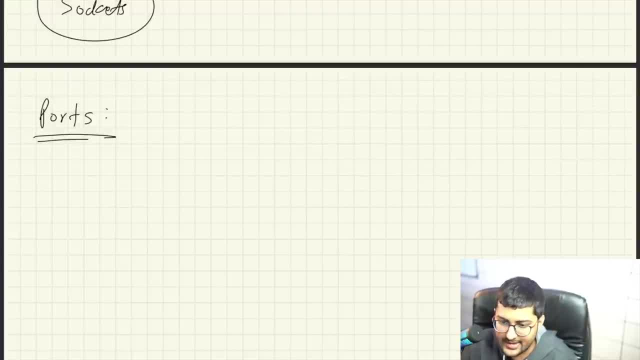 about ip addresses but let's talk about like ports a little bit more in detail so let's see okay let's talk about ports 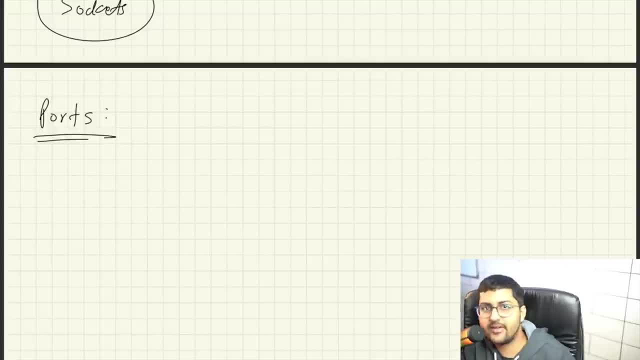 already covered about ports ip addresses tells which device we are working with ports tell us which application we are working with now there may be possibility that many 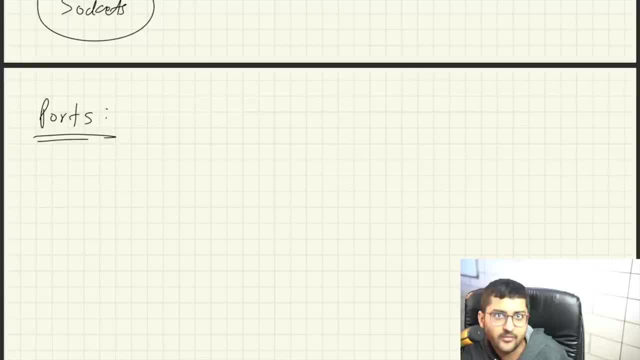 processes are running of one application you have many chrome windows open okay so like kunal i know like this data that you have requested whatever is coming from my friend needs to go to google chrome but which instance of google chrome which process of google chrome 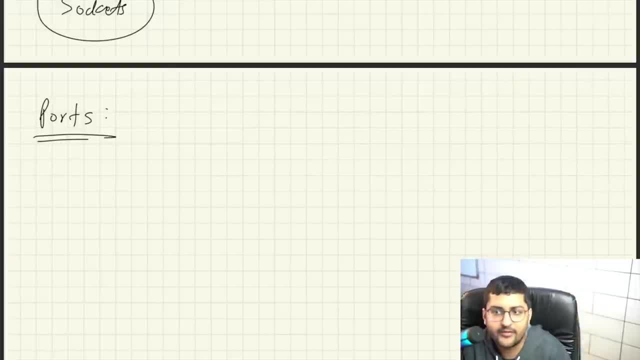 browser number one browser number two like tab number one two three or four or five how do we there's this thing known as e-formal ports for this e e-femal ephemeral ports ephemeral ports so basically the idea is that let's say you have uh you know port 80 reserved for uh 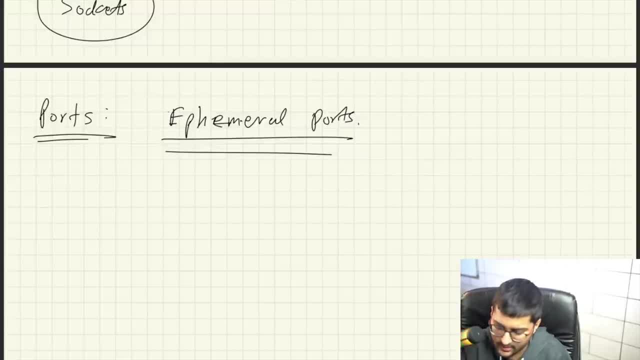 for your http so what the application like it will do internally is it will assign itself random 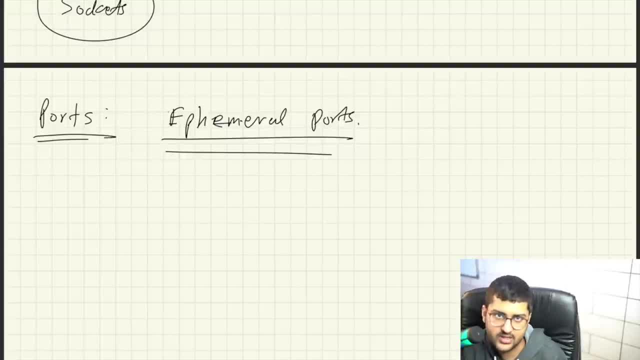 number port numbers and it will work with that if the multiple application instances are running 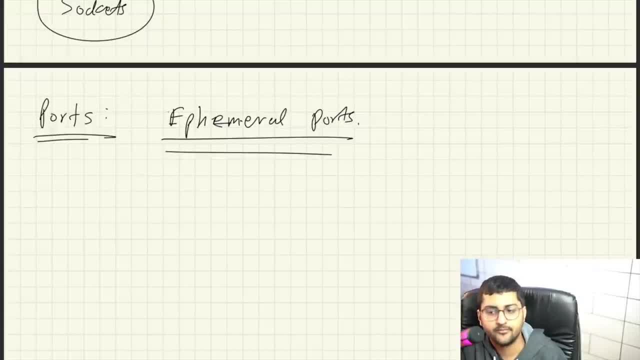 okay once the process is done it will be freed okay sound good cool so once the application is no longer using it the port will be free now these e-formal ports e ephemeral ports they can exist on the client side but on the server side you have to know the port number okay so servers uh you know you have should have like defined well defined split port number because clients need to know know about it internally internally they may use on its own like after the client has given the 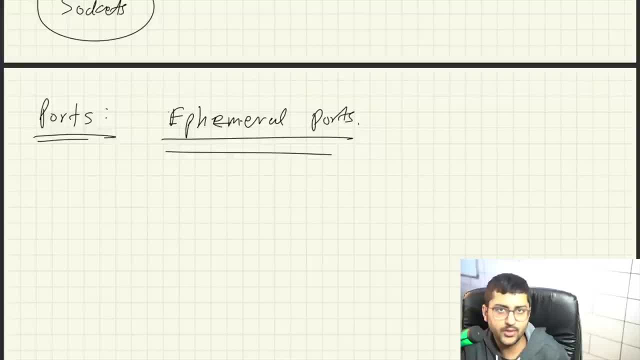 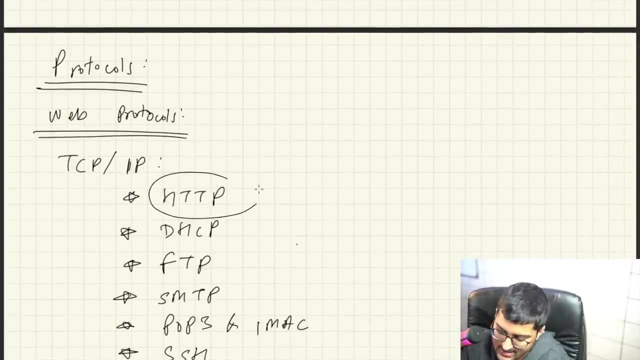 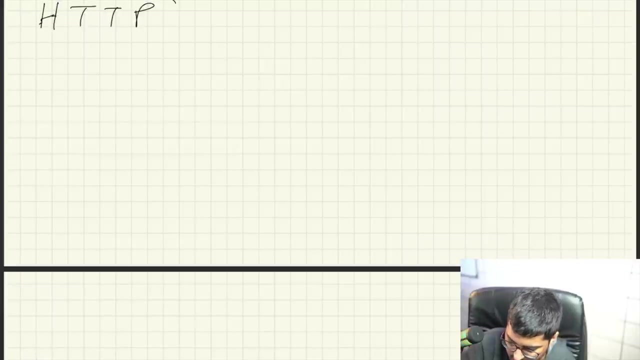 request then internally they can use these e e ephemeral ports but yeah that's basically about it cool so that was about how this communication stuff happens all right so we're still on the application layer and we talked a little bit about the brief let's talk about http in detail http what is http and how it works all right so http i know we have covered this before but 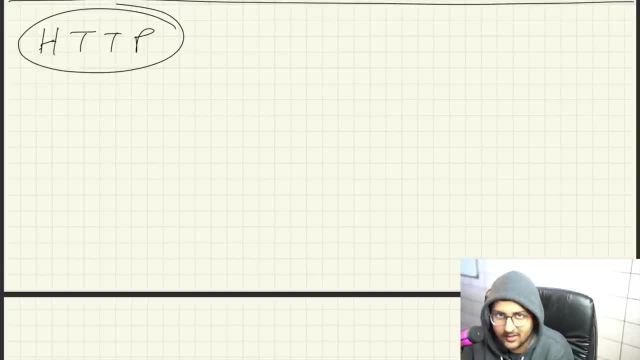 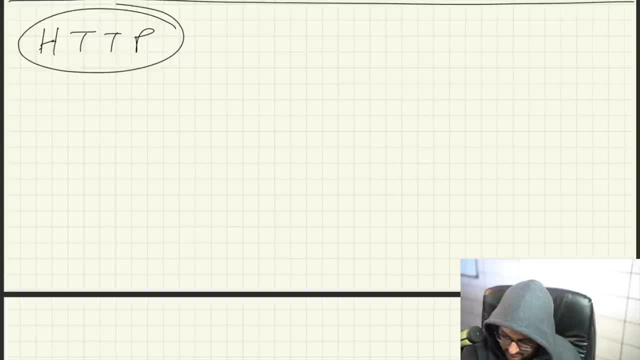 architecture okay you have a client i'll draw this diagram one more time because it's very important you have a client here you have your server here i gave you a little bit of an example 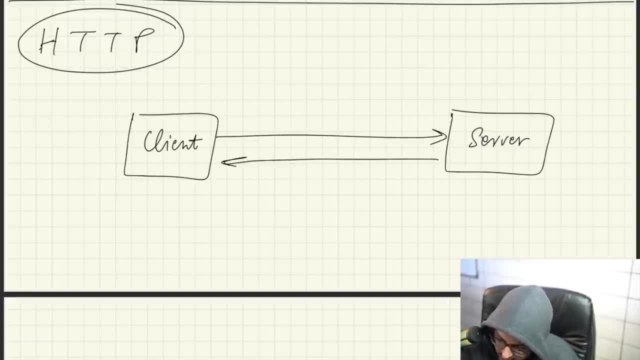 of like you know when you write google.com it gives yourself so you request something and the server will send you a response okay so this happens using the hdtip using the HTTP protocol you are like Kunal you are now annoying me please tell me what is HTTP 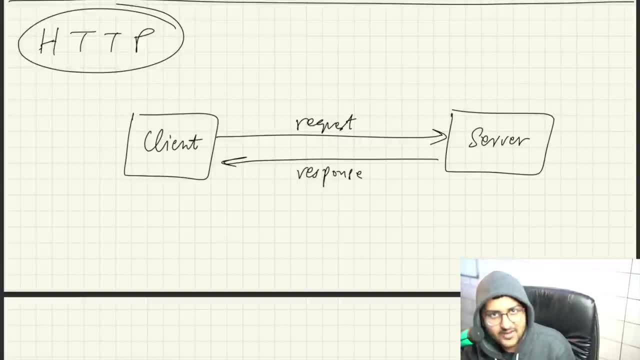 protocol I've actually told you pretty much a lot of times but here it goes again it is a client server protocol okay and it tells us how you request this data from the server and it also tells us how the server will send back data to the client so when you make a request when a client makes a request to the server that is known as an HTTP request and when the server sends back a 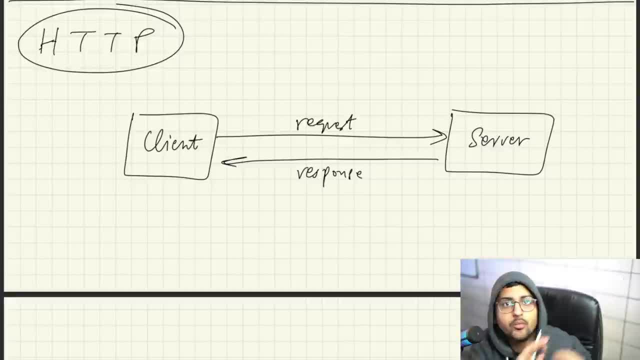 response to the client oh you wanted the google web page here you go I'll send you a bunch of stuff that is known as an HTTP response okay so basically these are application layer protocols 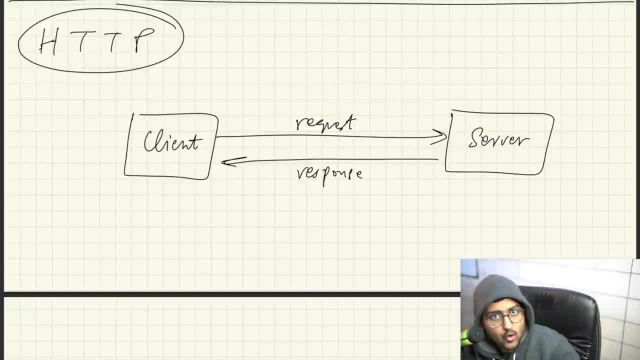 okay so every application layer protocol also requires some transport layer protocol okay 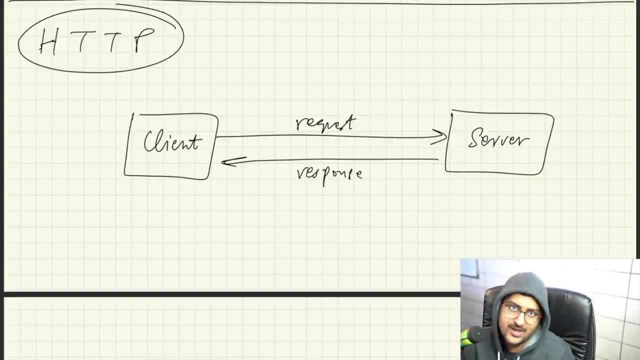 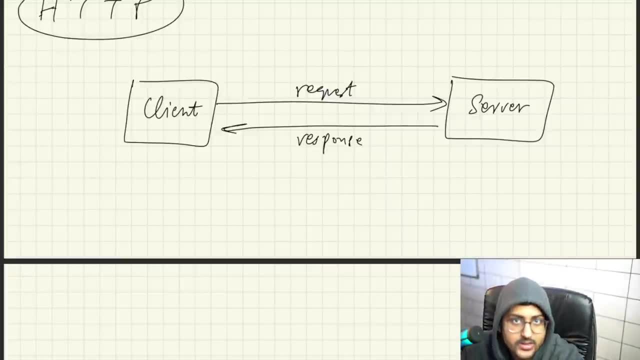 so this is basically an application layer protocol HTTP okay it has some methods like HTTP methods like get method push method so you want to get something so you use the get request 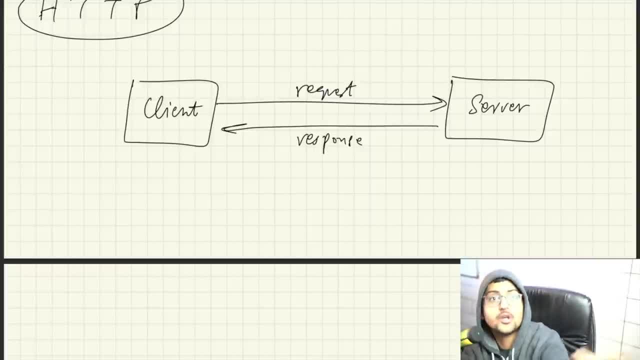 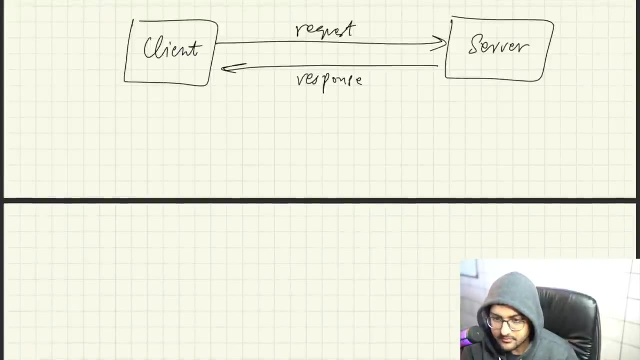 you want to post something when you submit a form you use the post request for example so here we know that uh what are some of the transport layer protocols TCP and UDP okay transmission control protocol user datagram protocol we have learned about this in brief that uh UDP like uh 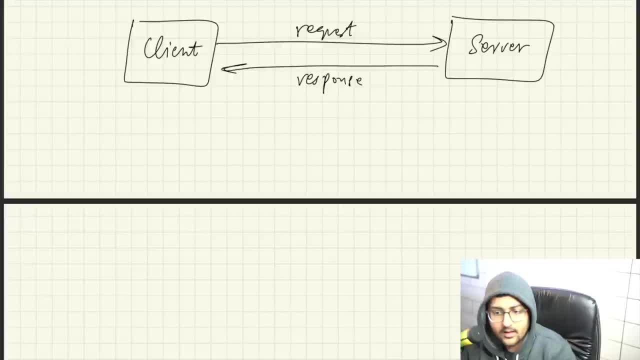 is used in like video conferencing and stuff so here uh HTTP actually uses TCP okay so HTTP now you know what it is uses TCP transmission control protocol inside it for example okay because TCP makes sure that all the data is received and everything okay HTTP does not store the state it's a stateless protocol 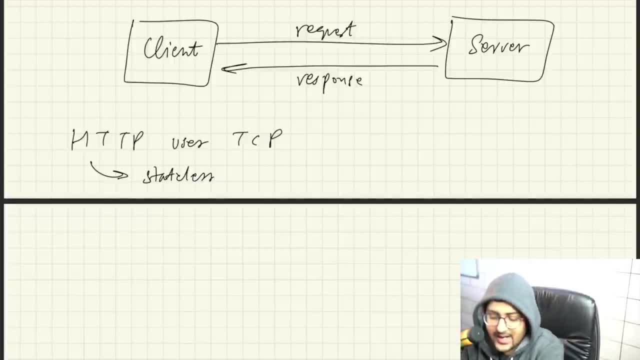 very important okay okay stateless protocols so server will not store any information about the client by default okay 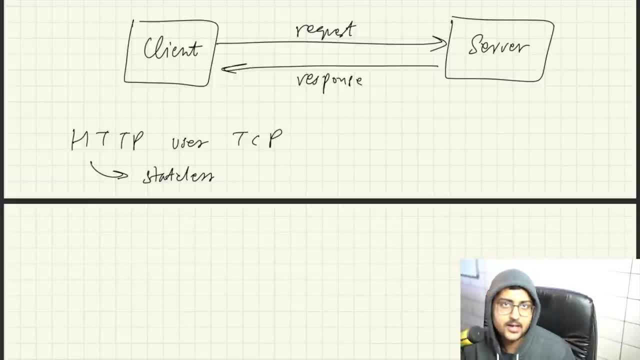 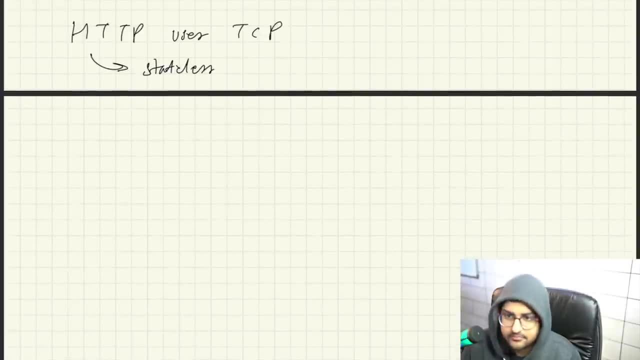 cool so example if the server is this client is making requests again and again and again server will not treat that as like a one single you know good client back there and go to straight to the website no good client okay cool awesome okay 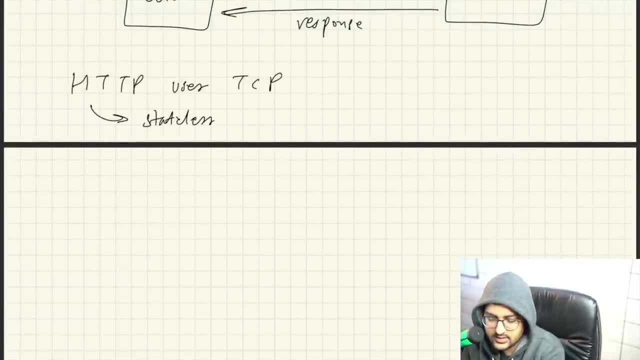 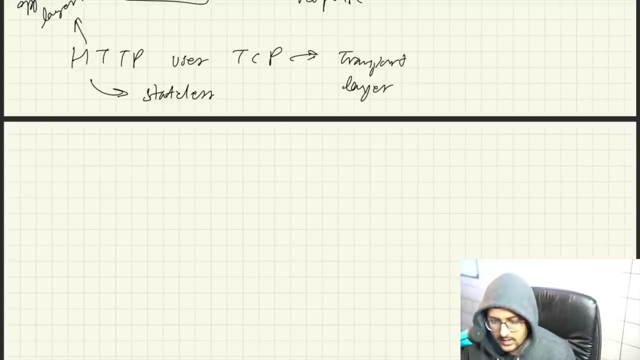 So, that's basically about it, this is an application layer protocol, application layer protocol, it's in the application layer obviously and it uses this in the transport layer, HTTP uses this in the transport layer. This layer, application layer, okay, sound good, TCP when we learn about it, this is actually connection oriented, it does not have to, you know, we don't have to lose any of the data that we are sending, that is why a connection has to be made with the servers and then once we get the connection, we will be able to send the data. 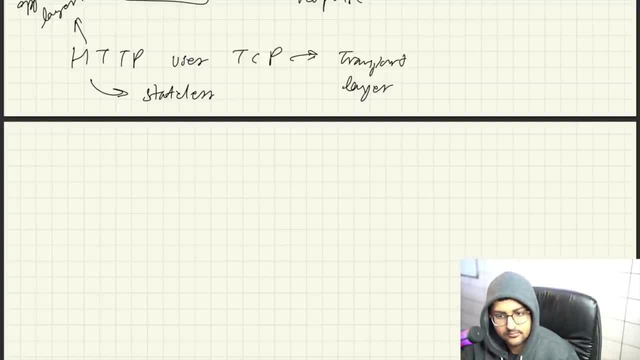 So, this is an application layer, application layer, okay, sound good, TCP when we learn about it, this is actually connection oriented, it does not have to, you know, we don't have to lose any of the data that we are sending, it does not have to, you know, we don't have to lose any of the data that we are sending, it does not have to, you know, we don't have the connection has been made, then you can exchange your data or whatever, okay, that is basically about it, okay. 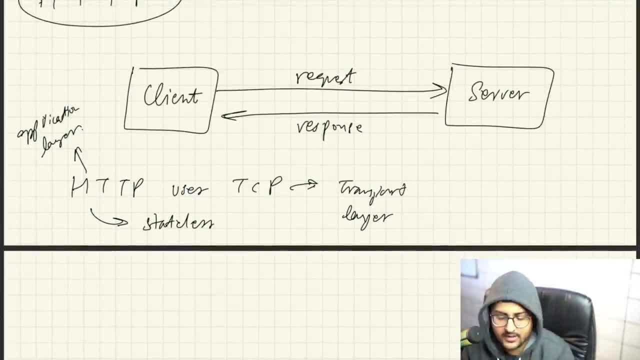 So, whenever something we get in the response for in the website, we know that web pages, www when we talked about it, what is it? It's just a collection of web pages. 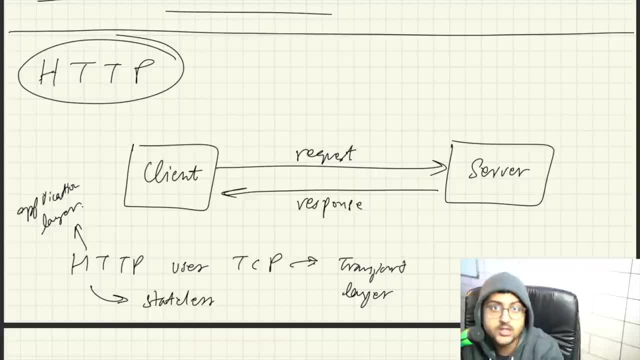 So, on web pages, you see links, you see text, you see documents, you see videos, you see images, you see objects, all of these things have their own specific URL, that is known as World Wide Web. Let's try to see it. Okay, so let's try to see this thing. 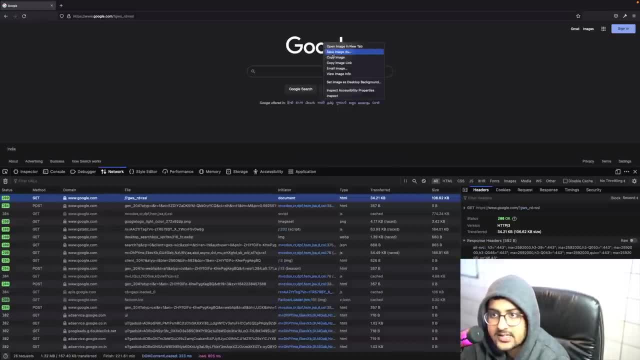 So, if I just talk about this thing, if I say open image in new tab, so this is a Google image, you can see this image itself has its own URL. 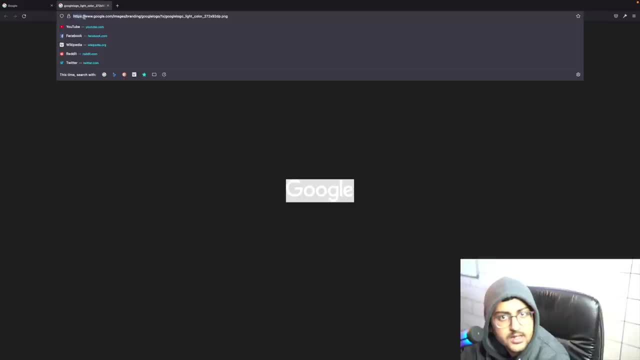 So, here this is the protocol HTTPS, this is the URL, okay, and this particular thing is the link to the resource. 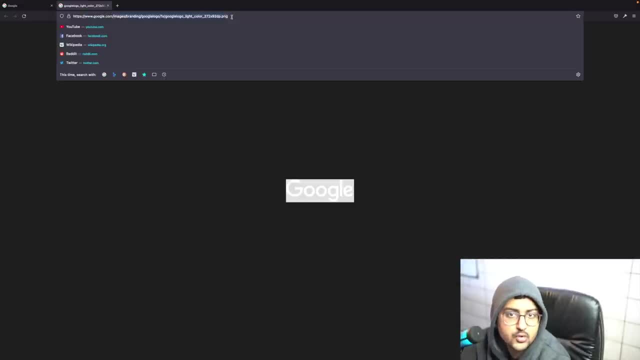 This google.com is the URL and this is the link to the resource of the, basically google.com is the URL. 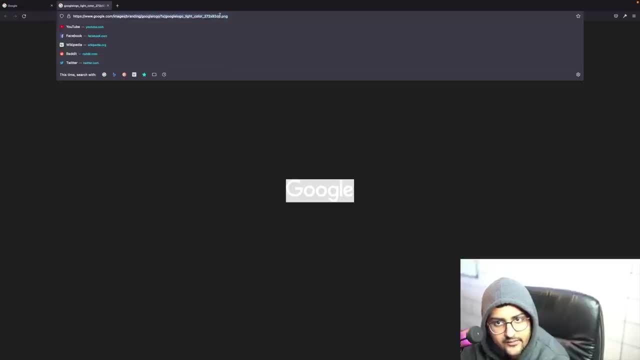 Okay, and in this server, these are the folders and stuff and it contains the dot png file over here, google. 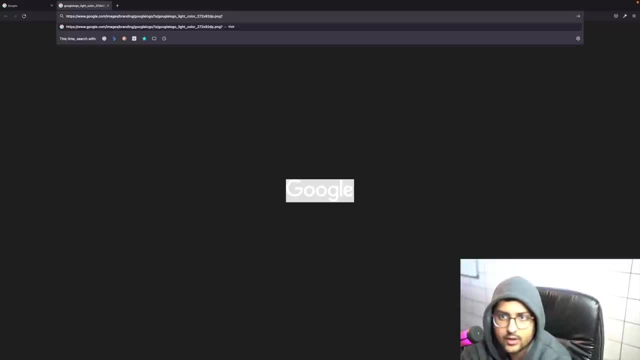 Okay, you can also add some arguments, like you know, many of times you have some arguments or something like that. So, you can add arguments over here as well. 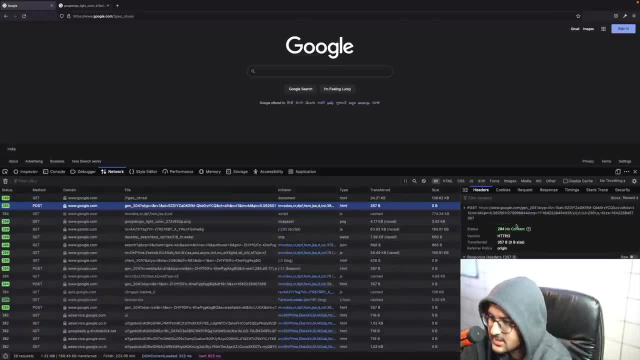 So, over here, if I talk about this thing, so you can see that it has the file question mark type is equal to IE or something like that, this question mark stuff. 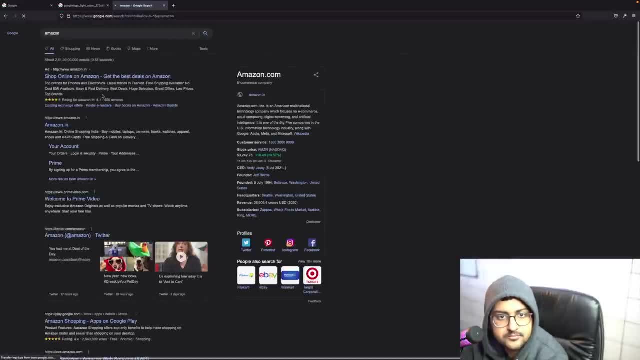 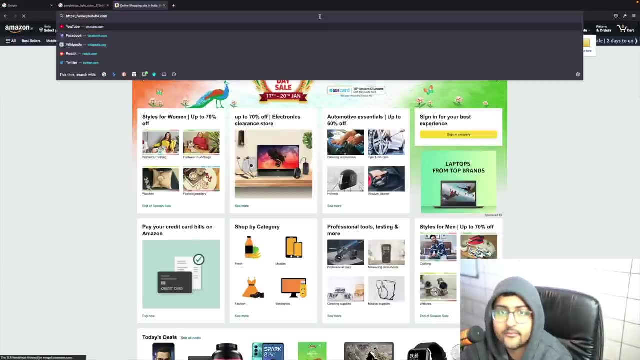 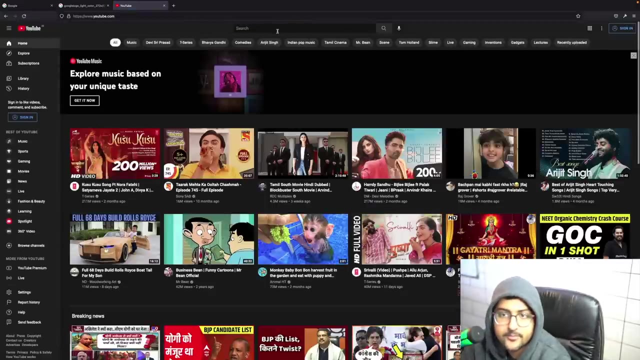 It's actually pretty common, you go to amazon.com, okay, so here you can see, it has a little bit of, or if I just go to youtube.com, okay, I play Mr. Bean or something. 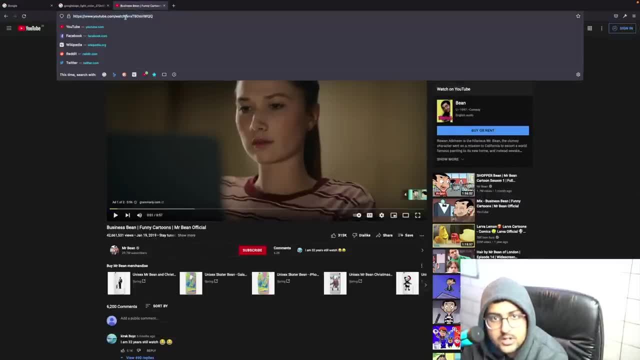 So, here you can see, here's some argument, video is equal, so you go to this URL and the argument is question mark, after question mark. Everything you put is an argument. So, video is equal to this video ID, hence it will play this video ID. Okay, cool. 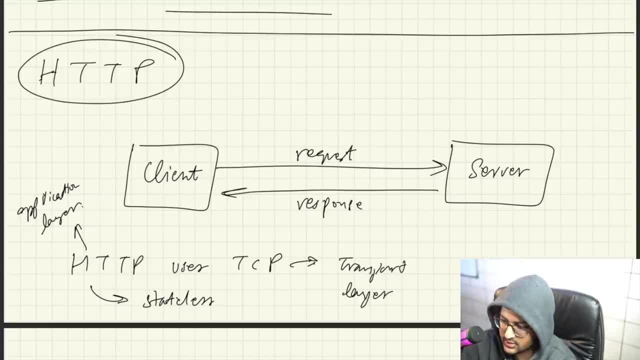 And in this photo, I'm talking about the request and response, you can see that as well. Refresh, click on any particular thing, say this one. 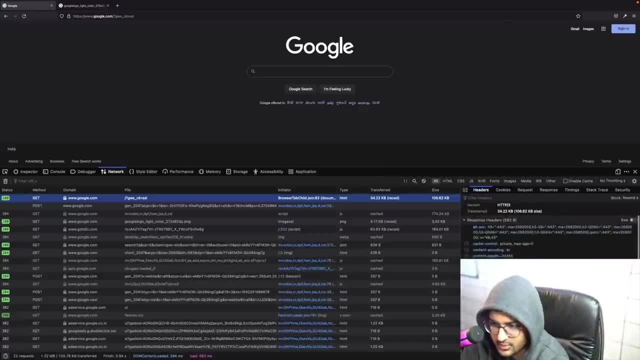 So, you can see these are the response headers, these are all the things you got into response, these are the request headers. 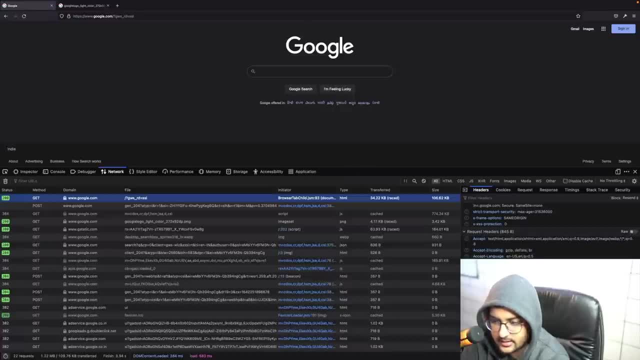 Okay, host name is there, TLE. Okay, so many cookie and connection and cache control, so many things are available. 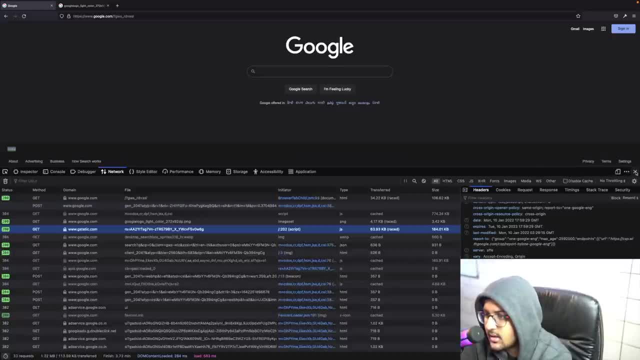 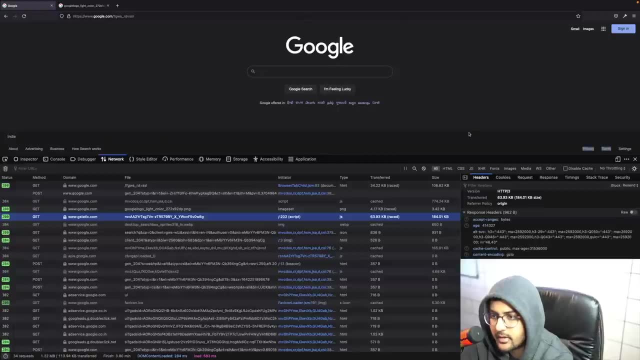 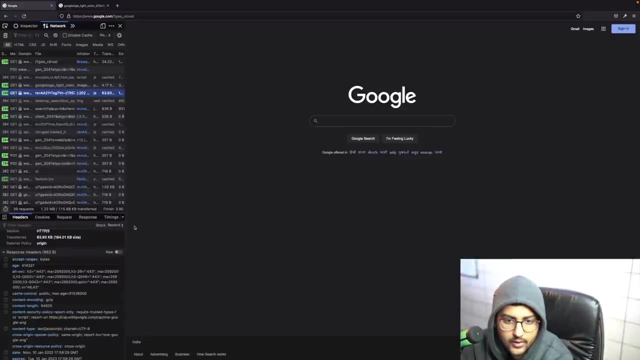 Okay, okay, I'm just going to move it because I know you can't see. Let me move it somewhere. How do I, how do we move it? Yeah, I can do it to the left, for example. Okay, and I'm just going to expand this. Made a request, refresh. Okay, how to get this thing? Just right-click, inspect. Okay, you can do this in Google Chrome also. 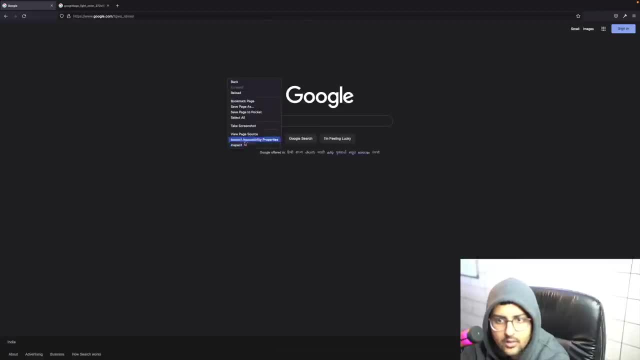 Click on any link, you can see the status. If I just go back, okay, inspect, network, refresh. 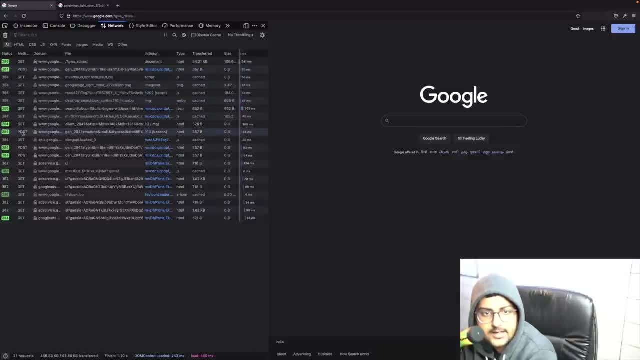 So, you can see type of method, get, post, get, get, get, get, get, post, get, post, get, etc. Okay, let's talk about the types of these methods. 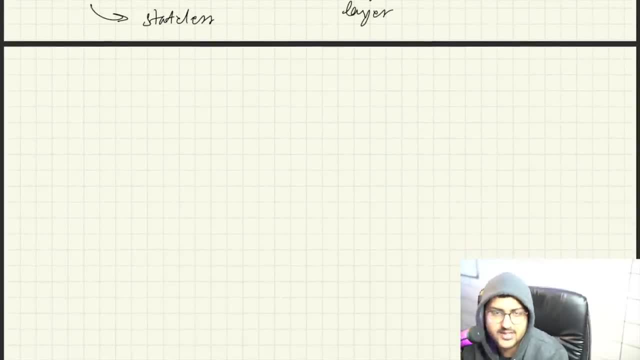 Okay, so we have, when we talk about like HTTP methods, what is the method? Well, first of all, tell us that. 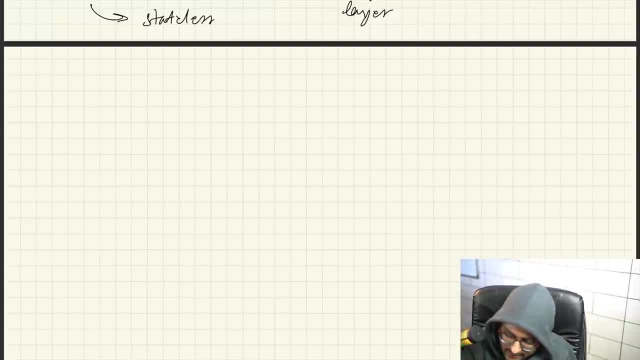 The method is basically that is telling the server what to do. Okay, if you have get. Get method. So, you made a get request, let's say. We say something like that. HTTP methods. 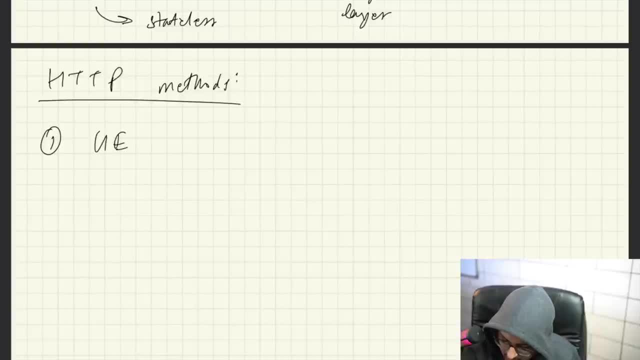 Okay, let's talk about first one, let's say, get. So, get basically means that you are requesting some data. Hey, give me the web page. 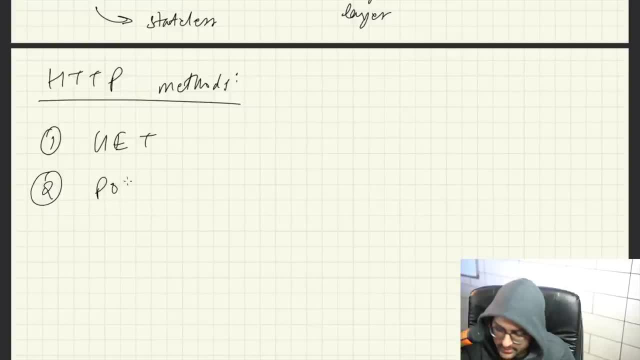 Give me this YouTube video or whatever. Second one is post method. Something like, hey, I am a client and I am giving something to the server. Like a web form. When you register somewhere, username, password or whatever. That is a post request. 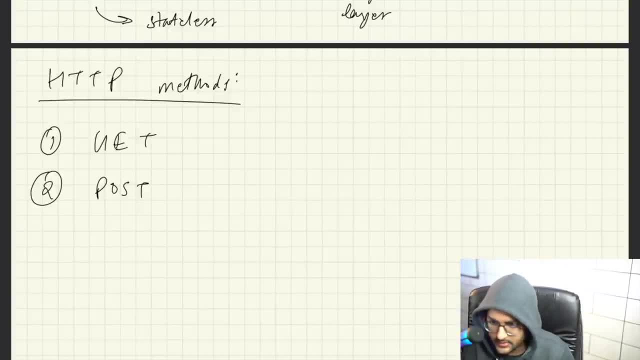 Okay, and then there is something known as put. Okay, put as well. Cool. 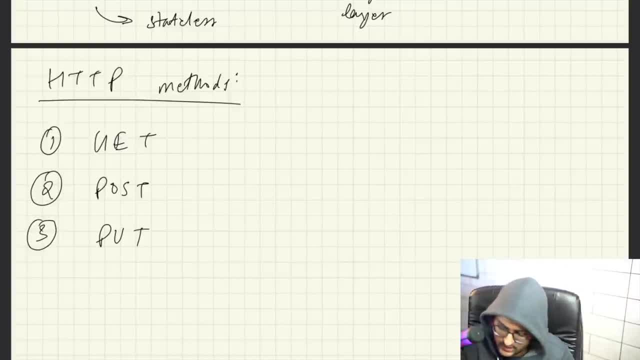 So, it basically puts data at a specific location. There is one known as delete as well. 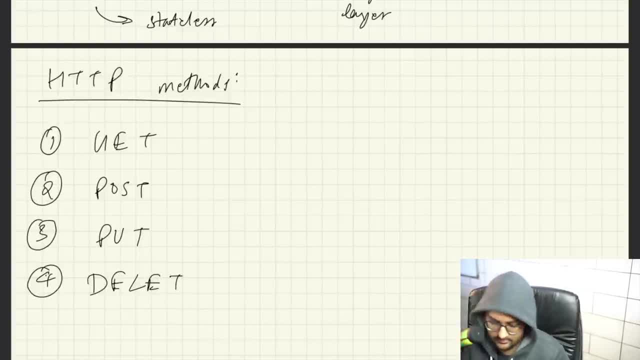 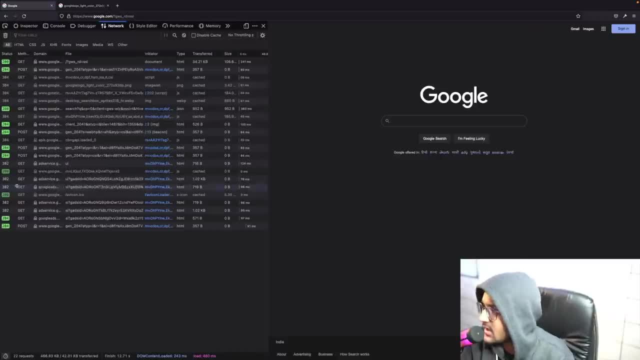 Okay. Okay. Okay. Okay. Okay. Okay. Okay. I had a lot of questions so far. Okay. No problem. 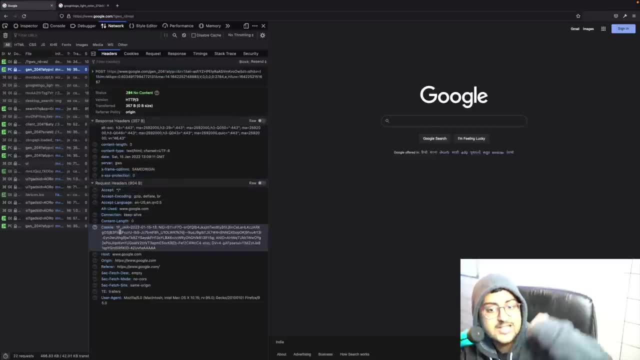 Okay, and here you can see the request headers and the responses of what did we send to the server. Okay? 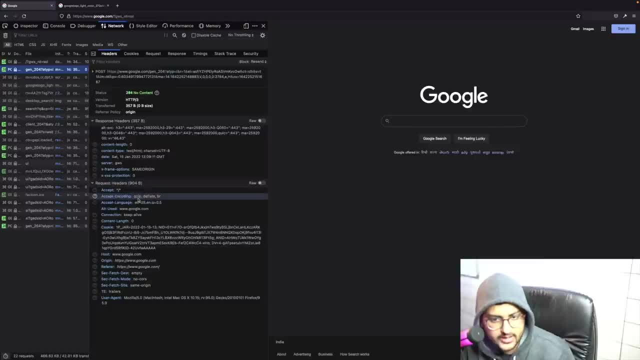 So I think over here, you can see X except except encoding. It encodes it's except this encoding, except language. You want to see what all these tags? 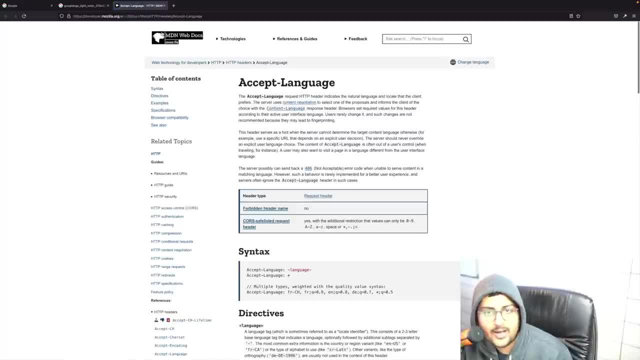 present just click on the question mark it will open up mdn web docs okay so it says accept language request http header indicates the natural language that the client prefers for example here it says english 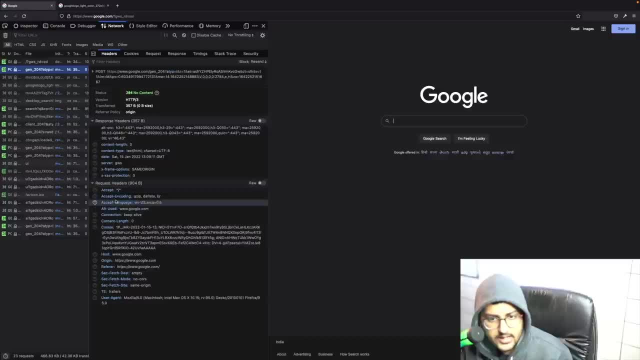 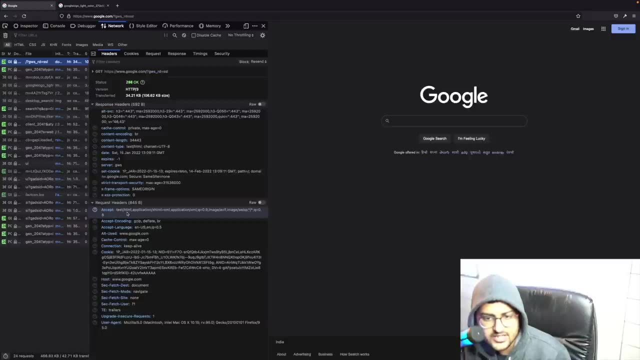 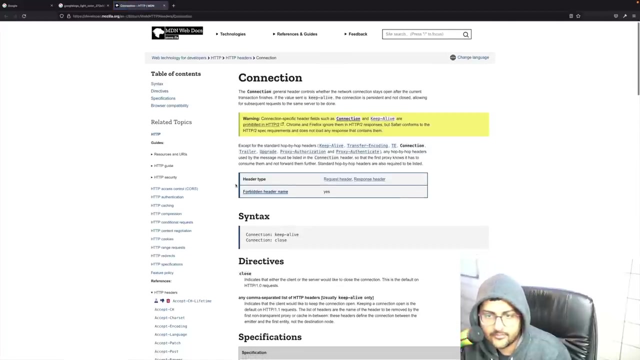 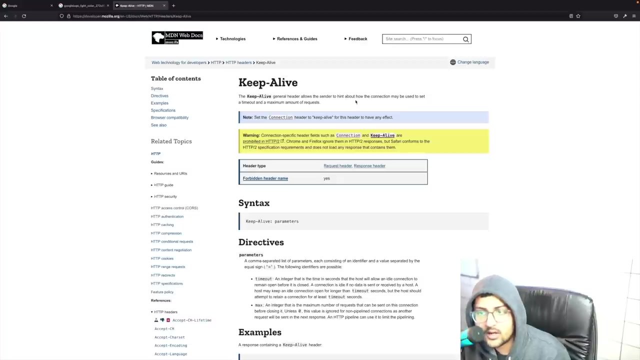 okay and here it says accept like what type of response are you trying to accept so here it's saying let's say i am only trying to accept text html application stuff okay encoding is mentioned over here connection keep alive is mentioned over here right so it's the type of the connection so here you can see more about it cool keep alive keep alive general head allows the sender to hit above hint about the connection may be used to set a 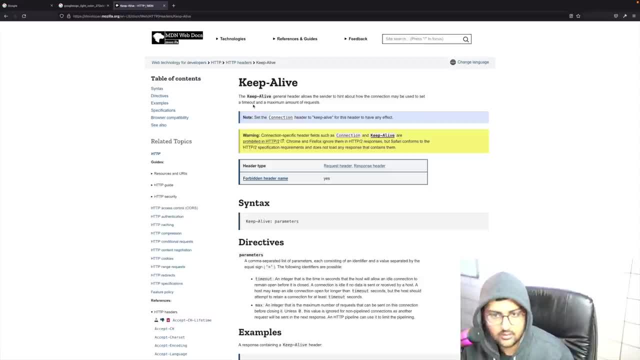 time out and a maximum amount of requests for example okay so for example if uh if you if you're talking about 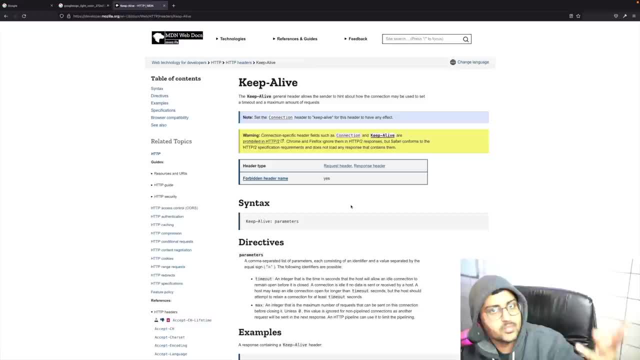 uh the connection to be like closed i believe as well then it's not persistent okay here it's saying that this allows us uh to hint about like how the connection may be used to set a timeout 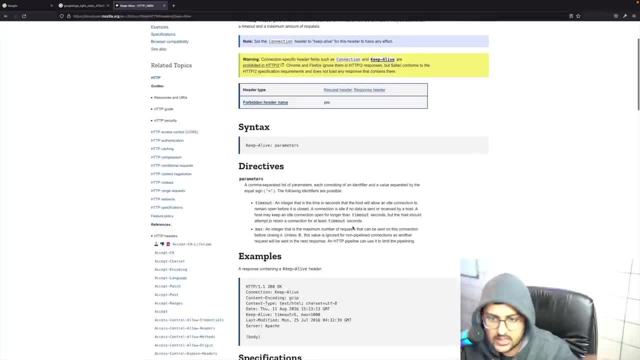 okay so you can set up a timeout out of the amount of requests like after this many amounts or whatever okay so you can set a timeout and the maximum number of requests that can be sent on 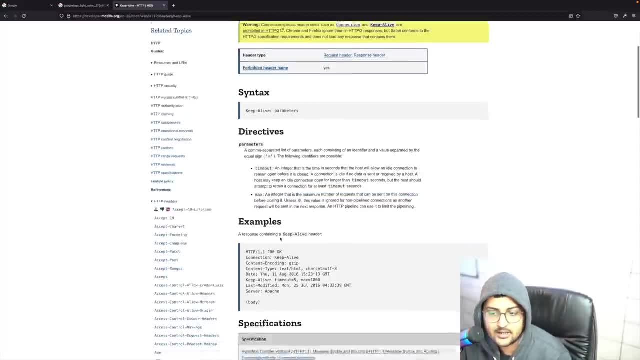 this connection before closing it you can mention that okay so these are the responses that is also 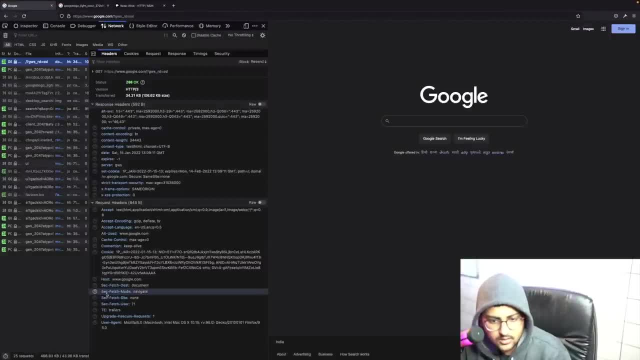 being today one of the most popular responses i have seen is uh a comment on an app called vpn that's basically a function which is uh the thing that or a convo in vpn is 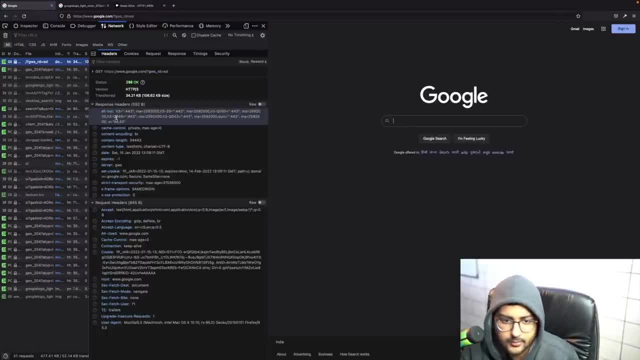 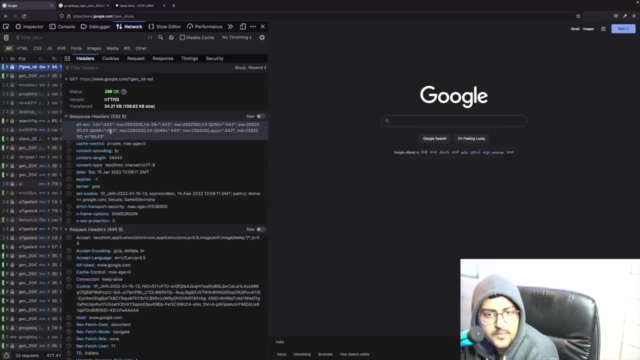 essentially you have to uh apply the method of this app to our vpn which is to import the account um the code from the vpn which is the vpn which is the source code the vpn name of the 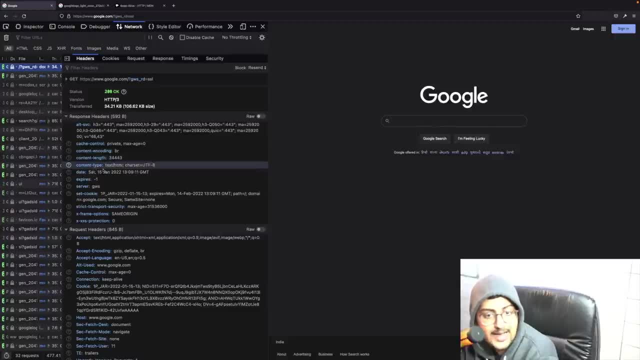 account uh so this is the link to the vpn you can see it's basically the same thing just change it to a different class or a discus code you can see it's like that okay and i will see later on you know the server and the cookie information so on and so forth everything is available over here 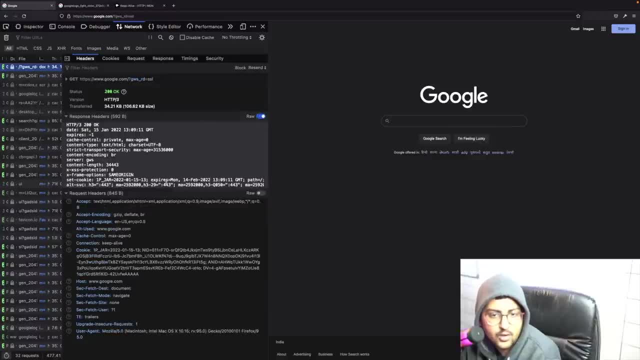 this is the raw raw one okay these are the status codes let's talk about this is the http version 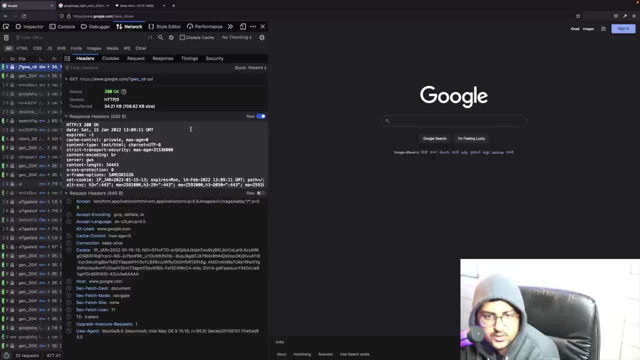 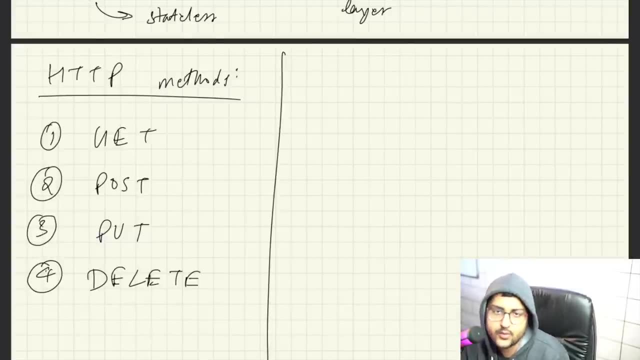 http version this is like the status code let's talk about the status codes a little bit more okay so when you send a request to the server you need some sort of a way to know whether the request was successful or did it fail or something like that or what happened okay for that there 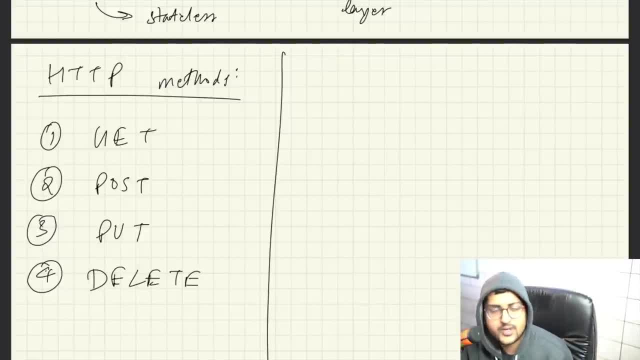 exist status codes status codes exist for that for example 200 means that the request was successful 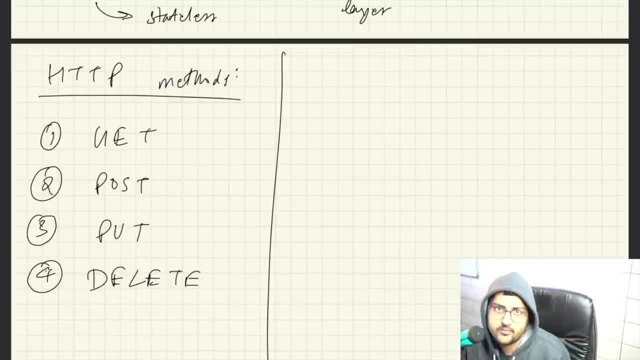 okay and we have everything 404 means what it you know you could not find it okay 400 means like it's a it's a bad bad request right um and 500 means like there's some internal server error 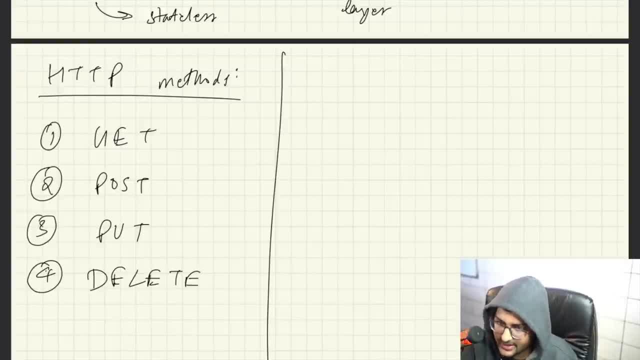 for example so there's like a class for this like uh error codes okay or status codes there are like some classes for this status codes if it lies in like the 100 range okay these are basically like uh informational category codes 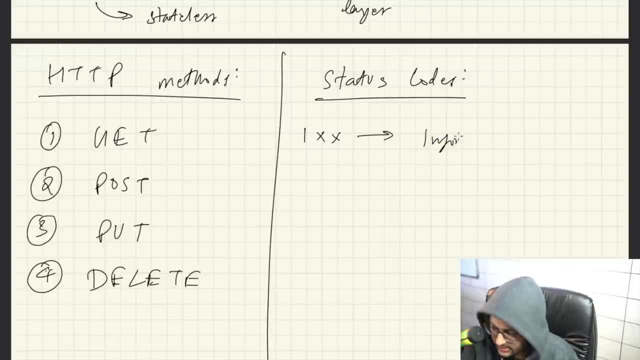 okay and if it lies like information related informational category when we're talking about 200 ranges success codes okay when we're talking about 300 range codes 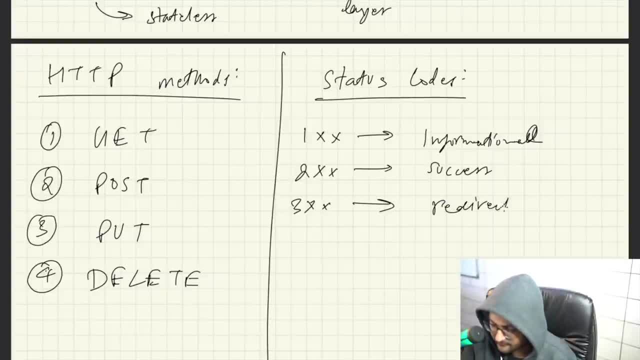 redirection purposes redirecting when you talk about 400 codes this is the client error that's something you did client error like you may press the false url or whatever 500 means server error 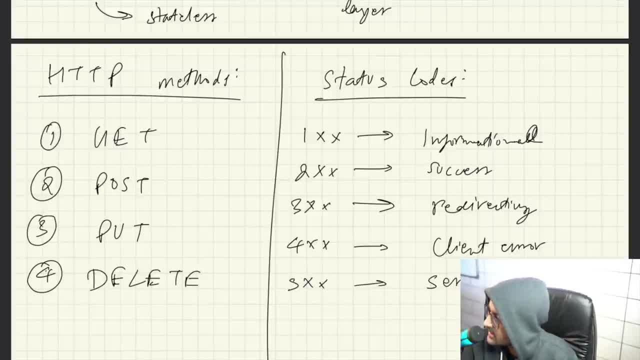 okay then this is that there's a error with the server cool so we saw requests in like the real 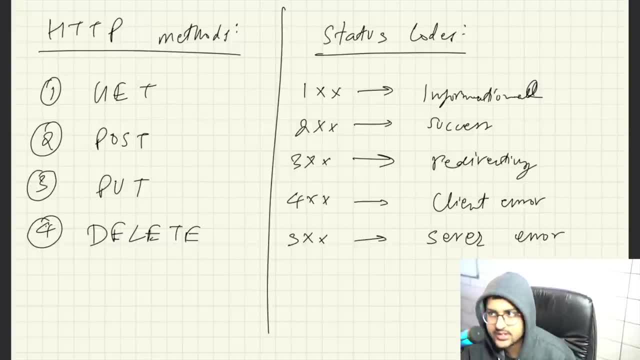 world and that was basically about about http requests and stuff so so many types get put to you know post and stuff like that 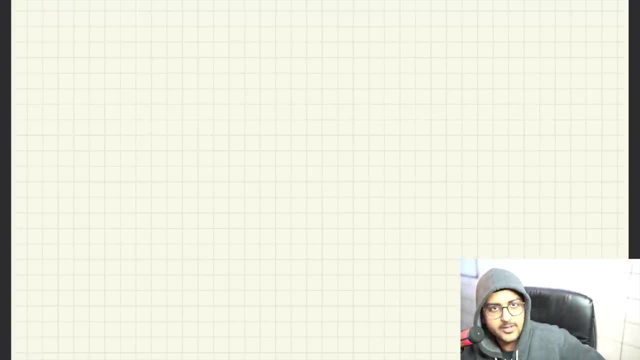 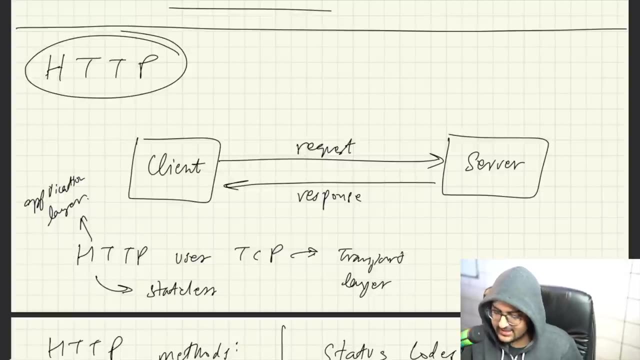 all right let's move forward okay now let's move forward so we're still talking about the application layer we're still talking about like http let's let's give you let me ask you a question now so i told you that this is like stateless over here you can see that http is stateless protocol 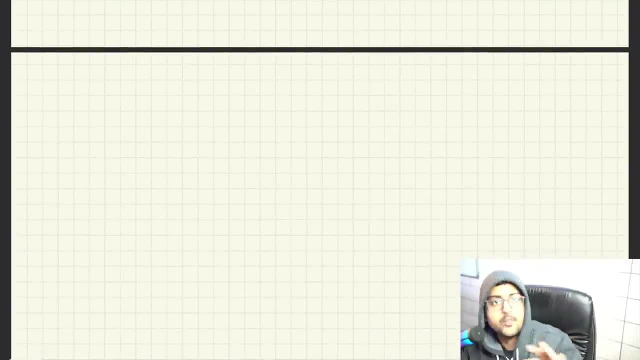 means you're visiting a website you visit the website again and again it will not maintain the state of you every time you visit a website you'll be like hey it's a new person visiting a website or 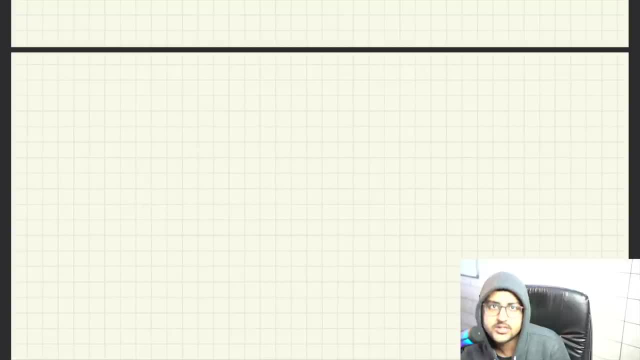 whatever but you might be confused like you know that's not how it works in the real world if i'm making like if i log into amazon or something and then i close the browser and then i start the browser again and i go to that particular website again it will stay it will save my session right it will save the items in the cart you will still be logged in it will not ask you to log out and 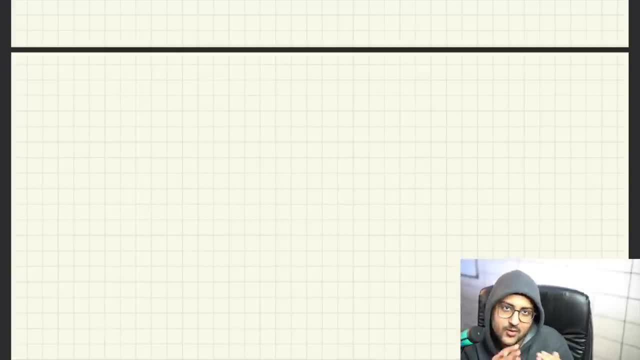 log in again right does that happen when you log out so when you close the browser it automatically logs you out no right so like kunal 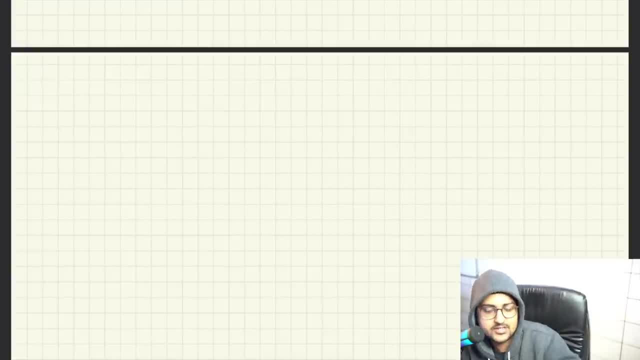 http is stateless with every time you visit state is not saved uh but you're still saying like this state saving behavior exists like this we have noticed it ourselves how does it happen the answer 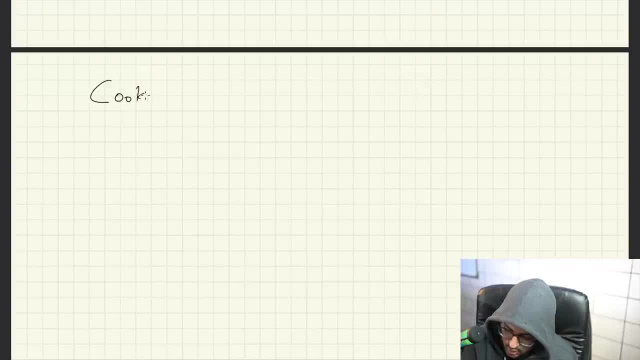 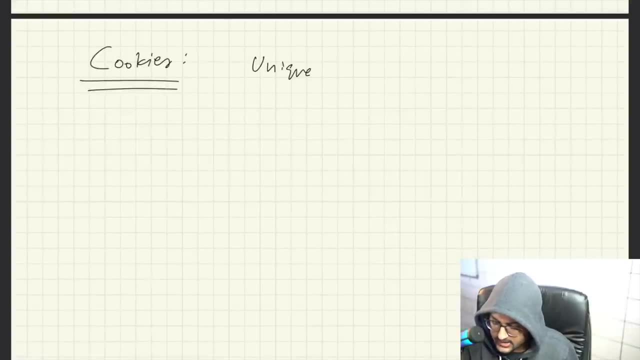 is cookies cookies what is a cookie cookie is a unique string okay it is a unique string 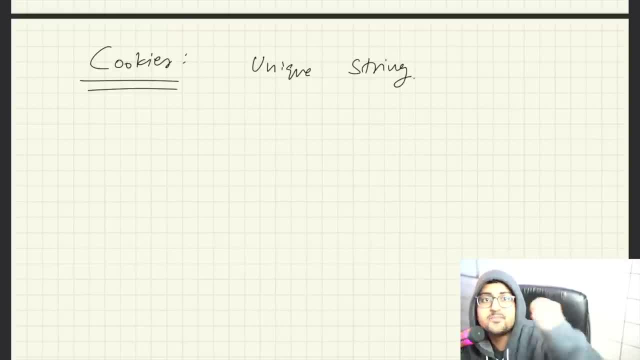 so basically it is stored on the client's browser our browser it is stored over there it's a file that is stored in my browser okay stored in my 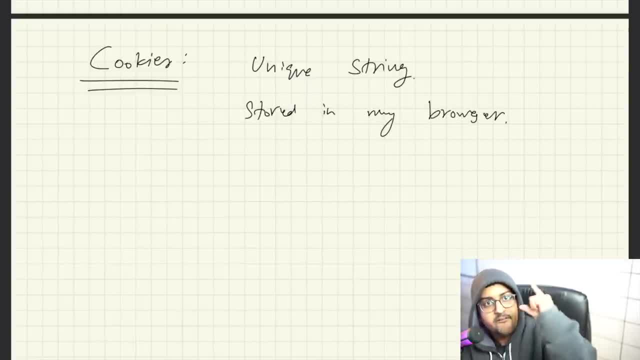 browser okay when the first time this cookie is set when you visit the application on a website you visit for the very first time it will set a cookie 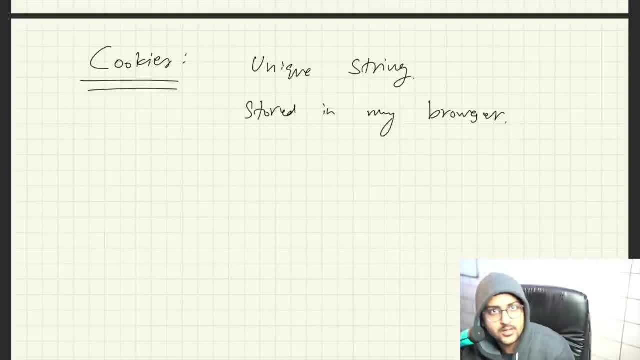 okay and after that whenever you make a new request in that requests header a cookie will be sent then the server will know oh this request is coming from kunal and uh kunal has sent me this cookie let me check my 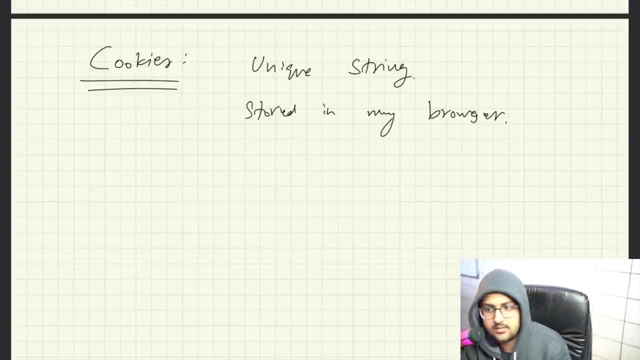 database then the server will check the database and it will find the uh the state for that 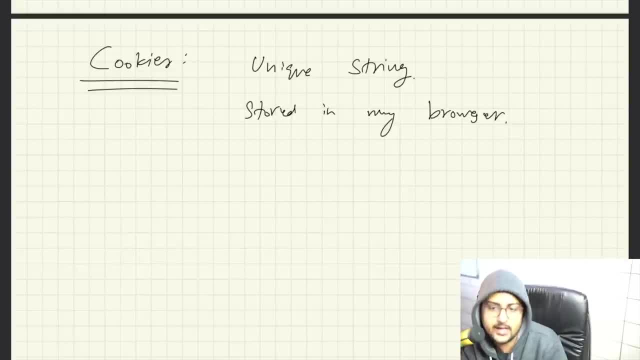 the server will know like who is contacting okay so you will send the request in a http you know in an http http request you will send the cookie and in the http response this will be cookie this is going to be a cookie stored in your browser and there's going to be some cookie data in the server 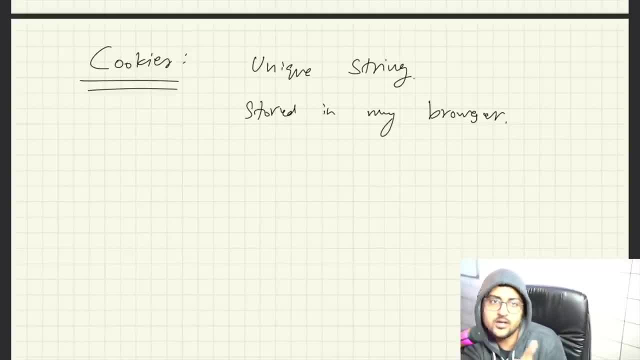 okay user value basically okay this cookie user value is kunal's cookie for example okay so let's see how little a little bit more how it works in detail so here you can see in the 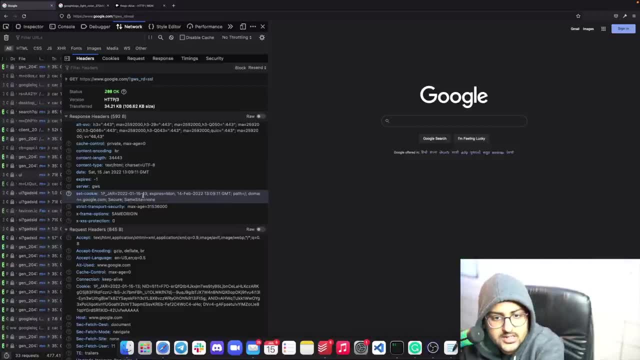 response whenever a server wants to set up a cookie here you can see in the response it has a 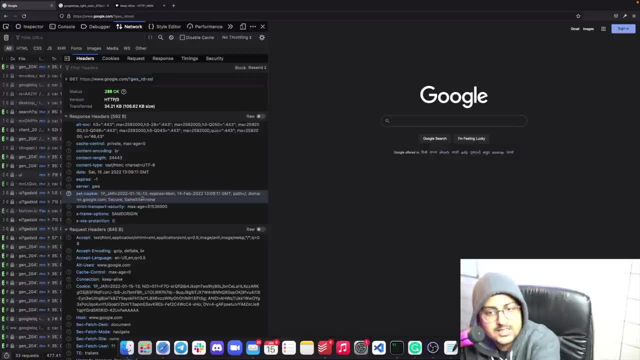 tag called set dash cookie it has some url names and like some path and stuff like that and here it has the expiration date so this is the expiration date for the cookie just like you know like cookies expire here also cookies expire that's basically how it works okay you can see in this header or here you can see the string over in this header as well 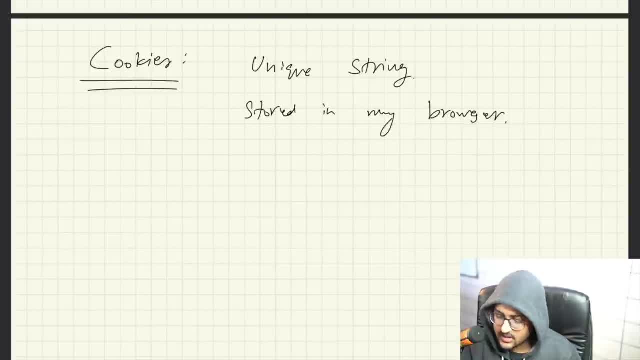 that's it we talked about headers already okay but sometimes like cookies uh you know can be misused by like websites and companies and things like that to you know just track you when you visit the website and show you like what's nice or whatever like it it's not everyone is comfortable with such things right knowing when you visit the website or whatever okay there's one more thing 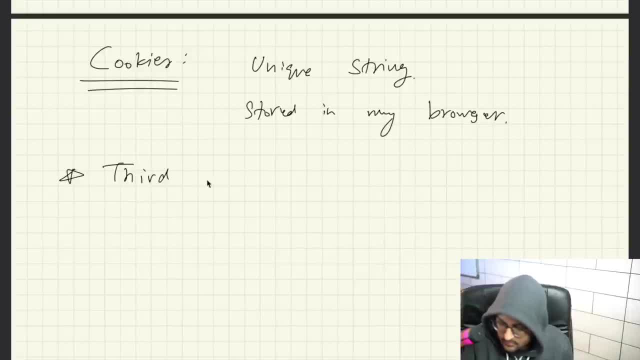 known as third-party cookies in safari and stuff you know in browsers you may see some options at times like uh you want to disable third-party cookies or whatever okay so third-party cookies basically cookies that are set for the urls that you do not visit okay for example you visit uh flipkart.com or some other website xyz.com it has it an integrated like um you know um ad for example for some other website so that way some website may use your cookies the website you may not have visited so try to google about this on your own like how to block third-party cookies what you want to do is you want to make sure that you have a website where you can use your cookies 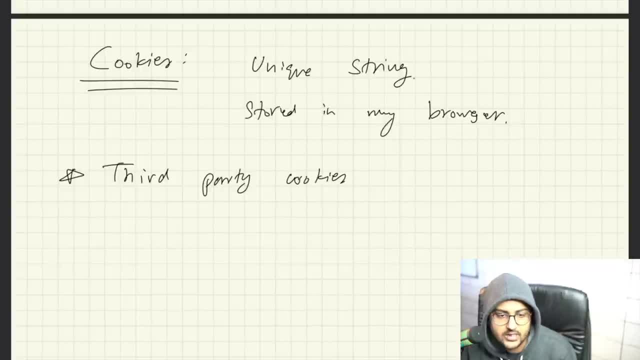 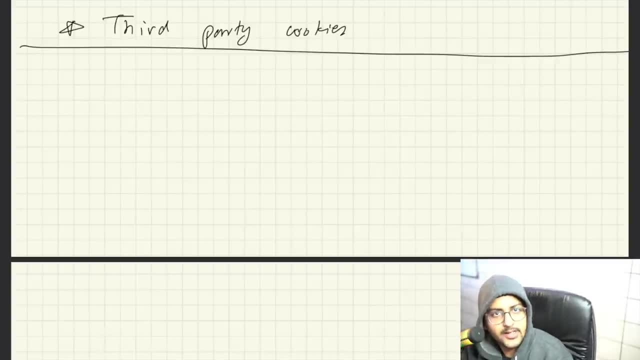 all measures you can take and how some companies are you know managing cookies and uh what always they use cookies for so google about it okay so that was about like http okay that was it 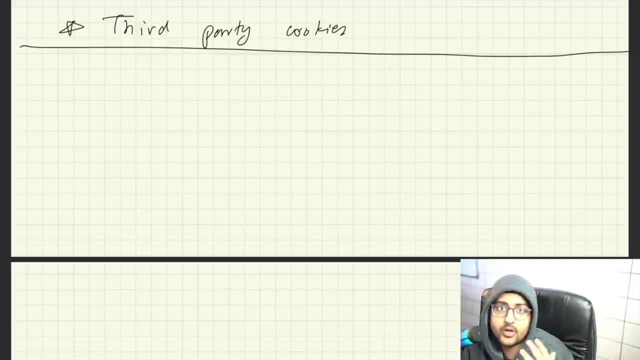 about http um one more thing than an application layer what other applications do we interact with email also right so let's see how email works how email works so .whatistheapplicationlevelprotocolforemail. 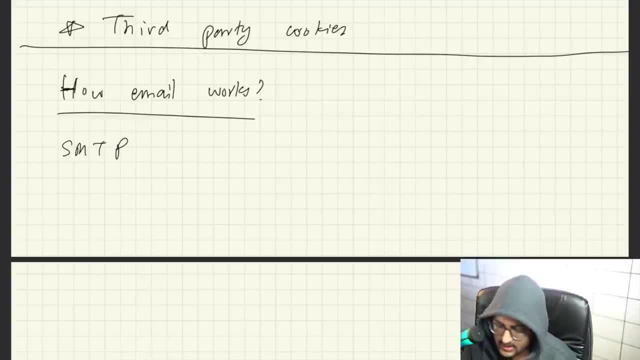 for sending email it's smtp as i mentioned previously uh it's known as simple mail transfer protocol okay it's used to send email to people in order to receive it you can use something 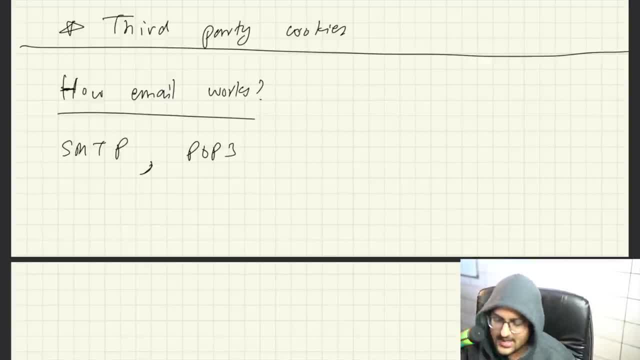 like pop3 or something okay so this is the application layer protocol at the application 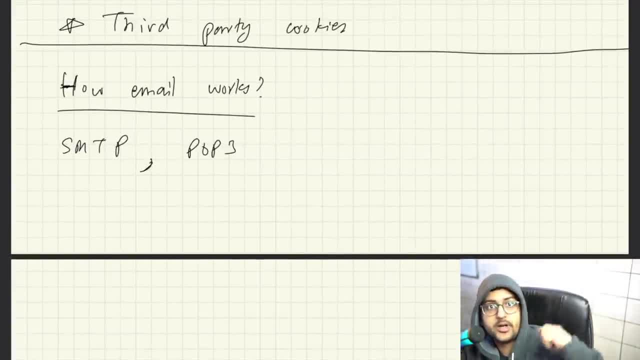 layer but how is the data going to be transported which transport layer protocol do we use 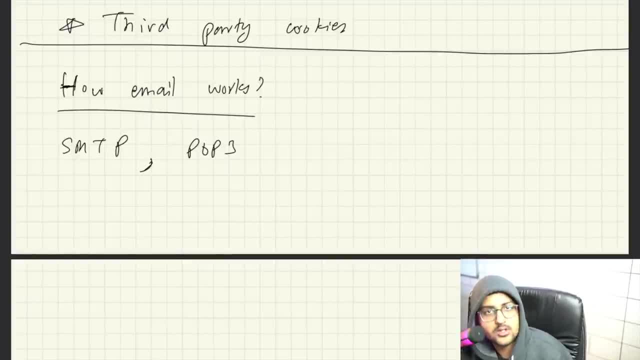 pcb or udpi UDP we know some data will be lost do you want your email data to be lost emails are very important 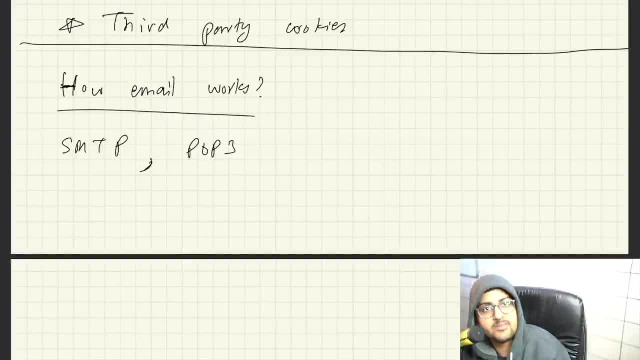 things you want to be you want to send entire email right how tcp works how udp works i will teach you in transport layer okay so forget about that right now just think about what it's doing 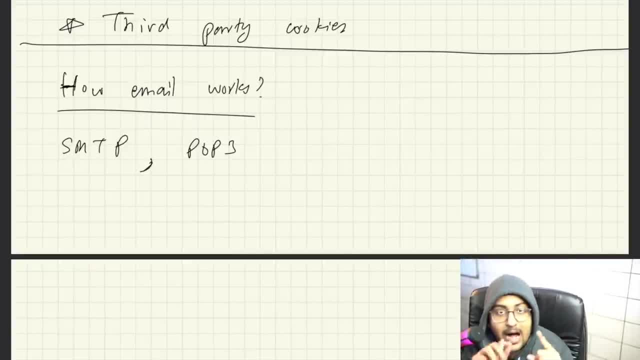 tcp and udp what tcp and udp are doing the how how it's happening we are talking about application layer now okay so i'll be teaching you how application layer protocols work so i taught 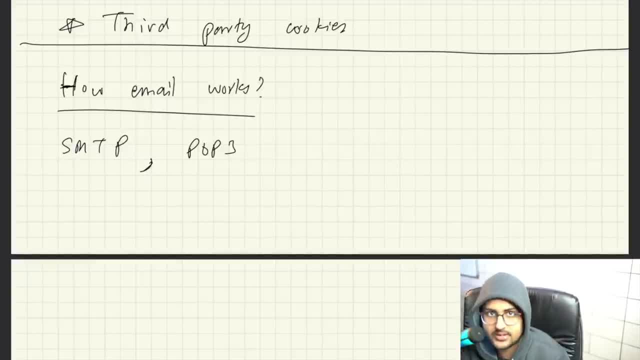 you how http works now i'm teaching you how email works okay so which transport layer protocol will email use tcp or udp tcp because we want the entire data available to us isn't that what we want 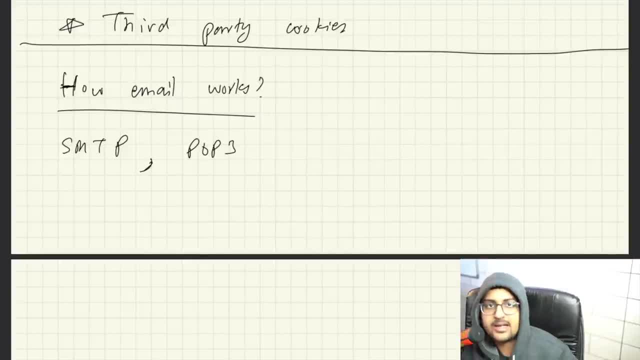 so that is what happens if i'm talking about s smtp like simple mail transfer how to send the email so basically the email clients like if i'm using google 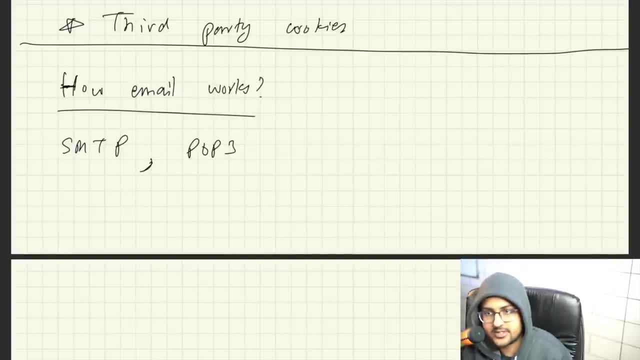 dot gmail.com or whatever they will have their own servers they will have their own servers so let's say you're sending an email from yahoo.com to gmail.com and what will happen is 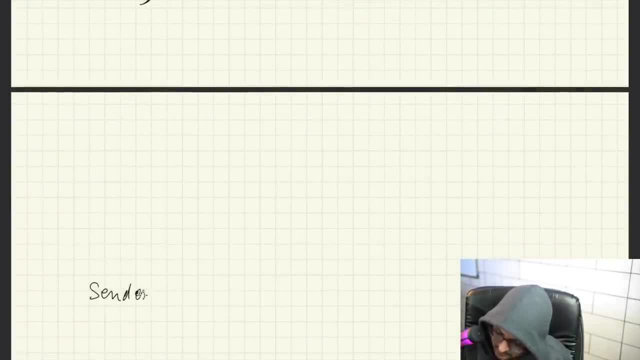 that you are sending the data this is the sender okay so what will happen is that the sender is going to send the email to the sender's smtp server 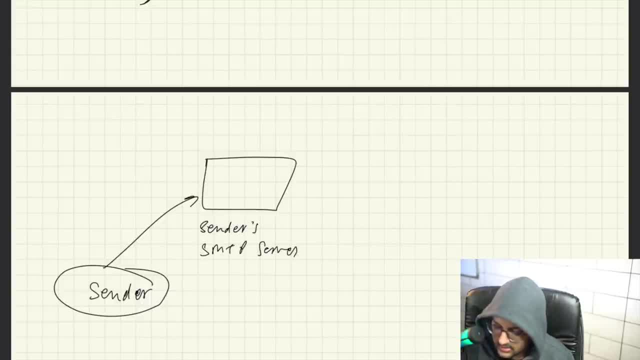 senders smtp server the email will 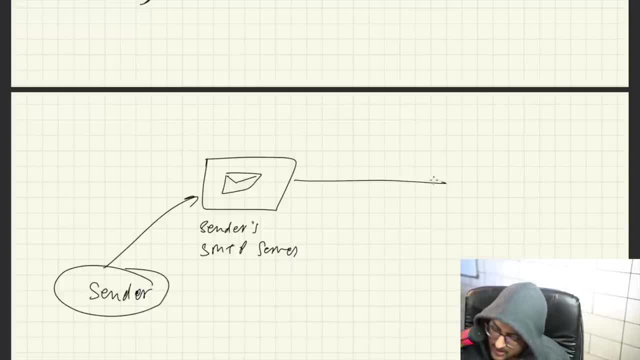 live over here for a while okay it will then make a connection with the receivers smtp server 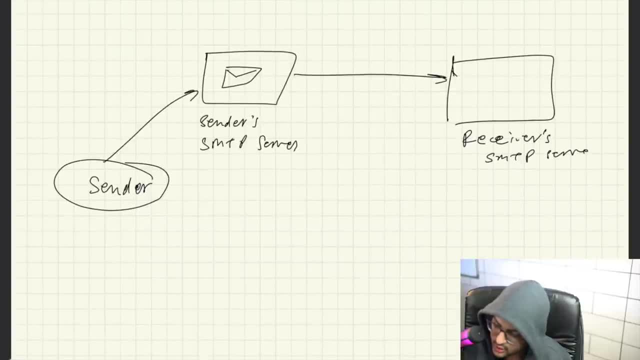 you can get the data of this server as well uh information which i'll show you later on okay after the connection is established this is transferred to this server this is the receiver 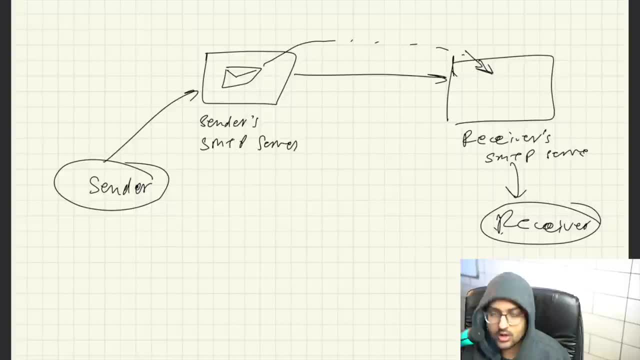 now when the receiver logs into the system as you may see whenever you log into an email client when you log into your email application and refresh it it's it below it says downloading email from server in iphone it does right that's basically what it does after that receiver is like a is it downloading something then it downloads the new emails that is how it 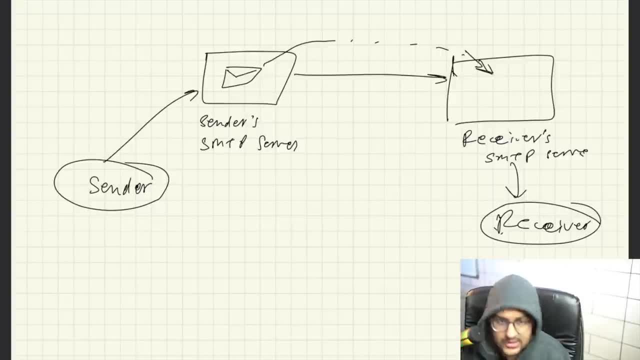 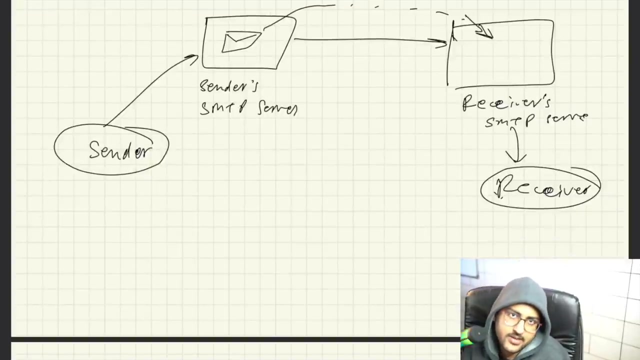 works so internally it's using tcp how tcp works we'll cover in transports here right now this is what is happening so you push the email to your server that will connect to but by the way if both the receivers are on the same uh you know account for example both are using google gmail.com then this thing does not happen this thing this connection thing does not happen it directly transfers it okay cool and there may be many scenarios in which like uh 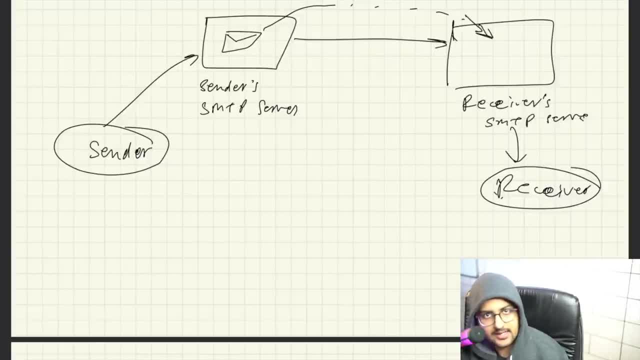 error handling may be required like message not delivered or something like that 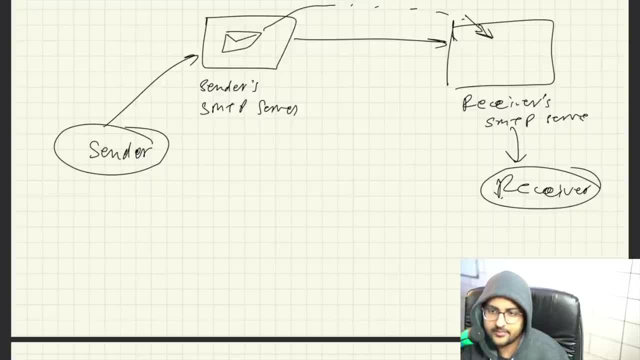 right so it uh sometimes happens that um you know if the if this server is offline the receiving server is offline right then this sending server will keep on trying after a few for a few few few days before it gives up okay we'll talk more about that how error handling happens in like tcp okay 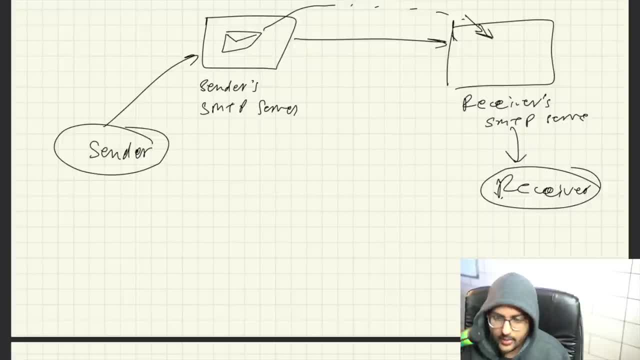 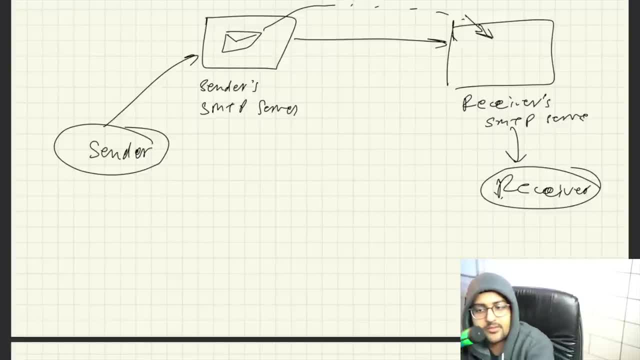 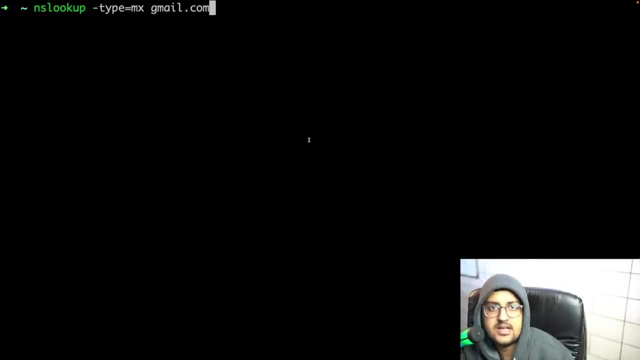 um the the name server lookup you can use the name server lookup command and you can find the name and the ip address of the smtp servers for various domains let's try to see that okay so you can use this i'm saying uh in this lookup type mx pins mail exchange it basically means smtp servers and for gmail.com there you got all the information 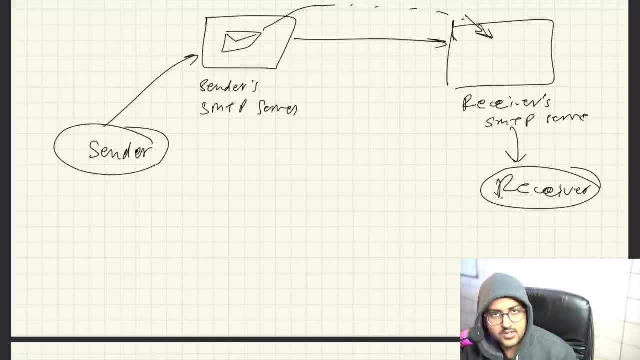 sound good all right okay so we learned about smtp which is used to send emails now let's look how you can download emails so one is known as pop okay pop uh pop basically means uh post office protocol okay basically this is how it works um you first connect the client connects to the pop server okay using tcp you can connect it it uses a port i believe 110 so you can connect it on port 110 it does all the author authorization you can obviously you have a username and password 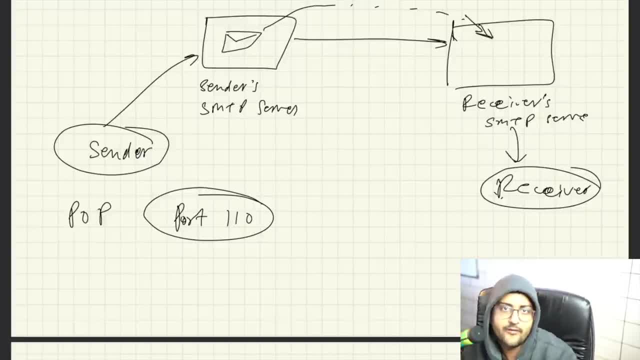 right and then the client asks the servers for all the emails hey give me all my new emails that 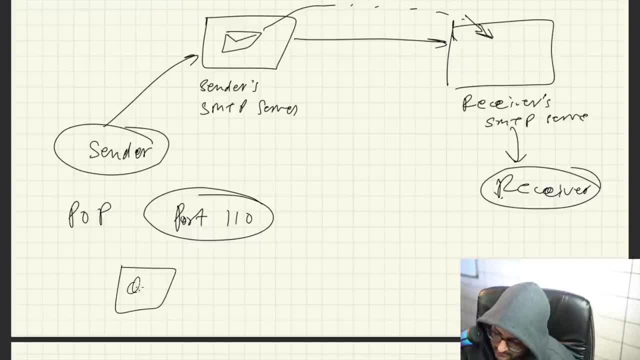 are unread or whatever okay so you have your client you have the pop server 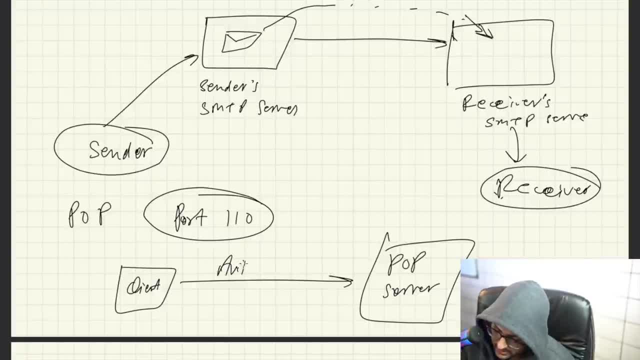 okay you uh authorize it connect and authorize and then you transact all the emails transact all the emails get all the emails okay and after that you can update it 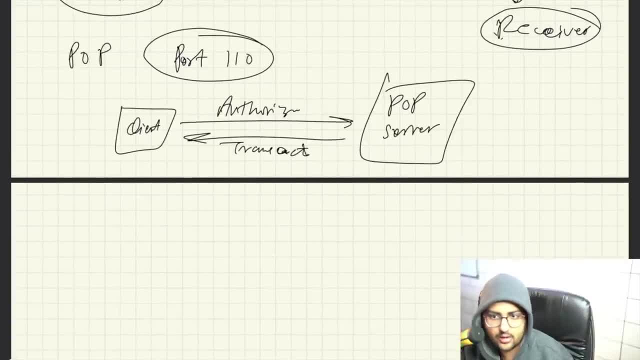 okay so you can close this session and the server will make update on your command right so for example if you uh ask it to delete something it will delete it okay cool 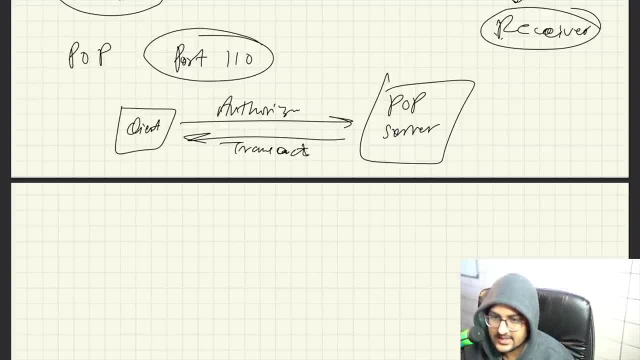 one point i'd like to make is that uh the the other folders like uh sent items and drafts and all these other things these are not synced when we're using this protocol pop okay cool so you can either download the emails and then delete those right from the 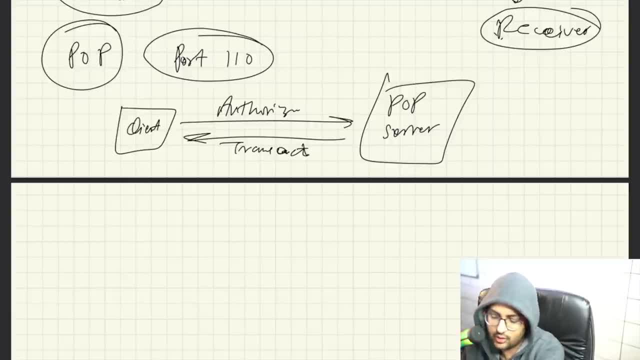 server um or you can download and keep the emails like on the server as well cool notice something if you download the emails and delete all the emails from the server then emails will only be 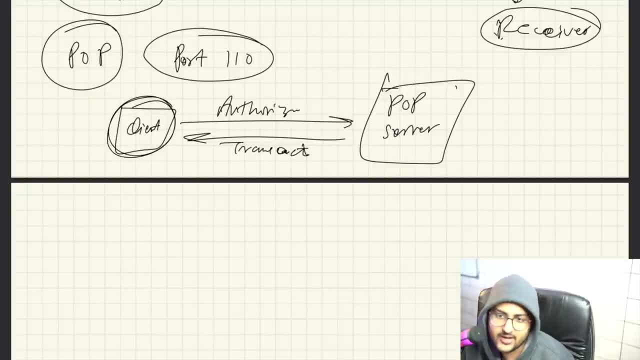 available on this client it will not be available on any new device you use okay the second one is i 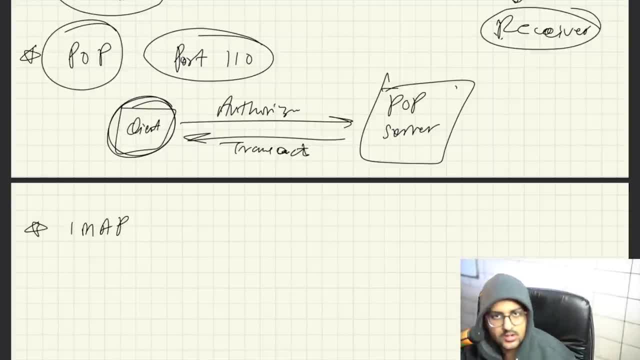 map this is also used to get get your emails it's known as internet message access protocol okay it's a little bit more complex but it allows you to view your emails on multiple devices 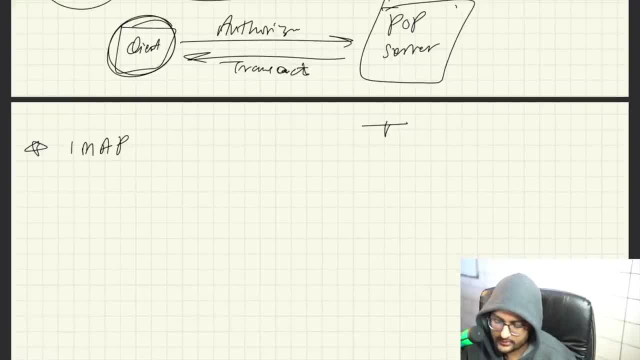 okay so obviously emails will be kept on the server forever and it will not be like deleted unless you delete it you know manually right um local copies will be you know available on various various devices and you can also use the time map so you can see the testing times on multiple devices 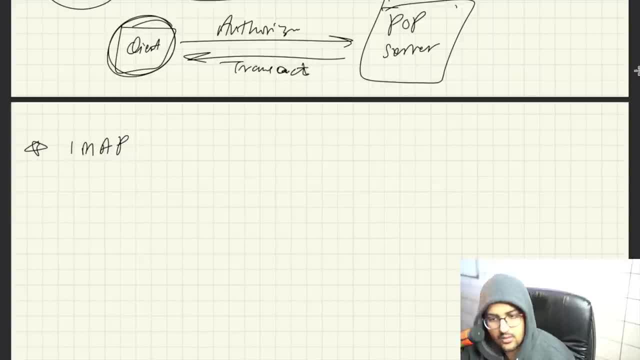 you can sync all your folders as well and all these other things okay so example i use my you know mac os like if i'm using an email on my if i delete an email from my iphone it will be deleted from my mac and my ipad okay sound good so that's basically about how email works you all know about 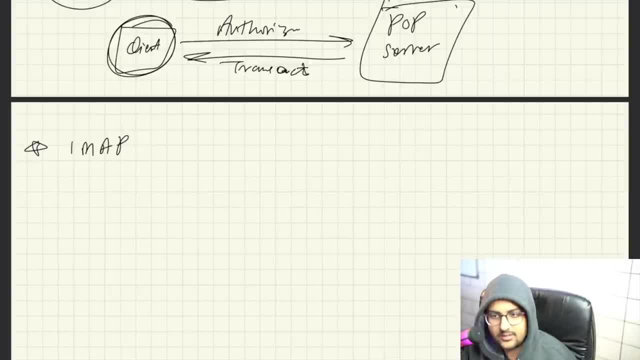 the email stuff like the message and subject and you know headers and bodies and things like that 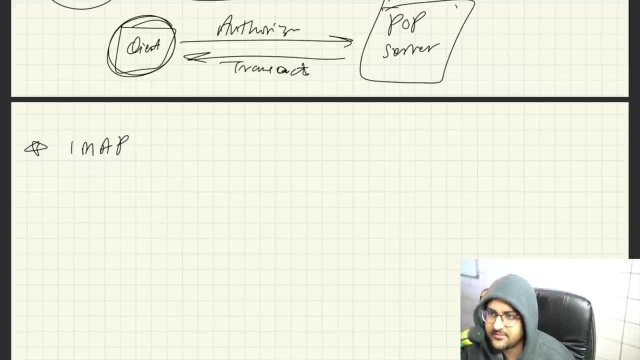 so you all already like know about it so no worries cool so that's basically about it all right uh that was it about emails and uh yeah pretty much about it all right let's move forward 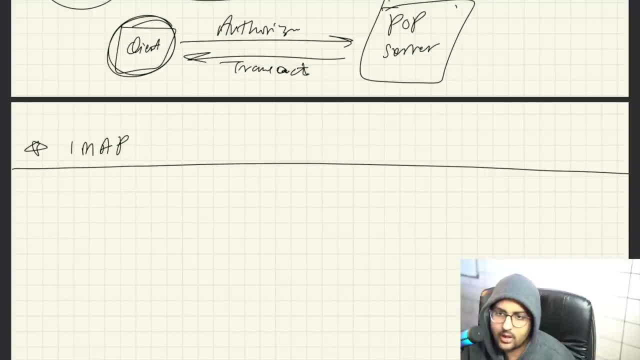 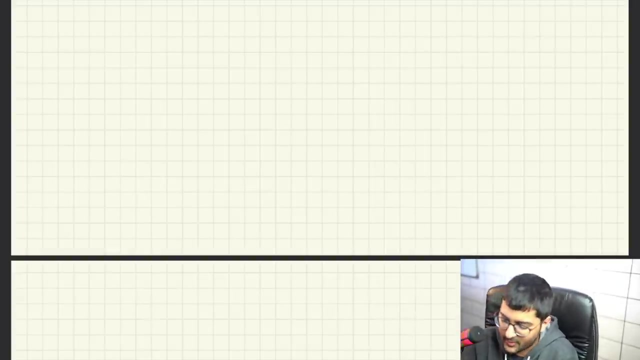 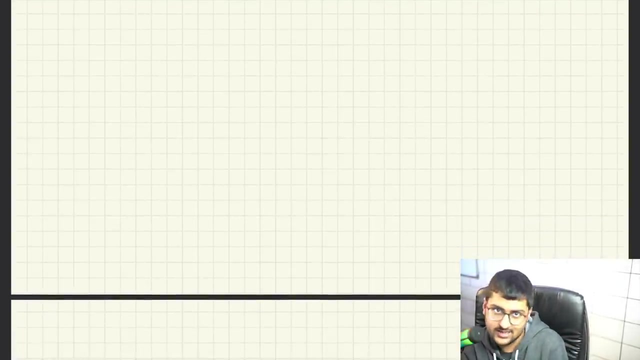 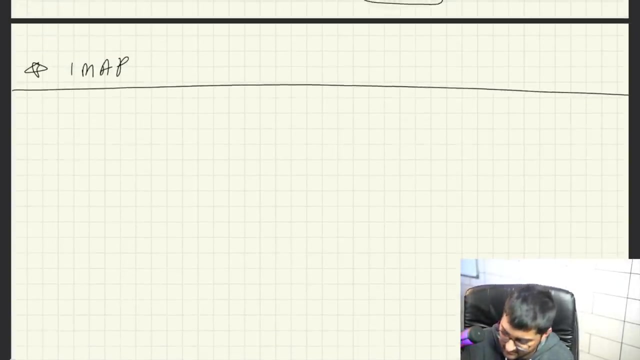 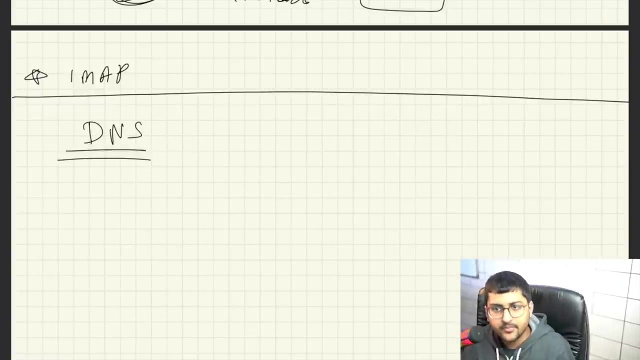 one more thing i want to cover in application layer is uh when we talk about uh ip addresses and uh urls right so we did not talk about that in detail so what is the url what is this dot com dot io dot edu.org domain level names or dns which i was talking about earlier let's talk about that okay now let's talk about we talked about like uh this is an important point now let's talk about like we know that uh when we type when we type www.google.com it connects us with the google server that has some ip address okay so it's sort of like um you know phone in your phone book you have contacts names and every name has a phone number similarly you have like your domain names and every domain name will have like a ip address associated with it okay but now the question is where is this being stored where is this phone book stored and how does it find when you type google.com how does it find that server that is the real question now okay comes into picture dns it's a very very important topic dns okay cool awesome so dns basically means domain name system 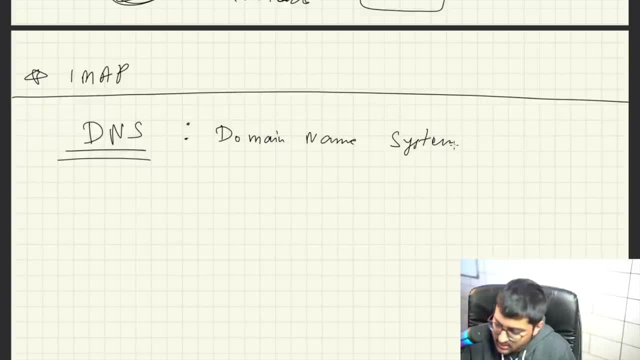 domain name system okay so basically domain names are mapped to ip addresses we know that and uh we use a service uh let's say they're stored in some database or whatever and uh we use a service to look up into these databases the most popular service for this is domain name system dns okay so when you enter google.com uh it will use dns to find the ip address of google's server okay cool okay so you'll be like how how is this a part of application layer how does that work 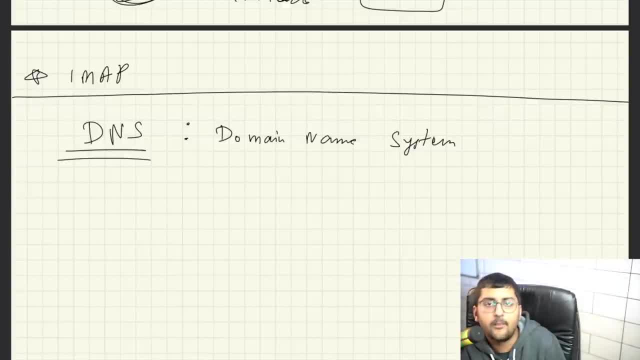 well because you know it's very difficult for us to remember the um you know the ip addressing so that's why we use uh the domain names so what happens is when you type www.google.com http protocol is going to take that domain name it's going to use dns okay domain name system it's going to use that i'll tell you how it uses it but let's see how what it's doing so it's going to use it and it's going to convert that url into the ip address and after that it will connect to the server make sense i've let this go and then um so come back to the library later on if i want to do my work again i just attach it to my booking again after that and then the dns 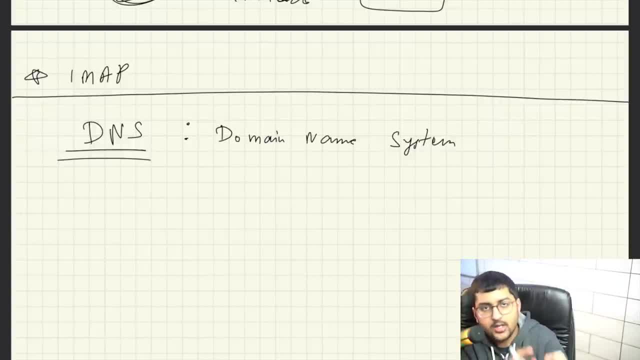 sense type google.com you type in the browser okay http we already covered what http is http will take that url and it will try to find its ip address and once the ip address has been found 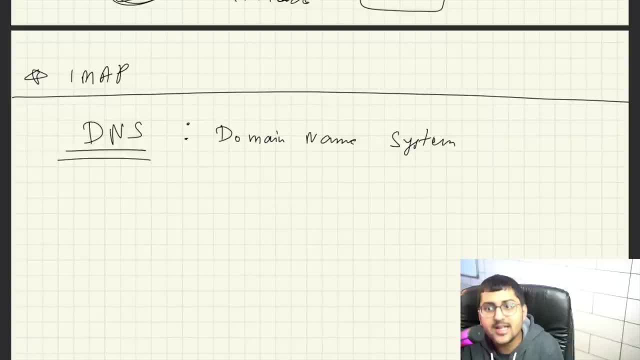 then it will connect to that server so what is dns testing so it's basically a directory a database service example let's say we have some friends in the world who have some big big databases that have a store of all the a record of all these things like okay google's www.google.com has a server name this thing or this thing this is the ip address for that so on and so forth so we ask our friends hey http asks the friends hey you are a dns directory service database can you please tell me i have a google.com can you please give me the uh ip address for it like yeah sure let's look 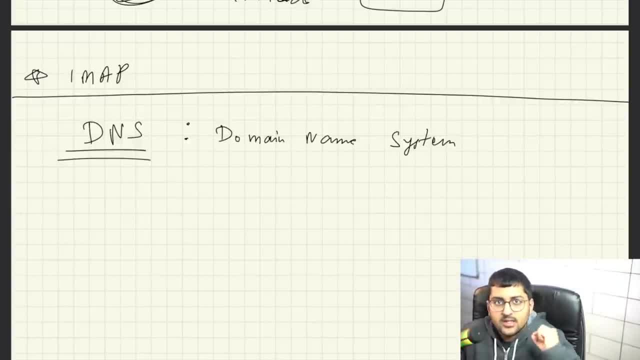 into this in a little bit more detail there are so many urls in the world right there's so many urls if we had just one single database that's not going to be enough for us because where would you put it okay where would we would be located and what if that database goes down you will not be able to resolve any d any any domain name right so and also everyone will be directly trafficking on that database only so these databases are divided into like various classes 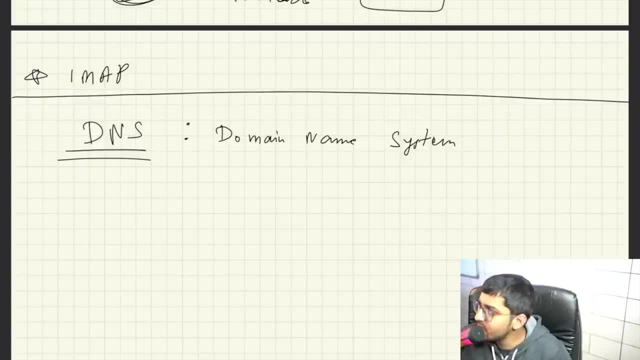 of domains okay let's see what these classes are 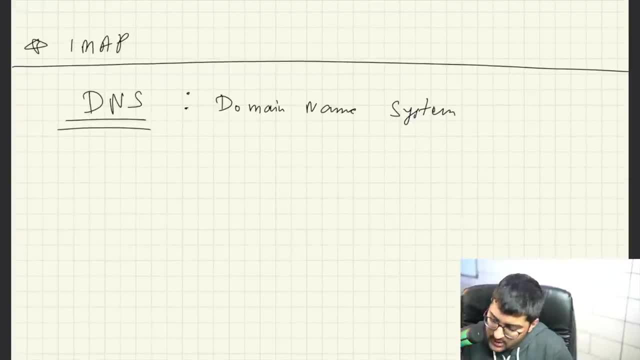 so when you type something like this let's say okay so something you have like let's say mail.google.com or something so you have like a mail service of google.com this is known as the subdomain 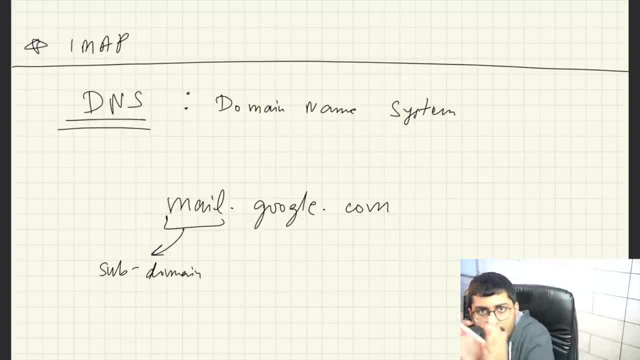 okay what is a subdomain subdomain is basically like a a part of the bigger domain okay google has a mail service so google is the this is the main domain this is the this is known as the second level domain what is this this is the top level domain 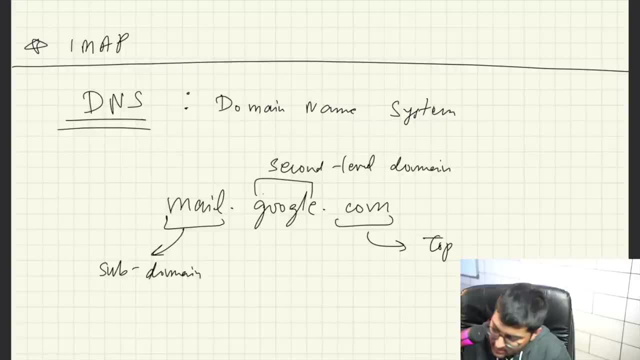 i'll tell you the differences one second this is the top level 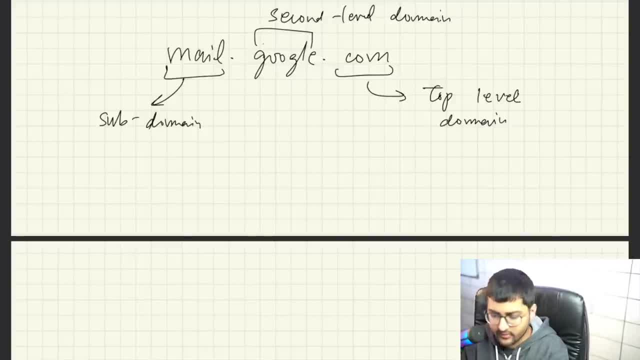 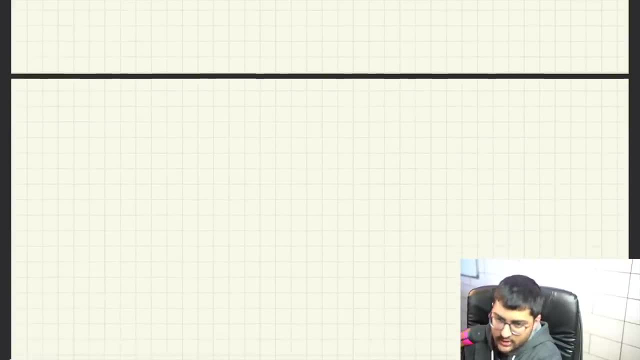 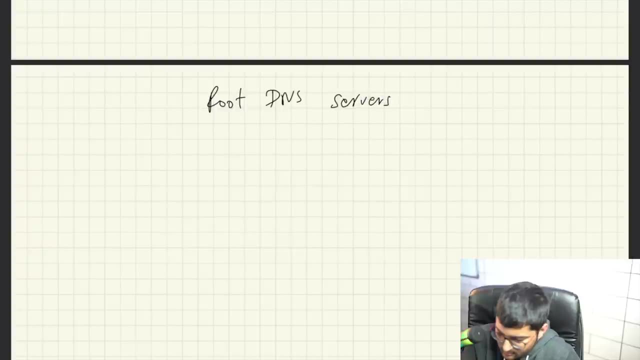 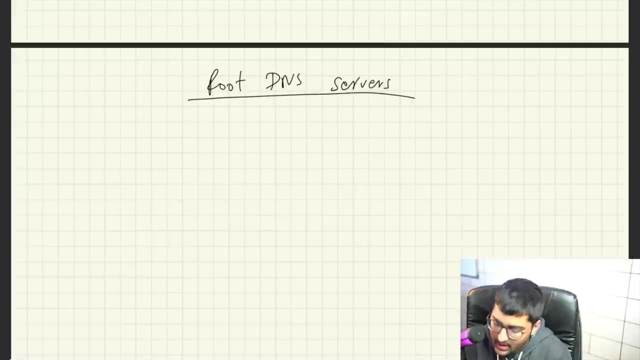 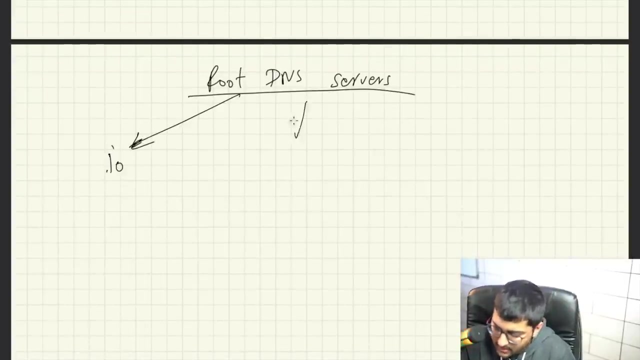 domain okay now let's talk about this so instead of storing everything in one database there are multiple databases for these three categories okay the top ones are known as you're root servers root dns servers okay root dns servers this is like the first point of contact for your query anything like a whenever you write a domain name okay after your local system we'll talk more about that later okay so this is the root dns server they have their top level domains dot io for example dot org for example dot com for example so on and so forth top level domains okay these it's these themselves have something like student.io or com classroom dot org something like that dot com like google.com or something 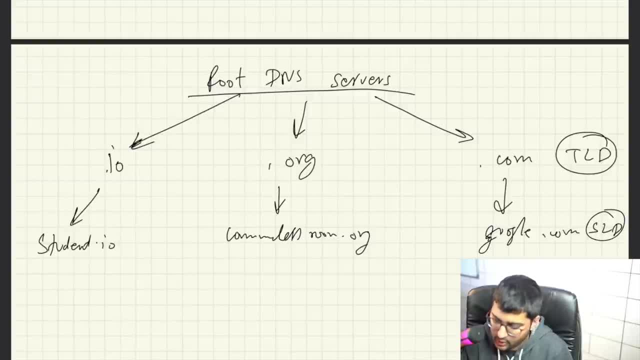 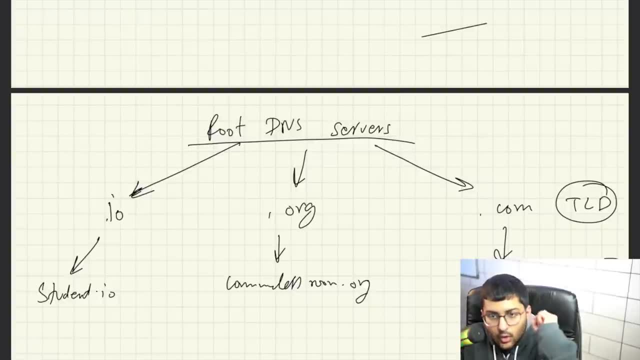 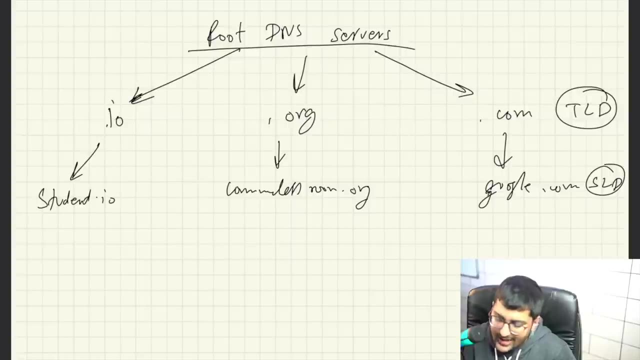 okay so these are second level domains we talked about this over here second level domain 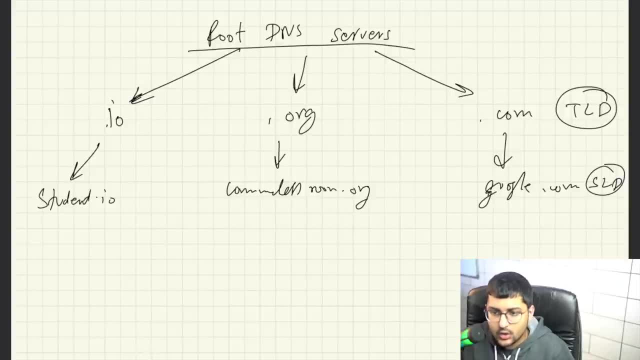 about it so the root dns servers are the main ones the first point of contact so how it actually works let's see let me tell you a little bit more so what happens is that uh when we talk about root dns servers so you can 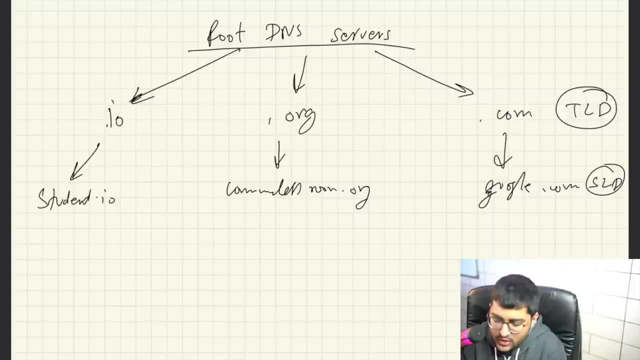 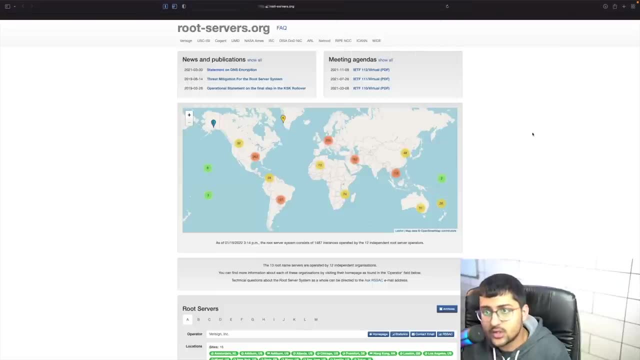 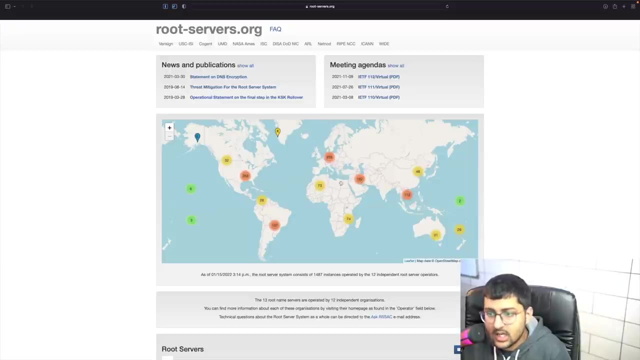 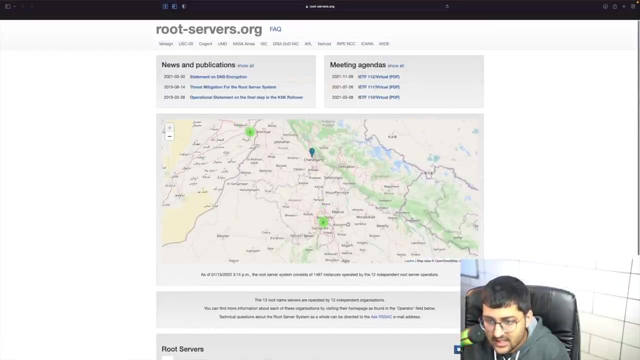 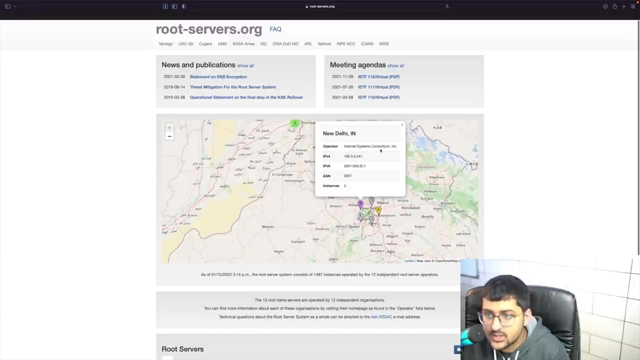 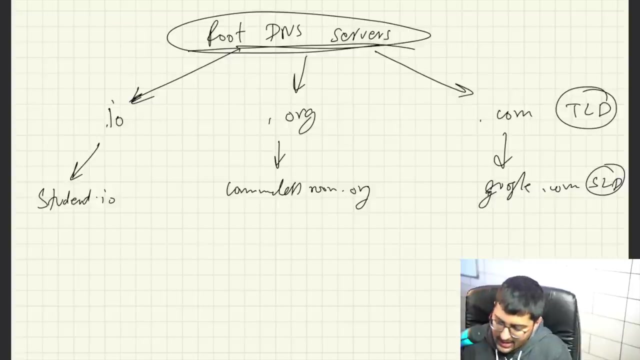 can actually check out all like who is actually maintaining the root dns servers like who is maintaining it we can check that out on this website so you can go to this website root servers.org and here you can see that around 32 are here the you know root dns servers around 162 are somewhere over here around 10 are here and so on and so forth around six are here there's five around new delhi there's one in new delhi it's operated by internet systems consortium for example this is the ipv4 and ipv6 ip addresses by the way we will talk about ipv4 versus ipv6 as well okay number of instances so on and so forth so here are the root dns servers okay and then we can talk about these top level domains like dot com dot org and dot io or whatever companies have their own such uh as well right some companies that have their own uh such such uh domain names right so basically um this one the top level domain okay the top level servers this is basically uh organization type specific so dot com is being used for commercial organizations dot edu for educational institutions dot org for like non-profit organizations for example right but 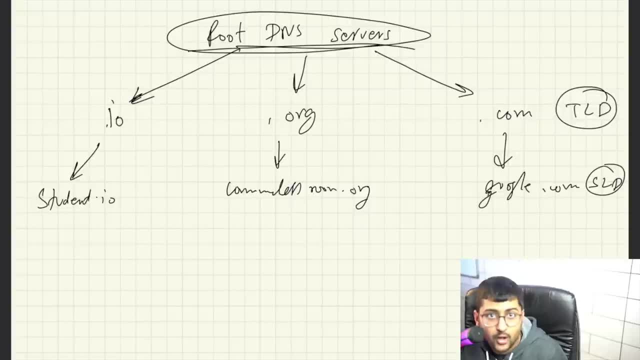 is now open to general use also okay dot uk.us.in are country specific okay so these the database for this is stored like they are uh these are the ones that are managed by i can internet corporation for assigned names and numbers organization i can so you can go to icon.org and once you go to icon.org 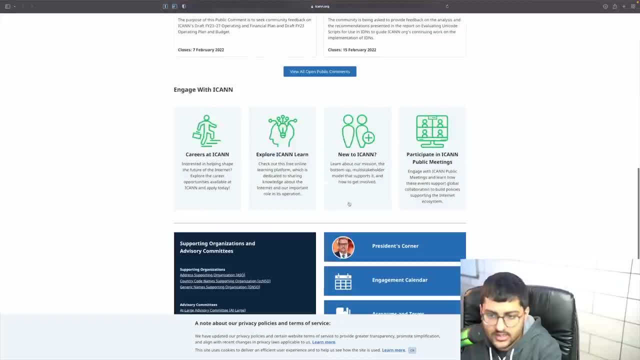 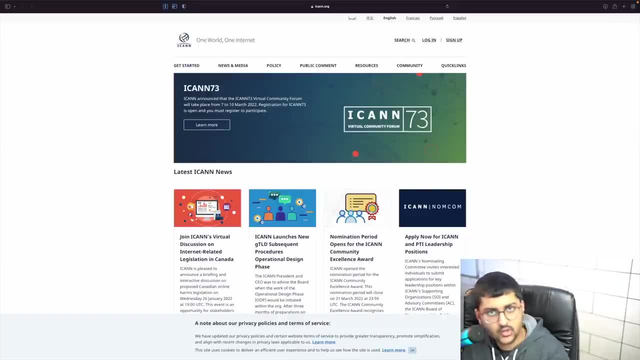 you can see that they are the ones who register all of these uh top levels domains i can so now you know the answer where these are stored i can okay okay so what happens 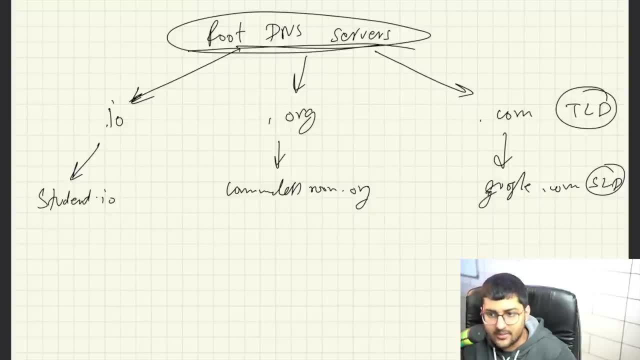 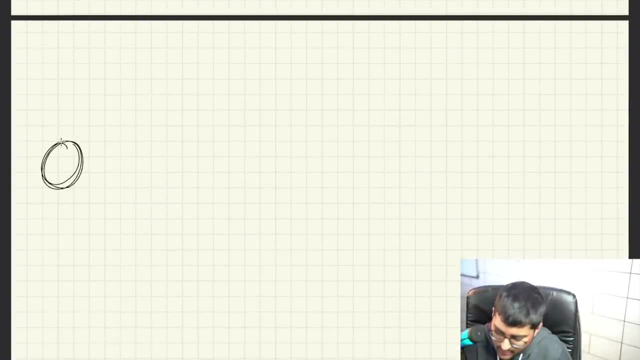 when we uh put google.com in our website okay what will happen let's see when we write google.com this is your computer okay this is your computer you write google.com what will happen so the idea is 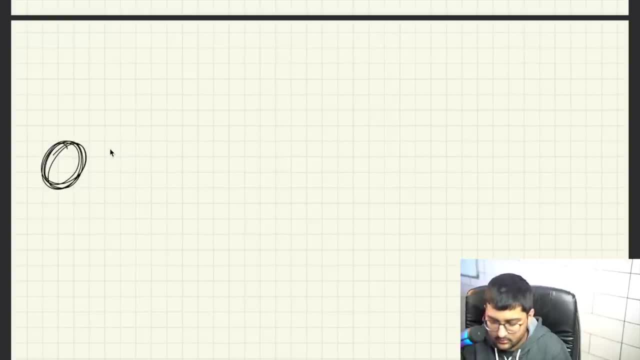 that first it will check in its own computer first i will check in my own computer first it will check computer okay so basically what happens is whenever you visit a website for the first time it will store the value of its IP address that it has found in your 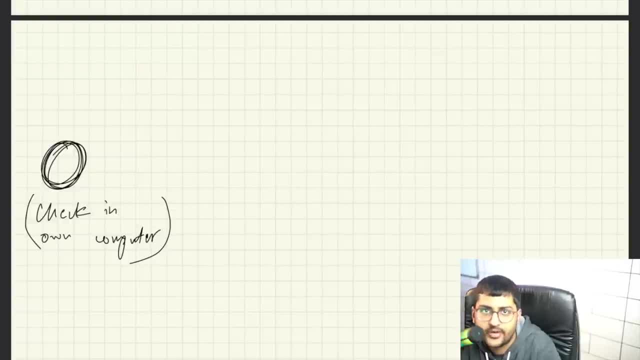 local cache local database on your system from there why because you don't want to search for it again and again you may visit google.com again and again do you want to visit it do you want to search for it in the entire you know globe again and again no imagine you are not able to find it imagine we are not able to find it let's say in the in the local system and what what happens then 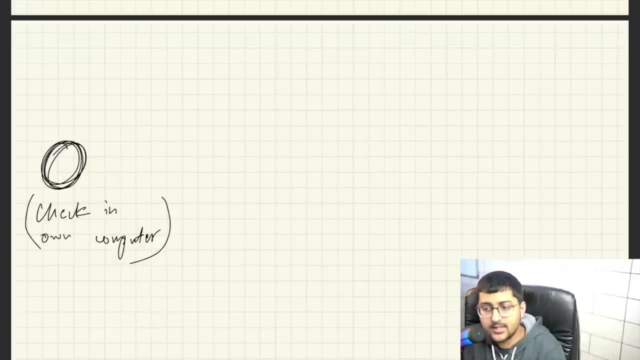 basically it's going to look at in the it not in the local after it's not finding the local cache then in the local DNS server okay so users local 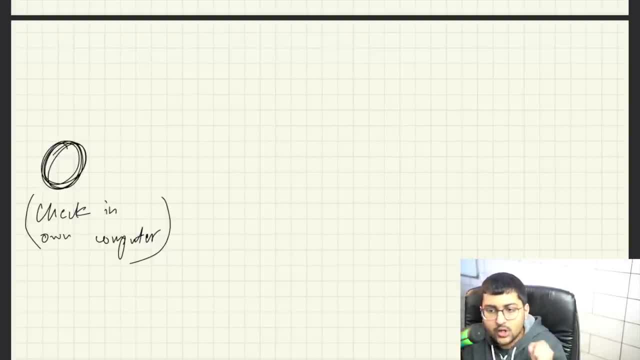 DNS dns server okay so the local dns server is basically uh the first point of contact okay 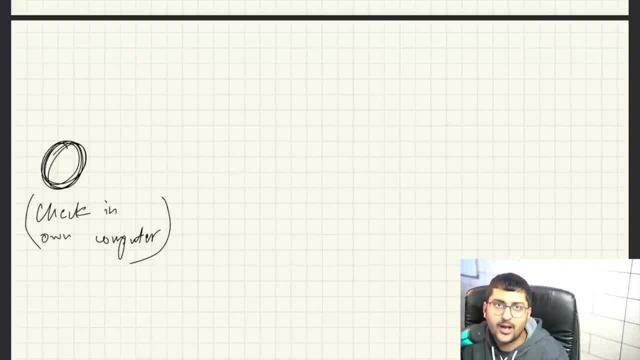 okay so for example many times it's your internet service provider this is one more point so your local dns server your internet service provider for example local server so what happens is one 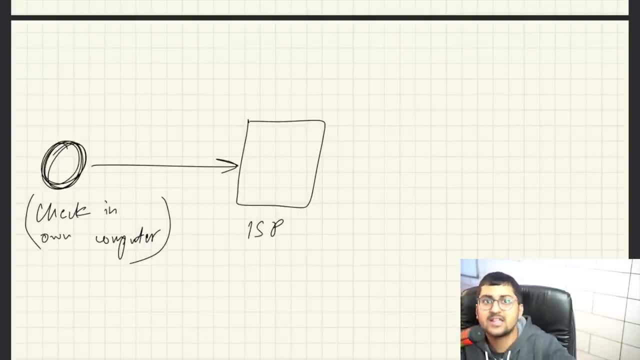 one thing i want to share is your internet service provider actually has information of all the websites you visit it does not matter if you're turning on incognito mode or whatever 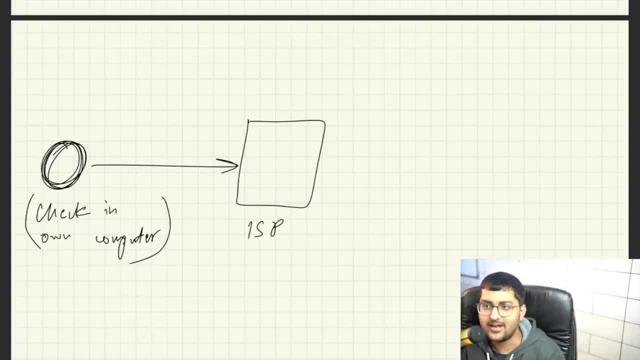 they they know everything okay and if something bad happens then they are liable to tell the police and the government everything okay so next is your local dns server if you are not able to 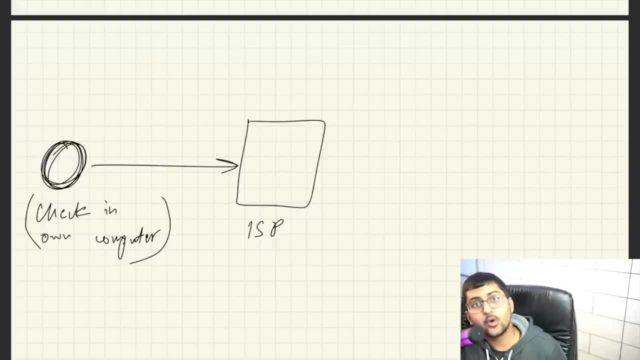 find it over there as well then it is going to check in the root server in the root server like if you're searching for dot com it will search in the root server hey do you have a dot com in the 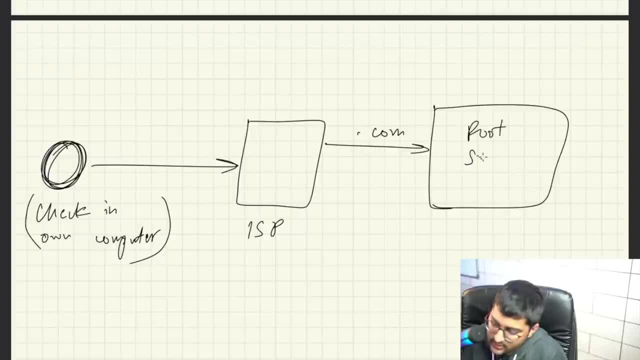 root server somewhere in the root server that we just mentioned okay then root server is going to be like hey i don't have a dot com please ask the top level domain so top level domain is going to be like okay it's 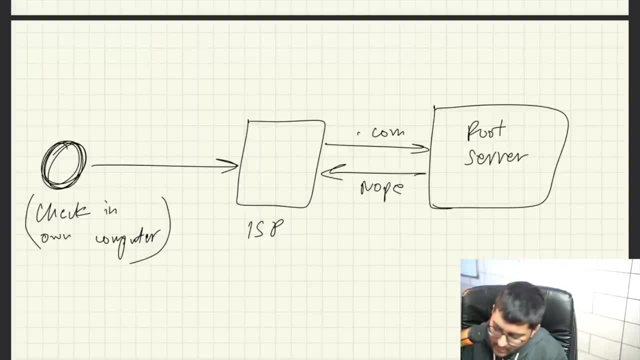 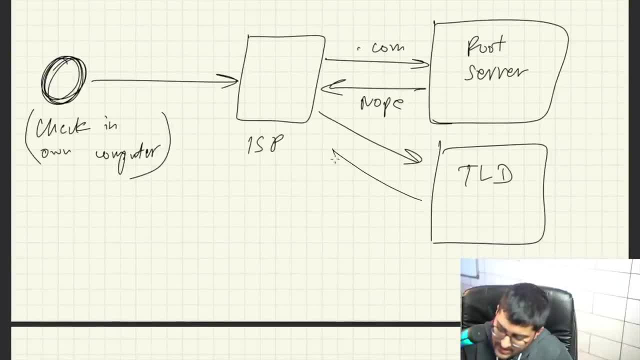 nets and dot org so this will give you the ip address answer it will give you the ip address 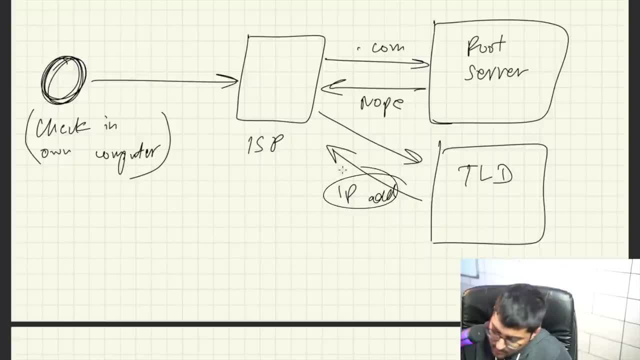 okay sound good and then this will connect to the server of google.com 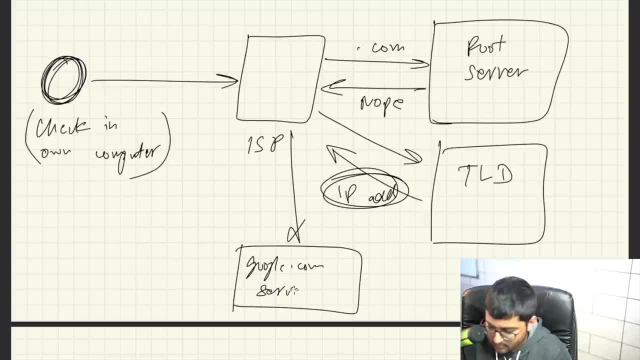 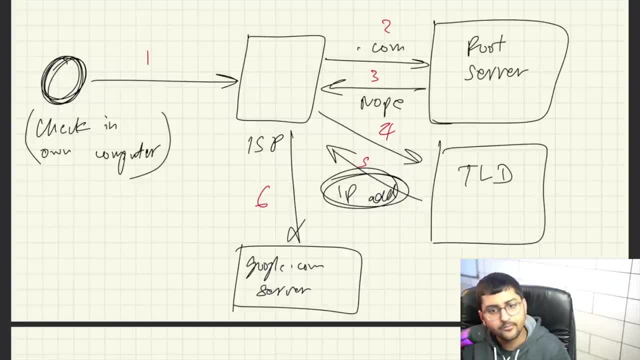 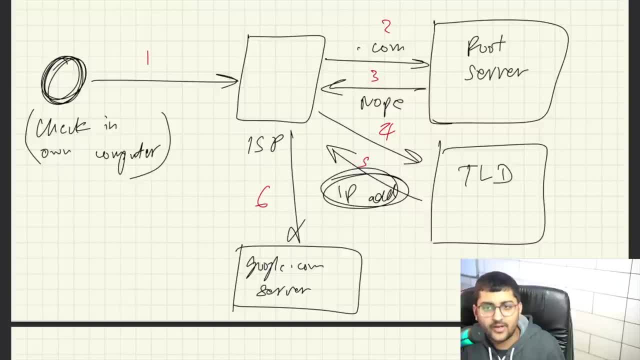 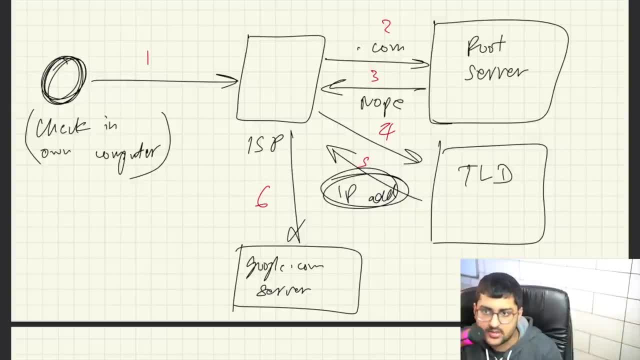 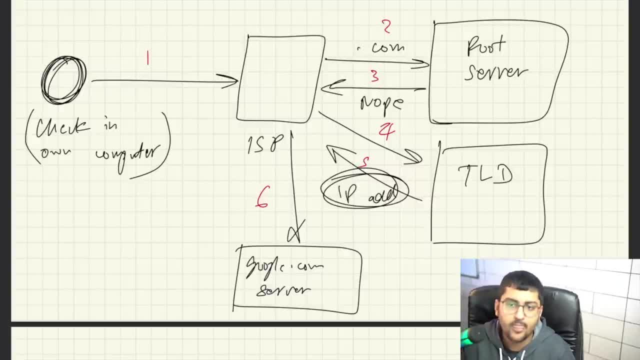 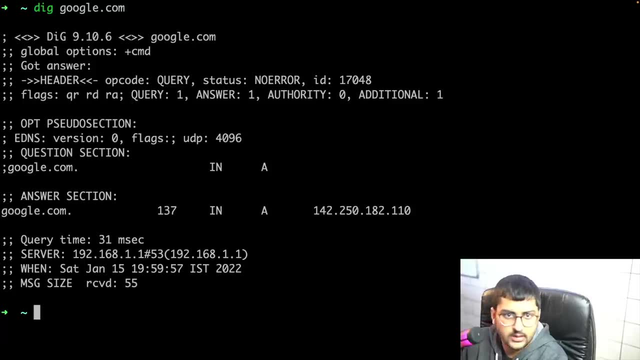 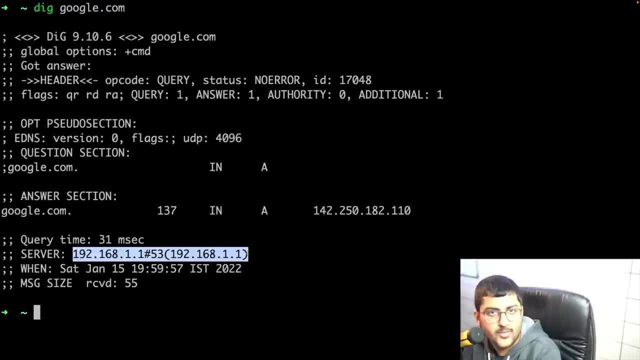 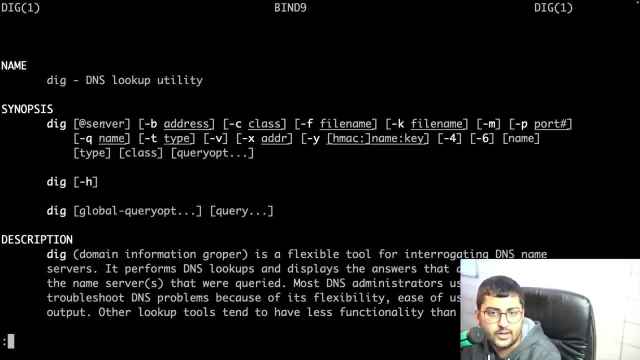 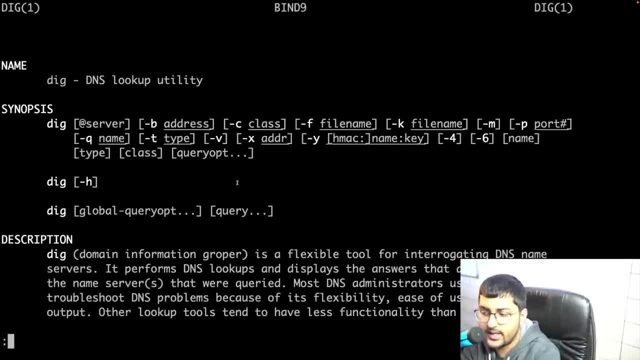 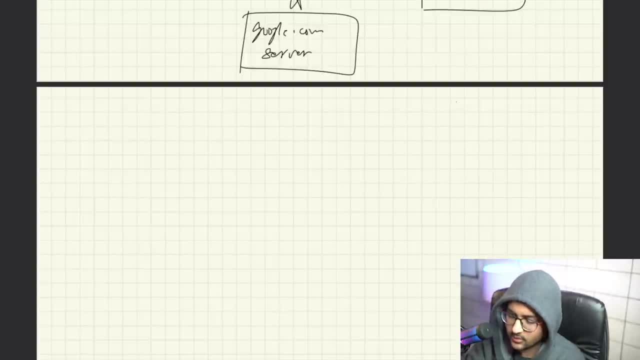 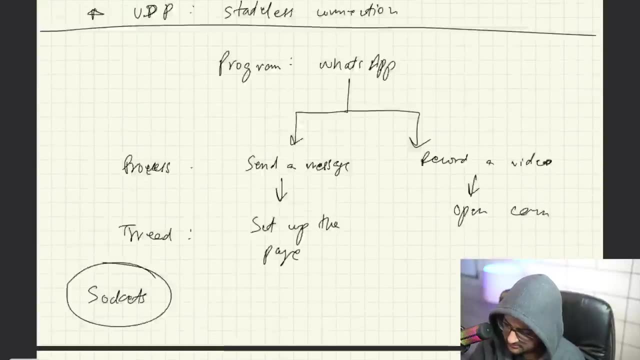 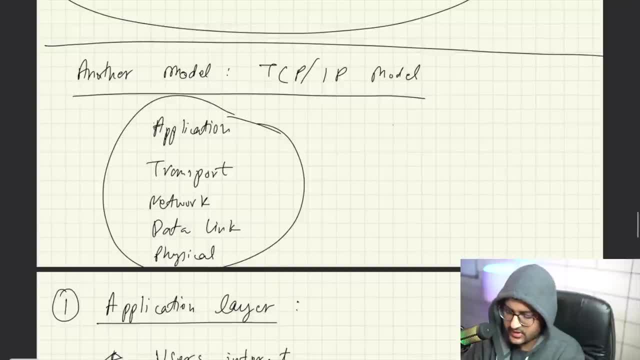 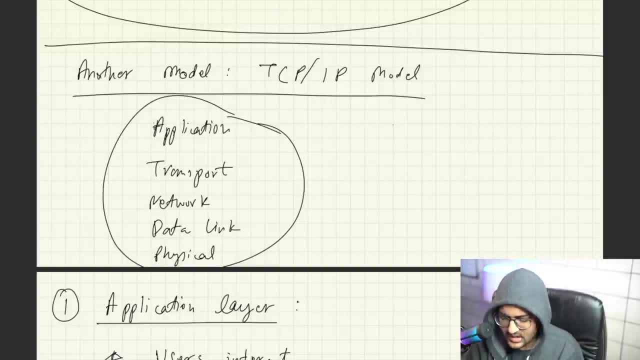 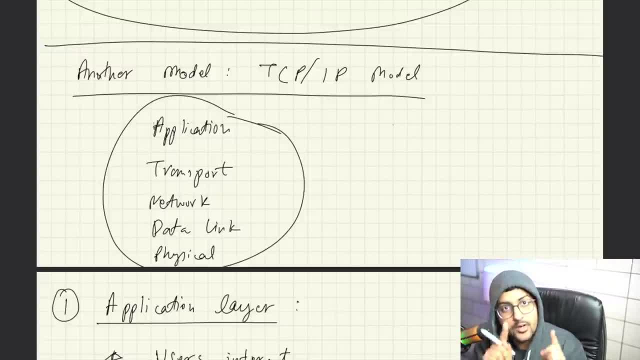 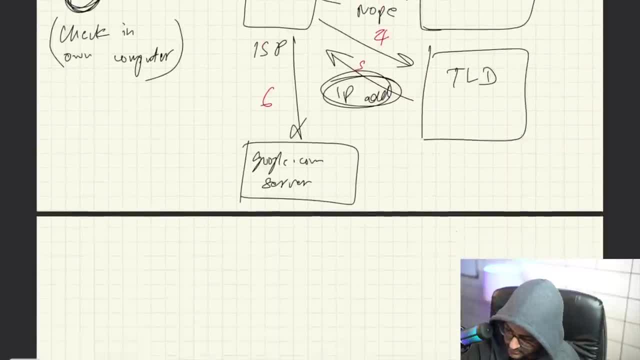 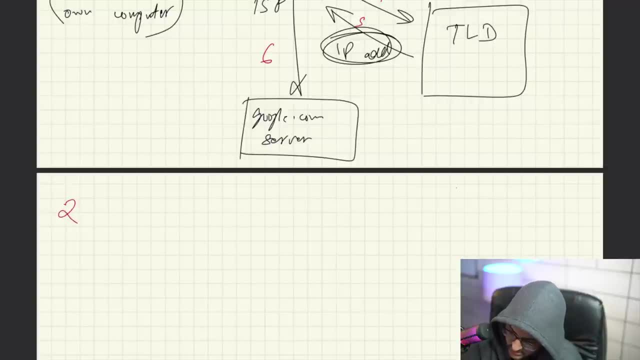 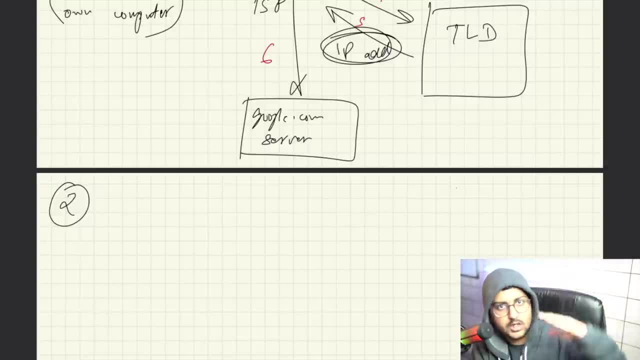 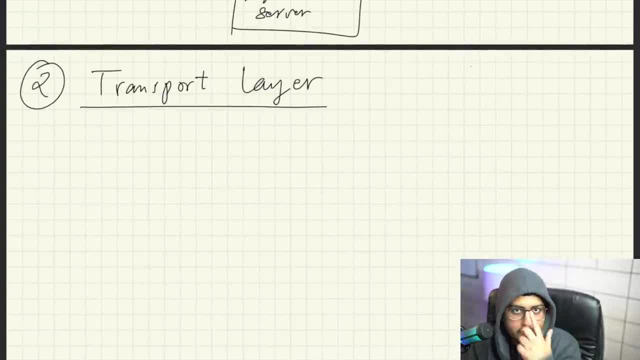 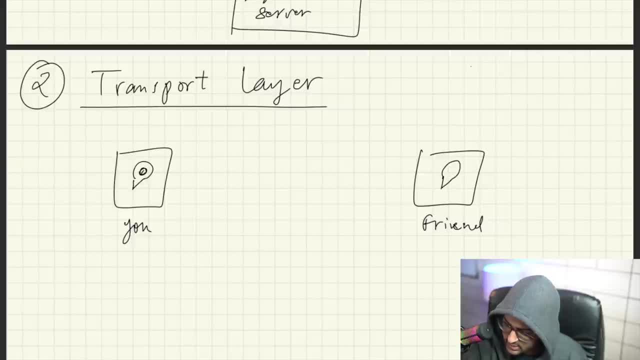 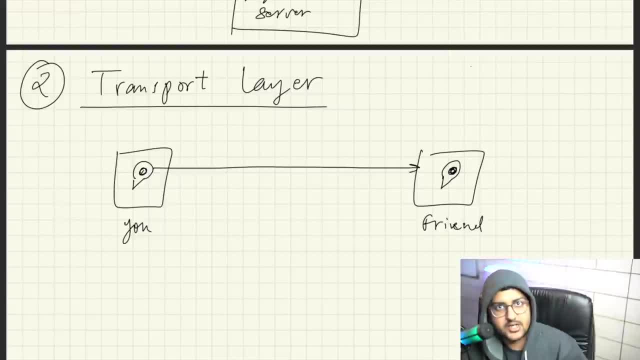 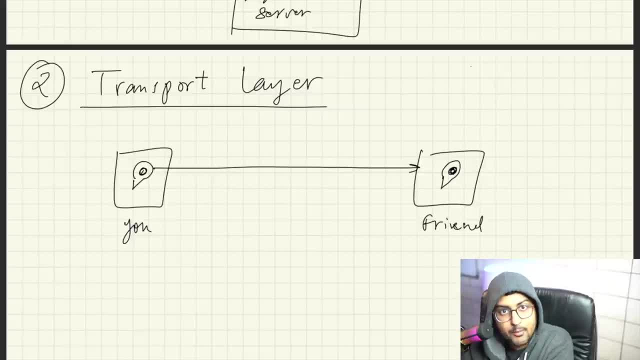 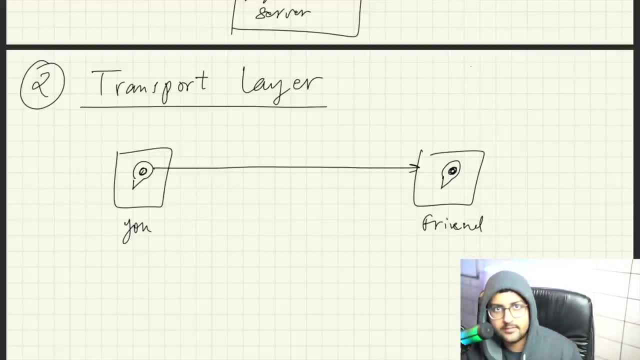 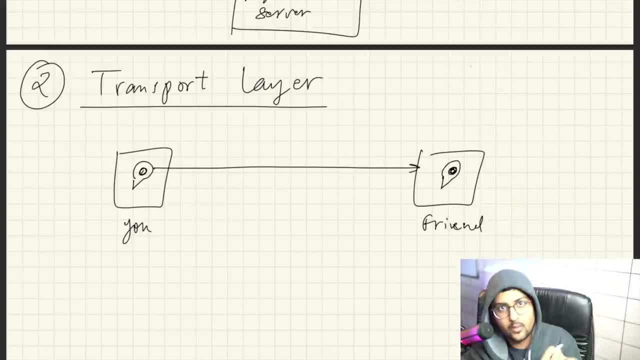 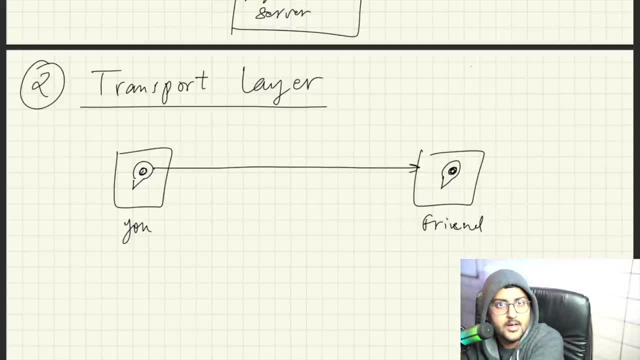 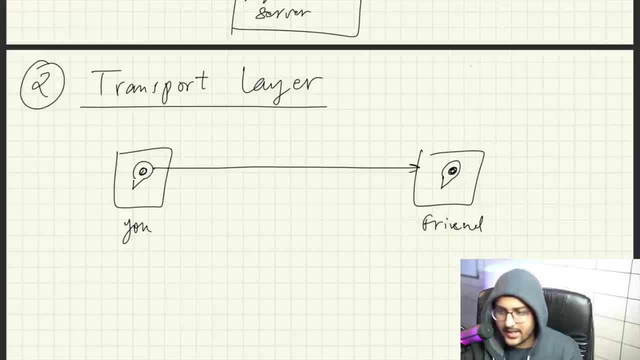 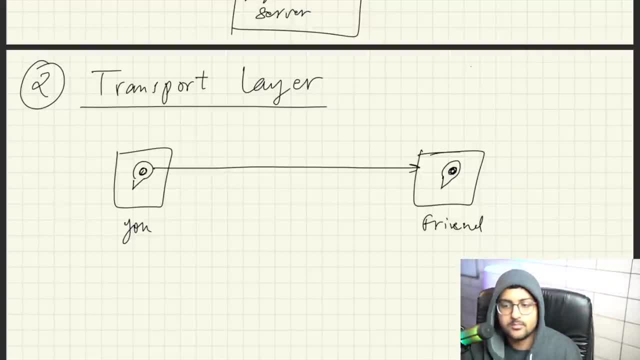 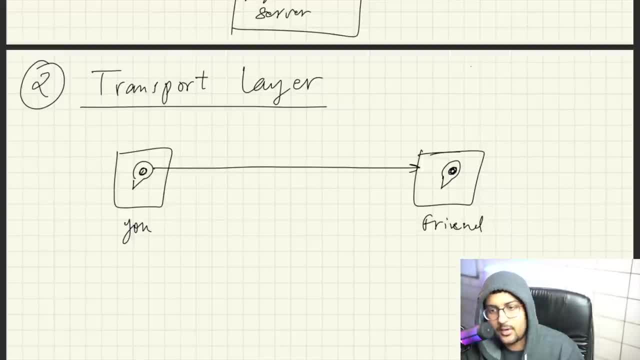 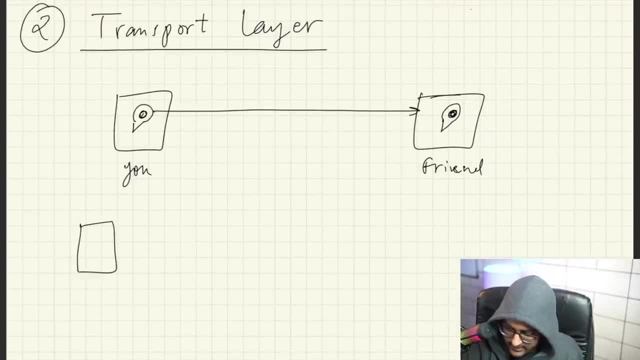 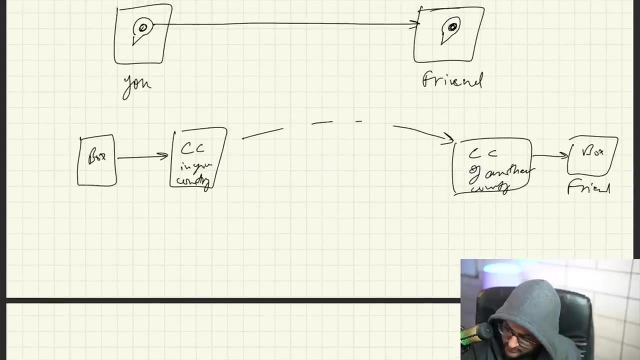 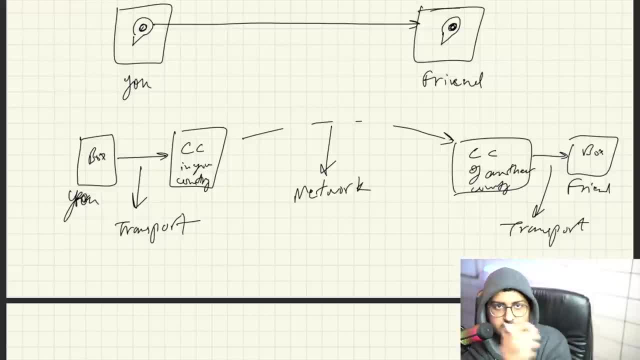 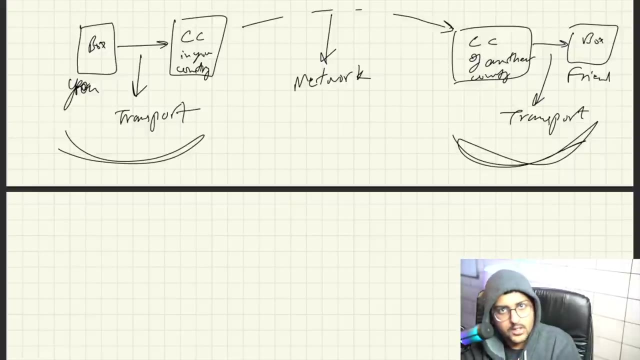 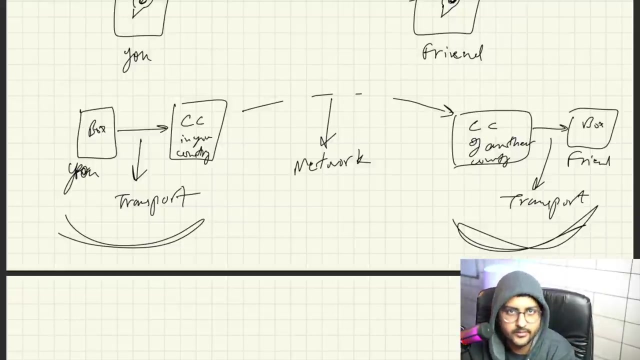 from one device to another device data transferred it uses the network layer but within the same devices okay within this device and within this device that is happening on transport layer okay so transport layer only works with like first it's working on its own application then it trans then it it's basically giving the data to the network layer okay i'm an application i put whatsapp in the message and then that transport layer basically will give it to network 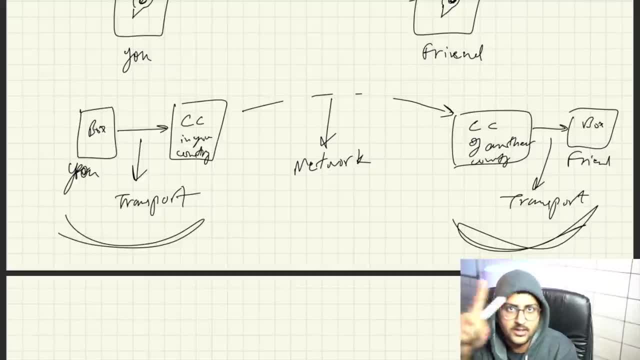 layer like hey this is the message please give it to my friend network layer to network layer will be transferred to your friend's phone and then your friend's phone's network layer will transport the data back to transport layer which in turn will give it back to your whatsapp application 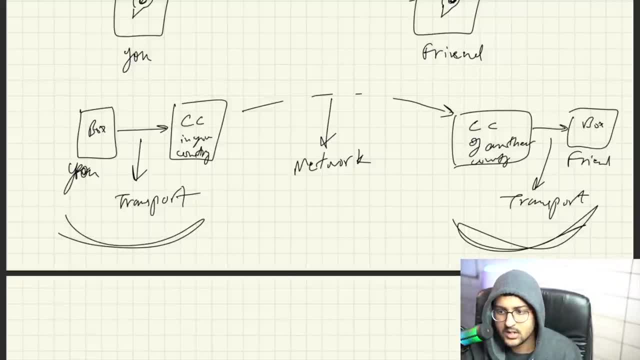 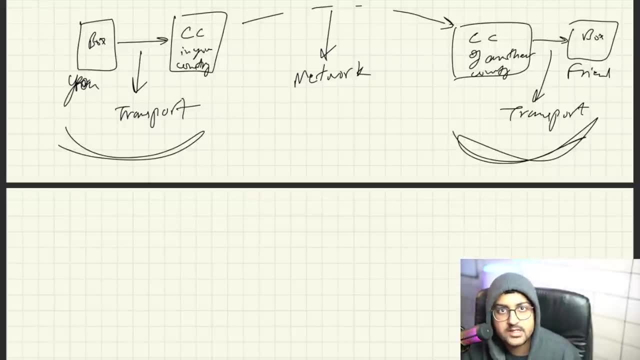 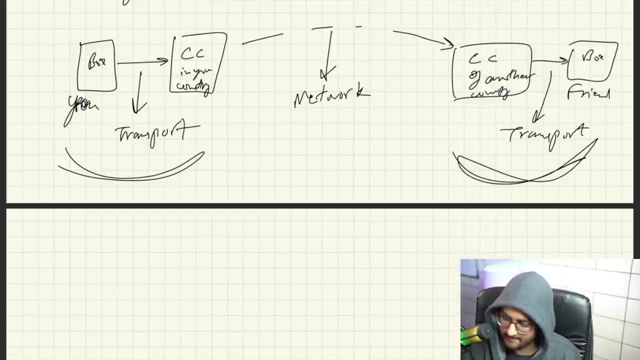 okay so that's basically about it okay now you may ask where is this transport layer you want to visualize this where does it locate where is it located so on your devices right on your end systems computers or whatever that is where transport layer is okay so transport layer has 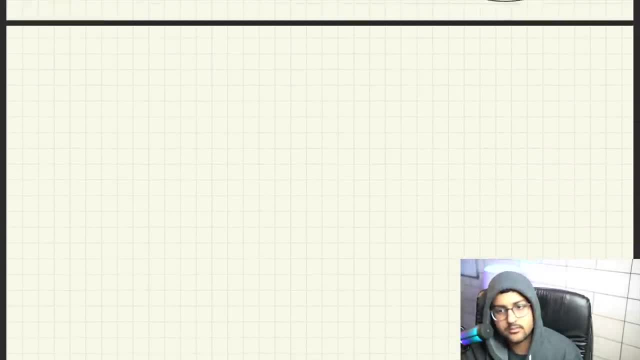 some protocols we've already talked about this we have talked about tcp and udp okay so tcp is basically um you know um it handles uh 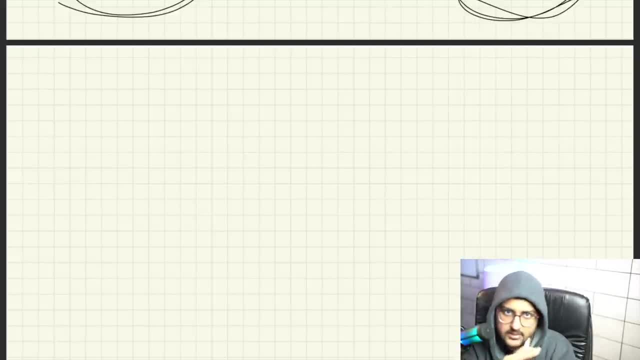 like a hundred percent of like data can be sent like if something is missing if some data is like if you want like entire data to be sent we talked about what tcp is already um and in the order the 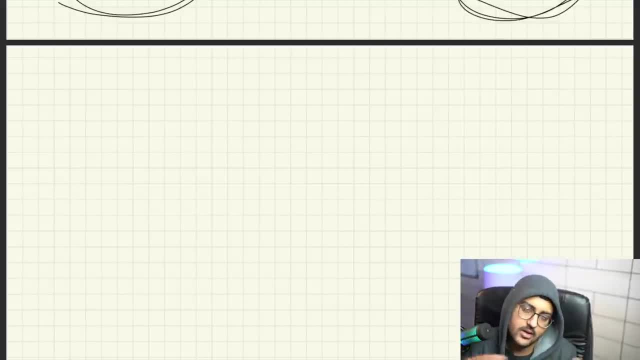 data will be sent and everything in udp that's not the case data data that is being sent may not be in order some data packets will be lost things like that okay so let's look into what tcp is and 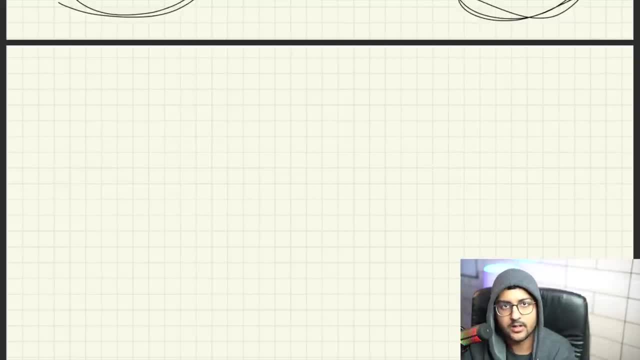 what udp is okay so these are some of the use cases of the transport layer so for example if one application to another application if they're even across the world and stuff so you can visualize it in terms of transport layer you can make sure like your entire data is being sent 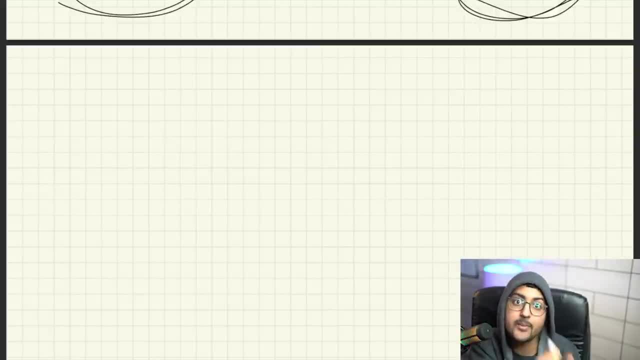 it also you know divides the data into like when we talked about previously segments right so we'll be looking into what segments are and how this data is being transferred we'll look into what is tcpip and how does it make sure so basically if you're sending to your friend15 files in different applications so network layer will send some different files to your friend15 files in different applications so network layer will send those 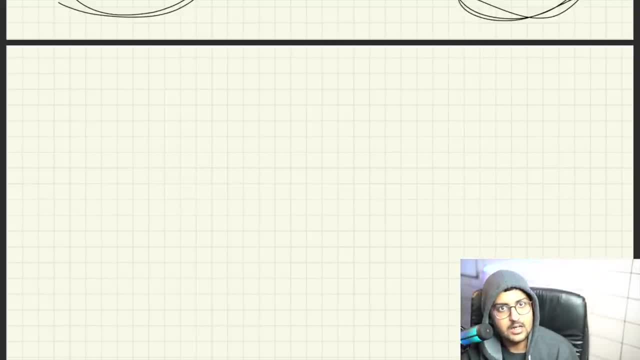 to the исp files but those different different files need to be sent to which particular application of your 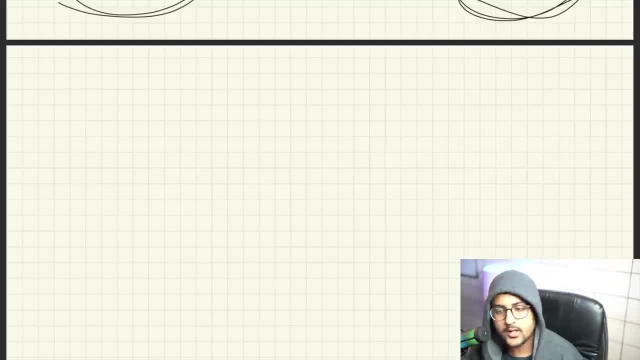 friend right that depends on transport layer okay now let's talk about how this thing happens kunal we're talking about end systems we're talking about devices you are telling us that the role of transport layer is to basically take the data like whatever you receive from network to 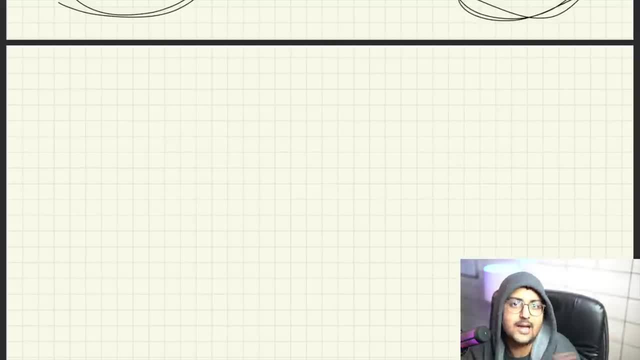 applications and from applications to network okay on the end system only how it travels on the air from one country to another that will be looking into network layer but in in transport layer what 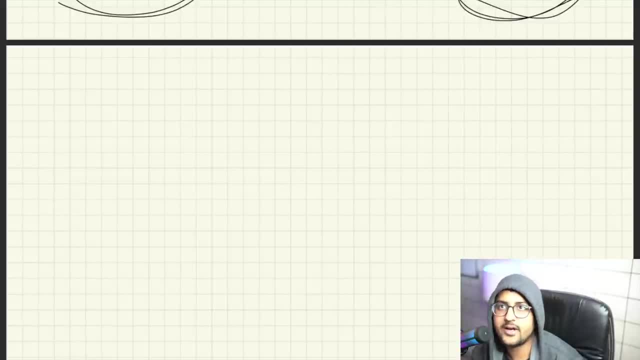 is happening that let's say you are sending your friend like a file over whatsapp and your video conferencing them on skype and you're sending them an email also okay so you're sending your 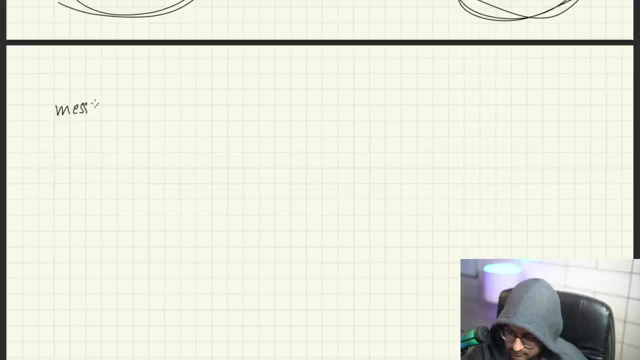 friend like there's a message okay there's a mail and there's a video call three things are happening with your friends in the same time this is all happening on your system 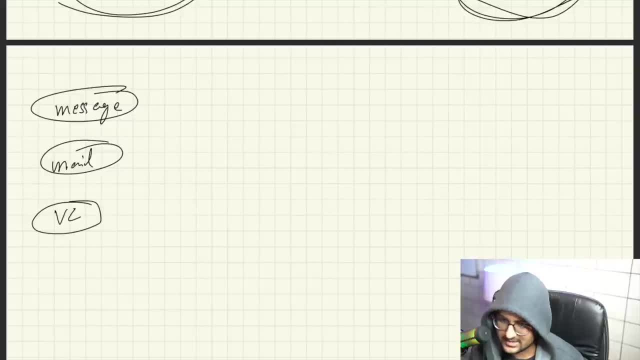 okay okay this is all happening on your system now for your friend they also need to receive a message 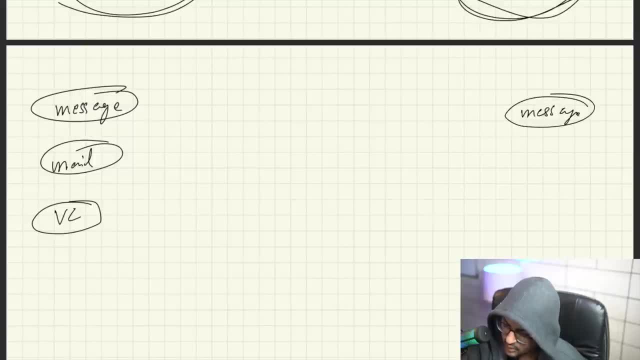 on their whatsapp or whatever okay they need to receive an email or something or whatever like whatever you want to call it or a online file or something okay i can just call it a file 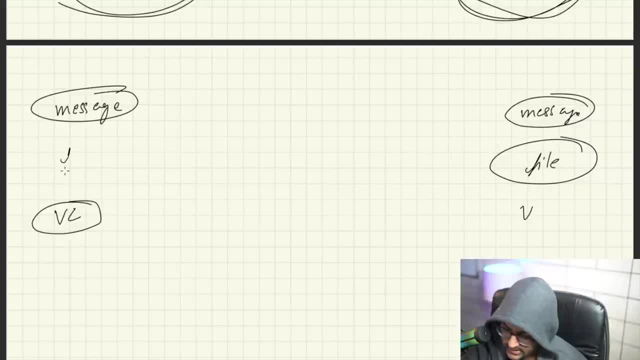 you're sending a file let's say for example okay you're sending a file for example and you're video calling them as well so all of this data i know will be traveled through 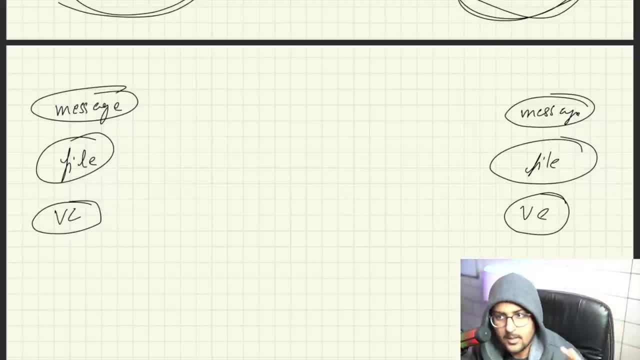 internet how it travels on the internet that we'll look into later on but first let's focus on how you know our computers will determine that which type of how to send these three types of data 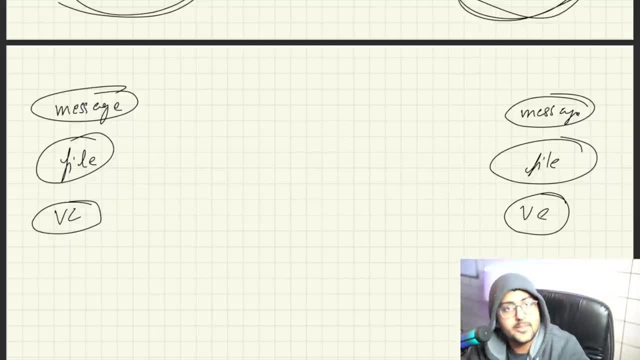 to the network and how will our friend determine like when the network of even your friend's device 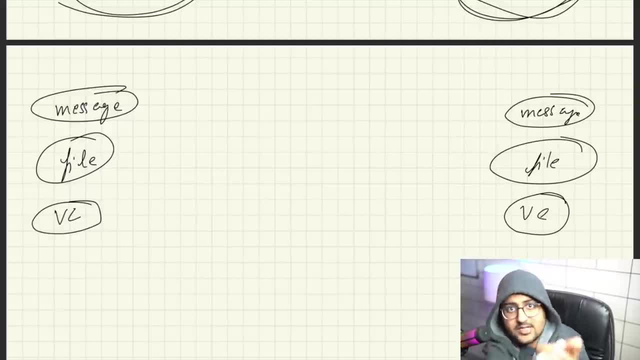 has gotten the data how will that determine which application to send which data we are sending data in a bundle right okay 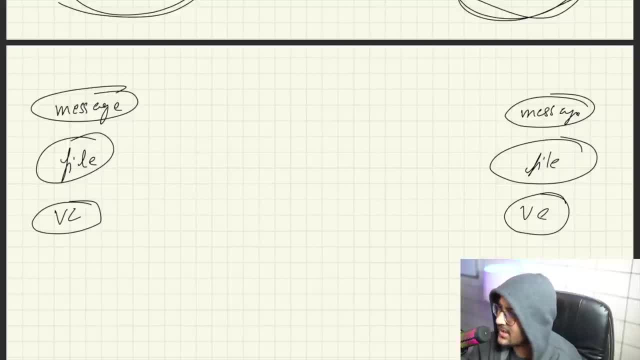 so this thing is known as multiplexing and this thing is known as de-multiplexing so multiplexing is what multiplexing will allow us to send all these messages and things to a lot of destinations so three messages we are sending to three three applications three destinations just via one medium okay for example you put something in a box you you are sending your friend uh cookies and a playstation and a mobile phone you put this in a box and you give your friend a box okay so transport layer has a multiplexer 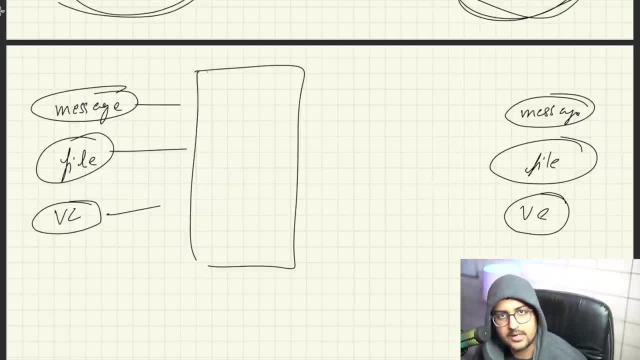 you're sending all these three items in the multiplexer transport layer multiplex okay 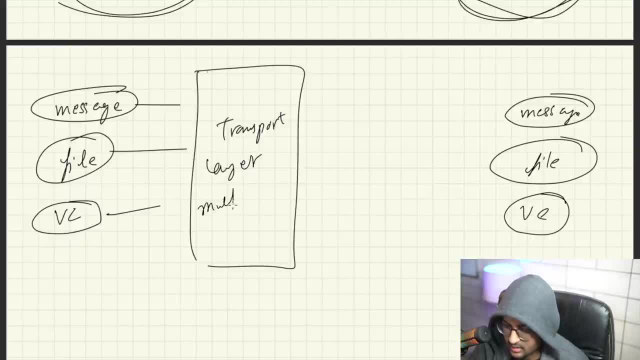 transport layer multiplex and this will pass it to the d multiplexer so one is multiplexer and one is d multiplexer 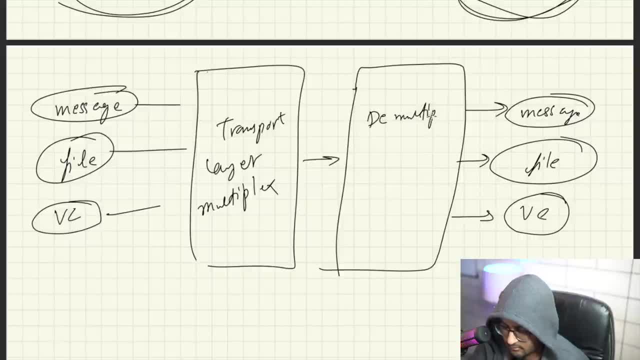 so d multiplex is just opposite of multiplex obviously okay so applications will be sent to like here you have the d multiplexer and basically it will pass it to whatsapp and your browser and your video call skype or whatever okay so this is multiplexing this is demultiplexing 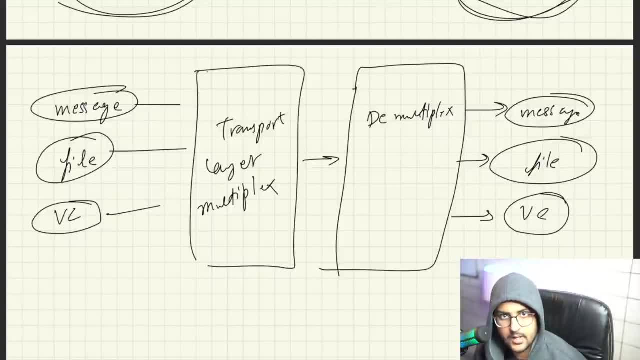 as simple as that okay but how does it work internally how does it happen what is it that we use to refer to applications tell me that what is it that we use to refer applications what is it we use to refer machines ip addresses and what is it that 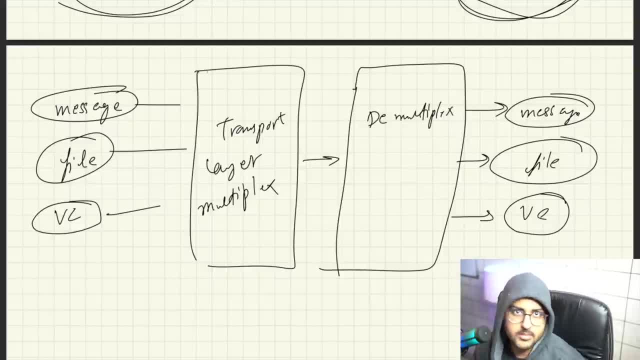 we used to refer applications i covered this already port numbers okay we also covered about 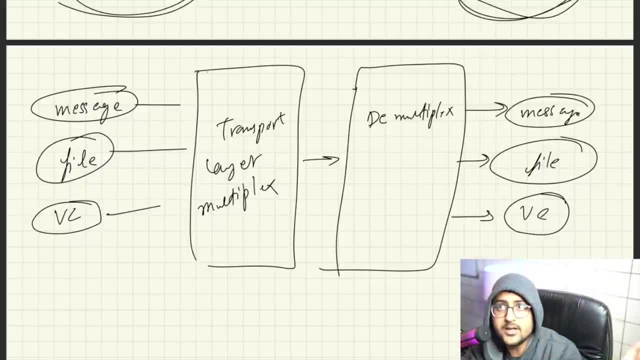 sockets what are sockets sockets are just like some some sort of like a connection between two applications like a gateway okay between the application and the many application 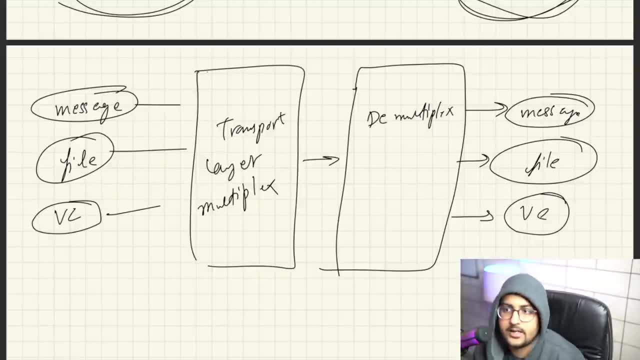 the what network that's how applications are connected okay so if this message application wants to send something to another message application it will give it to the socket it will give it to the socket over here this will give it to sockets this will also have sockets over here and these sockets have port numbers okay so you all know that these things 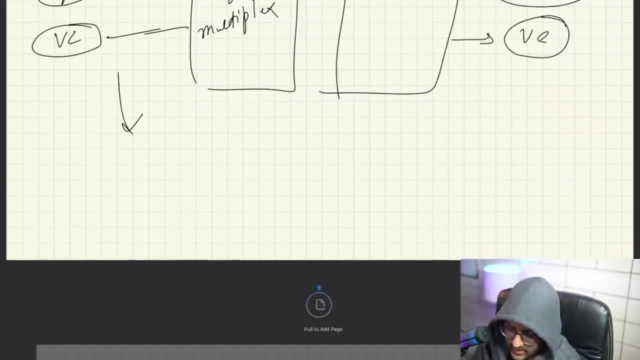 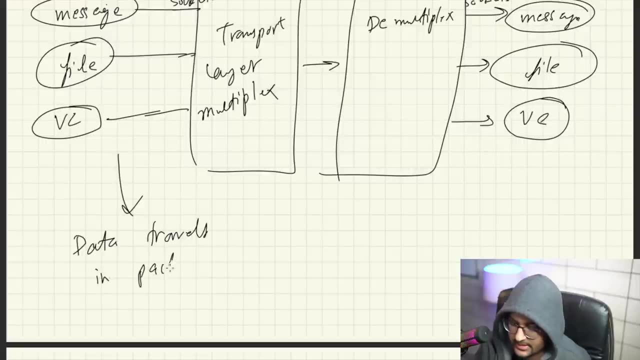 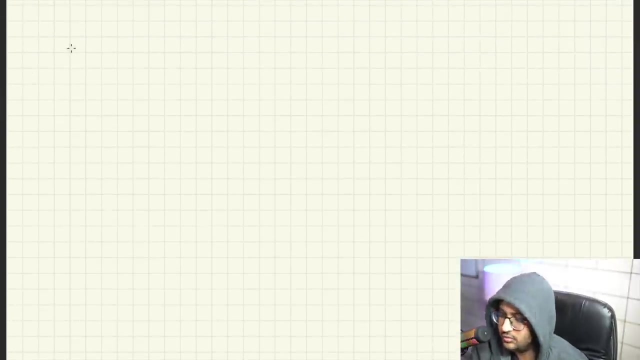 are traveling in packets data travels in packets we all know that we have covered this previously okay so data travels in packets we know that okay so the transport layer will attach transport layer will attach these port numbers these socket port numbers that's why it knows where the application is coming from and to which application do we need to send the data okay cool okay 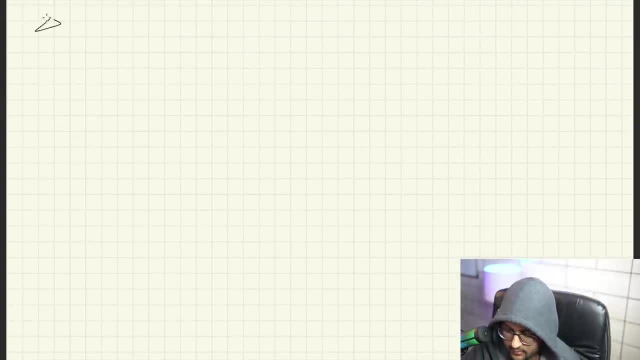 and there's one more thing transport layer another point i want to add over here is that transport layer also also 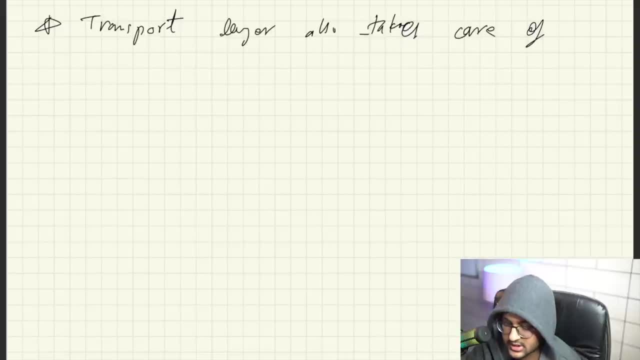 also takes care of congestion control congestion control congestion is what congestion is traffic you know when so many cars align or something and so many people are there and the the space is limited the entry is limited but so many people are trying to get in then there's like a lot of congestion so that's basically what it means so in transport layer condition happens in like network layer also in transport layer also for example network uh has a lower bandwidth but you are sending data packets so rapidly some packets will get lost and stuff this is known as congestion okay so basically it will try to like uh send that packets at like a slower rate and things like that it's going to take note of all these other things okay sound good so it uses some algorithms for it you can check it out congestion control algorithms since we're talking about transport layer so this will be built into which which protocol transport layer protocol like tcp and udp 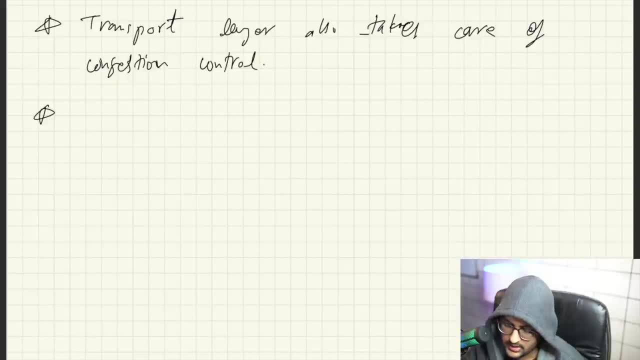 you can check it out congestion control algorithms since we talked about transport layer so this and UDP so here it's saying that congestion control algorithms built in 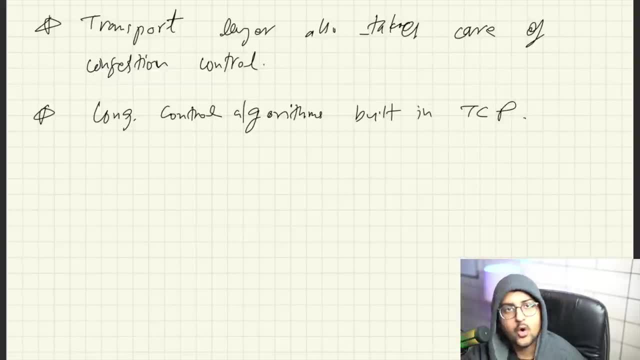 TCP okay cool okay let's move forward now we all have a good understanding of transport layer now okay you send the data to network layer and in your 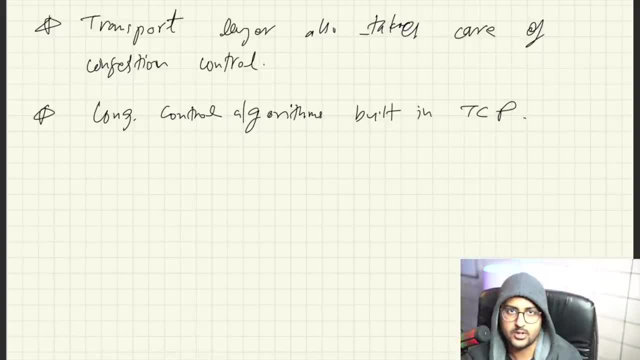 friend's house network layer will send the data to transport layer so transport layer to network layer and then the data travels through the world then network layer to transport layer gave a very nice understanding to you okay let's 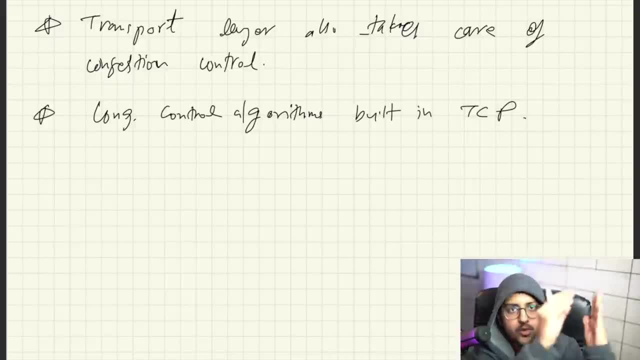 think about your friend let's think about your friend you are sending this data from network layer to network layer sometimes it may be possible the data gets corrupted in between may be possible nothing is perfect right we all 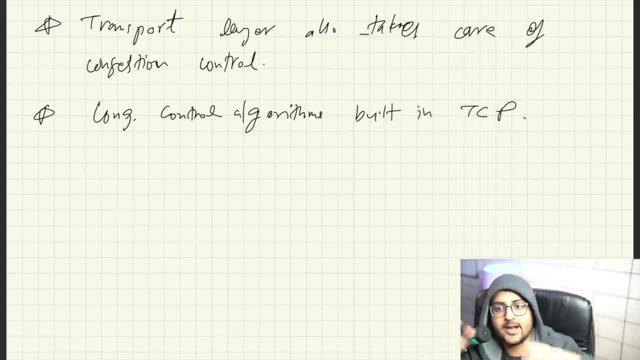 have flaws so sometimes it may be happen like get data gets corrupted you are sending data into what you're sending data in segments we have looked we have looked at this term called segments before right so it says data 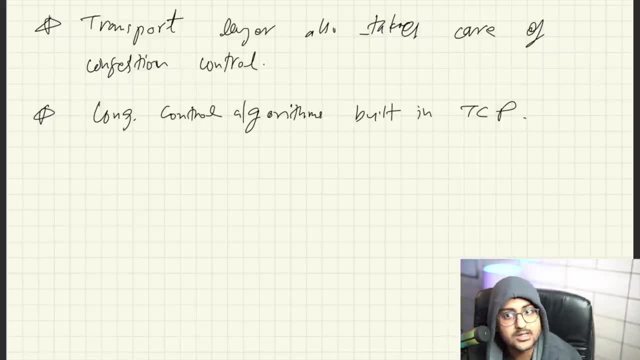 packets for example okay so these bit data packets can be lost for example right or something like you're sending some files and you're sending a file 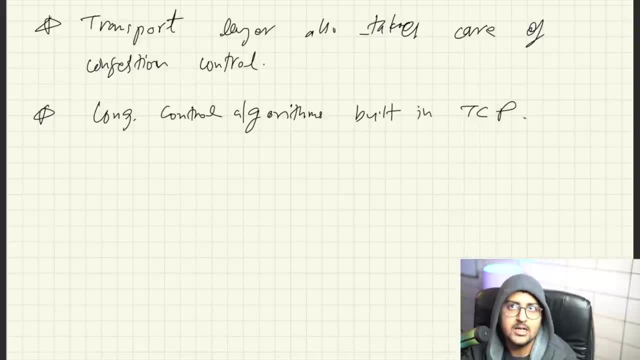 obviously you know can't send an entire file you send the file in packets some for example one are you sending an audio file and something that you said obviously you want it to arrive in that order only 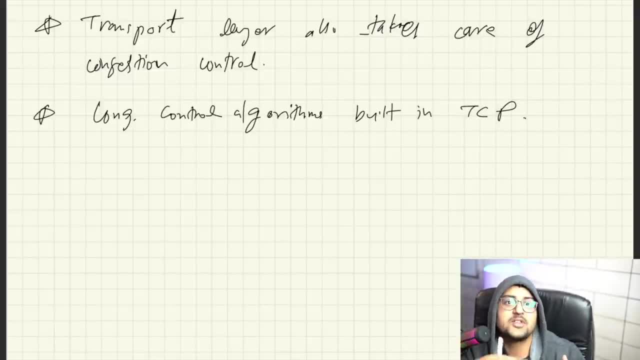 would it be that something you said previously arrives first and something you said said like much earlier arrives at last okay if I'm saying hi my name is Kunal and your friend gets received it something like this my hi Kunal name is that is also not cool right so what you want you want your friend to get all the data if something is lost we you want to know that okay I was sending this 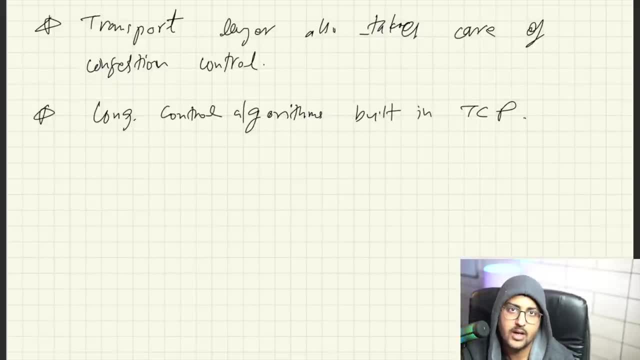 message and these packets were lost due to some error or whatever and you also want to make sure that your data that is you're sending to your friend is in order okay so how do we work with this transport layer protocols they take 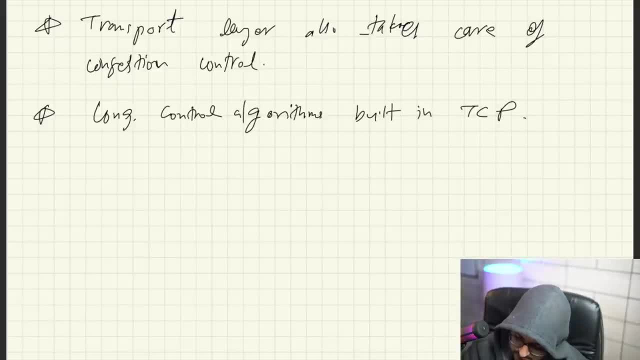 care of this using something called checksums checksums okay sound good so what is a checksum so basically you are sending some data to your friend checksum 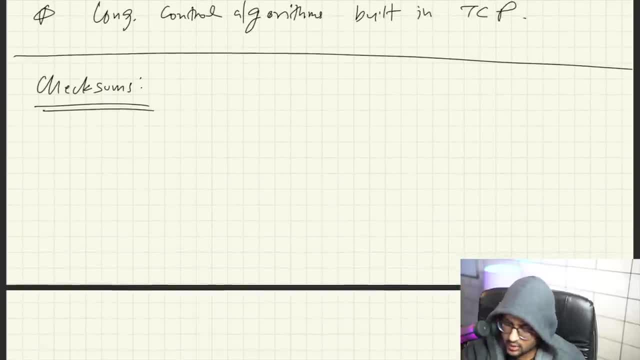 you can imagine it's like a number okay a random number or whatever so basically you have your computer you are sending a data to your function 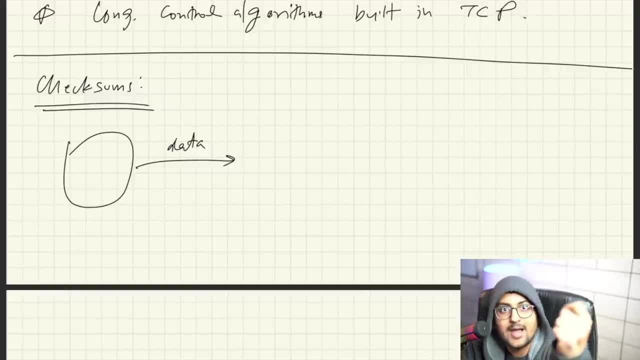 data to your friend using this data you will calculate a particular string value or something okay that will call check some okay then your friend receives this data friend receives the data so friend gets the data and since the checksum was calculated using this data and basically this data will have a checksum associated with it weekly 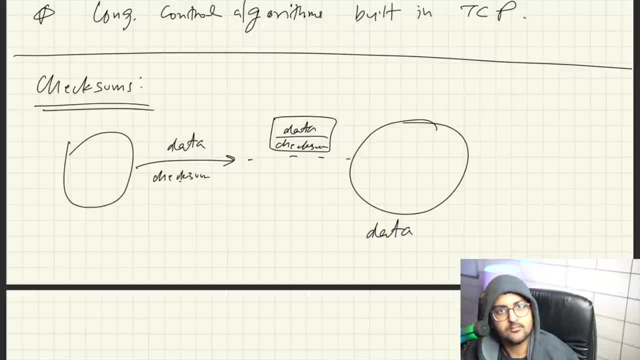 one only checksum so now when you're sending this data over to your friend you will attach the checksum that you calculated in your home and when your friend receives the data they will also calculate the checksum using the same algorithm if the value is different then something is gone wrong if the value is same then it's cool okay sound good that is basically about it 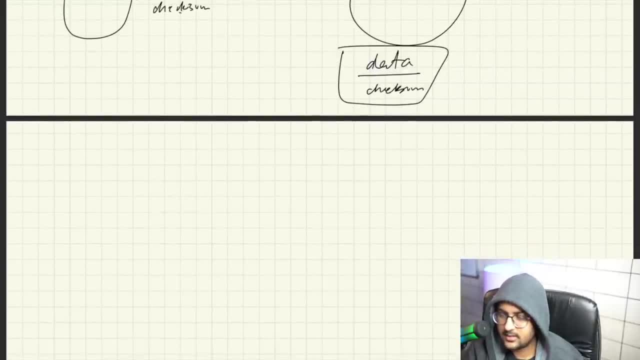 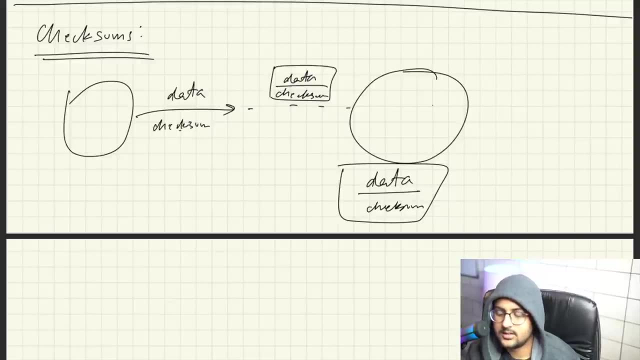 there's one more thing that this was about like if correct data is given or not or whatever okay and uh like if data is not being corrupted or something like that okay but you have to also understand that uh what if the segments are being like you know the the the packets and data packets and things like so you're talking about what if they get lost or something how would i know that my packets have 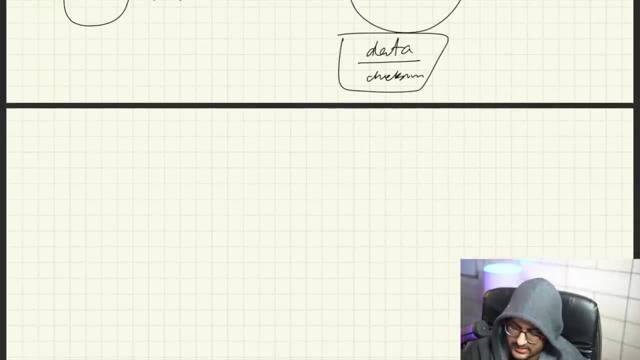 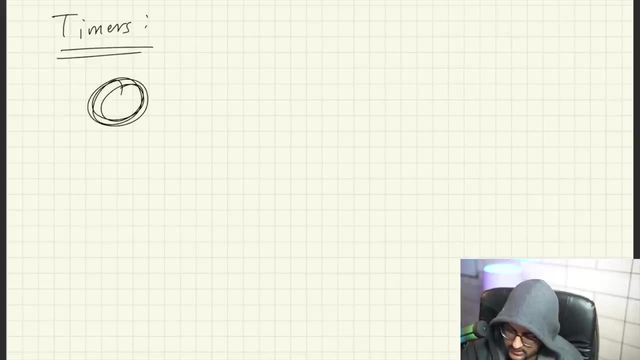 received to my friend something known as timers timers okay so what will happen you are at here you are with your friend like you have you have a computer over here this is this is you okay and this is your friend 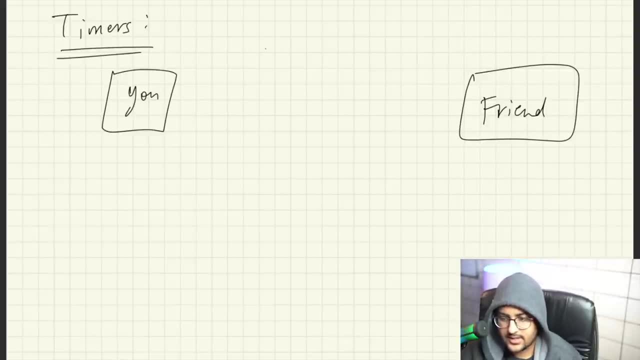 okay cool and basically you are trying to send you are trying to send your friend a data data packet okay so data travels in packets so let's say first packet is being sent to your friend okay your friend is going to be like 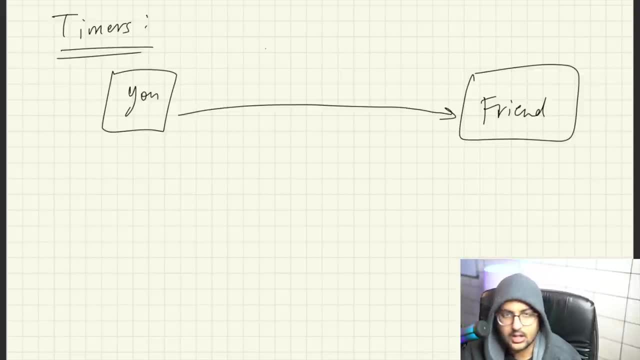 okay i got the packet and your send will send you are like a confirmation but when you send your packet to a friend you will start the timer okay you will start the timer 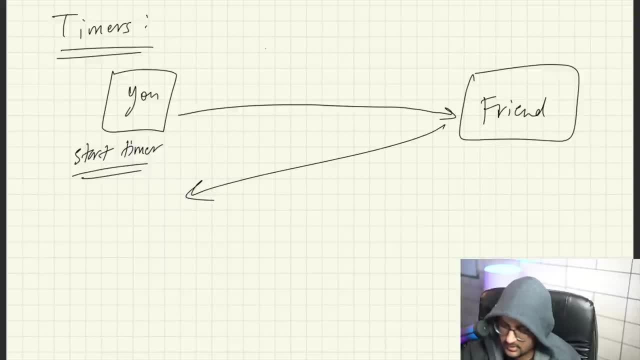 you can be like okay i have gotten the packet i got it so now you will know okay my friend got the packet now let's say you send 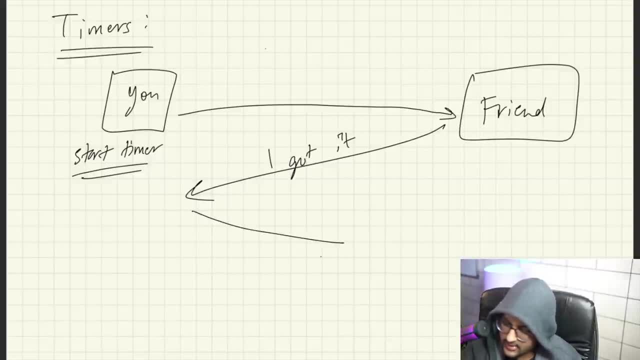 another packet over here and let's say in between only this packet got lost in between only it got lost obviously 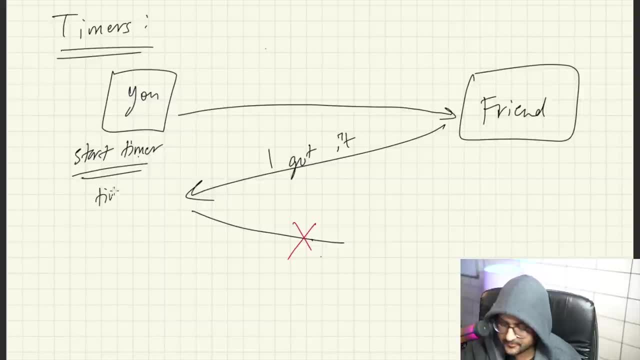 timer will be started and when you receive it back timer end timer end when you send it again timer start again so now timer is running this will never receive over here and after some time 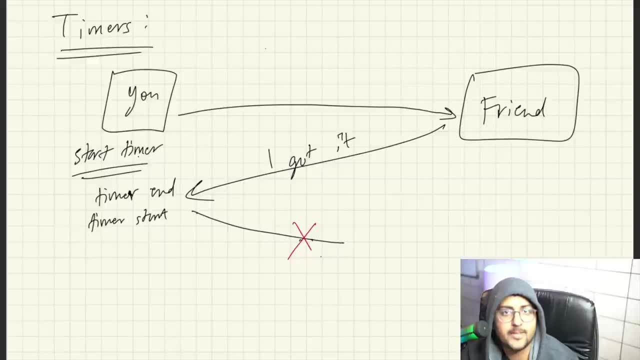 since it's never received your friend will not be able to say hey i got the packet back so hence timer will expire 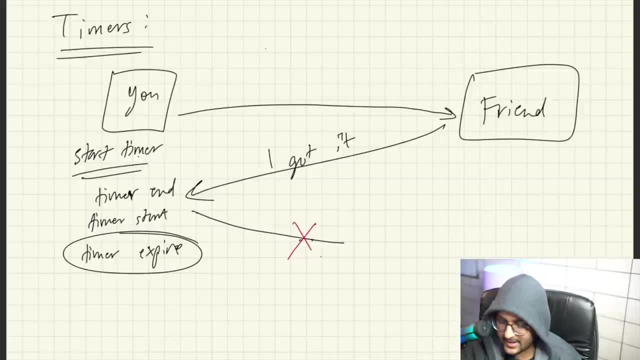 so this is the reason why that you should send this packet to another friend and you will know that this packet two was not sent okay sound good so this is known as timer 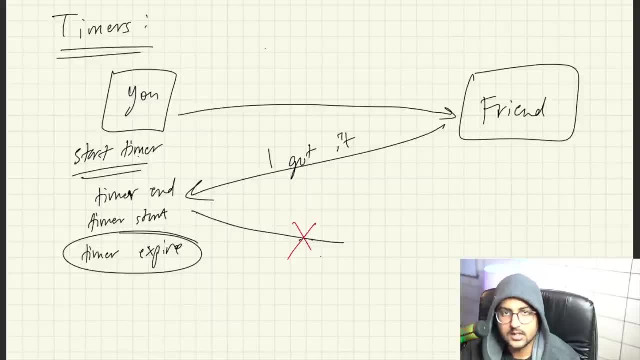 retransmission timer okay it's known as retransmission timer 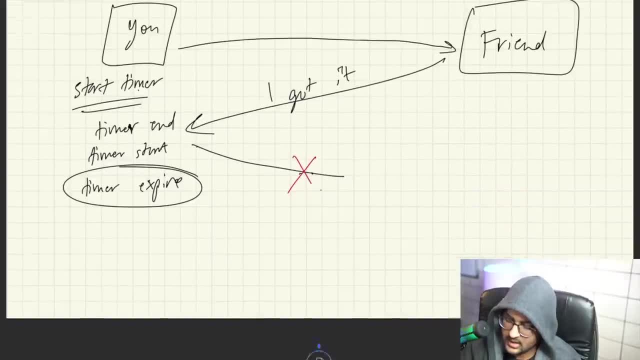 sound good all right imagine that you are sending something to your friend your friend 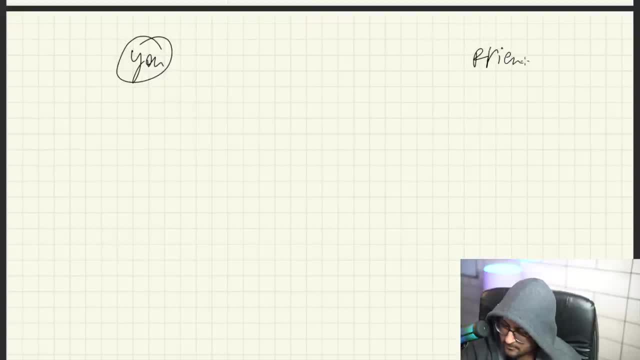 okay so you are sending please don't get confused now with tcp or udp or whatever what are transport layer protocols what are http what is application layer protocol everything i explained to you in details with real world examples so you send let's say data packet number one okay your friend is going to you start the timer your friend is going to like hey i got it you end the timer then you send it again packet number two you will start the timer your friend will let's say send you back again but let's say this friend does not tell you like while it's receiving back like hey kunal i got packet number two so you have not received 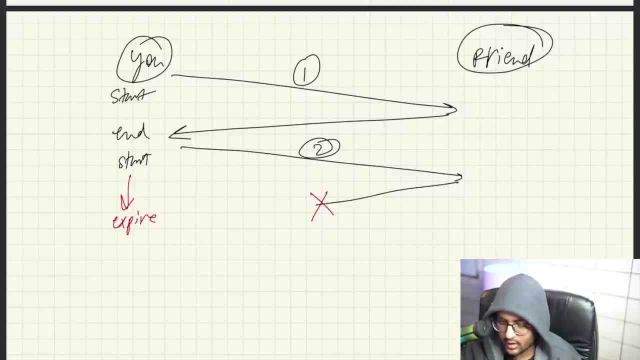 that and timer will let's say expire for me i don't know now that if they received it or not 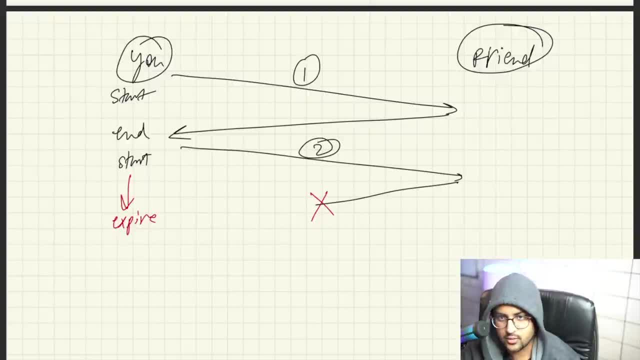 so i'll treat it as that they did not receive packet number two i'll try to send another packet number two you now this person has two packet number twos duplicate 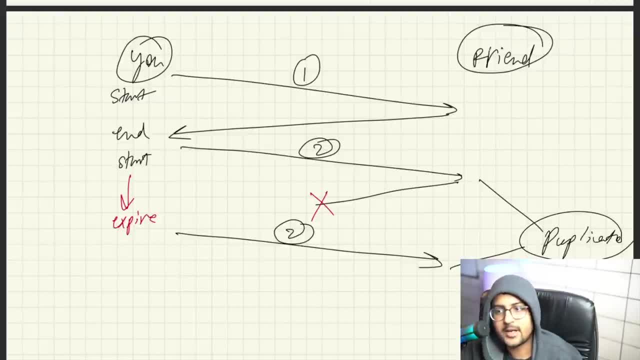 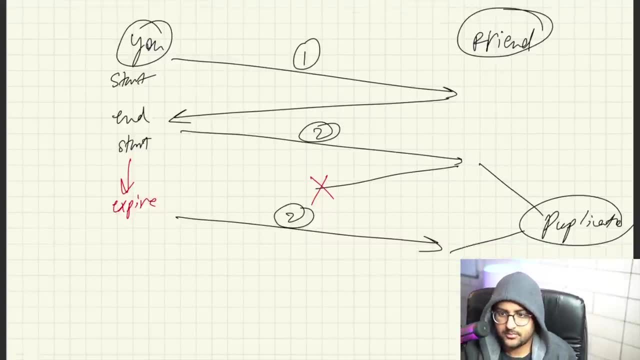 duplicate packets are available are you able to understand what is happening okay how do we solve this problem we solve this problem using sequence numbers 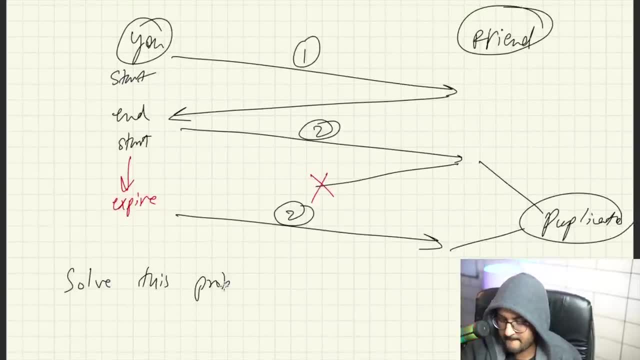 sequence numbers okay so unique like identification uh like a value number will be provided every every packet every 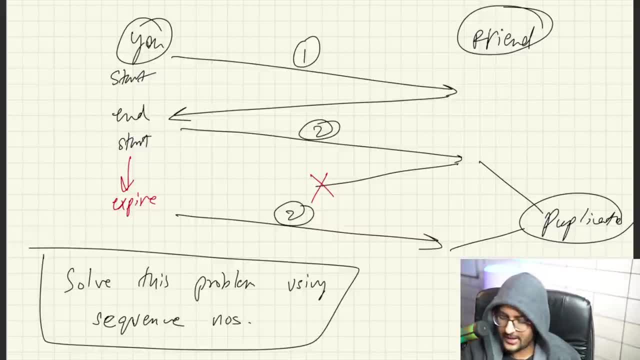 segment will get it okay so that's why how we can i identify okay you got a segment with number two uh number two was already present with us so it's a duplicate one all right okay so that was basically 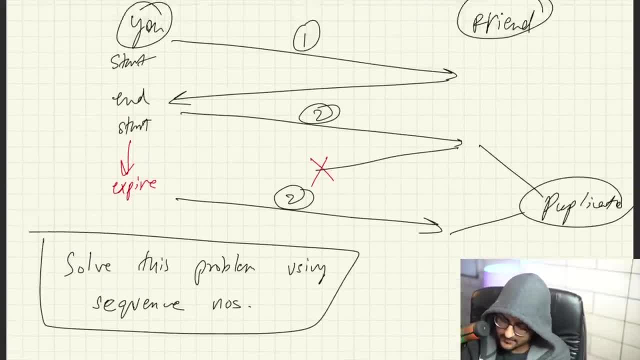 about how it works so we looked into detail about http and like application layer and what transport layer is what it does how it works so that was basically about how it works so we looked into 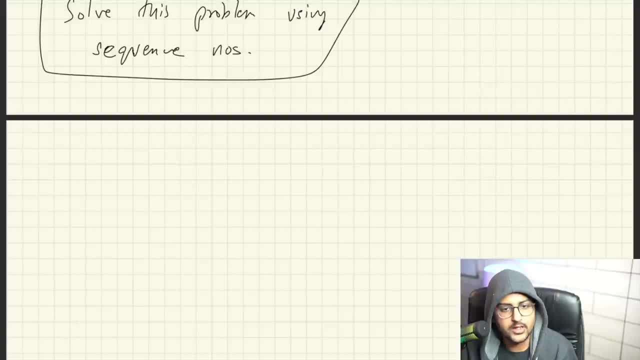 it does it only thing we need to look now is uh we need to look at in details uh about tcp about udp about ip addresses we haven't looked into that much um like obviously we'll look at 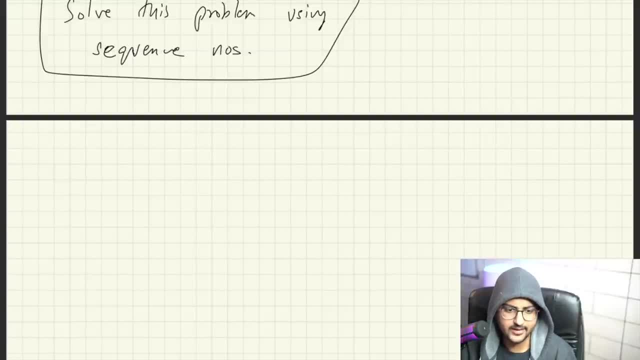 we'll look at that in the network layer and uh the data link layer and the physical layer is nothing 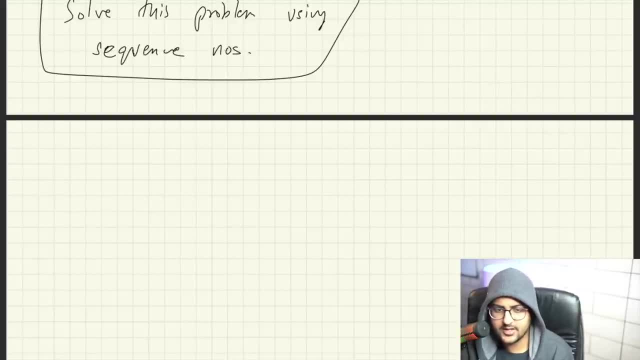 so it's just like physical devices so not much to cover over there but this is the only thing remaining right now okay so let's start with uh protocols deep diving into protocols now uh what are the transport layer protocols we are still on transport layer so what are the transport layer protocols tcp and udp what are the application layer protocols http and stuff right 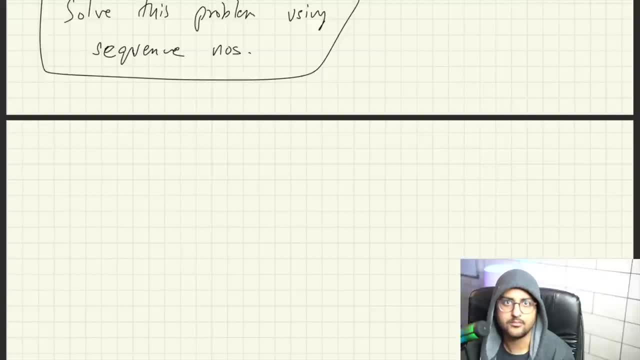 what is the network layer protocol ip internet protocol uh so we'll uh we'll take a look at all of these okay cool first let's start with the um transport layer protocol so since we are transport layer we know where transport layer works and let's look into udp now udp 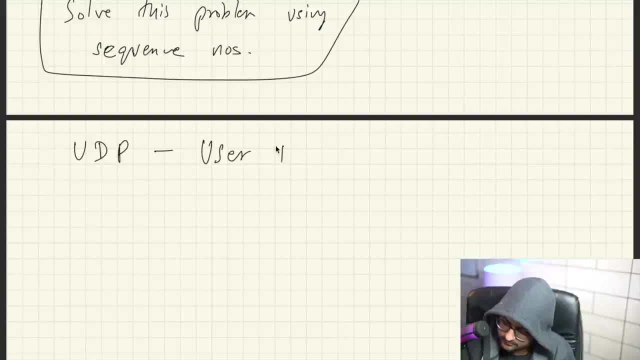 udp stands for user datagram protocol is it recording yes okay 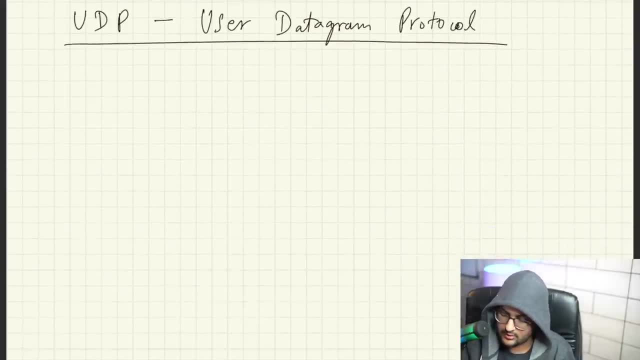 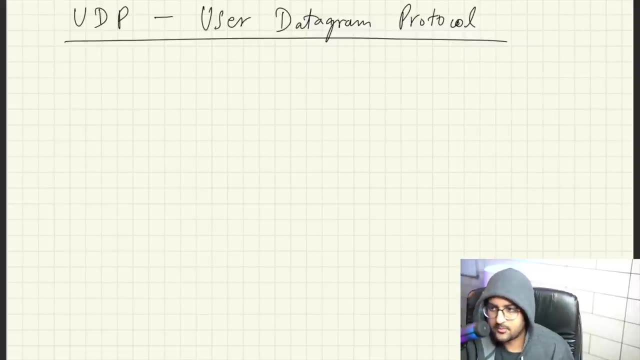 let's learn about user datagram protocol so what is ucp udp it's basically pretty simple it's uh the transport layer protocol right and uh it basically uh uh you all know what it is like it's used to transport you know like data in the transport layers like from network to transport layer and from transport layer to network right but the problem is that uh here your data data may not be delivered okay data may or may not be delivered okay data may change on the way 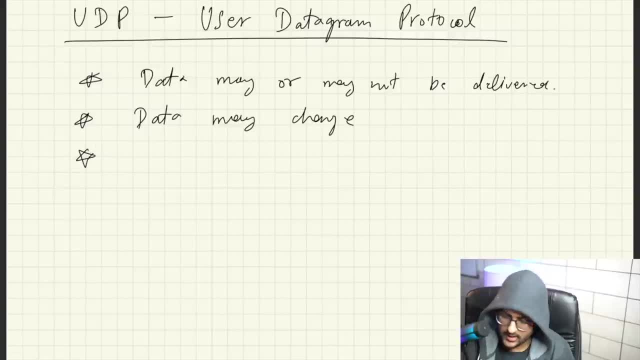 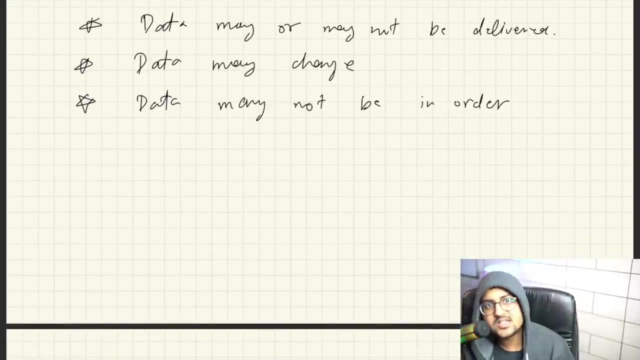 data may change on the way okay data may not be in order when your friend receives the data data may may not be in order so this is the problem so obviously if you want to send some documents emails or whatever do these technologies use udp then no if they use udp then your email may come in different order or some data will be lost or whatever important files will be you know corrupted or something like that right sound good all right so let's see how it happens so basically uh it is a 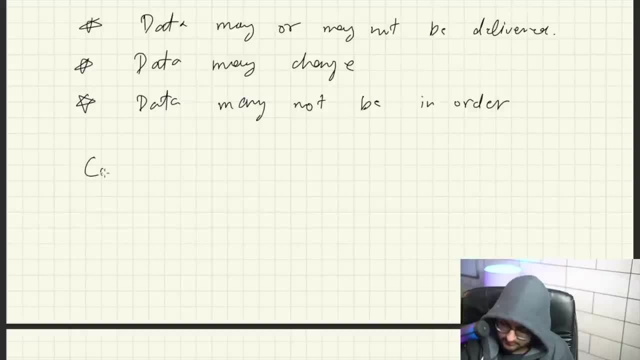 connectionless protocol connection less protocol okay means no connection will be established between the two computers and it will still send like the data in tcp it will be like hey let me make sure there's a connection between these two and after that i will send data which i'll look into later on 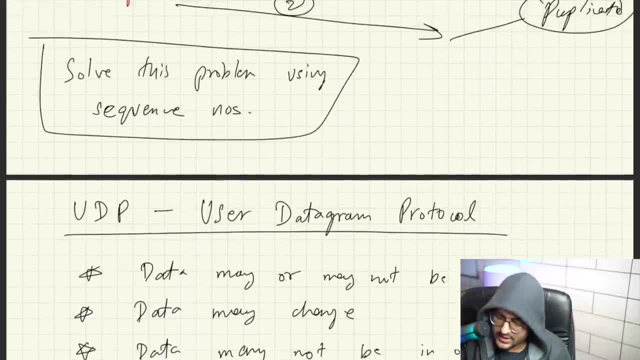 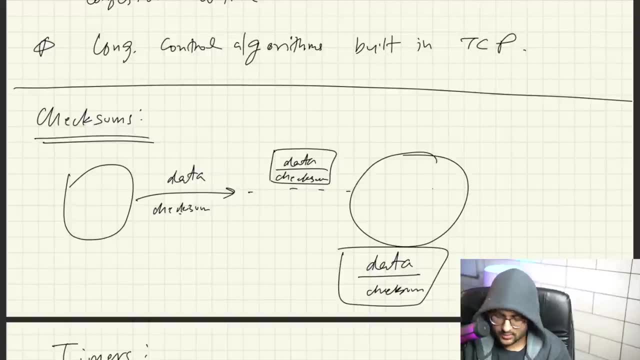 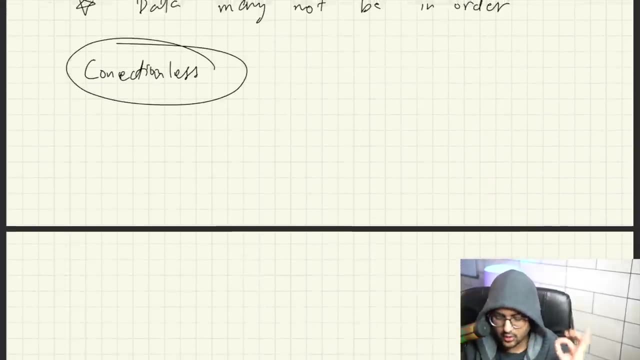 okay connectionless protocol okay and this thing that i mentioned over here this thing this thing the check something so checksum is used for what to to check whether the data has been corrupted or not okay udp uses this so udp uses this udp uses checksums udp uses checksums 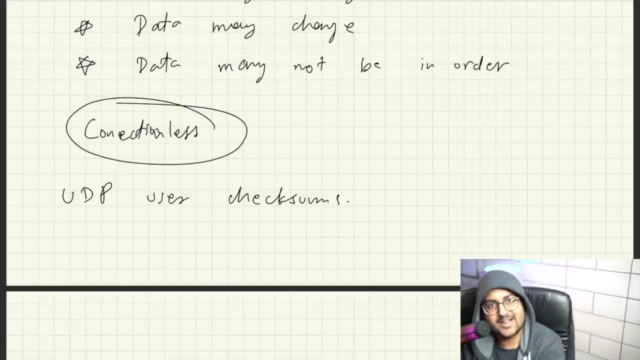 okay so you will know whether the data has been corrupted or not but udp will not do anything about it okay it's corrupted there's an error okay no problem it is what is it what it is okay so let's look at this particular header and this particular like 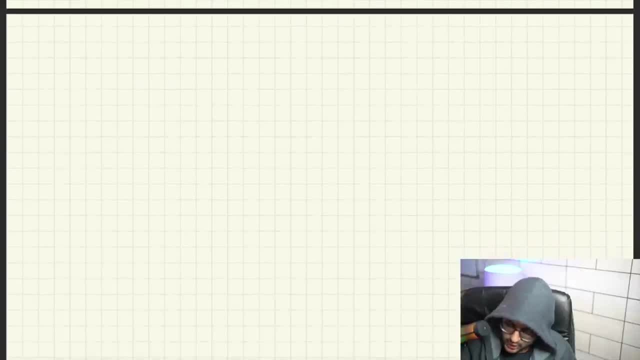 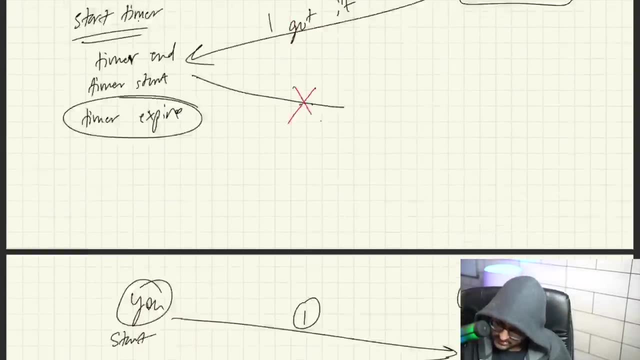 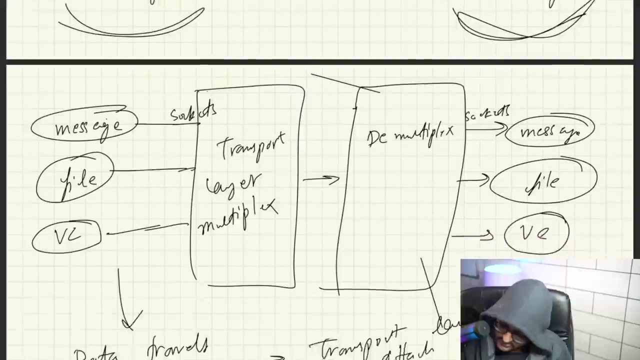 uh the packet that we'll be sending so udp packet what does it look like uh previously we mentioned port numbers um obviously if we're talking about like transport layer in transport layer we have port numbers where are those we mentioned it somewhere over here sockets and sockets have uh 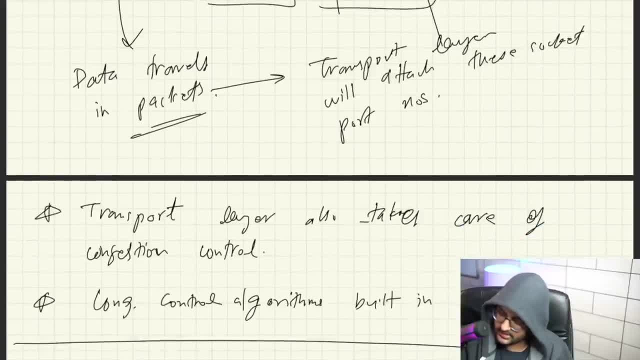 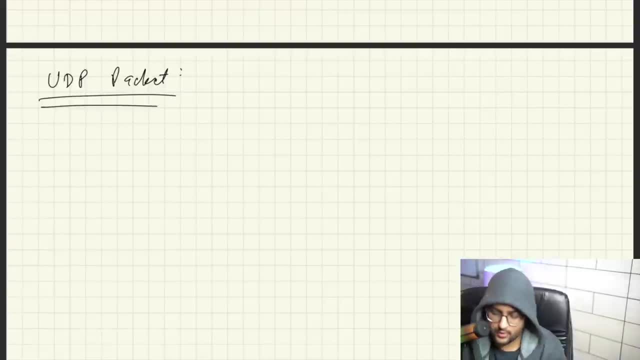 sockets and sockets have port numbers okay so the port number in the transport layer will attach these socket port numbers it is written over here okay so every data packet will have a port number your port number and your friend's port number so 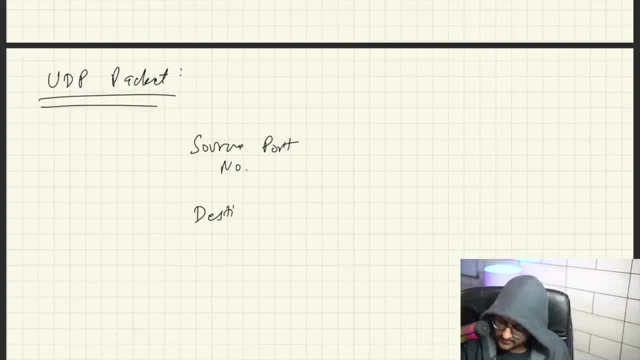 your source port number and your destination port number 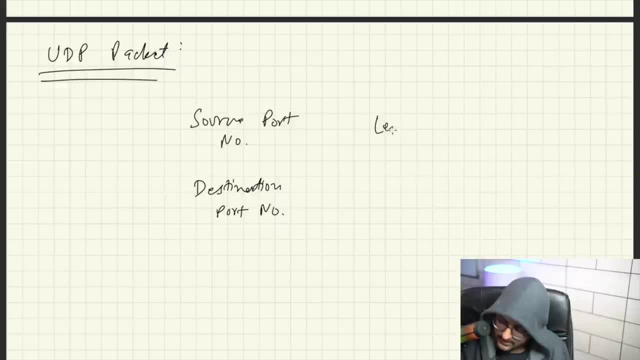 destination okay the length of the packet the length of this data gram it's known as data gram length of 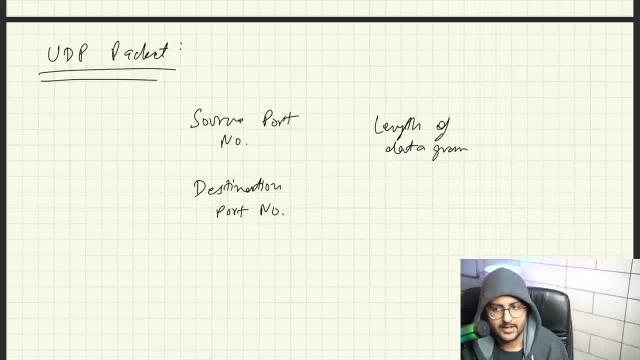 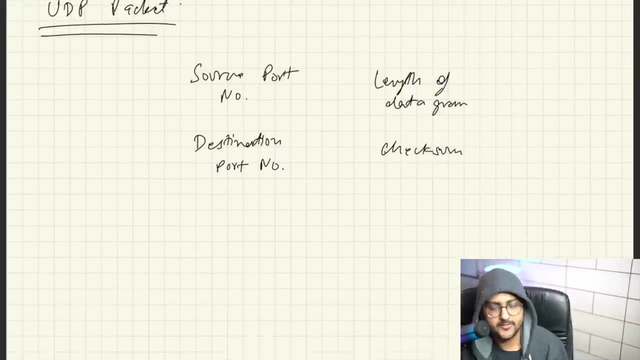 data gram will also be added okay and what else checksum checksum will also be added so these are all the additional things that will be added and 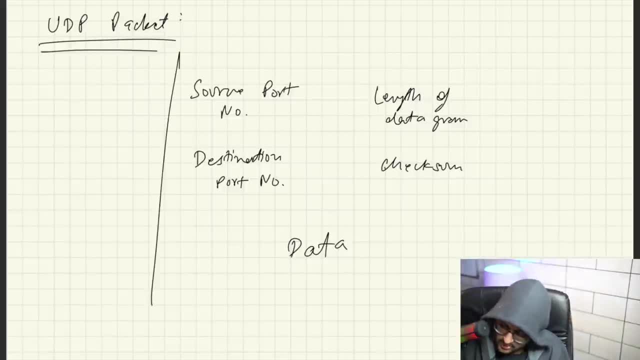 then obviously your data will be added what data you are sending okay this is what is added if you want to check the size of this then uh this is two bytes um this 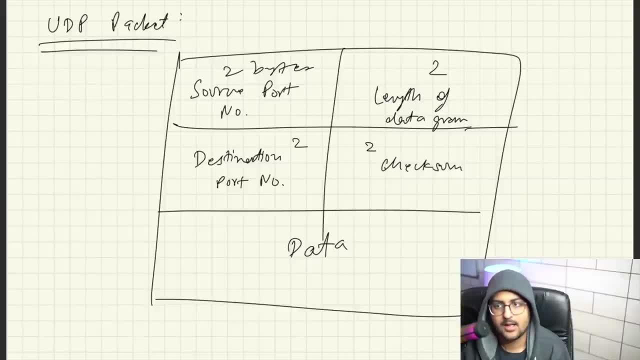 is also two bytes two bytes two bytes and the data is also i believe uh two bytes okay so one 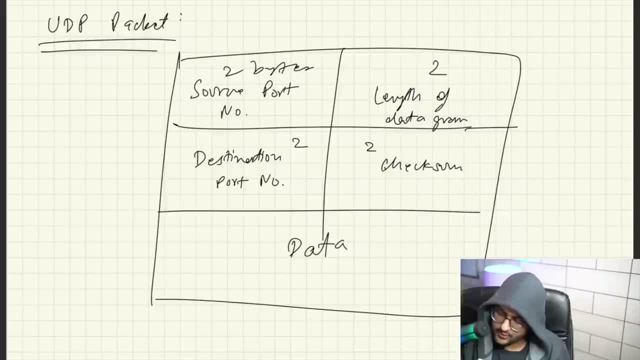 two three four this is total eight bytes and then you have your data oh no data cannot data is not two bytes two bytes is very less um data is like if you're talking about the total size right so let's see total size total size is equal to 2 raised to power 16 and this particular thing 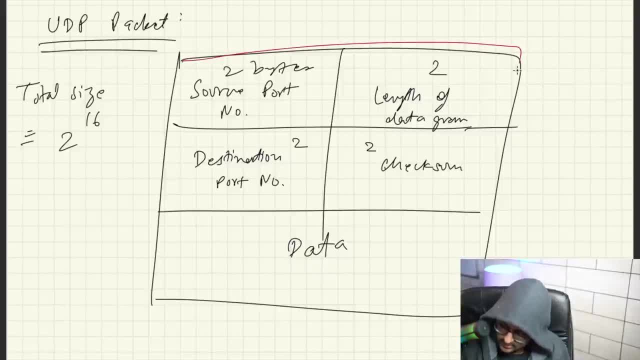 okay the the header this is known as the header something that is attached to you this is header this is 8 bytes 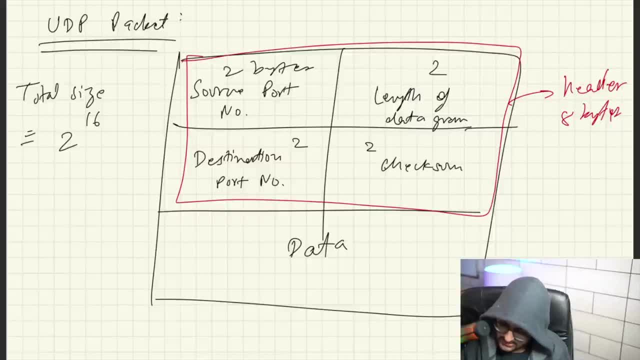 okay um so total size of data is 2 raised to power 16 minus 8 which is equal to 1 6,000 65,000 something these many bytes this is the size of the data that you can send in one 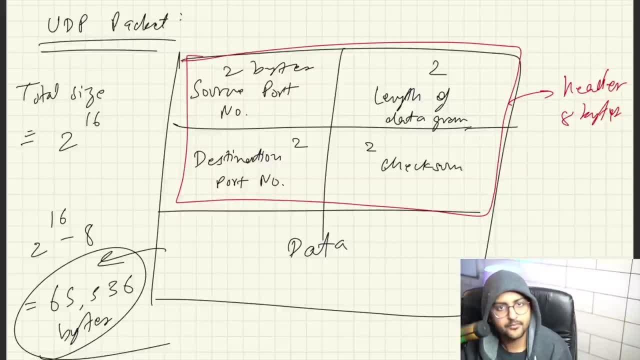 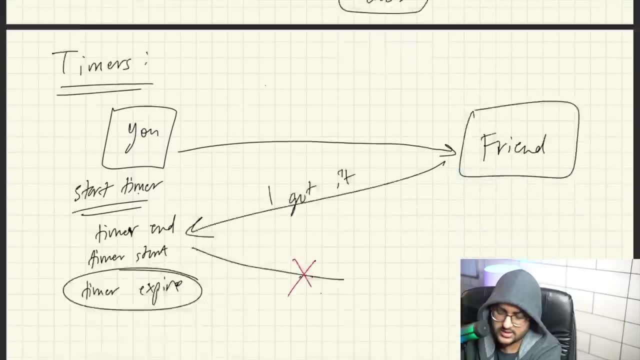 but okay cool so that's basically how it happens same thing we've mentioned previously that's it these all things we mentioned okay that was it no initial connection or whatever just like we 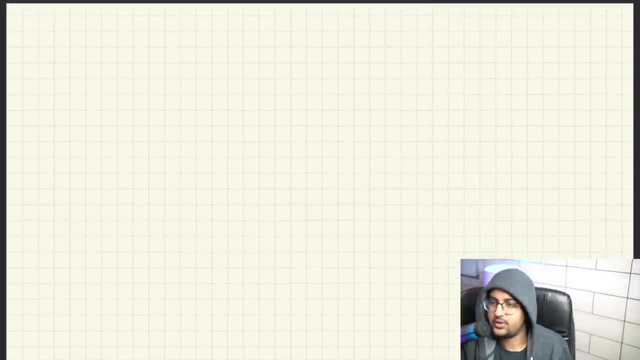 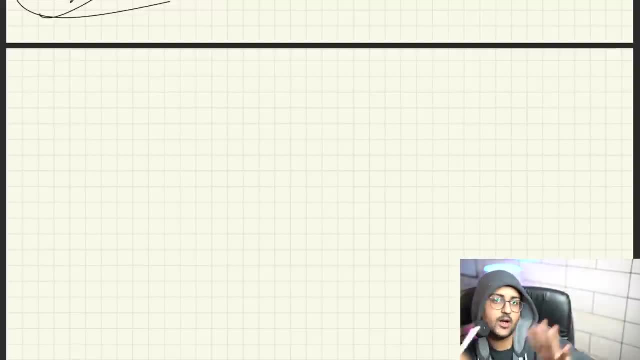 mentioned previously it happens like that same checksum theory okay so why do we use it because UDP is like faster right because it's not like always checking for hey did you get the data or whatever okay sound good cool all right so that was about UDP and it's a lot lot 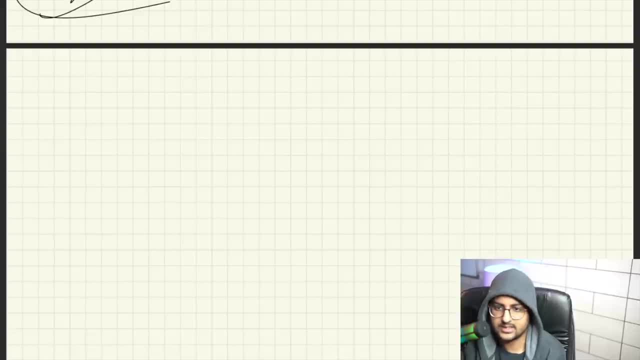 faster that's why we that's why we use it and that's pretty much about it cool 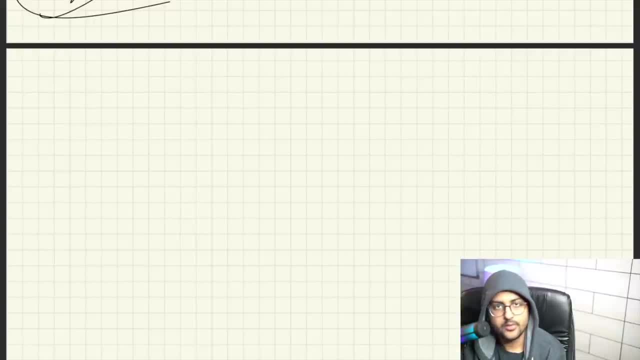 and when we talk about DNS use cases of UDP use cases it's very fast let me just 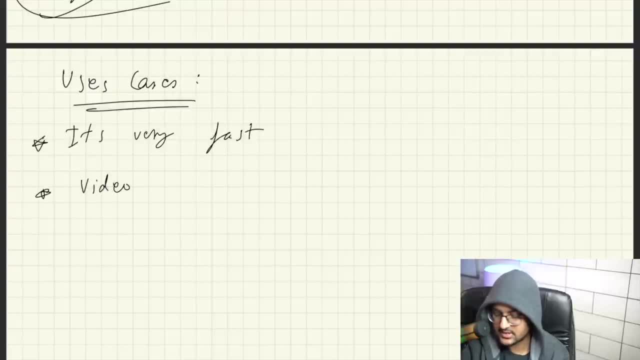 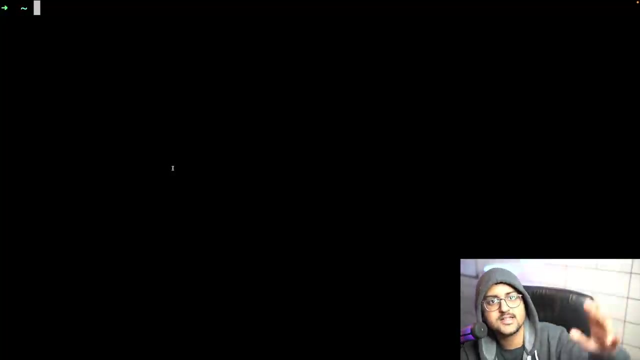 write some use cases video conferencing apps video conferencing apps and the DNS thing we talked about previously this also uses UDP because it's fast okay gaming gaming also uses UDP okay cool okay you can actually use a command to see all these data packets that are coming in and out of your computer okay so you can say TCP dump and I can say only give me five packets okay if you remove five this see my dash c5 then it will show you all like that are coming okay I only want to see five so here you go five packets 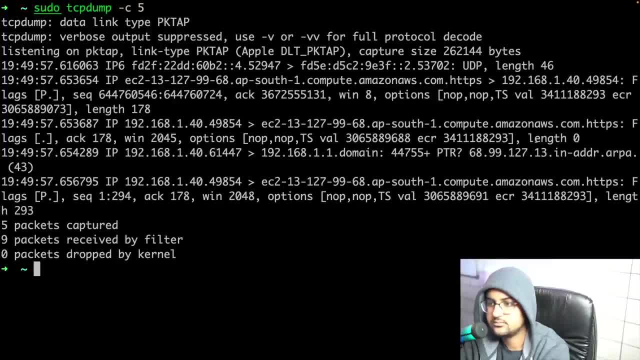 captured and there you go and that's it guys thanks for watching and I'll see you in the next it has all the information you see udb packet okay sequence is there length is there and so 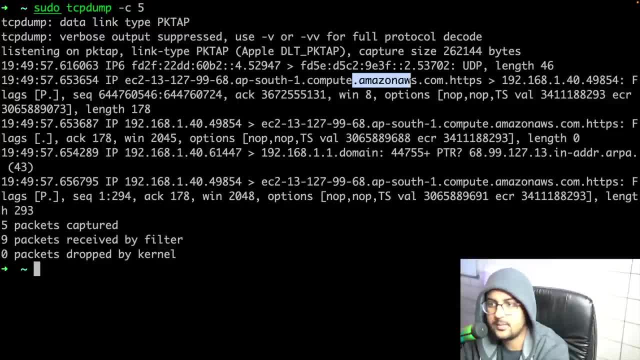 many other things uh ip is there aws it's coming from somewhere right um that's pretty much about it okay so these are the ec2 instances these are in ec2 instance we'll talk more about these things 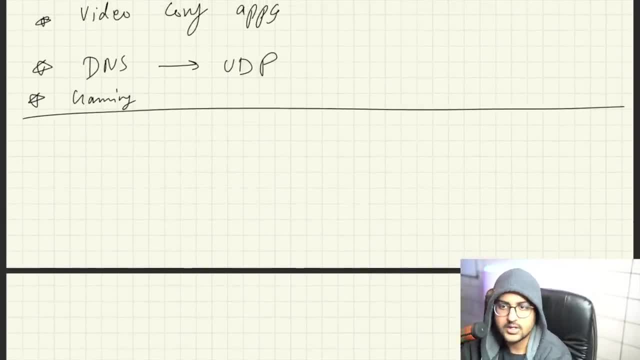 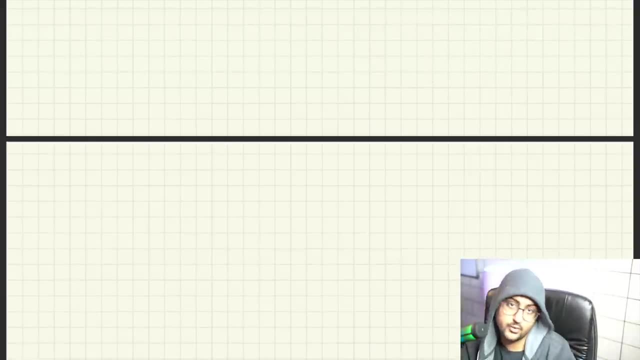 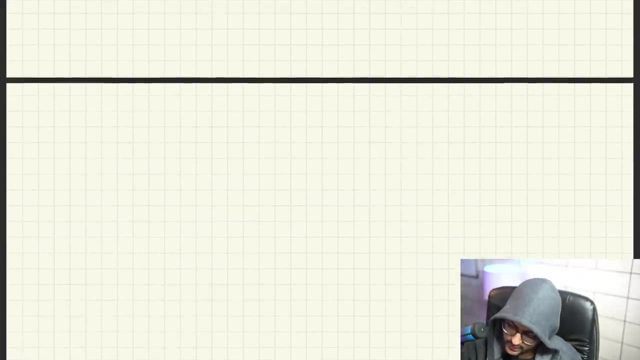 that was udp now let's talk about tcp protocol so tcp means transmission control protocol uh we have already looked at it in brief and we're talking about http so http uses tcp right and we we know like let's talk about tcp i'll write and i'll make a new page for this okay because this is an important topic it's also asked in interviews quite a lot explain tcp how it works 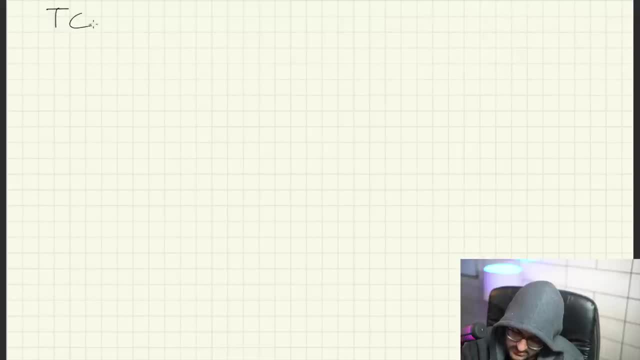 okay transmission control protocol uh tcp tcp transmission control proto call transmission control protocol we already looked at udp and now it's time to look at tcp so we 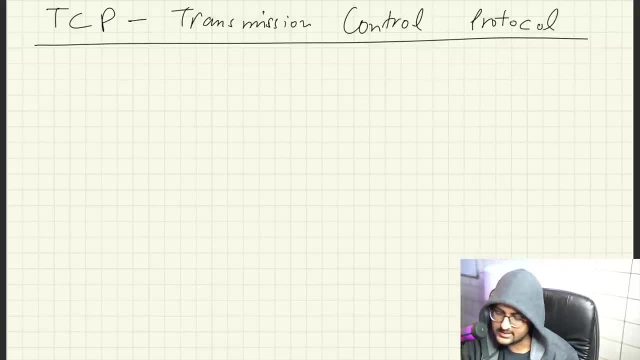 know that it's being used in sttp and it's like very uh you know uh like the data we have is uh you know it stays with us so what is the difference between tcp and tcp what does it what does it do like what is the use case of of tcp obviously uh we talk about tcp so it's on the transport layer so we know it's from uh taking the data from your transport to your network and from network to your transport layer okay so basically it allows us to do that it's at 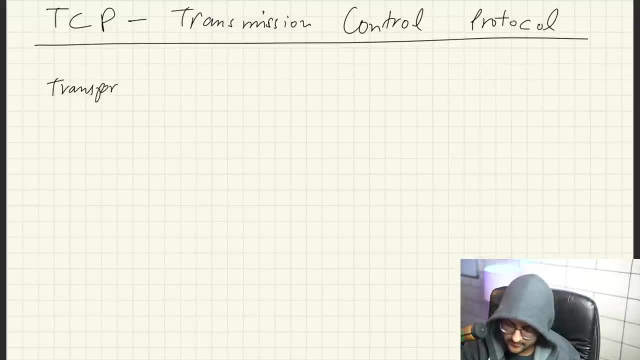 the like the transport layer protocol okay transport layer protocol it does the same thing that udp does but differently okay when you um uh you know when you get the data when you get the data in the transport layer from where application layer so you get data segments okay so application layer sends data application layer sends lot of raw data let's say it sends lots of raw data and tcp 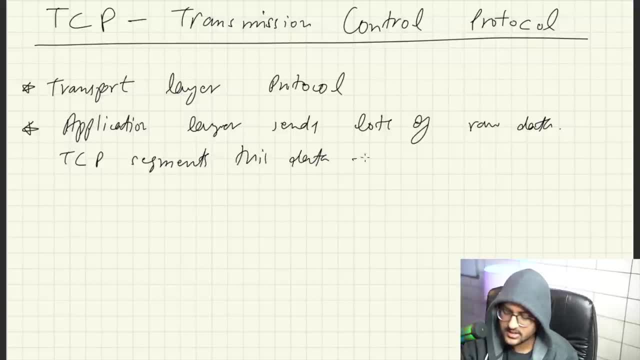 segments this data means divided in chunks or something divide in chunks add headers you know check sums so on and so forth all these other things okay it may also 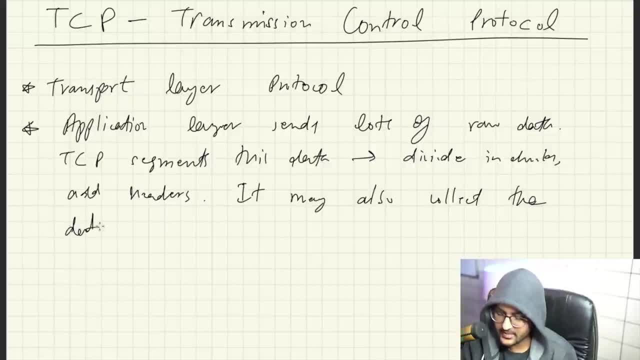 collect the data from network layer 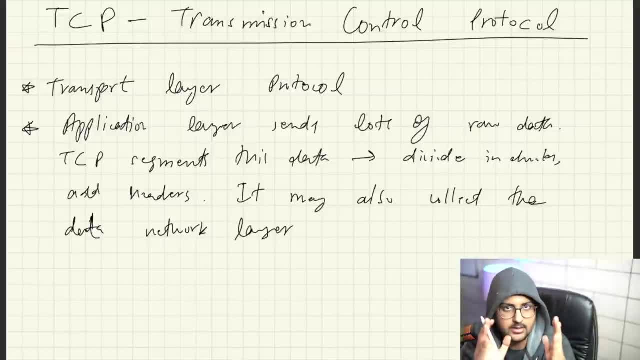 uh when network layer distro for example you have a network layer distro for example you have a network layer distro for example you have a data uh and transport layer passes the data to what layer network layer network layer may divide that data into more smaller chunks so at the receiving end of your friend those more smaller chunks will be put into one okay check video i can't write this so yeah you can check this video 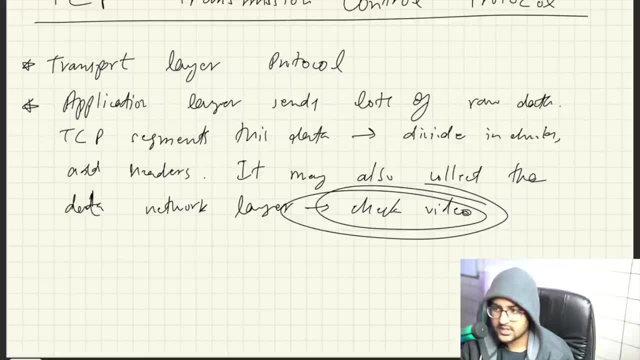 when you look at notes okay sound good so it also provides one more thing which is congestion control that's we talked about previously congestion control okay sound good cool 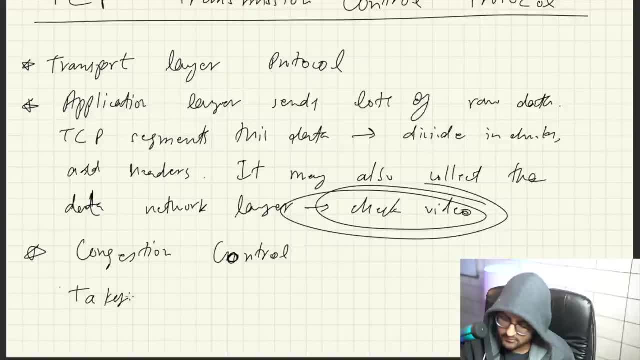 it takes care of two things takes care of um when data does not arrive okay so it will work with that sometimes data may not be covered so it will work with that 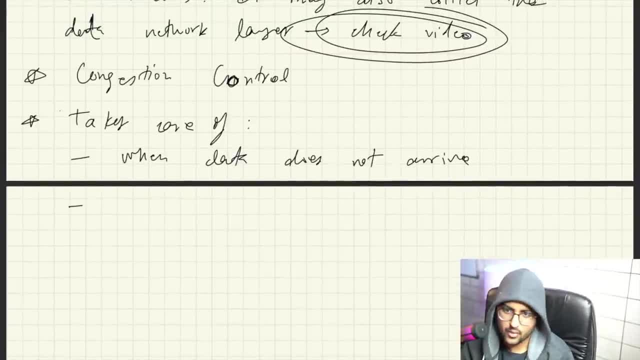 sometimes data may not be delivered so it will work with that sometimes data may not be delivered so in that case we have to work with it and also rearranges and maintains the order basically okay 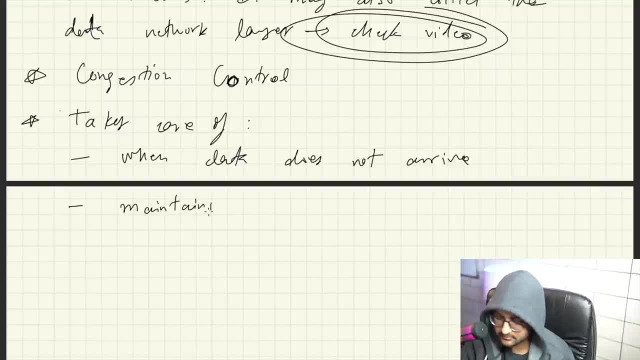 maintains the order of data maintains the order of data and we looked at it previously how it does it using sequence number 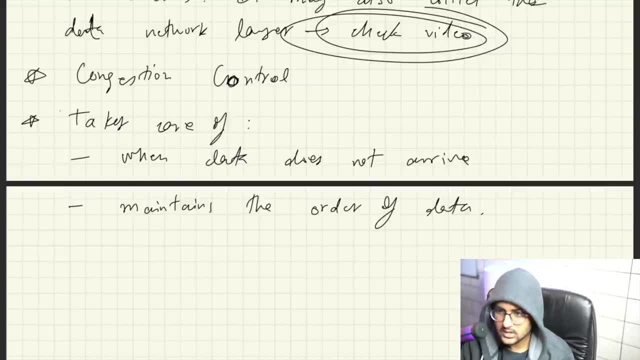 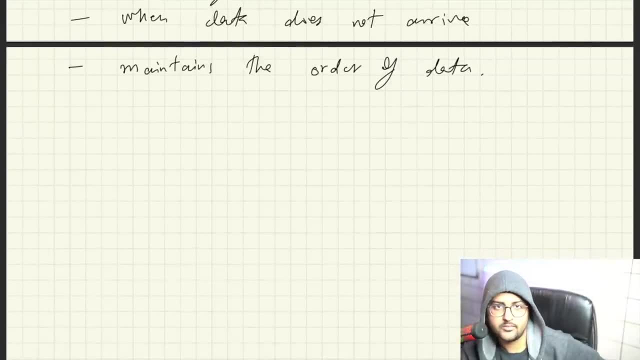 okay cool so tcp is pretty pretty awesome we can use it in various various places like we can transfer some pdfs you know um email and uh the http uses it so web browsing and so many other things like email and email service and things like that okay so what are the email application layer protocols smtp right pop imap we talked about these previously so these application 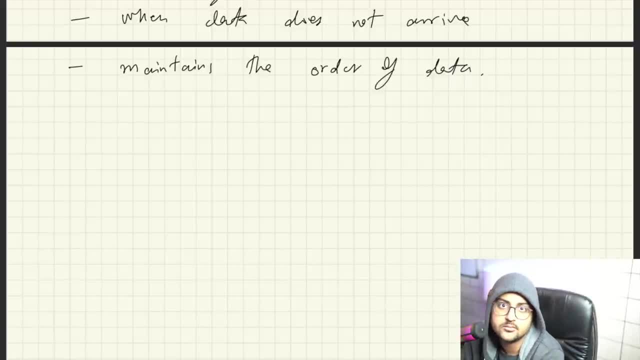 layer protocols use which transport layer protocol tcp okay what are some of the features 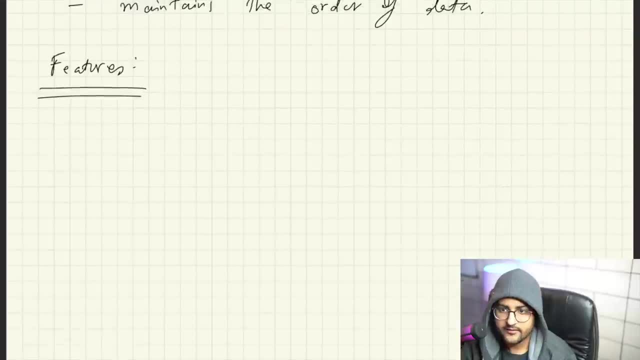 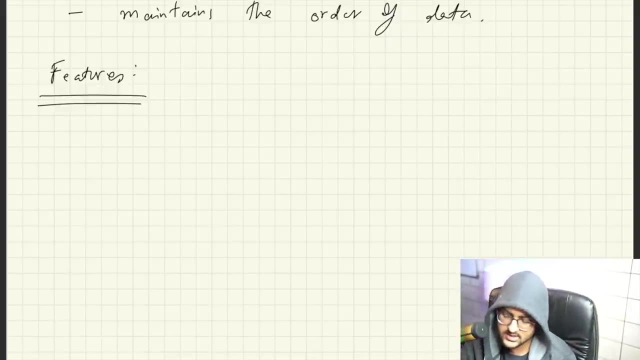 features uh it's uh it's pretty straightforward so basically udp was connection less this is connection oriented means first a connection has to be established and then you can send data 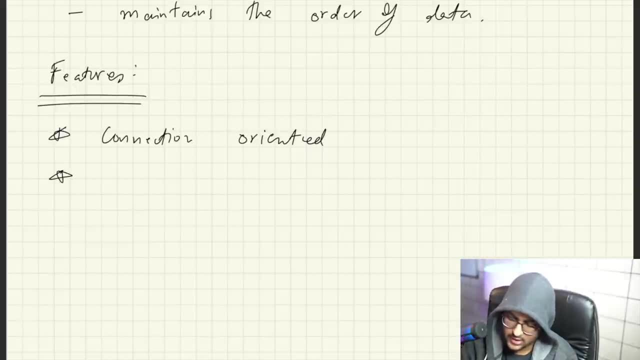 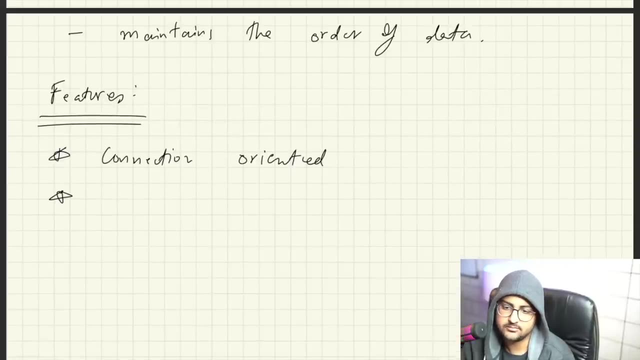 okay cool it is also um you know um uh it is also also provides us um like um 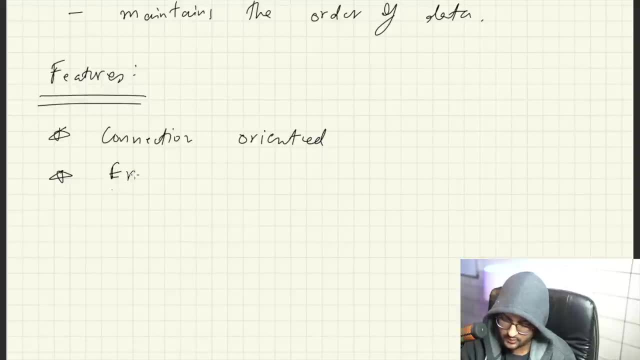 error control okay so error control we talked about this obviously error control okay congestion control we've talked about this also 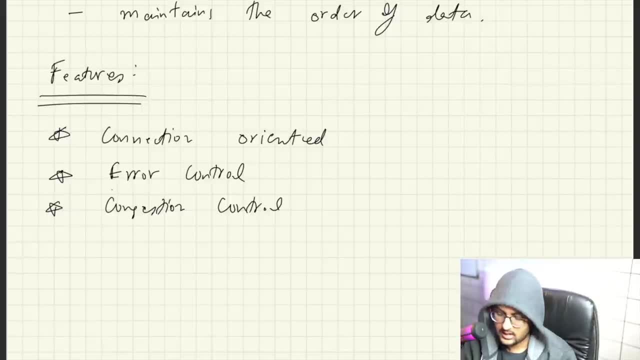 congestion control right um it also is there's one more thing like uh bi-directional okay i mean like duplex full duplex full duplex so what do we mean by full duplex basically this means that 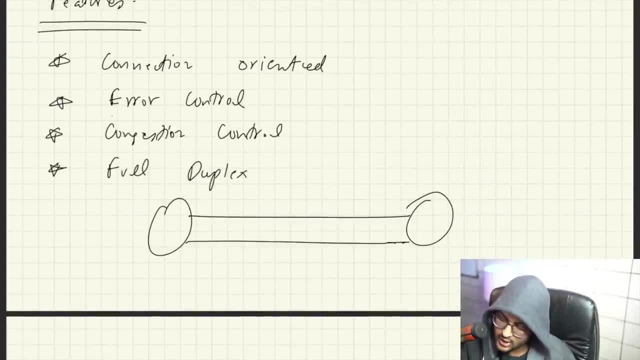 you are two computers connected to each other you can send one file from computer a to computer b computer b can then send another file like this or you both can send files simultaneously okay sound good cool 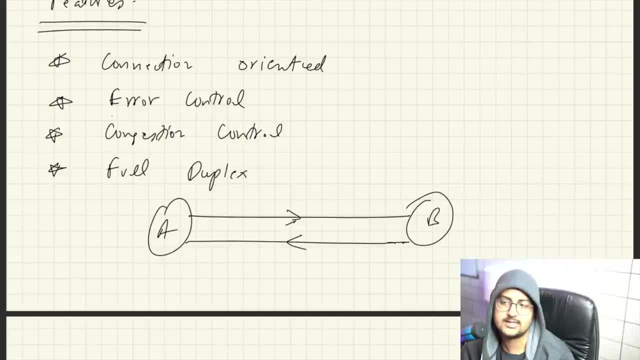 notice something that using tcp there can only be two endpoints like this okay so you cannot like send one message to 10 computers no they will they all will be having their own dcp connection one tcp connection only two between two 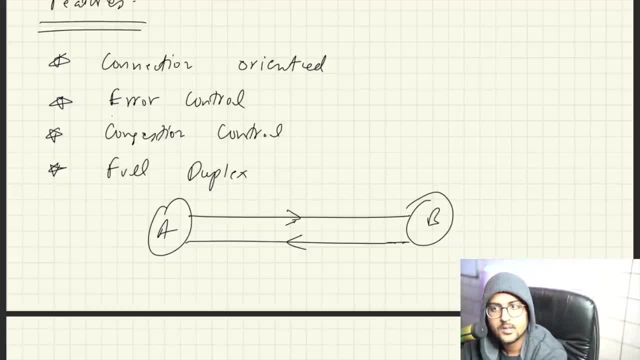 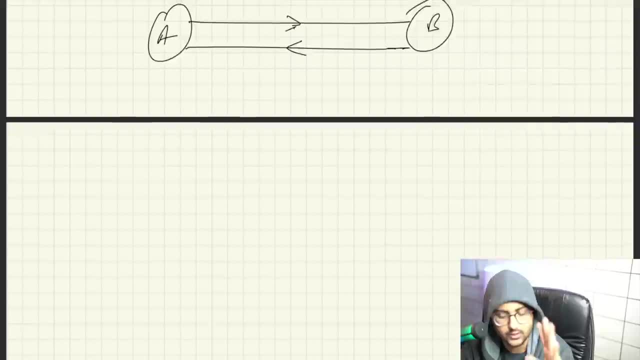 computers okay so that's basically about it okay so let's talk about this connection thing canal you're saying it first establishes a connection between two computers and then it transfers data how this connection happens media application data transfer perhaps something you've already heard about data当 common connection using during application or data connection only when flow actually nobody knows about it all right you know ok so you're already know about but then we go on to other things about data 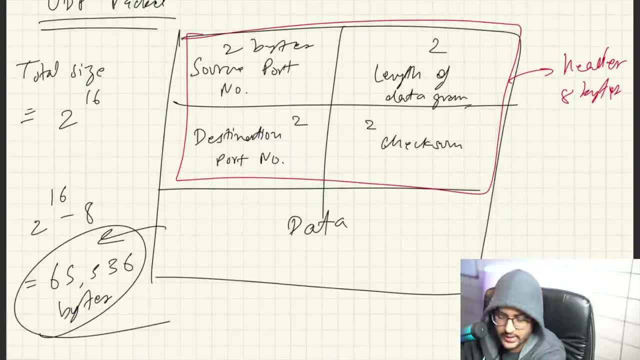 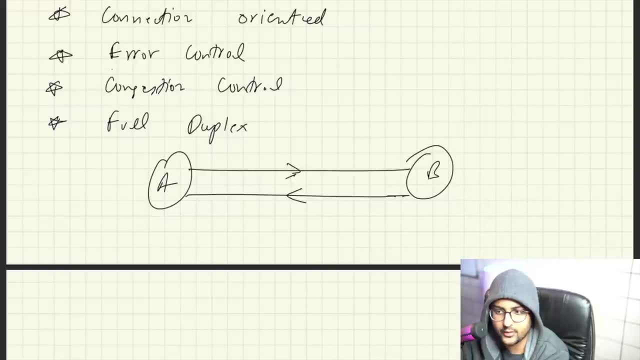 about like data segments this is the one that looks like for udp for tcp it's a little bit more complex okay so if you want to look into like the details of it you can you can check it out you know the research papers for that so i won't be going into much details of it because it has 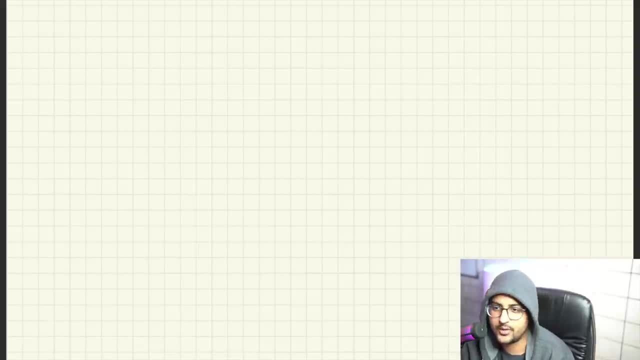 a lot of things obviously if it's connection oriented then obviously a lot more details are required but basically it has the same thing like the source and the destination port number the data obviously will be there um it will add a sequence number and an acknowledgement number okay and obviously your checksum and stuff so the sequence number and acknowledgement number are the two two different things that we have looked into right now so what does it mean so basically first i will tell you verbally then i'll draw the diagram what happens is that the client will request the server you will request your friend's computer hey i want to establish a connection with you then your friend won't ask you to set it up for you so you can make sure that you have the connection and then you can make sure that you have the connection and then you can make sure that server will respond back to you you're like yeah sure i want to establish a connection with you too and then you will respond back to your friend okay cool uh i accepted and uh connection established 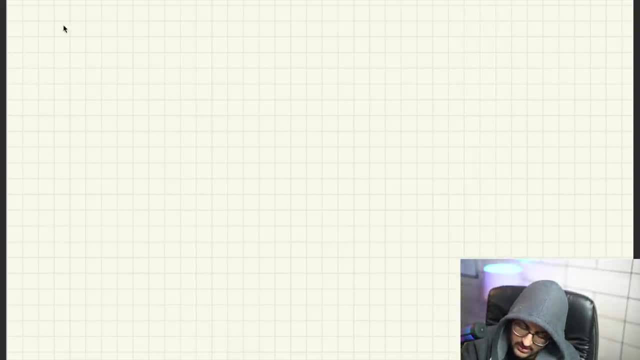 three-way handshake this is known as three-way handshake three-way handshake very important concept and also asked in interviews three-way handshake okay your computer let's say this is the client this is the server okay so you will send a connection request and in your connection request you're going to send it to your server you will send the connection request you are going to 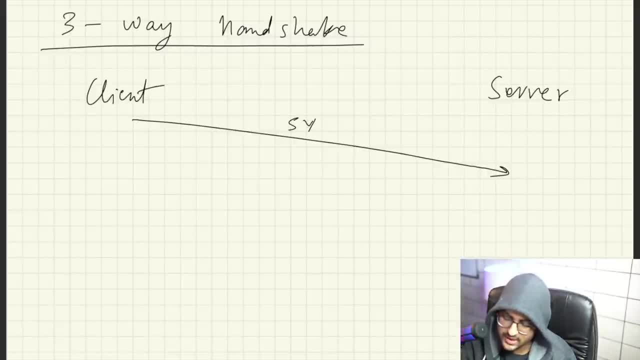 send a flag which is known as a synchronization flag this is a flag that you send synchronization flag it means that a new connection is being established this is nothing this is just like a flag a value inside the header 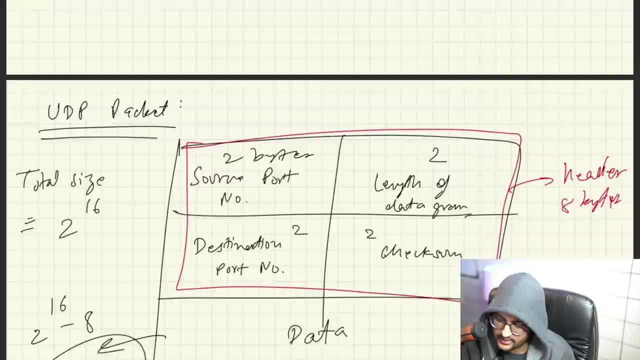 that's it don't ask me what a header is okay we already covered over here this thing okay cool 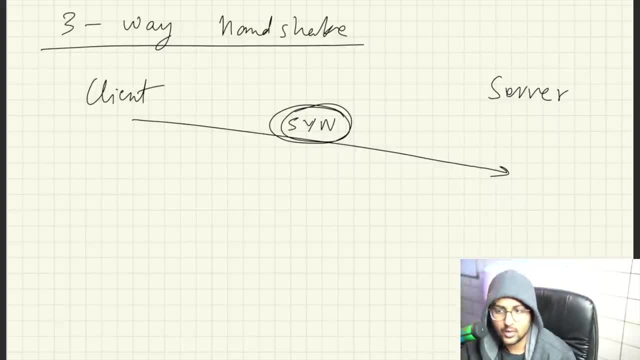 the server will be like oh i have got a new sin flag what do we do it also sends a sequence number so we know it's in order so sin flag and a sequence number will be sent okay let's say that the sequence number is something like 32 random number okay so sequence numbers are random numbers uh the question is why because 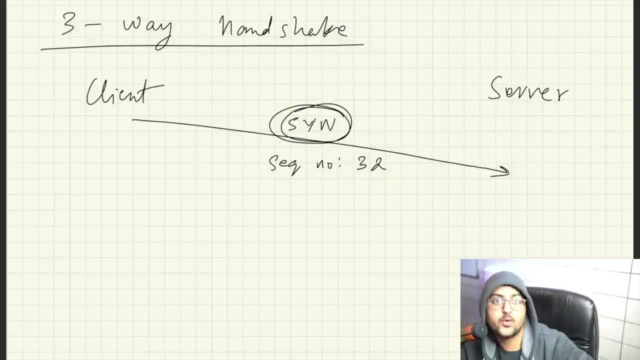 um if the sequence number were not random then it would make it very easy to guess and anyone would be able to make connection with the server and hackers could uh you know uh take advantage of this so security purposes sequence numbers are random okay 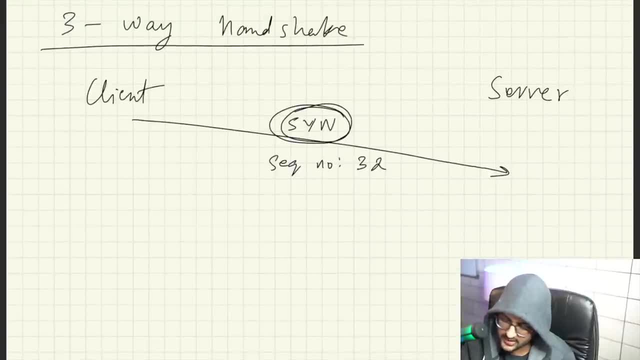 um server will be like okay sure i have got your sin flag and i will send you acknowledgement flag it will also have a sequence number of random something like 85 not i think it takes the sequence flag it takes the sequence number from the client 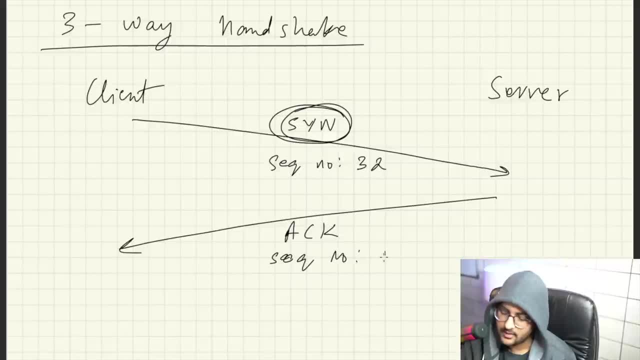 does some mathematical calculations on it yeah do some maths on 32 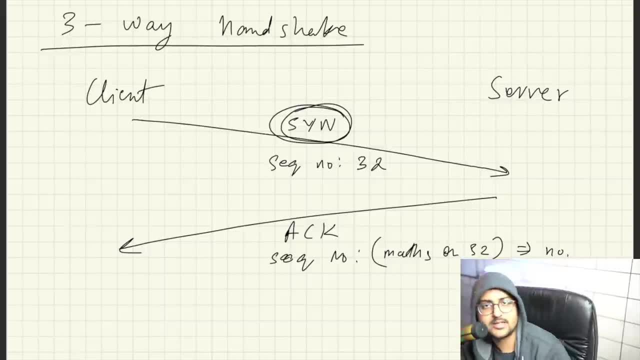 and that will give you another number that's going to be its sequence number 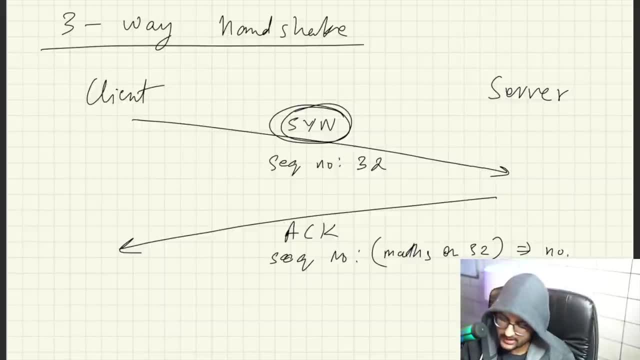 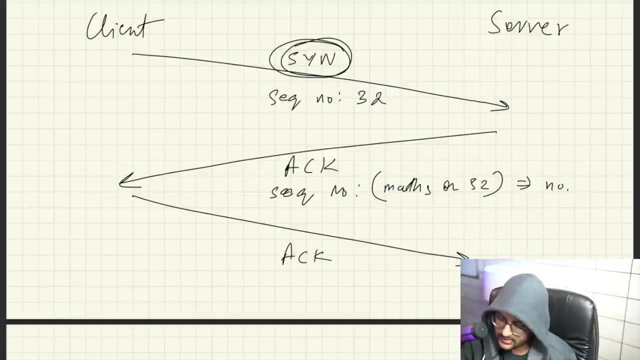 okay so that's how it works with its sequence number and then client will be like okay hmm um i have gotten it and i acknowledge it now client will again send the acknowledgement flag this will also send sin flag because it is also starting a new connection and then acknowledgement and uh the sequence number okay example let's say this is 56 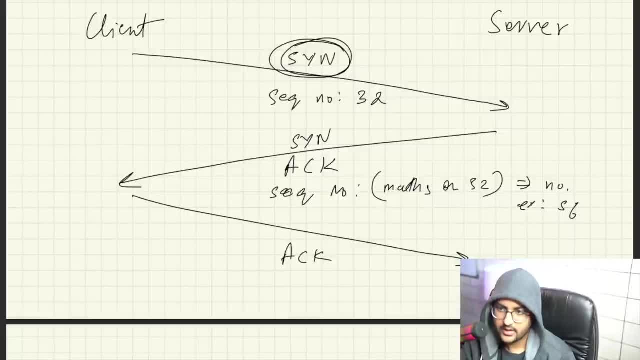 okay so it will send and sequence number first it was 32 the next time it sends a request will be 32 plus one sequence number will be 33. 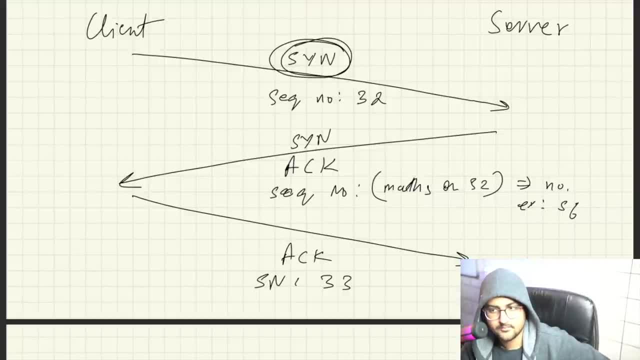 okay sound good cool it will also send an acknowledgement number there's a sequence number there's also an acknowledgement number acknowledgement number is equal to sequence number plus one previous sequence number plus one so 33 and here acknowledgement number it's going to be equal to what previous sequence number which was 56 um plus one okay 57 that's it and then the connection will be established and then they will be talking to each other 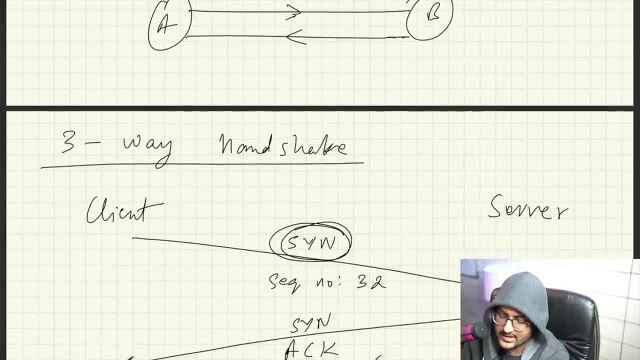 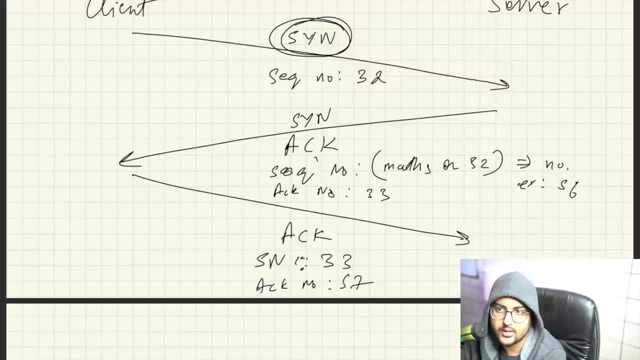 that's basically how it works this is a three-way handshake if you want to look into details what this header looks like i already mentioned it contains like the acknowledgement flags in flag there are so many other flags as well that you can check the you know internet for 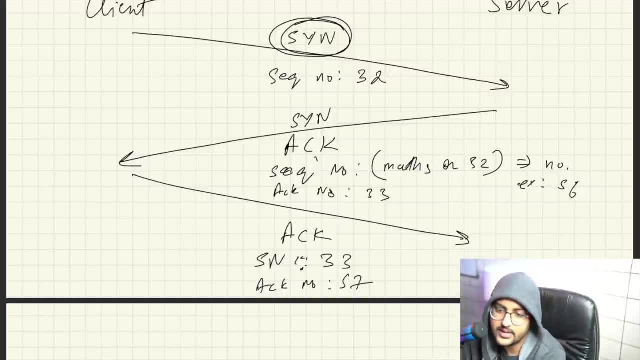 more more information uh there's the reset flag is there there's a finish flag is there right so all these flags are available over there so you can check it out and the checksum is also available 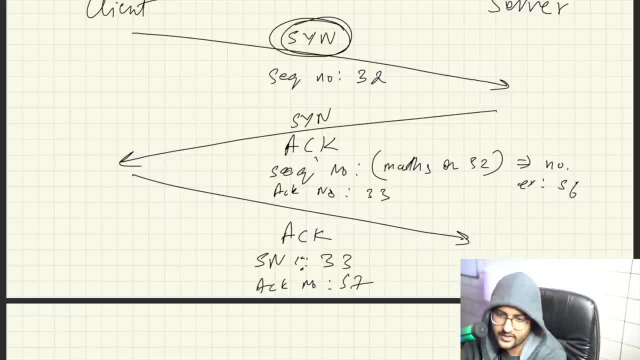 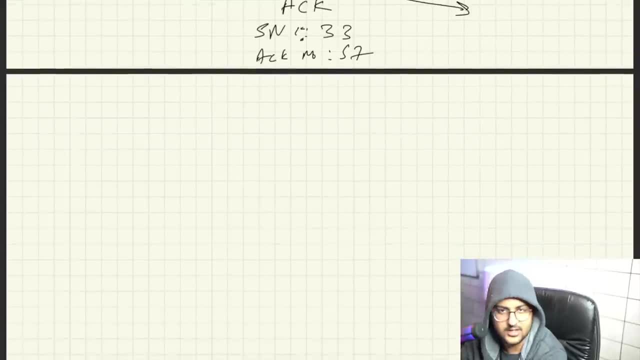 in this um which basically works in the same way and that's it okay so that was about tcp and i believe that was about transport layer also uh so that's it now let's look into the network layer 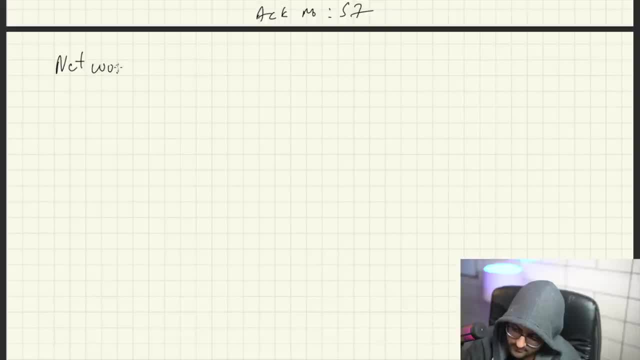 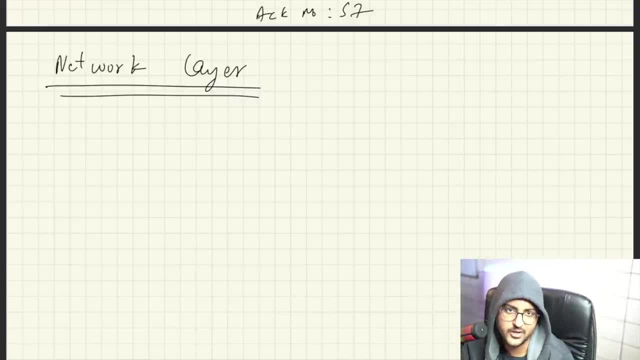 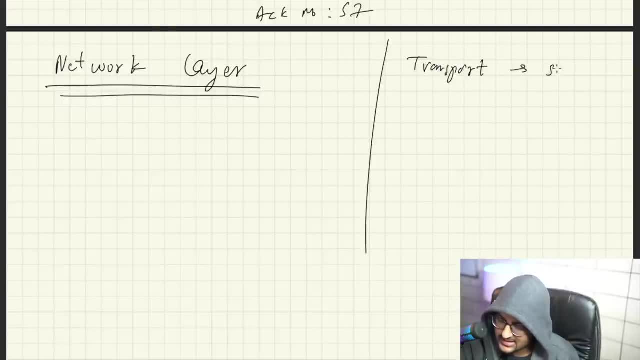 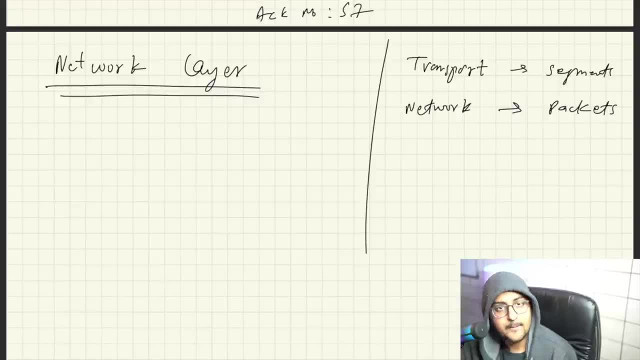 so the data we have the data travels in the form of packets and then the data link layer the data link layer has frames we will look on in all of these packets sorry segments have already looked into now it's time for packets and frames okay so what works at the network layer routers here we work with routers so here we work with routers this is the network layer that our team is proofs talent and now grey and blue so here we work with Line similar 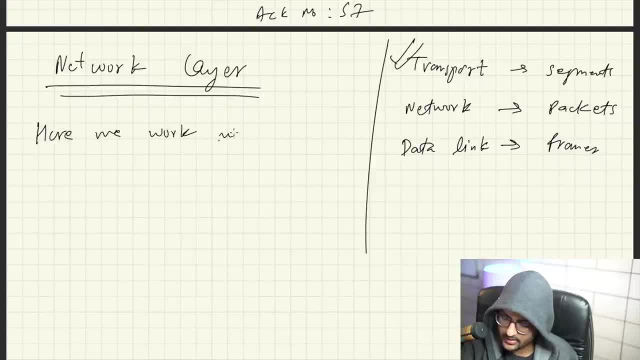 to the same line complete options where they work with 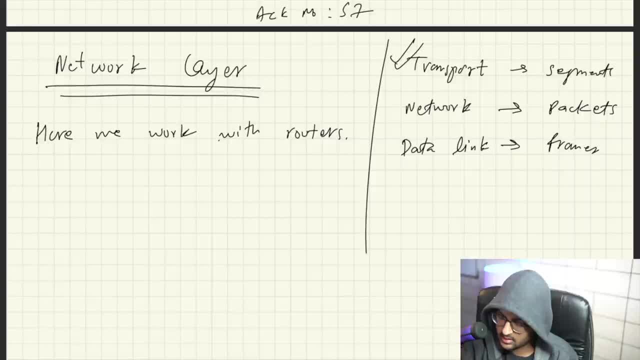 with routers okay we've already covered what routers are so basically this is the part where your data actually travels from one place to another we be that like across the world 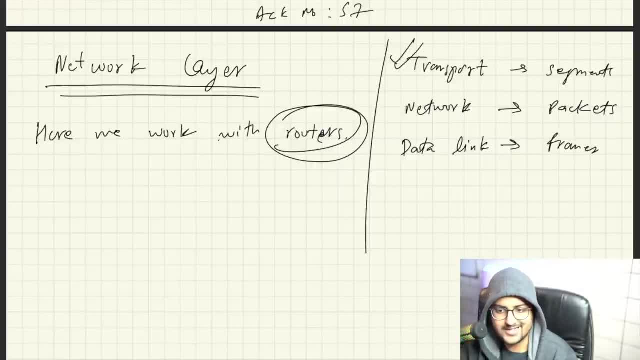 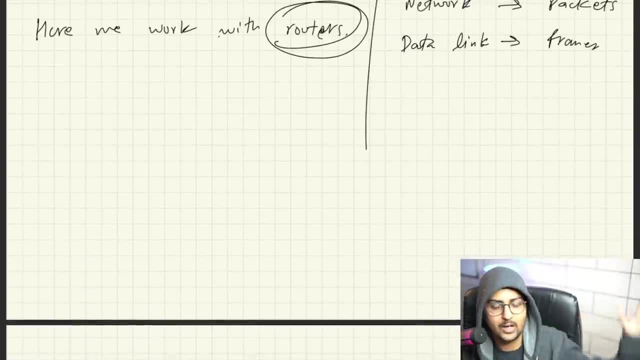 okay so that is pretty much about it and let's say how let's see how we can uh how we can do that okay so let's see how it happens so when we're talking about routers let's say so many routers 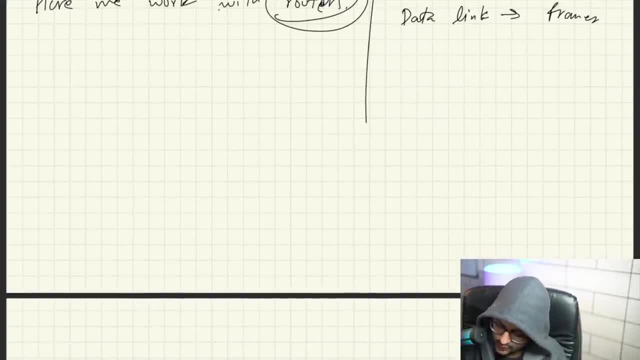 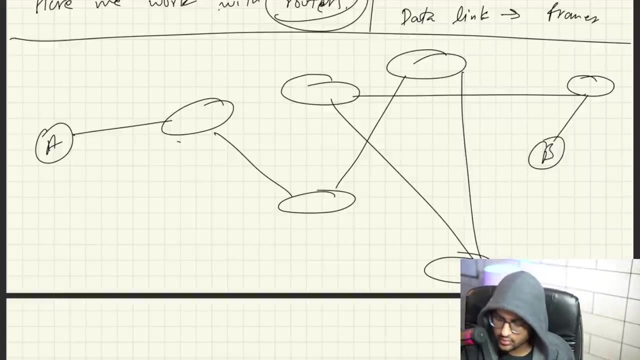 are router and everyone is connected together and you are let's say over here let me just erase this thing um just give me a second and let's see if we are over here somewhere okay um okay so you are over here your friend is over here point a point b you have to send data from computer a to computer v okay so many routers are connected in between so many routers are connected to each other so many routers are connected like this something like this okay many routers are connected to each other sound good this is basically about it so what happens is that uh this entire internet thing 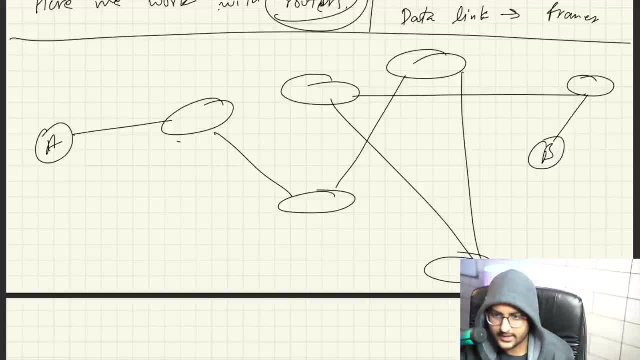 okay just like literally like the global global internet um every single router that you see over here has its own router its own network address so every device we know has its own what ip address mac address 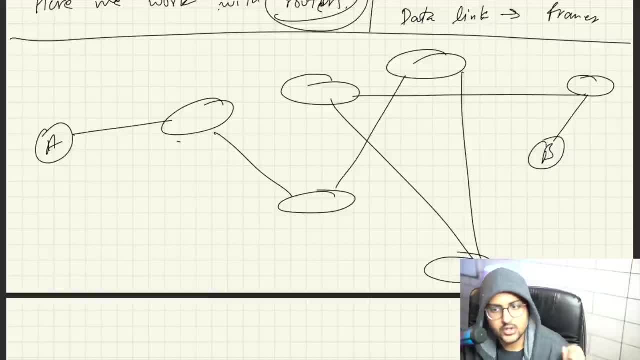 so these also have their own network address so network address basically means that it 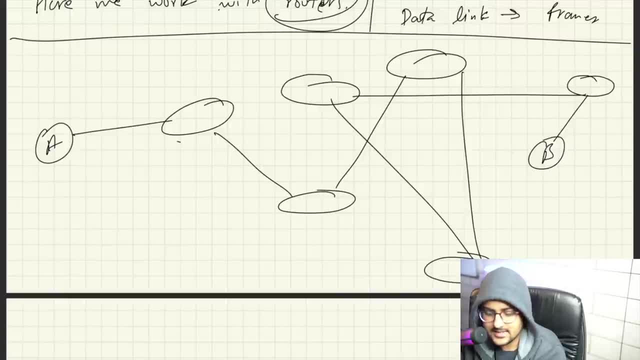 basically allows us to send these like data packets so if you're sending a data packet over here you send it to this one network one for example so what this network one is going to do it's going to check in its routing table okay it's going to check in its in its routing table or forwarding table forwarding table is a part of a routing table that basically consists of every destination address okay so for example let me explain it to you i know it's a little bit confusing but let's see so what does a packet contain let's first look into that so it will contain the network layer address of the destination it will contain the network layer address of the person who is sending it and what information you want it to send okay so when you send your packet over here you send your packet from here to here this will check this router will check it will check its forwarding table you're like oh i have received this packet uh and this packet needs to be at this particular location let me just check my forwarding table real quick let me check my forwarding table oh this this particular destination it's uh somewhere around east so it will send it over here like this this is known as forwarding table so routing table forwarding table don't get confused in this this is known as hop by hop forwarding hop by hop forwarding 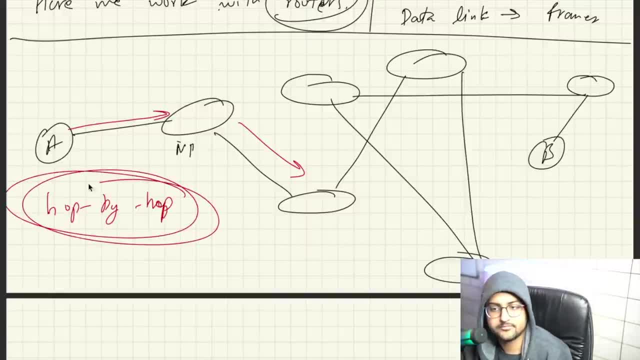 hopping routers to router routers until it reaches the correct router okay so this will be like okay i have received n1 will be like n1 router uh it will be like hey i have received a packet is this packet for me it's gonna be like uh packet is gonna be like no it's not it's actually for some other destination 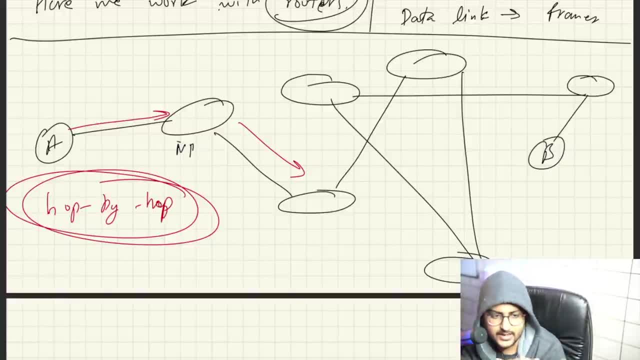 network layer address it's gonna be like oh okay then let me see where that is in my forwarding table you're like okay let me just check it and then it will move ahead 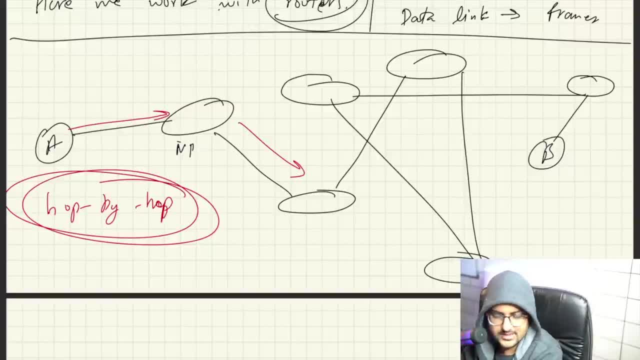 okay sound good so this forwarding and these routing tables actually live inside your routers 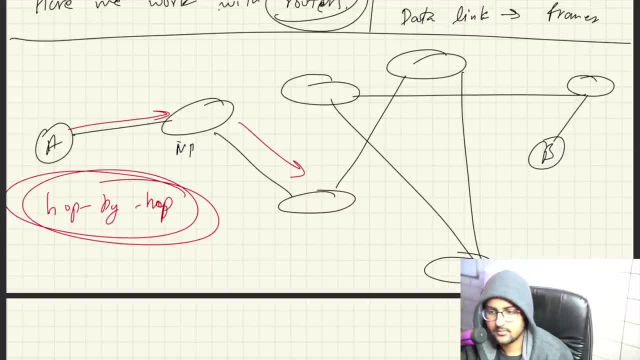 okay sound good good okay so forwarding table comes inside a routing table a routing table may have multiple paths if you want to reach point number c okay how do you reach point number so you can go from here from here from here all this information will be available in routing table and what is forwarding table forwarding table only contains one path okay it will be like 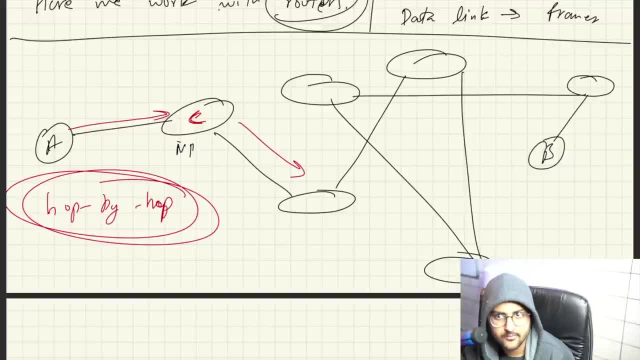 from here to here check it so it's a much much more faster way okay and it's uh it exists inside your routers these forwarding tables and stuff okay so forwarding table is just a data structure 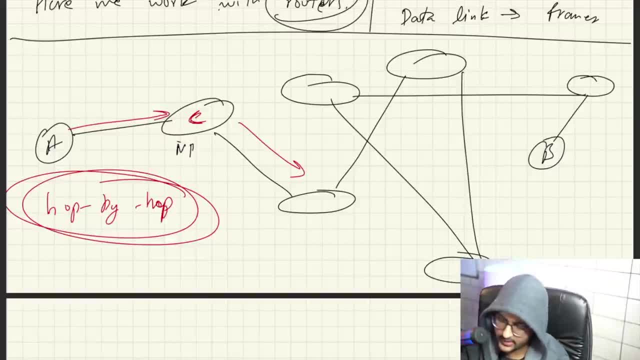 okay okay so like hey please send it the data over here and like okay let me check if this 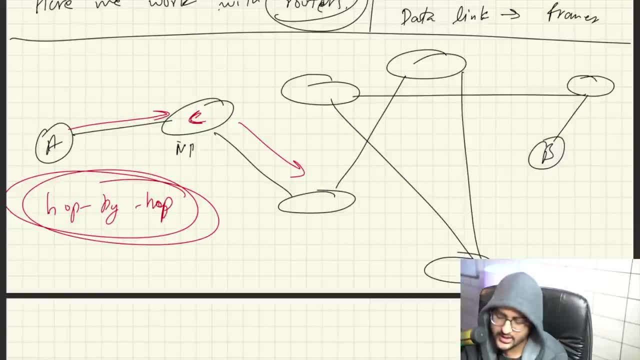 data is for me it will be like no it's not okay send it to your you know check in the forwarding table it will like okay forwarding table is saying that this particular ip address is somewhere over here it will send it here then it will send like let's say if these were connected also let's say if these were connected also it will send here it will send it here and data will be then received okay so every single router will have its own network layer address okay every 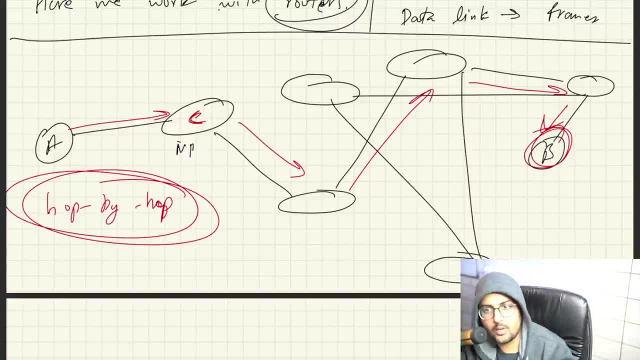 device has its own mac address but when you talk about the network interface um it also has its own like some some some logical address are being being created 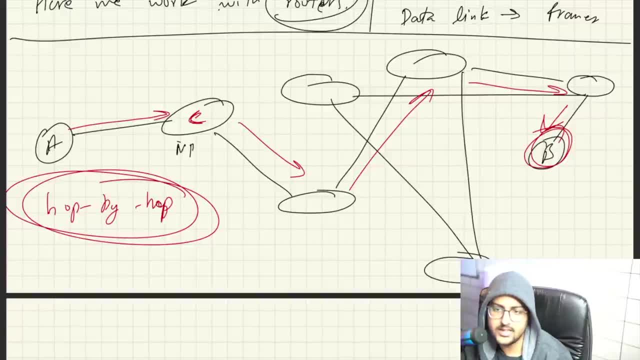 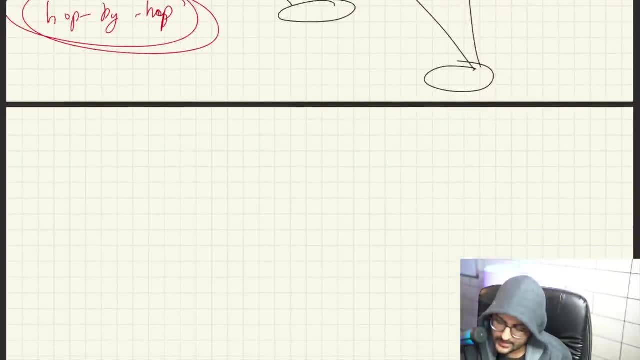 okay cool so that's basically what we mean by it let me explain it to you so there may be a particular network when we talked about ip addresses we talked about ip addresses right they're like there's four parts to it let's say one of the parts is like 192.168 point 2.300 and 0.30 or something 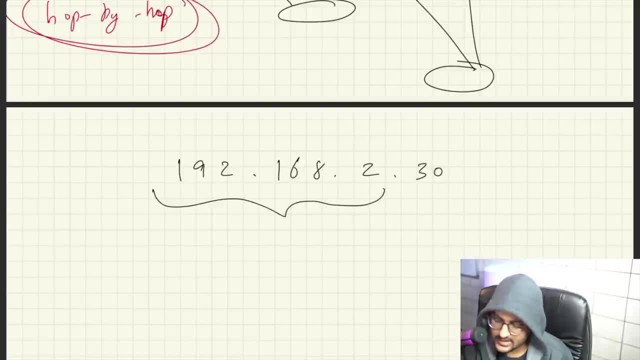 okay something like that so this thing is basically known as the network address of your device network address it basically tells which network your device resides in and this is the device address okay i hope it clear now we'll obviously look more into ip addresses later on ipv4 ipv6 and everything will cover it 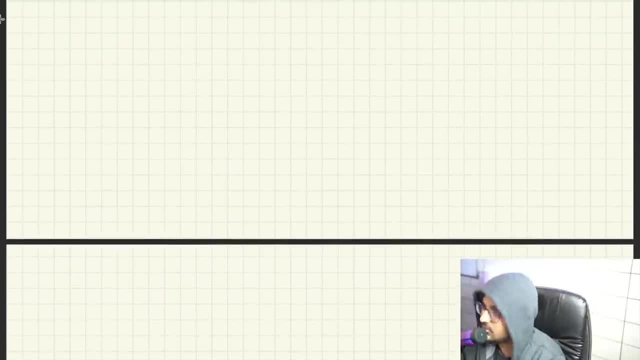 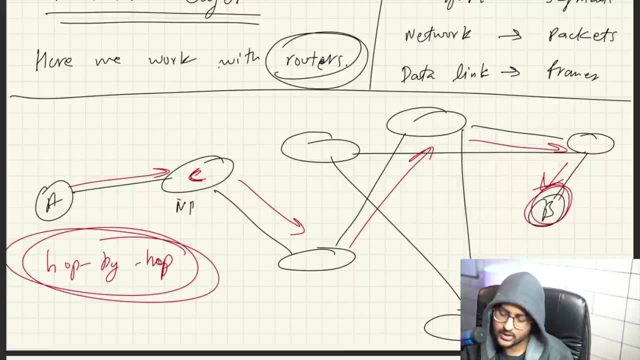 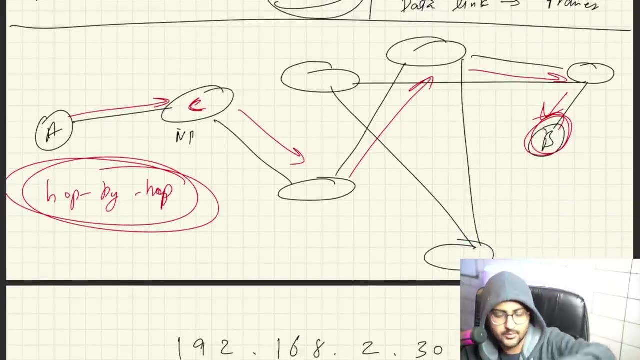 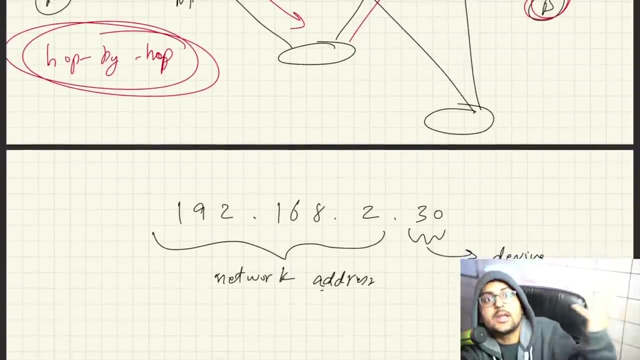 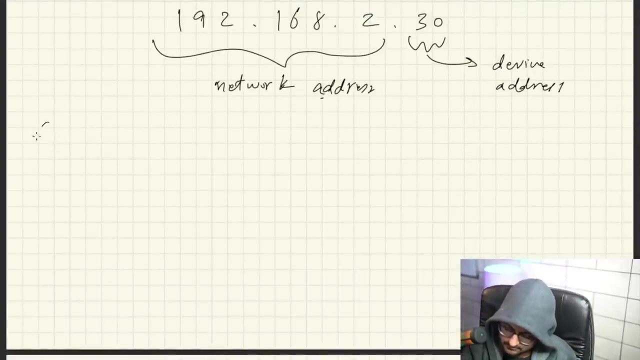 and this is how routing takes place okay now another important doubt you may be having kunal that is fine you have your routing tables in your routers and that's trying to forward things over here and here what if someone adds a new router in there you know some some locality or whatever you wanna you would that be included in the routing table also how would that be happening and who creates these routing tables who is adding these destination addresses and everything how does my router know where to forward data packets or whatever who is creating these tables you know how it's working but who created these tables where did it come from okay so who creates these tables control plane in the network layer there's something known as control plane so what happens is that control plane is used to you know build these different networks right so when we talk about the these routing tables and every router you can think of it as a graph okay so every router is a node and the links between the routers are edges of the graph okay routers are what very very big graph you can imagine it these are the nodes of the graph if you are not aware of how know what are nodes and graphs and all these algorithms then please check out my DSA Bootcamp, i will be covering it over there , so routers are nodes and the links are the edges the links between routers are the edges okay so there are two types 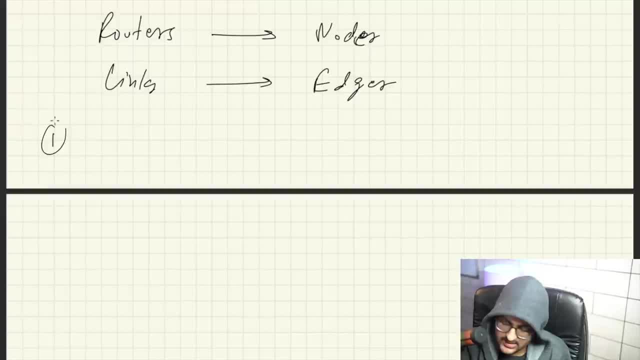 of routings that you use to create the tables first is the static routing this is basically adding addresses manually . Now obviously this is a periodic table like these are each pairs of physical tables , here those are the Sexual tables where you are adding lateral and Edu eliminal 위에 , these areShares which are those making the Arenas and All the scopes, that's okay, so all that ends there like this one to the notes also and we have just shown you its names but 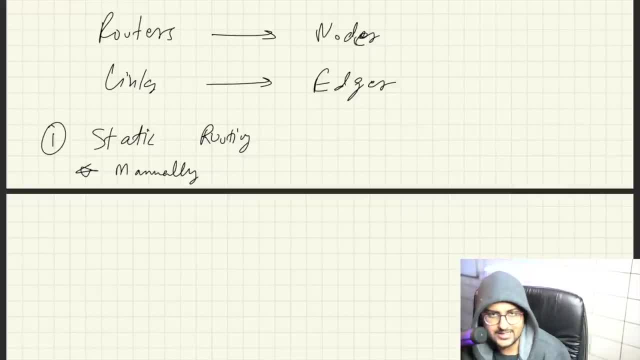 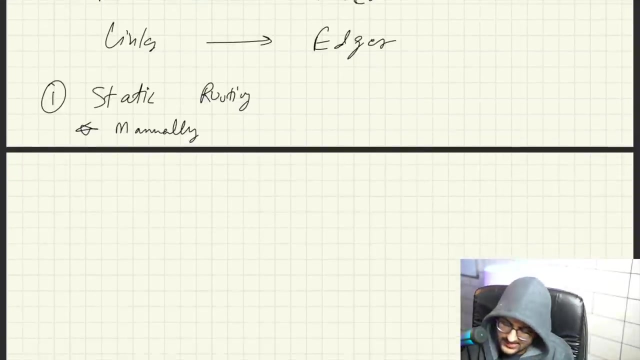 time consuming and uh if a if a new address is added then you would have to change that it's not adaptive really okay so that's basically static routing you manually add all these routes okay if you want to go to this network address then you go it via over here here here you add it manually in the routing table okay cool the second one is dynamic routing 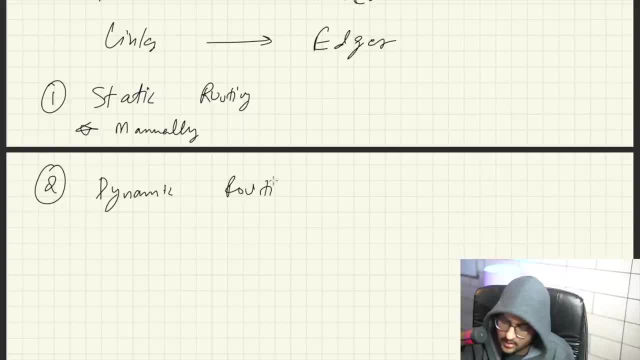 dynamic routing this sort of like evolves okay when there's a change in network it will evolve accordingly okay the algorithms they use are somewhat like this you know bellmanford dixtra pathfinding algorithms they have that those algorithms have been used in finding these paths to various algorithms and routers literally dixtra's algorithm has been used in this so some people ask kunal what 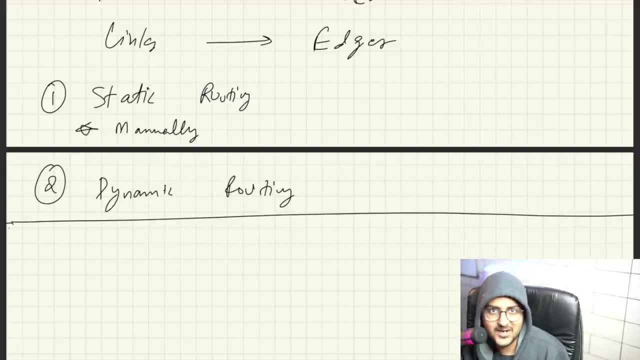 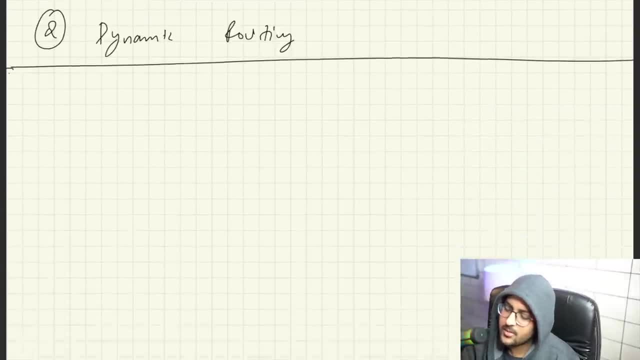 are the uses of these algorithms we are learning in data structures the entire internet is built on that all right cool sound good okay now let's talk about protocols in application layer we 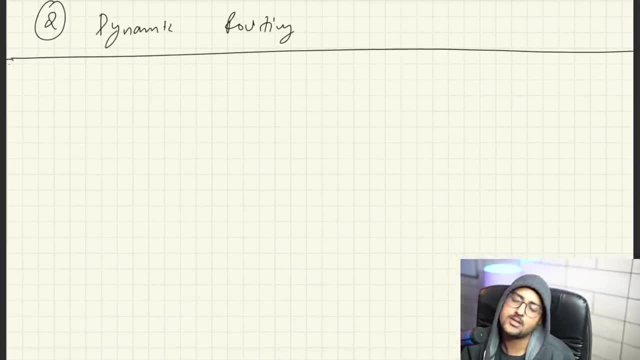 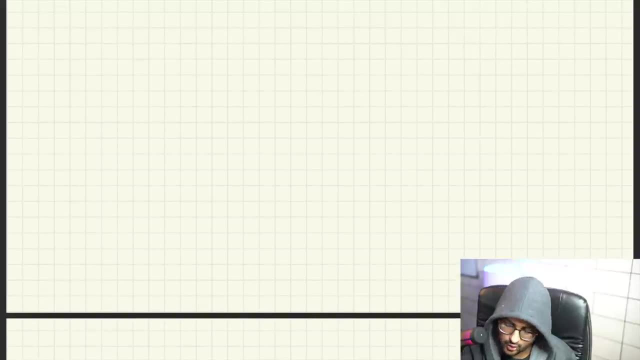 talked about protocols transport layer we talked about two protocols tcp and udp um there's one more protocol in the network layer that takes place which is internet protocol or ip so what is the network layer protocol if someone asks you it's the internet protocol okay ip so internet protocol here we'll learn about ip addresses internet protocol ip okay now what is the internet protocol you know when we talk about the tcp ip model that we talked about the entire five layers that we were talking about in that the ip part is the internet protocol so it basically is the network the protocol that lies in the networking layer 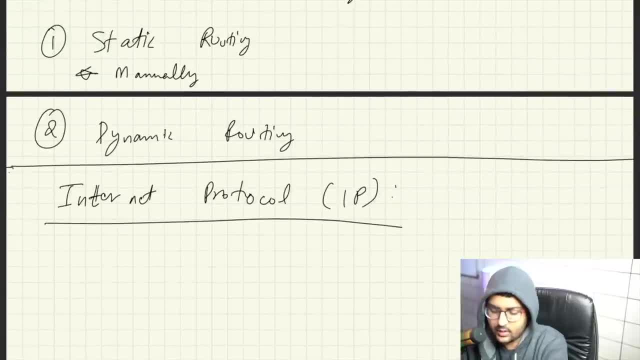 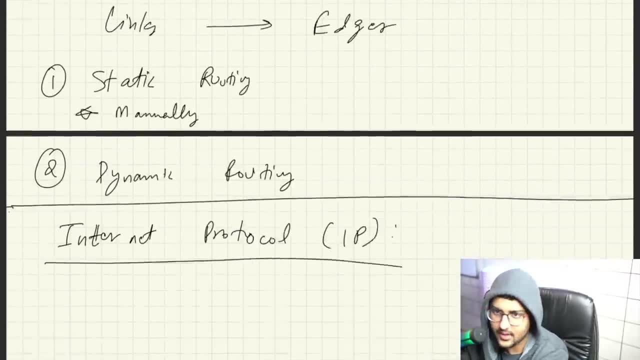 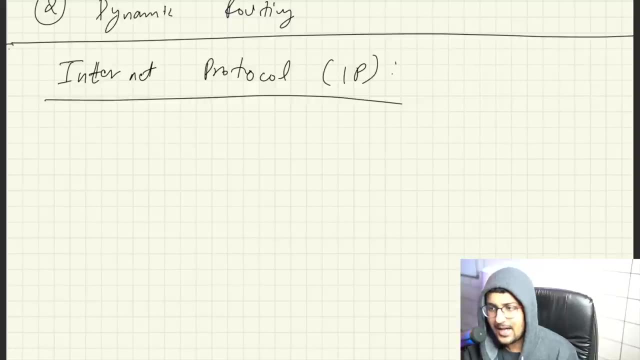 it we here we work with like you know how this uh this thing the the routing stuff that i'm mentioned happens uh this uh the control plane stuff and the ip addresses mainly okay so these are known as ip hosts okay so this is known as an ip address so ip addresses basically let's talk a little bit more about that first so i will talk about ip addresses what are ip addresses currently we are talking about version 4s okay we'll talk about version like uh the six version six uh later on first let's talk about the ones that we have been using so far so ipv4 ip address 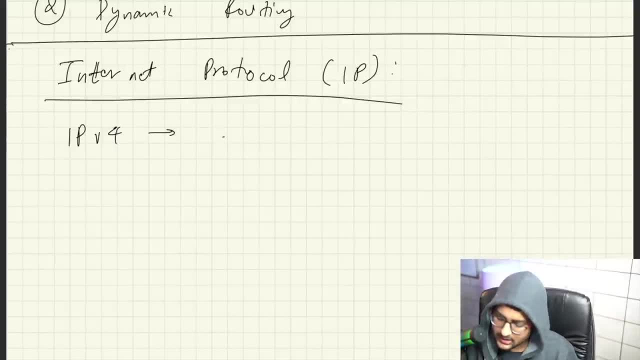 version 4 let's talk about that so these are 32 bit numbers okay with four words okay what is an ip address we already know it defines a server a client a node or a router 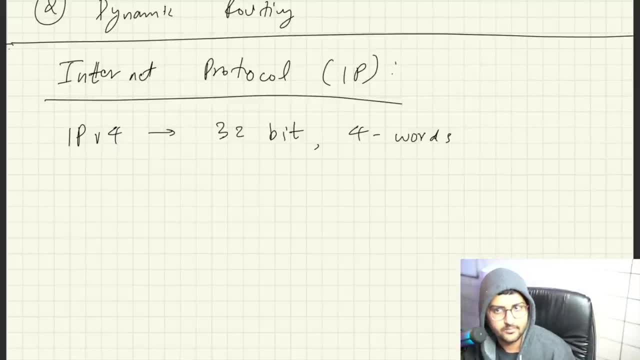 okay uniquely defines okay what is ipv6 this is the future okay so basically 32 bit may be like uh even though tourist for 32 unique numbers that's a lot of numbers right but uh still it may be possible that some someday we run out um that's why we have like some more you know features and additional functionalities and ipv6 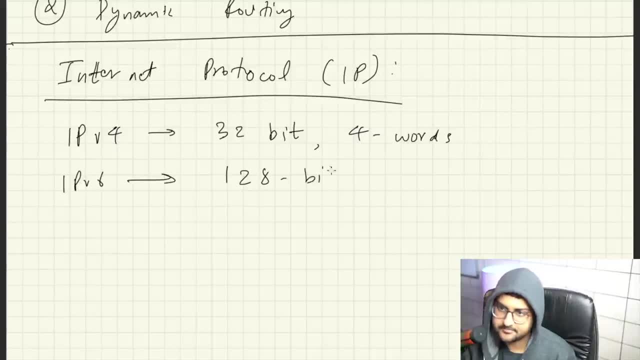 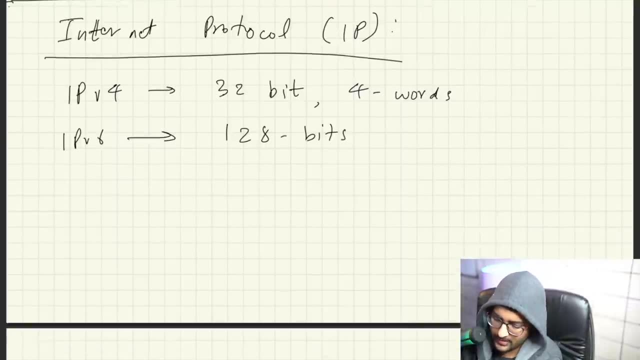 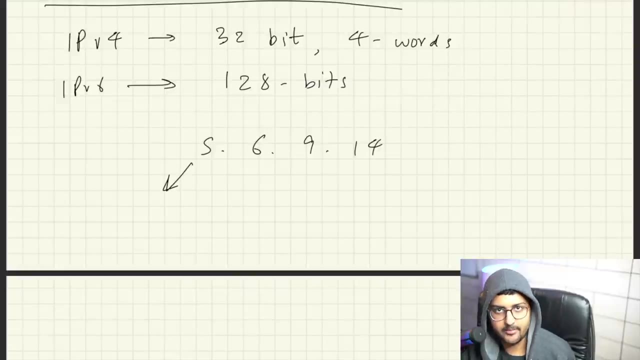 addresses these are 128 bits okay so we'll talk more about that later okay so when we talk about like ip address 5.6.9.14 so this is an 8 bit number okay this is another 8 bit number 8 bit number 8 bit number 8 4s are 32 so what is 5 in binary 5 in binary is 1 0 1 0 0 0 0 1 2 3 4 5 6 7 8 8 bits okay. 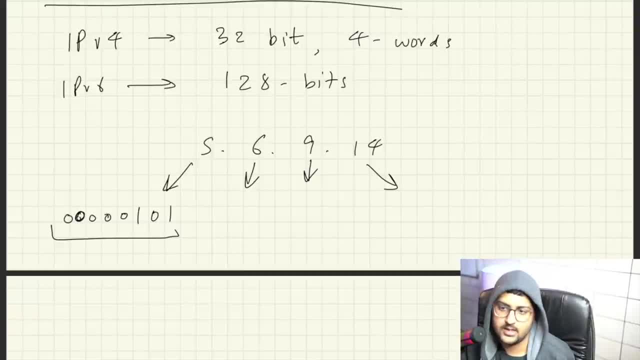 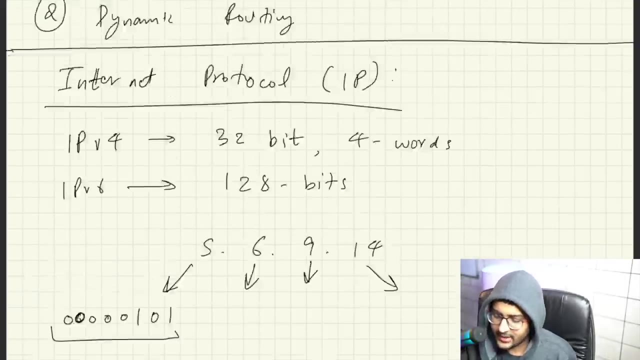 8 bits here 8 bits here 8 bits here that calls a you know an IP IP address okay cool now let's talk about it like we know that IP addresses are like you know used to identify your devices or whatever but when I told you about this hopping Kunal one device will go over to another to over to another to another so 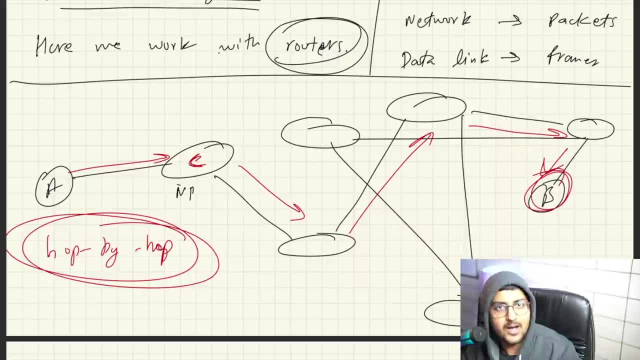 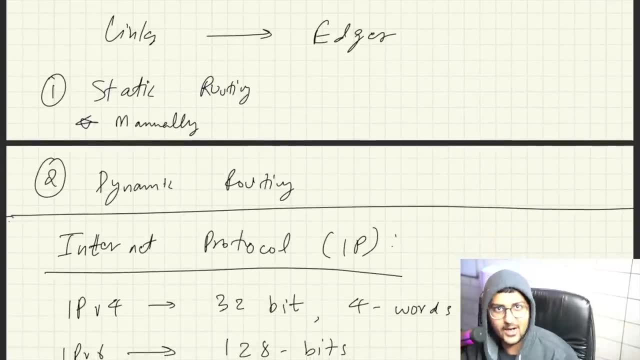 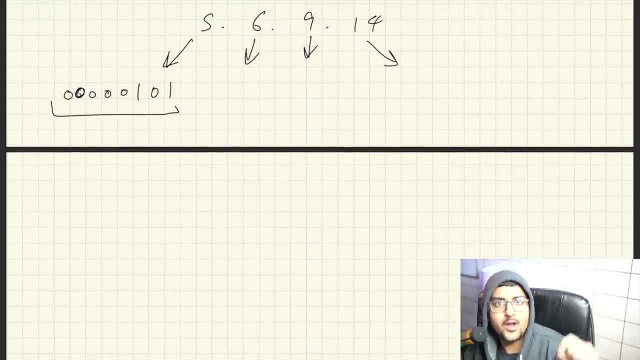 is it like my router in my house takes part in this hopping is it like you know I am serving someone else's traffic also is that how it's happening the answer is not really so what happens is that instead of hopping on your individual 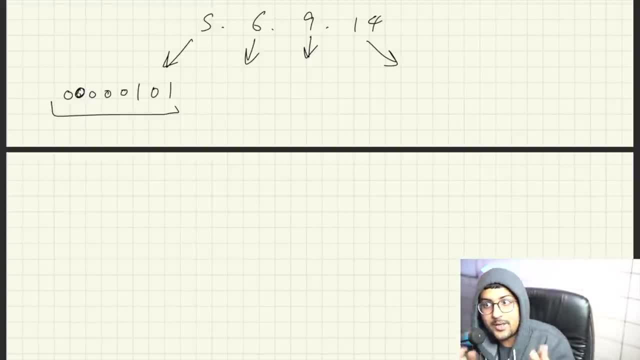 routers this routing path you may be confused Kunal this does not seem like doable you know it's like all of our devices are connected like you know one another my router is connected to my neighbor's router is that what you're saying in a way you can you know make that connection but the routing like this hopping things Oh actually happens over the internet service providers okay so the routing table and stuff that I mentioned it does not have like every single information of every single person's router in the world that's not 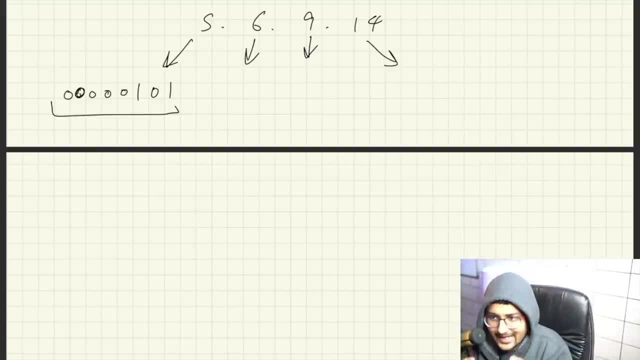 like how it works so the basic idea is that it has blocks of addresses not individual addresses blocks of IB addresses okay and these blocks of IP addresses are assigned to the internet service providers like Airtel Reliance Tata or whatever okay 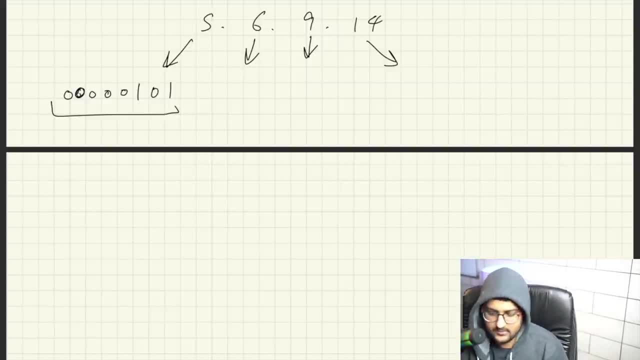 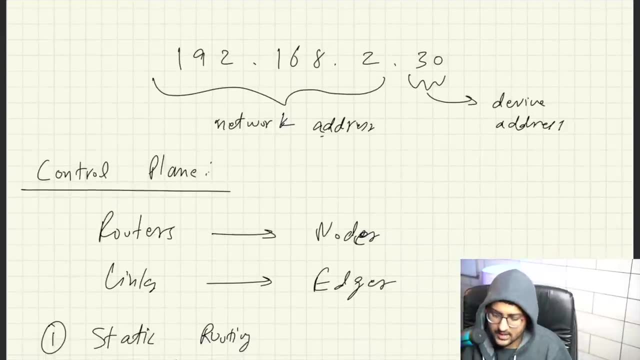 this is known as what subnetting this is the thing I told you about right over here this is the network address and this is the device address so 192 point 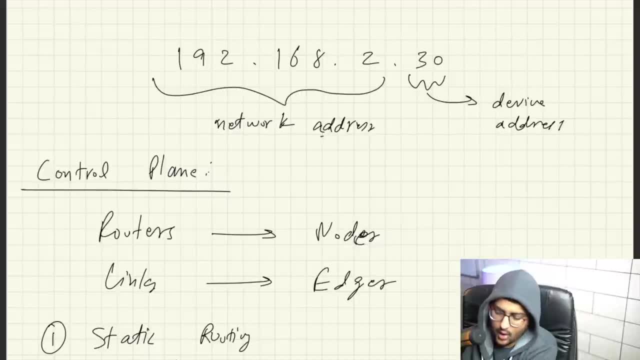 1 68 point 2 point something so all the devices that are in the same network will will start from 192.168.2 all the devices that are let's say in airtel for example 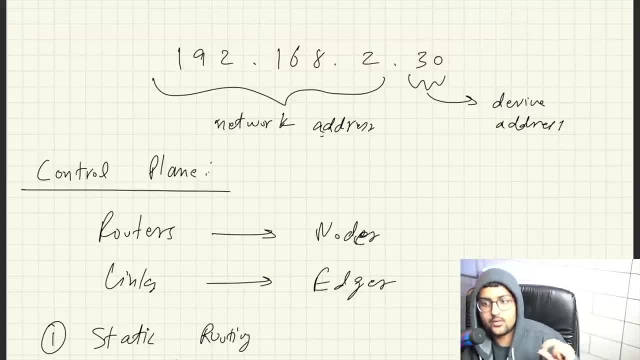 in simple terms okay these are known as subnets so this is the subnet id this is the host id host id means host 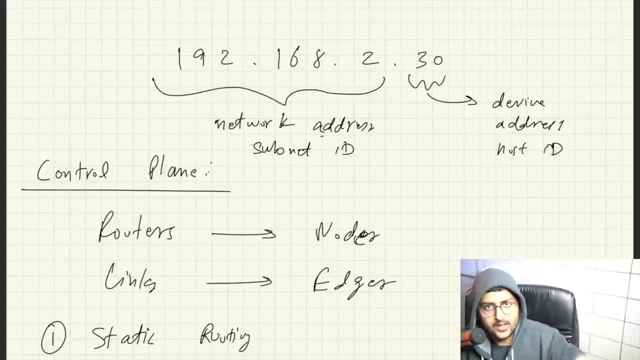 okay sound good so whenever a router will forward a packet like this it should know the subnet of the destination 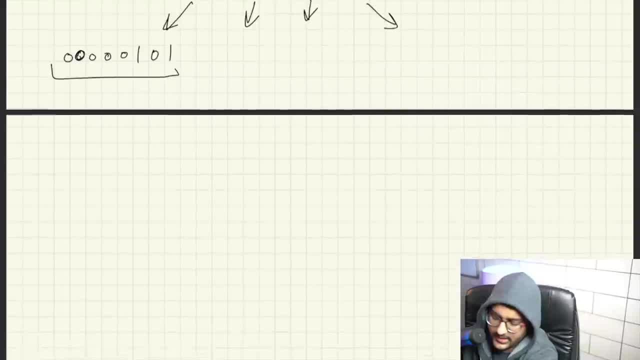 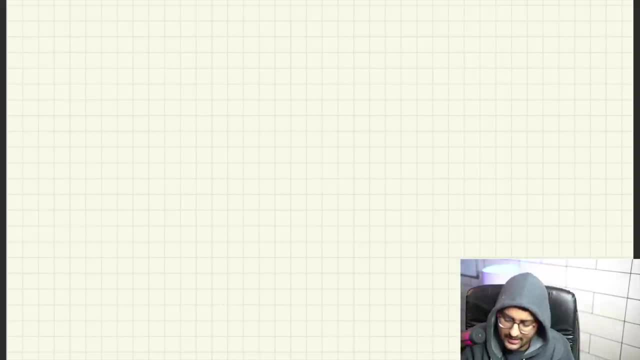 okay cool so the internet society or whatever they created classes for this okay they created classes for this so there are three types of like class address you can say ip address of class a is there class b is there and class c is there 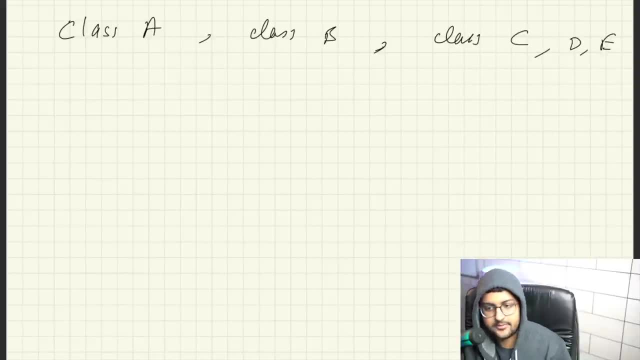 there's also class d and e d and e are also there 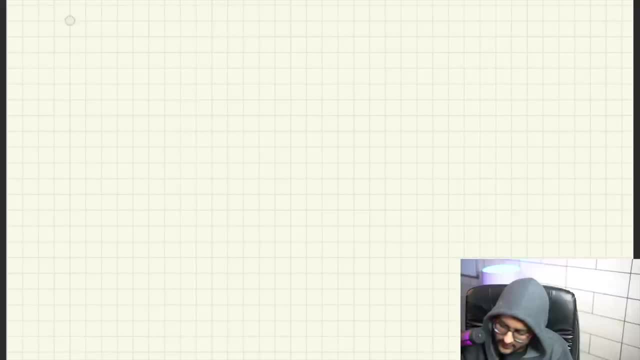 okay let me just write it down in a knight's way class of ip addresses the class is just a basic range class of ip addresses 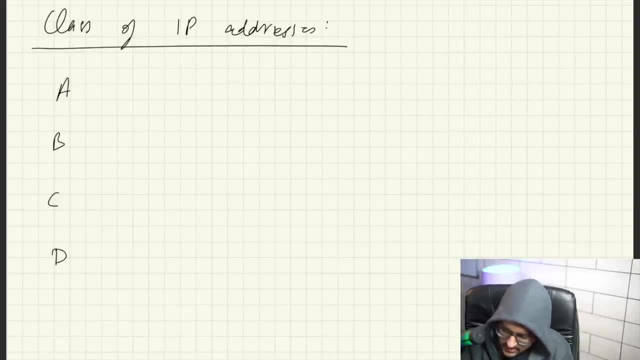 so i'm talking about class a b c d e all the classes starting from like zero zero zero zero two three 4 see there is a 3 point so this is just your basic 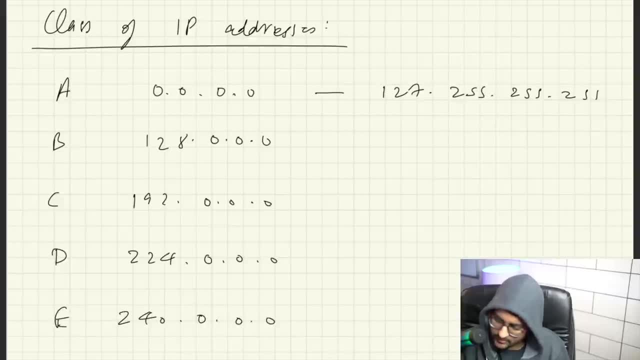 so this is this is my main point we're going to move into the third parameter which is the set computers somehow so let me open this up嚥 to 127.2 what is the maximum value 255 dot 255.255 and then we have 128.0.02.0 then we have 192 points then we have 224. 0.0.0 and then we have 240 and then we have 240.0.0 starting from 10 to 192-11191 223 223 227 226 questa sab applied till this until 192-190.01.20 7 until 128.0.01.0 starting from this back 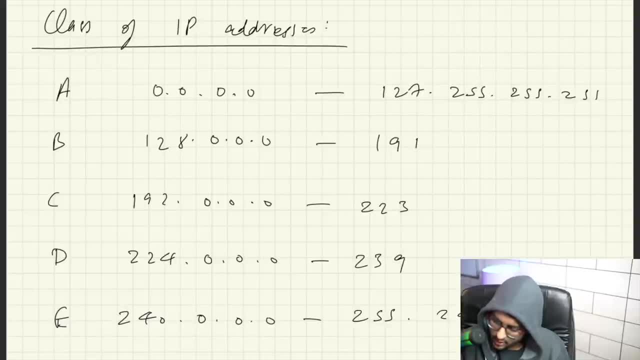 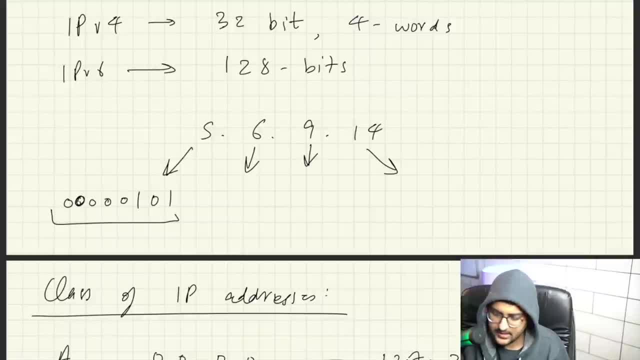 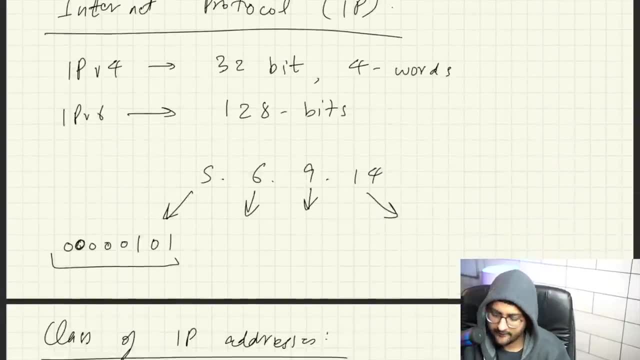 network address network address we already already mentioned right that last last one will represent the you know your host address and this is the network address the first three 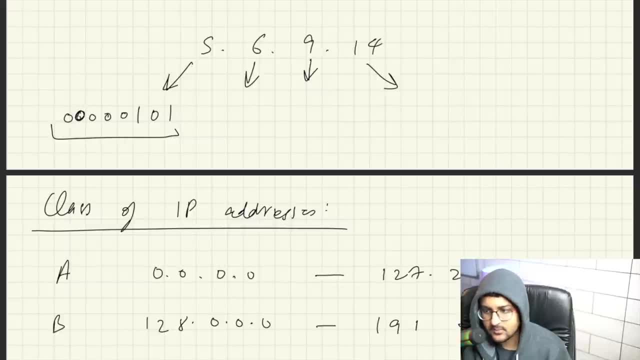 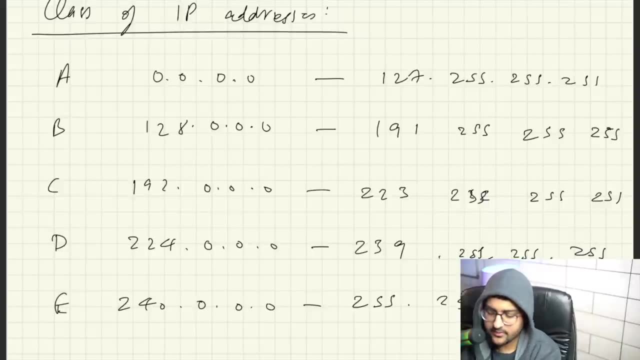 numbers okay sound good cool all right okay now comes up comes into picture one more thing called subnet masking okay so what is subnet masking subnet masking basically means that um that 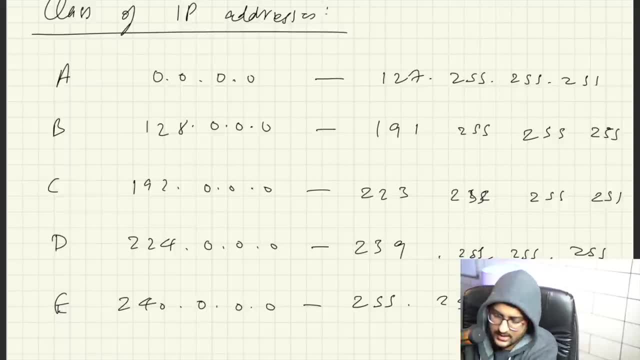 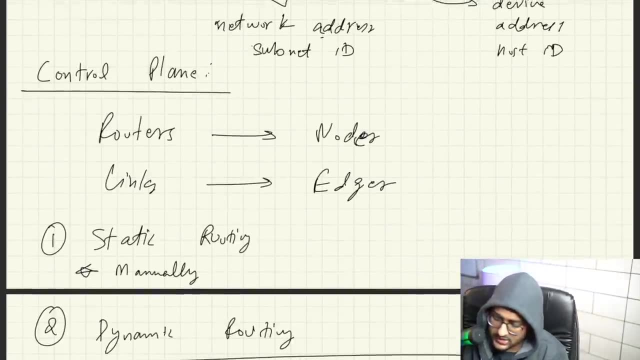 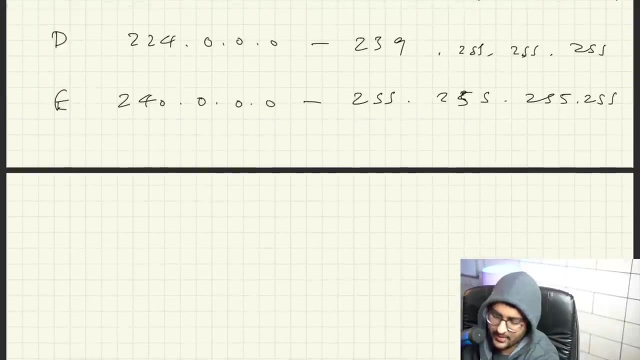 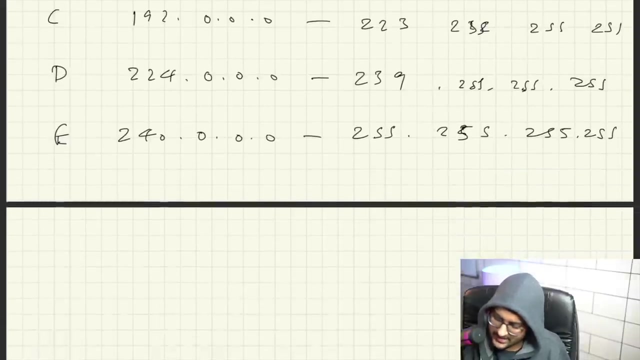 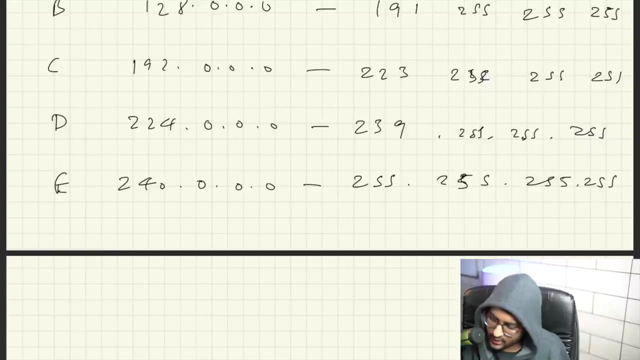 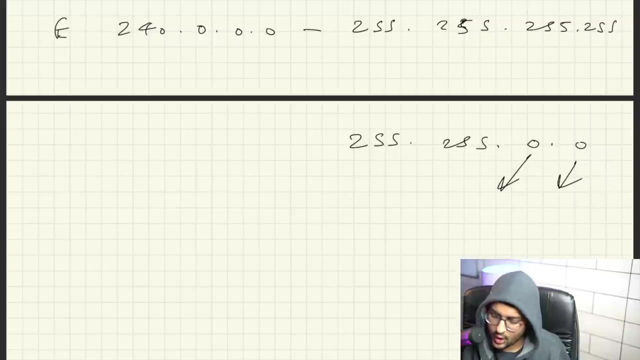 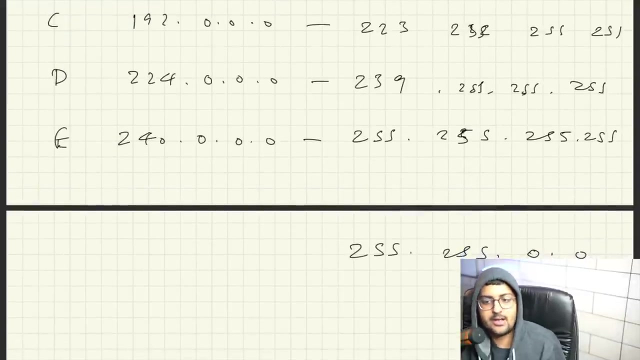 the subnet mask is going to mask the the the network part of the thing that we talked about okay the ip address network part of the ip address and it will leave for us to use the host part okay the device part so for example if i have an ip address like a network part of a of a of this ip address for example class c so class c ip address basically means that if we only want to have this thing so for example a subnet mask for class 3 is 255.255.0.0 that is basically what it means okay meaning i can add any numbers over here so all the devices that will be 255.255. any numbers over here that means that it belongs to ip address of class c 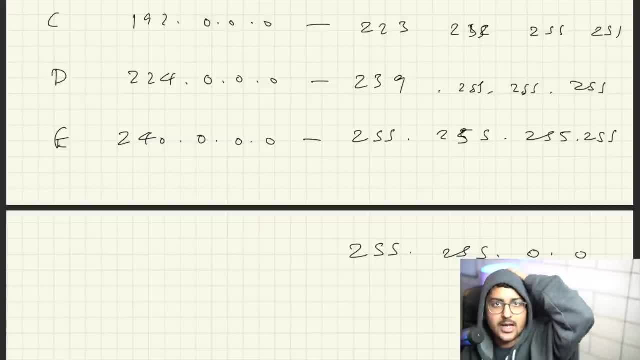 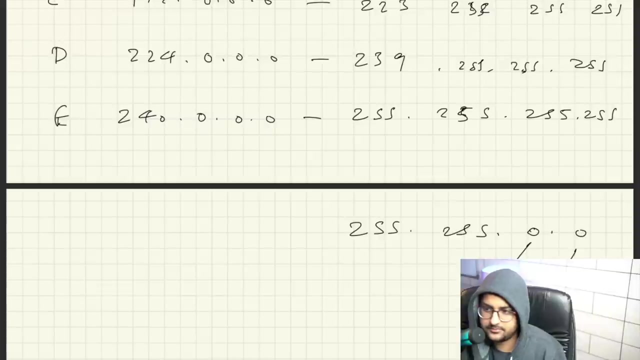 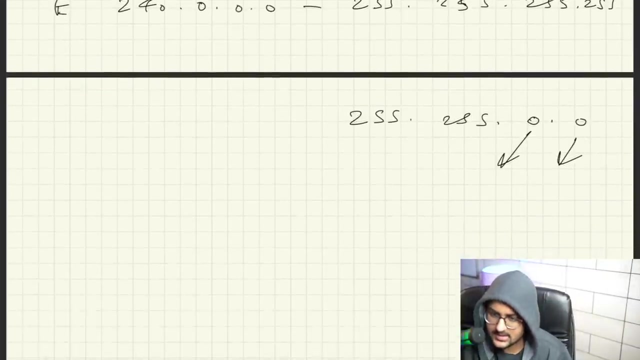 so don't have this confusion canal why are we using ip addresses classes or whatever because we want to be able to tell which particular category it belongs to okay sound good okay there are also like variable length sublets available okay but we can look into like uh into that later on all right okay so what do we mean by variable length subnets so variable length subnet basically means that uh you can set 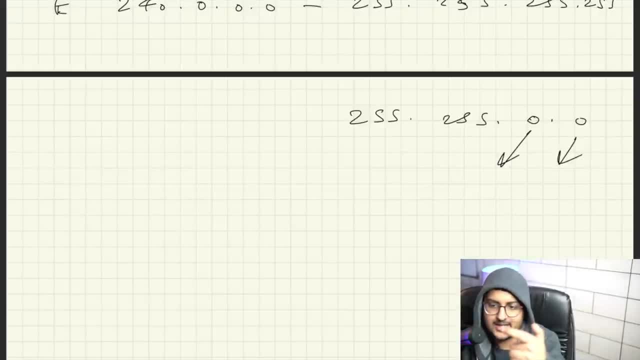 your own subnets to be able to tell which particular category it belongs to and which particular category it belongs to length of the let's say the network 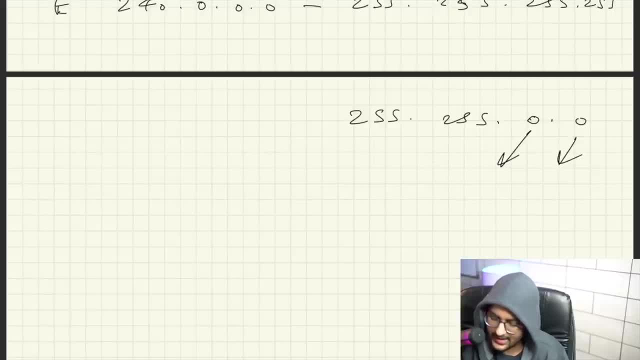 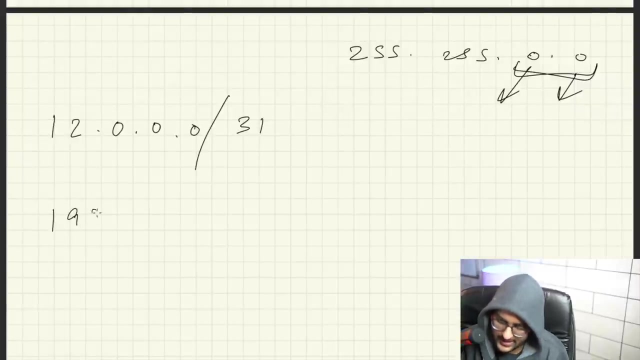 subnet network okay so example here it's saying that you can add items over here and here numbers over here and here so if you have a subnet like this one two point zero point zero point zero dash thirty one so this basically means that first 31 bits are basically my subnet part okay rest remaining remaining okay sound good so example if you have something like one ninety two point zero point one point zero twenty four so 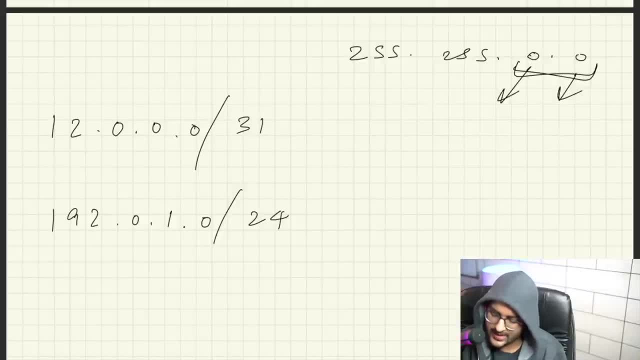 totally have 32 bits uh 24 are already occupied by the subnet remaining eight okay so starting will be what starting of the address that you can have over here is the first eight would be the same first first 24 bits would not change because these are the subnet 0.1.0 ending will be and then you can have zero point 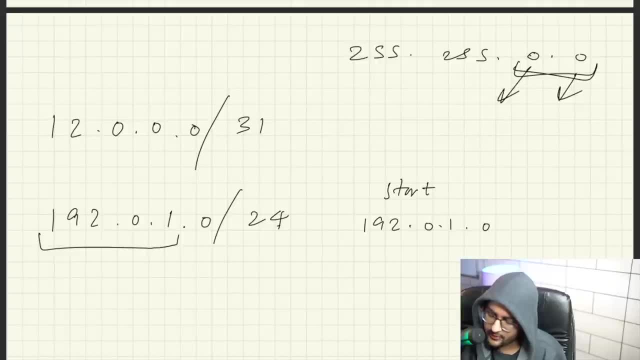 nine one ninety two point zero point one point one one ninety two point zero point one point two so ending can be one ninety two point zero point one point two fifty five total how many do you have 256. so if there's a subnet of size 24 bits then remaining bits are 8 so you can have total 256 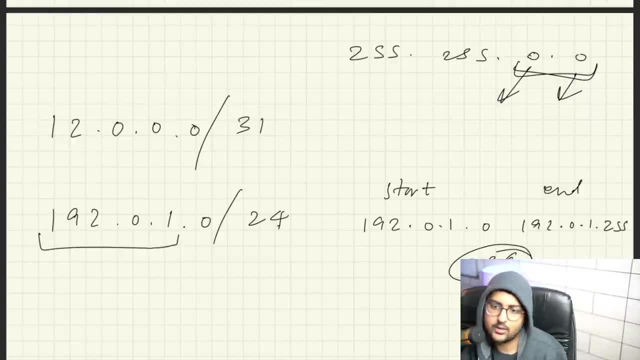 to each power eight okay that's basically what a subnet is and this is how it's allocated to ip addresses but another question is how do we allocate it to ip addresses like who allocates it okay how do we allocate which particular ip sorry uh not ip addresses um 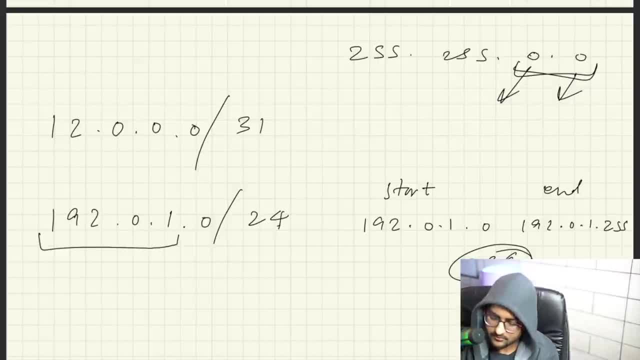 internet providers isps okay so initially what was happening was that it was on first come first serve basis 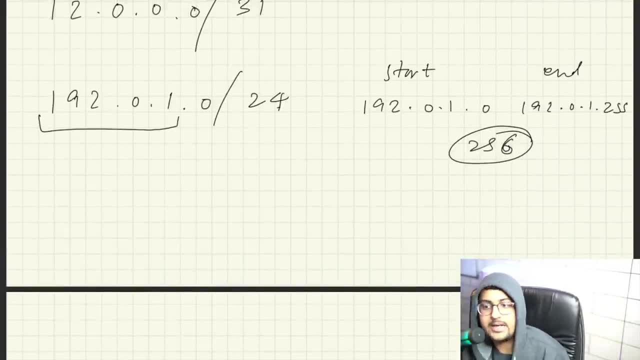 okay so larger bigger bigger organizations like there was uh mit and stanford and stuff and you know ibm was really pop you know really popular in terms of like the internet age so they all got the class one ip address block okay this one 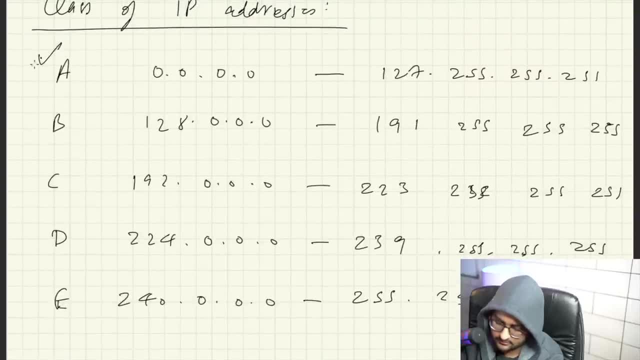 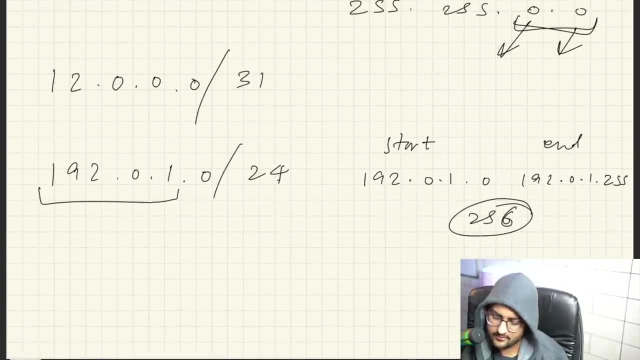 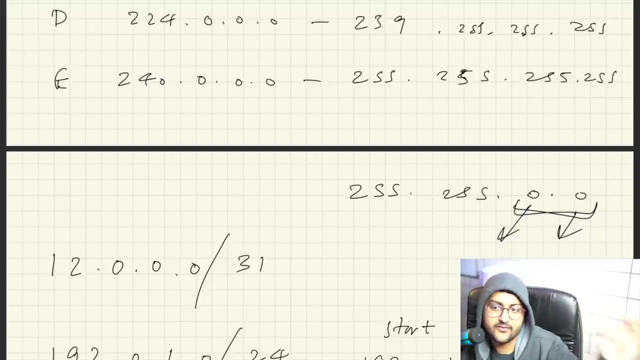 this one okay so it was on like first come first serve basis but then what did they try to do they say well like okay we are not going to worry about these classes and structure we are just going to focus on uh this thing the you know um like we are not going to worry about like the variable 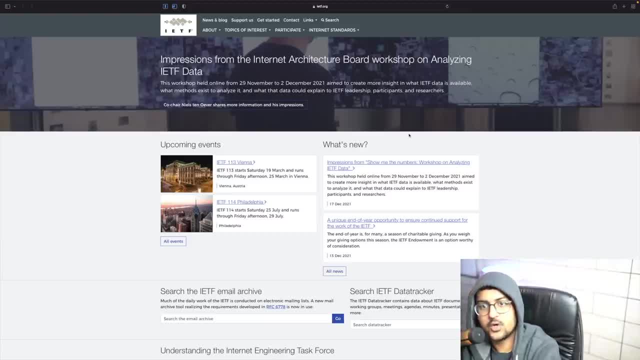 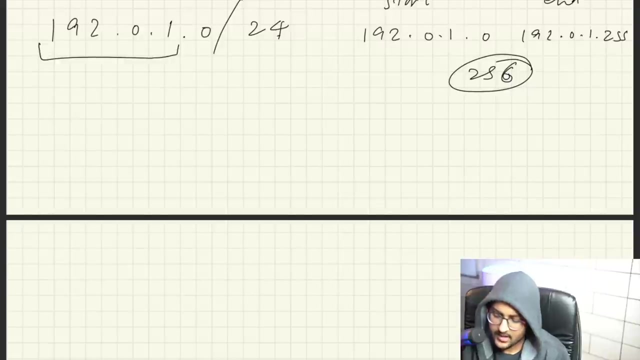 length uh subnet masking we can work on that okay so the internet society uh the iet if uh they are the ones um the internet engineering task force okay um so they are the ones who assign these ip addresses to your isps and stuff okay so they don't worry about the classes or whatever they are just like we are going to assign the ip addresses based on regions why because they want to minimize the number of let's say hops when you're finding your ip addresses and stuff okay so that's one of the reasons why they don't work with like you know they don't want to assign it based on classes they assign it based on regions all right okay some of these ips are important ips are are important in electric energy education and late Shooting. 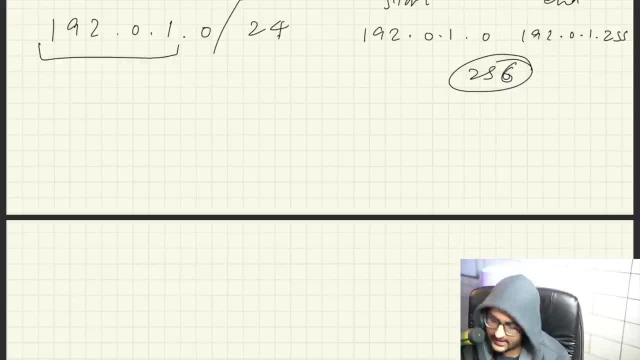 v4 addresses that we're talking about are reserved they are like special addresses for example uh the first bit is reserved to let's say uh like special one or reserved ones let's talk about this 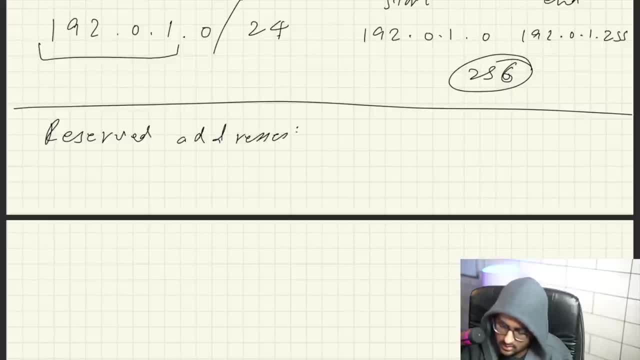 reserved addresses okay so first one is 127 dot 0.0.0.0.8 means first eight bits are reserved these can be anything so an example can be localhost 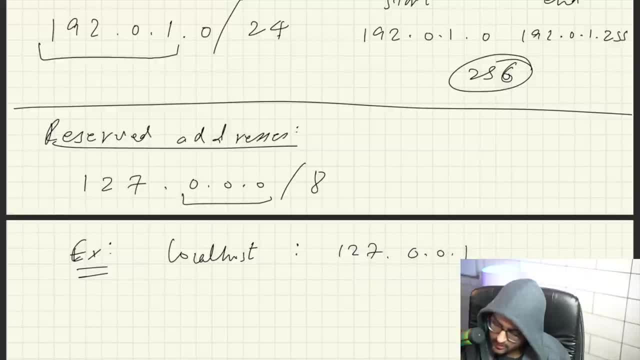 localhost is what 127 point 0 point 0.1 so these are known as loopback addresses 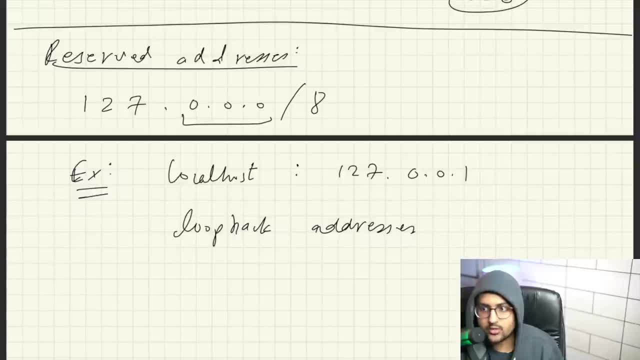 loop back addresses why is it known as loopback because the processes that are going to be running on your machine you know using your the tcp ip protocols it will allow you to contact the same processes so your device will a d 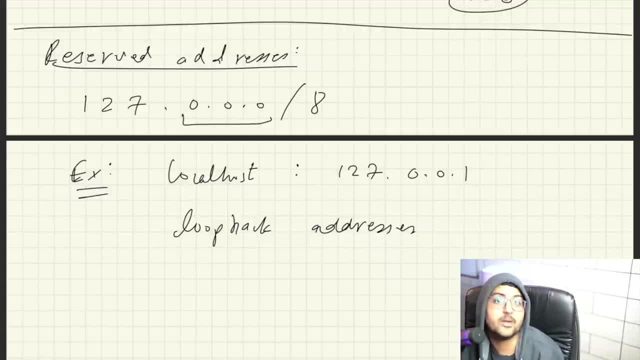 as client also and server also you know localhost these are also testing purposes if you are a developer you definitely know what localhost is but now you know the story behind it 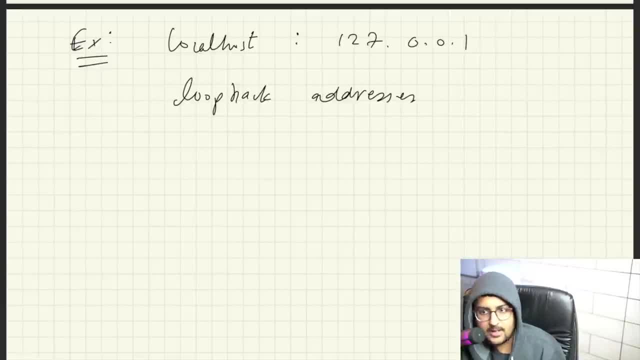 okay so it's it cannot be down it will always be up if the computer is running then you will have your localhost up and um you you can have like as many of loopback addresses of you as you 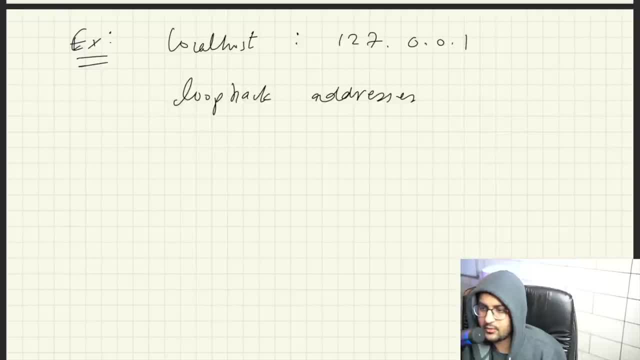 want okay sound good all right okay so now let's look at how these things the the packets thing we 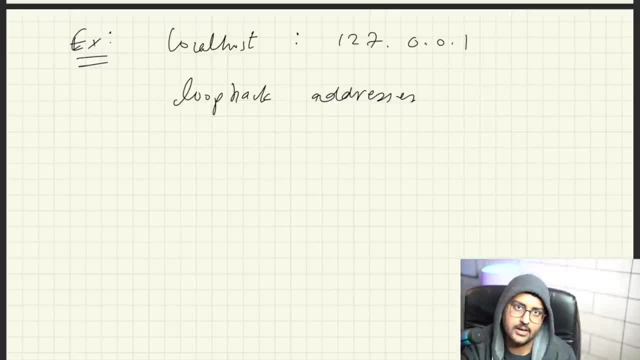 talked about right the data travels in packets and let's see how it travels and what is consisting inside a packet so one thing i'd like you to you know if you want to learn more about how it works internally then obviously learn watch you know check the research papers of how the internet 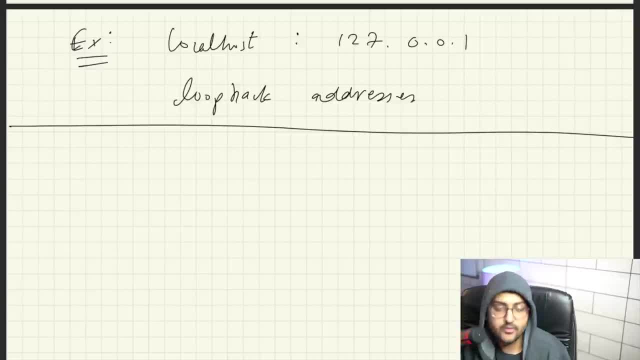 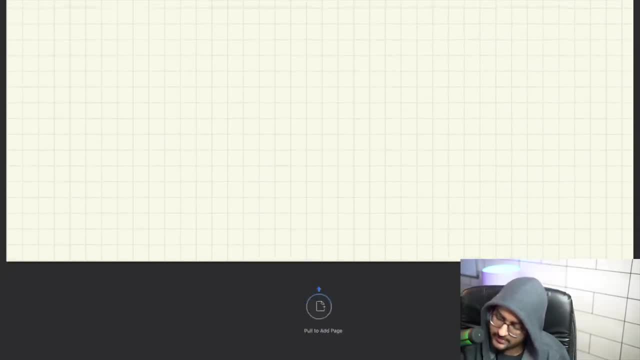 packets uh you know ip address packet the ip by ip version 4 packets work so we have already seen two packets um one was for tcp and one was for udp now the those are segments and the transport layer chunks are called data chunks are called segments there was segments i believe 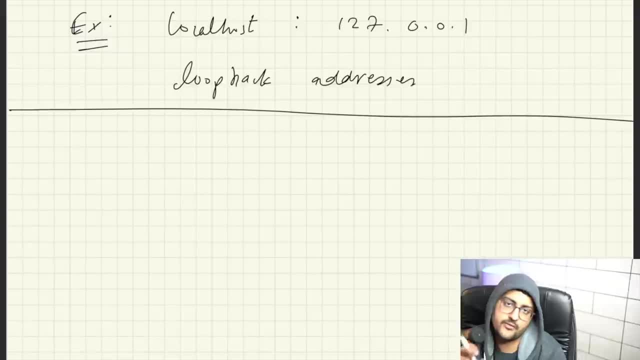 this one is called packets in network layer the ip version 4 data packets are units packets okay so packets so apart from the data the header is of 20 bytes okay so packets 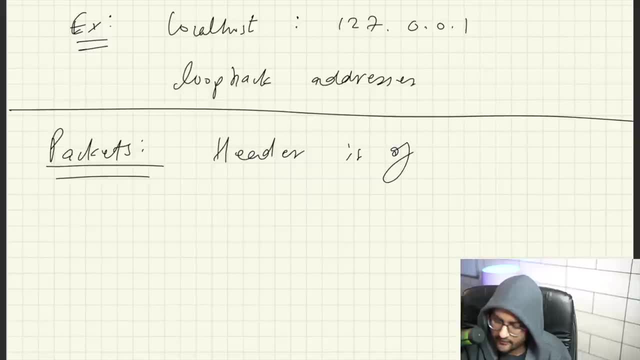 header is of 20 bytes of 20 bytes okay it contains the ip version and the you know the total length for example so like ip version the total length it 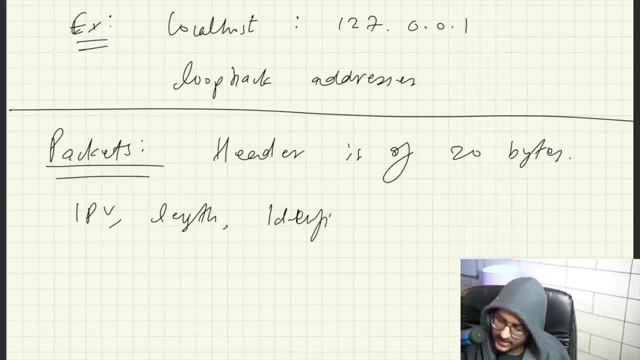 contains it contains an ident identification number for example uh in the previous example we saw some flags this also contains some flags we're working with tcp ip right and 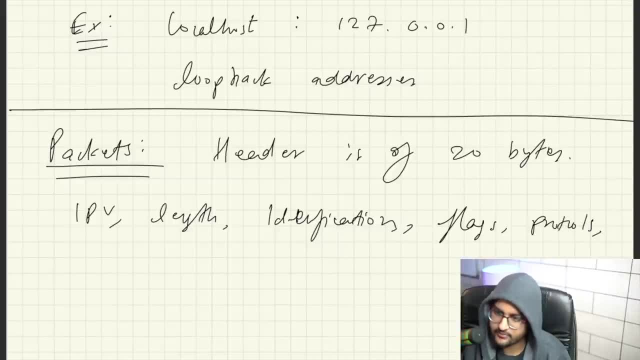 so many other things like protocols you can google it about yourself okay check some and addresses etc etc there's one more thing that contains which i'll talk about is ttl time to live 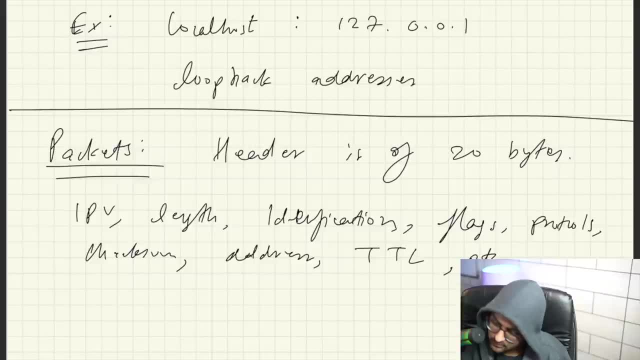 etc so what is time to live basically you know that your packets are traveling on various ip 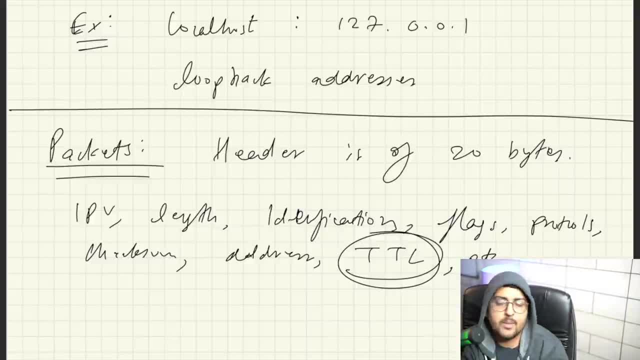 addresses like various routers it's it's hopping hopping hopping it may be possible that sometimes a packet may be like you know in a loop or something and may not reach after so many hops so that is what time to live means let's see in a in a in some detail let's see that so if i go to 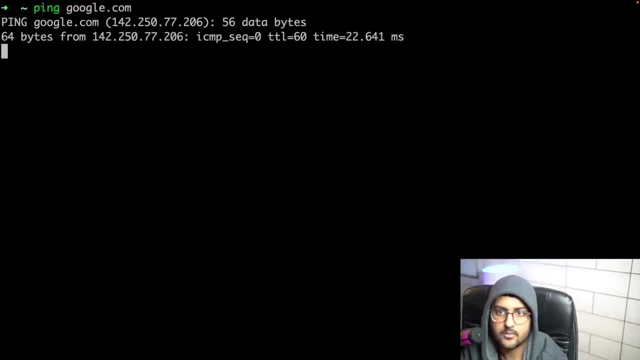 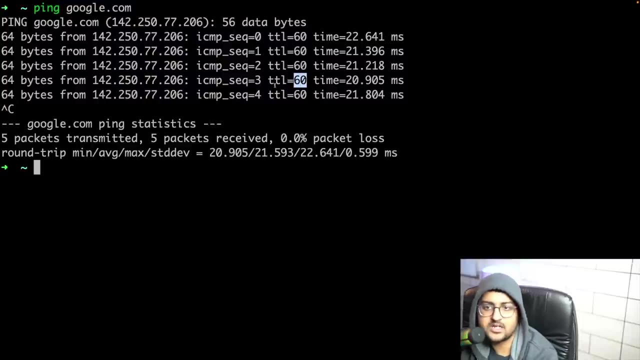 my terminal and i say ping google.com okay so this is what time to live is ttl okay so means after like 60 hops if it is not reached then the packet will be dropped the zero packet loss right 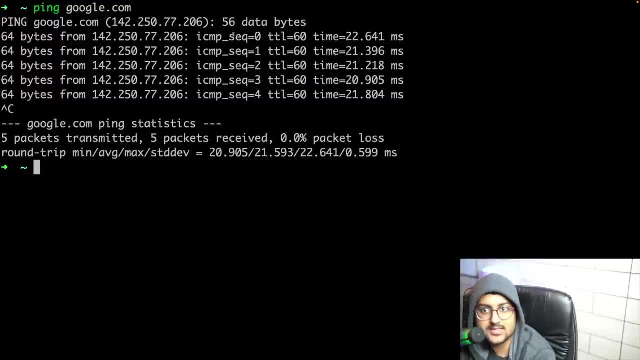 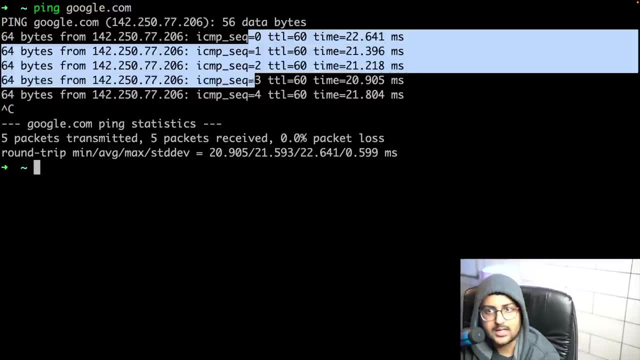 now but uh in case it was not then it was dropped and this is a sequence number i mentioned to you right the packets coming in sequence it has a sequence number or whatever this is that this is that thing okay let's move forward so that's what basically time 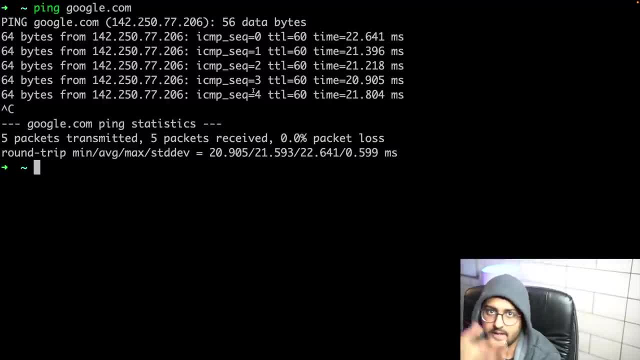 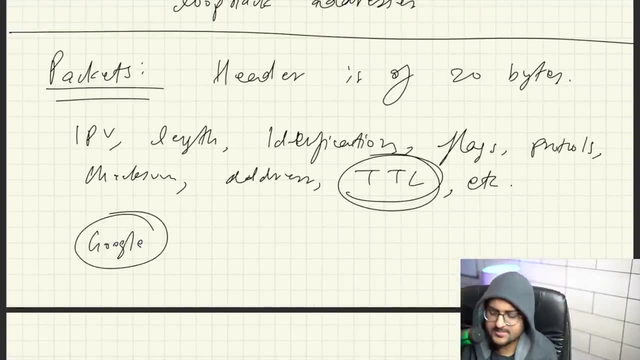 to live is so that it is not roaming inside the network forever if after some particular hops it's not leaving it's not reaching the destination then it will be dropped okay okay so this is a little bit more about packets you can you can google about it okay and how these packets like travel and everything we have covered that already you can google about it in the description box so you can google about it okay and how these packets like travel and everything we have covered that already 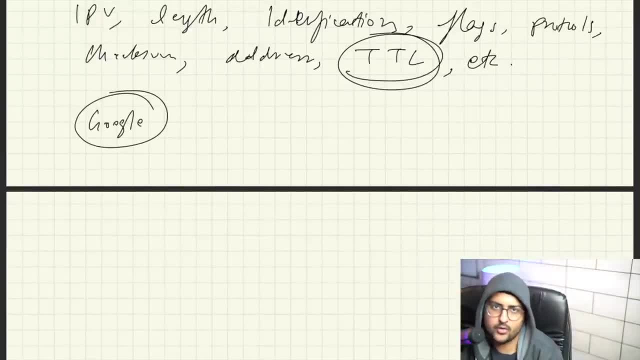 you know like ip like routers they do hopping and obviously now you know about time to live 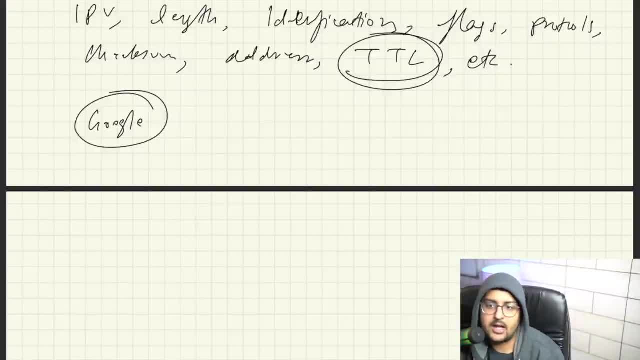 so whenever you are doing a hopping it will decrease the value of time to live and it has the checksum values and things like that okay so that's basically about if you want to learn more about it you can learn about and watch the research papers and uh dive deep into it like how these packets work like even at a very minute level uh but i think this is more than enough to understand like how the internet works okay two things one thing i already mentioned to you was 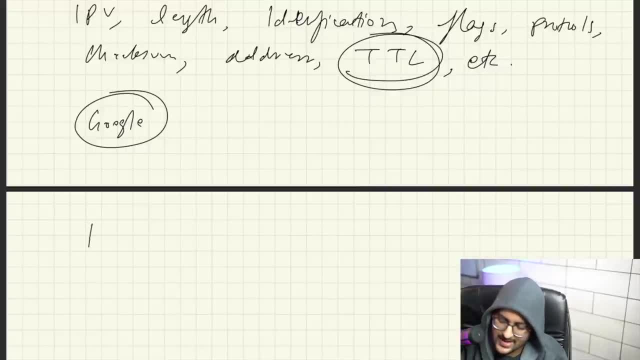 about uh this is the thing that i already mentioned which was dhcp okay so now we're talking about like let's talk about like the data link layer okay so let's talk about data link layer 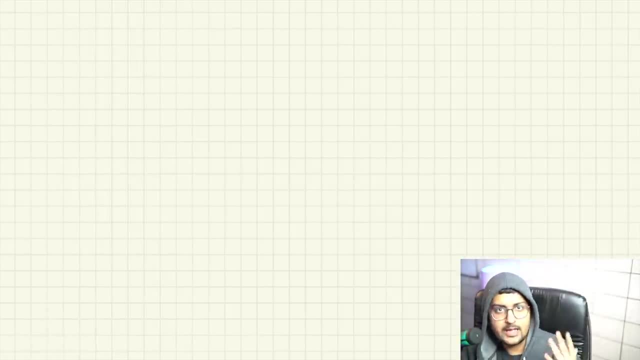 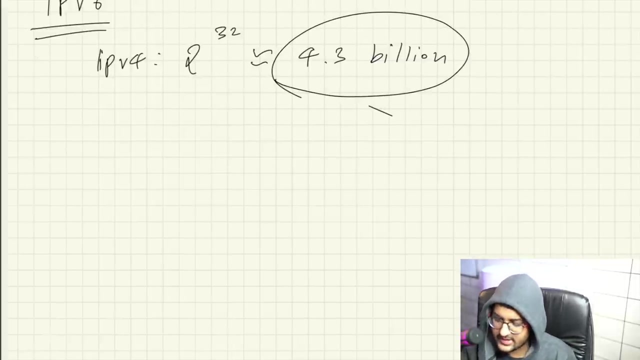 okay okay now that we have learned about ip version 4 let's talk a little bit more about ip version 6 ipv6 okay ipv6 so ipv4 means it's tourist power 32 okay so to tour is 32 bits ipv4 is 32 bits so in ipv ipv4 is 32 bits means tourist part 32 unique ip addresses you can create which is almost something like 4.3 billion ip addresses unique okay so initially people thought this was enough okay but now as more and more people are using the internet and smartphones and things like that we may run out okay so this is a new internet new version of 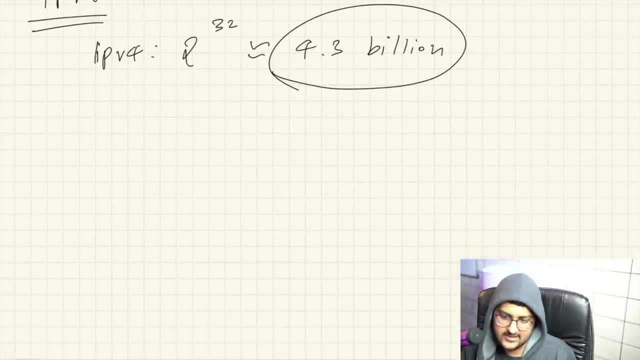 ip addresses called ipv6 okay ipv6 it is actually four times larger than ipv4 okay 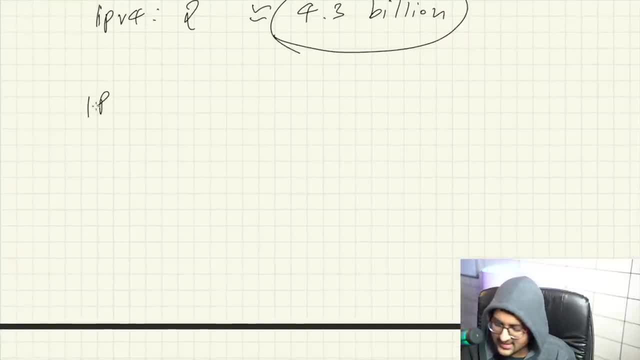 four times larger so how many unique addresses can be formed in ipv6 two raised to power three into four sorry 32 into four which is equal to a lot of numbers like uh you 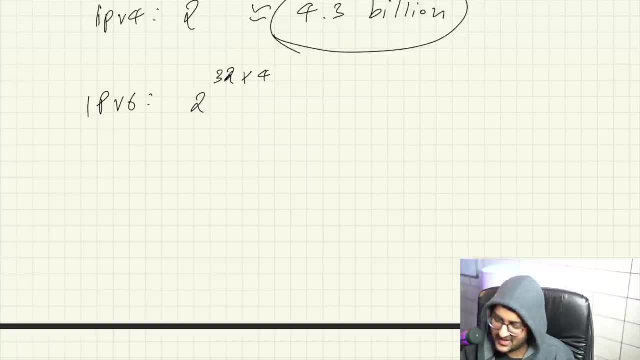 that's a lot it is a lot of number i can't even write it down so two raised to power some 128 just google it okay so this is 3.4 into 10 raised to power 38 numbers that's a lot of numbers these many unique ip addresses you can form 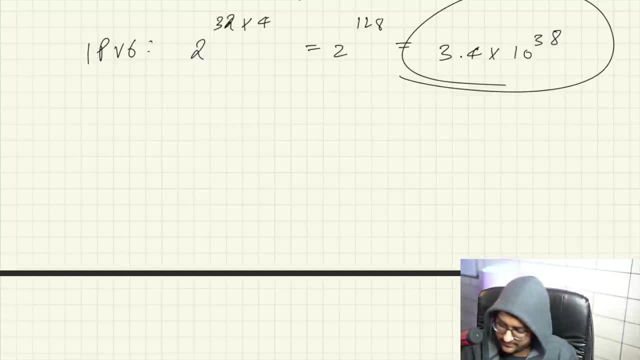 okay cool but there are some cons associated to it some of the like pros and cons cons that are associated with this is it is not backward compatible because it's a new technology okay not i mean people are using it some folks are using it and stuff 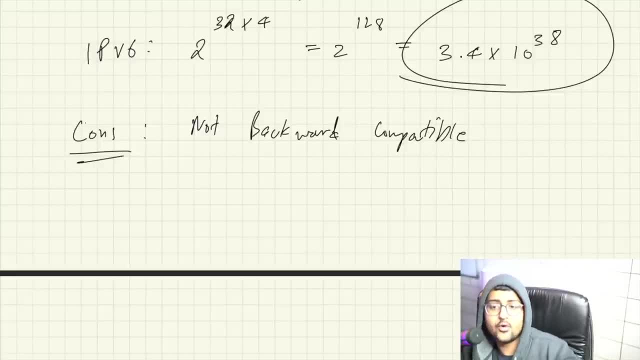 but that are the devices that are already covered configured like over your ip version 4 cannot access like websites or servers that may be configured with ipv6 okay 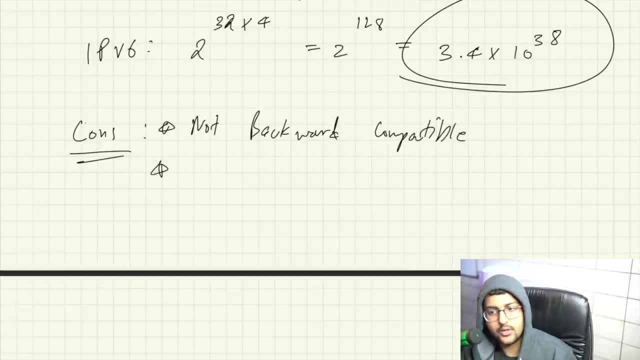 also a lot of you know like it's going to require some efforts okay this is a reason why the entire world has not shifted on ipv6 yet okay cool because isps would have to shift would have to shift a lot of hardware work work okay sound good cool 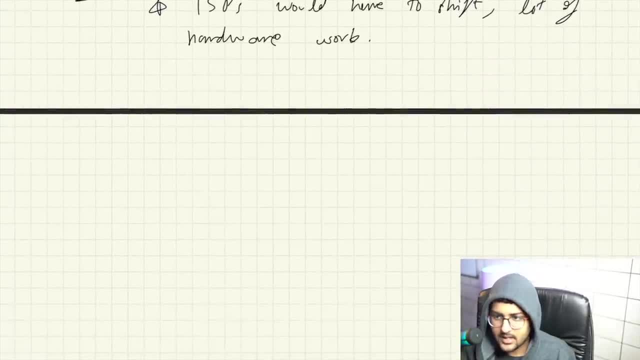 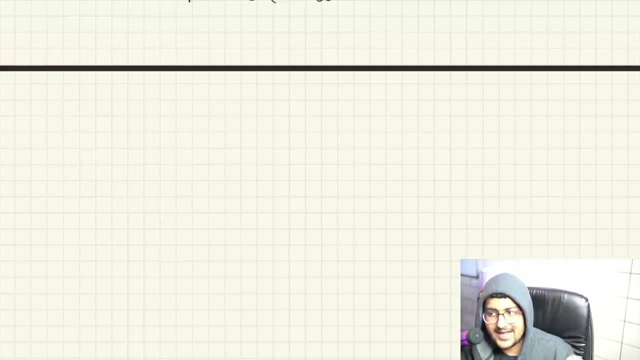 so let's talk about it um how is it represented so there are actually eight eight numbers and every single number is a hexadecimal digit okay represents like 16 bit parts of the addresses okay hexadecimal okay sound good so here if you have like something like two two three four 5 6 7 8 and this is a hexadecimal 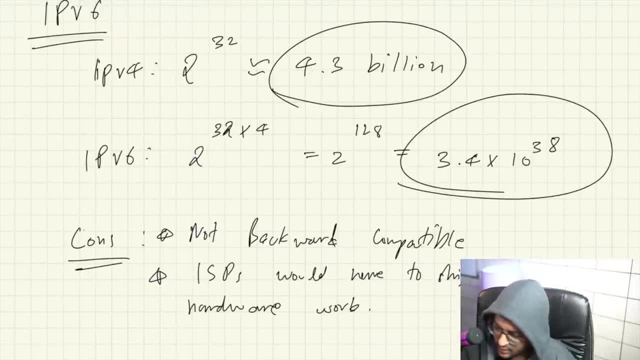 okay so this is 128 bits if i'm talking about you know like 30 20 24 and then since오라 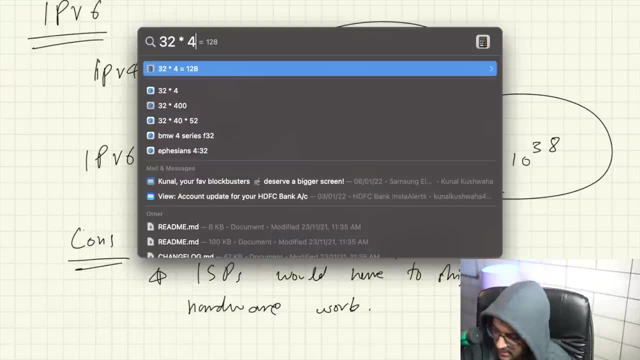 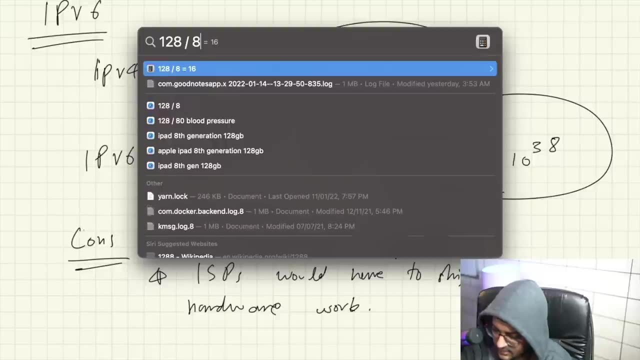 124 dawns 32 into 4 128 and 128 i'm saying dividing into 8 so what do we get over here 16 so it's a 16 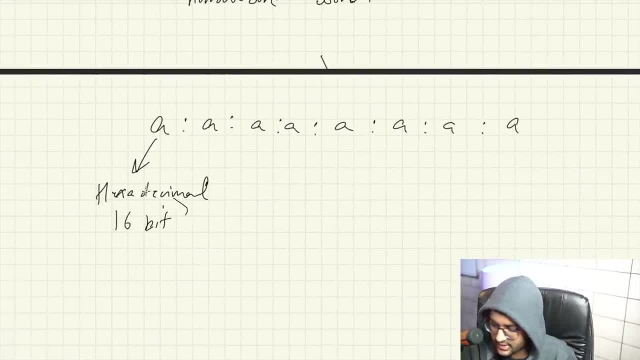 bit number hexadecimal this is a 16 bit string over here of hexadecimal okay sound good 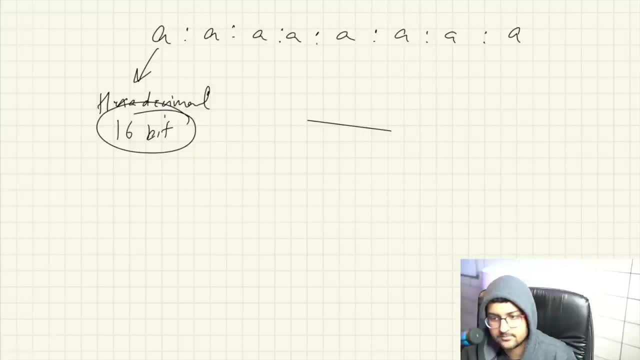 all right that's basically about it 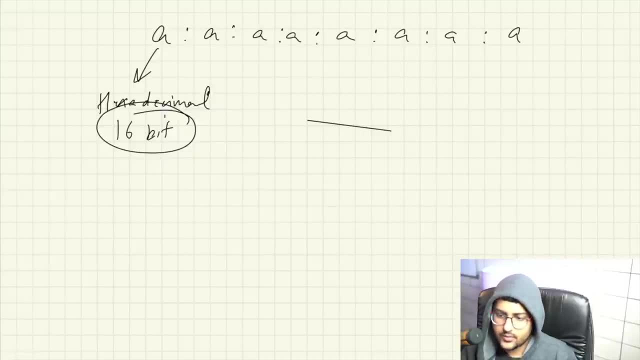 okay so we won't be diving deep into ipv6 but uh an example if you want to take an example and hexadecimal i can take something like 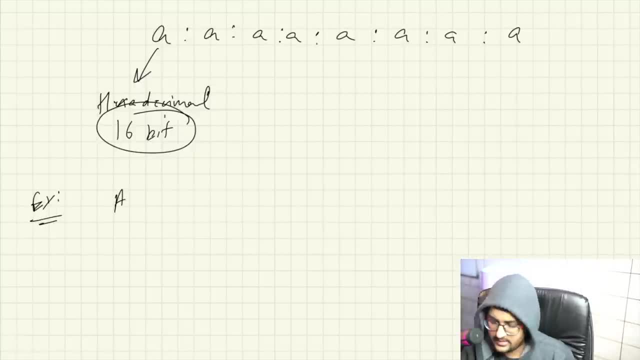 something like a b f e something like that okay f zero zero one three two one zero zero zero zero zero nine one eight two something like that obviously 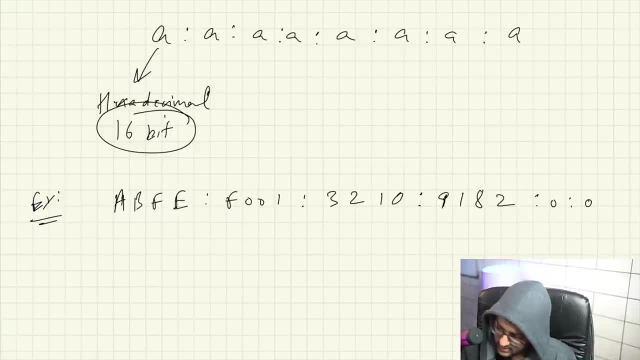 zero zero one two three four five six one three something like that i ran out of paper but you 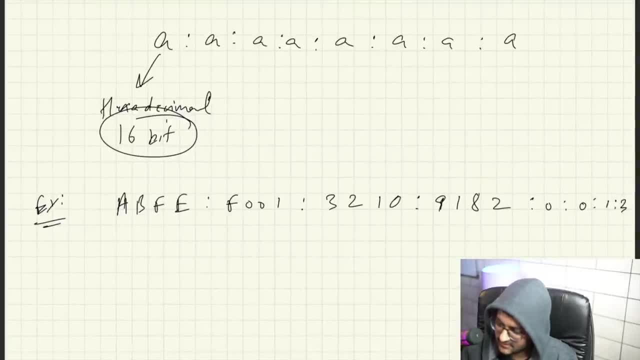 get the idea it's one of the examples so this is a little lot big number okay sound good cool 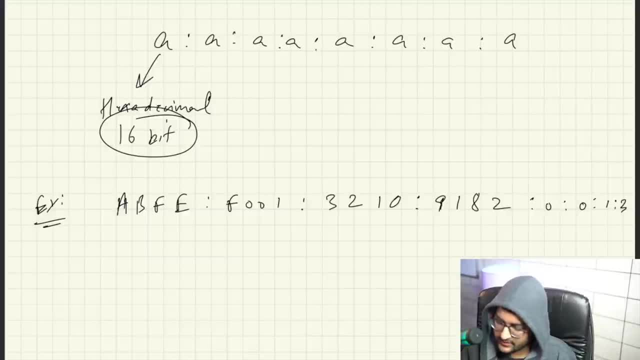 and you know in previous ip addresses we had something like like 127.0.0.0-8 eight basically means you know the subnet that is prefixed prefix so in this also we can do the same we can do the same representation here also okay exactly the same like that some can be fixed let's say first two are or let's say 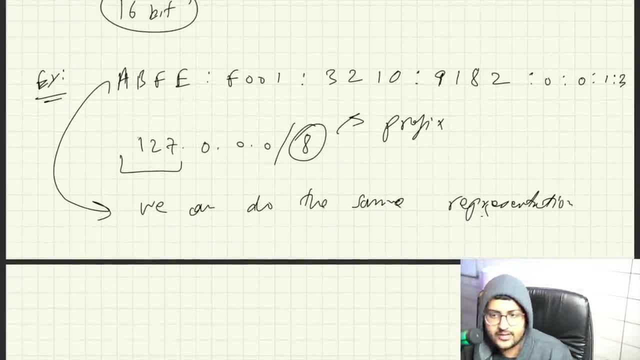 you know we have the first uh first four are fixed for example okay so you can have like a b f e f o o zero zero one three two and nine one eight two okay after this i can just say rest are fixed so let's say 60 sorry first 60 are fixed and then rest as it is 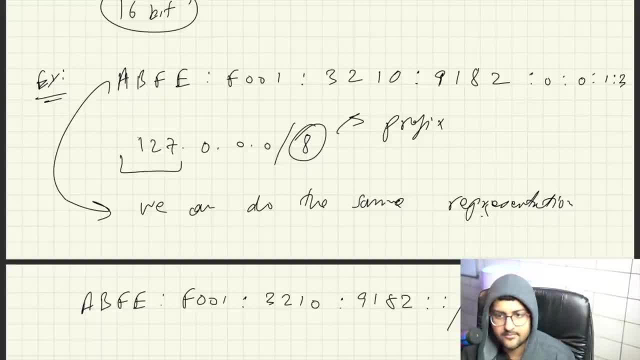 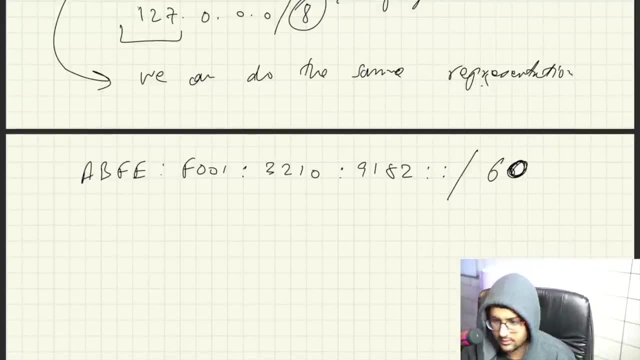 okay now it will be three no it will four that's fine yeah about four something like that sound good make it smaller like i think that's sounds good okay so if all the values are zeros for example if all the values are zero you can just represent this as zero or if you put just one zero over here or you put no zeros over here that is also fine so basically if you're just 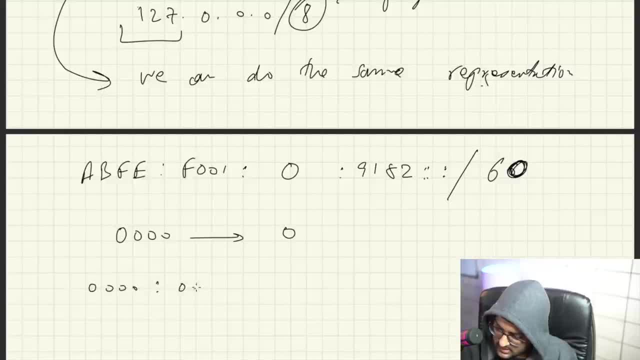 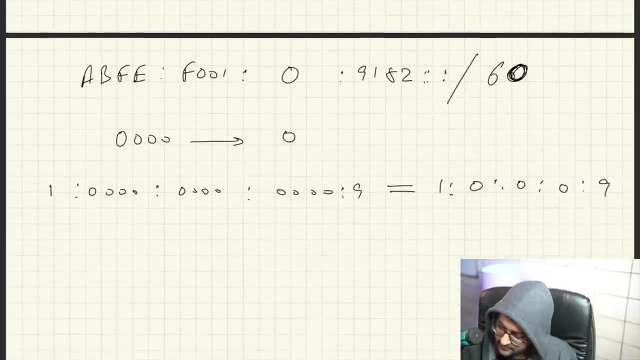 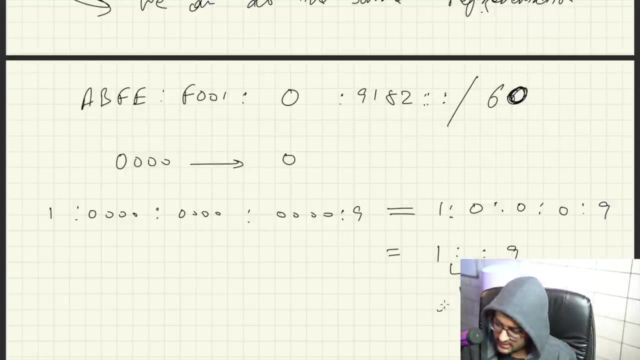 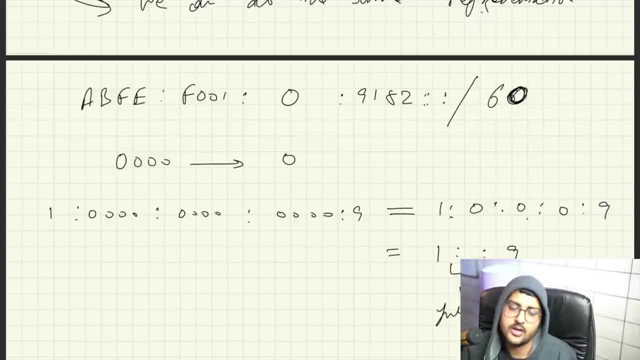 okay how many zeros that depends on like how many numbers you may have in in front or back okay cool 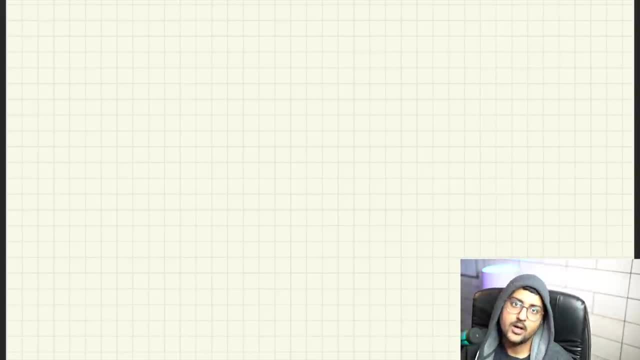 let's move forward okay so you can learn more about it and how uh you know companies are utilizing ipv4 ipv6 and how the government is you know transporting like deciding whom to give and what all are in use right now you can research more about it later on but we are not going to worry about that because we are working with ipv4 and during the course also we'll be working with ipv4 okay 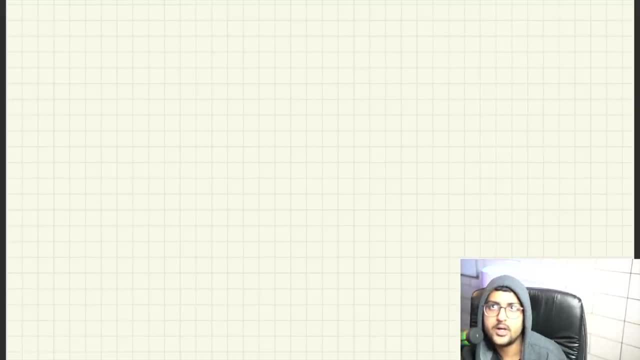 yeah okay one more thing i want to mention is that right now we have learnt about the computers that interact with ipv4 and i think we also took advantage of current support to get snow joy at home and have it up all right yeah yeah an important fact is that right now we have learned about the 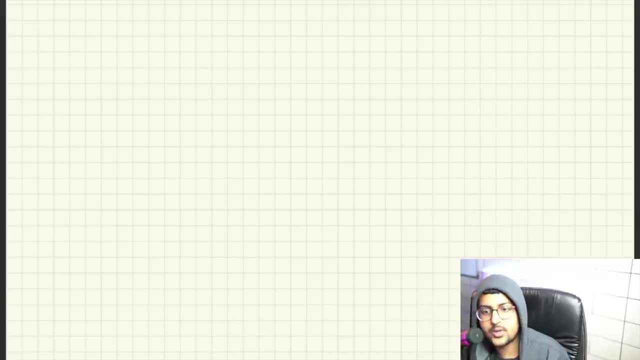 computers that interact with us and issues regarding IPv4 is also going to be taught for Epidemic Medicine in future videos and many more videos as well so thats a bonus kind of thing that's valuable in my opinion that interact with each other and the routers but there's one more thing that interact with 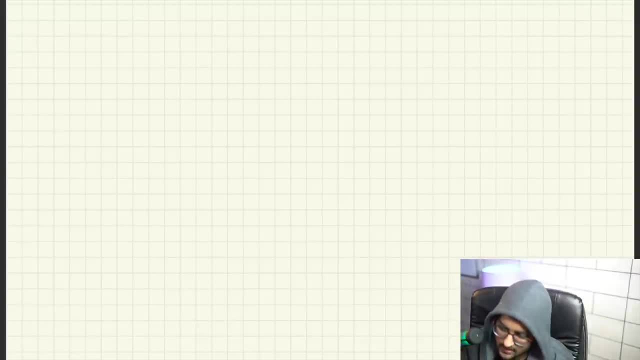 the network packets that come from the network layer these are known as middle boxes 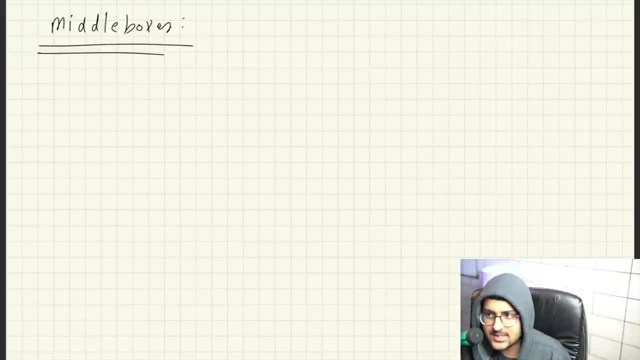 okay so these are like uh extra devices that also interact with the ip packets 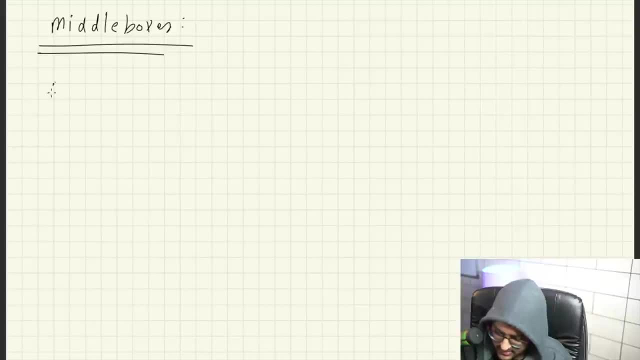 be in the transport layer first one that such first such device is firewall may have heard 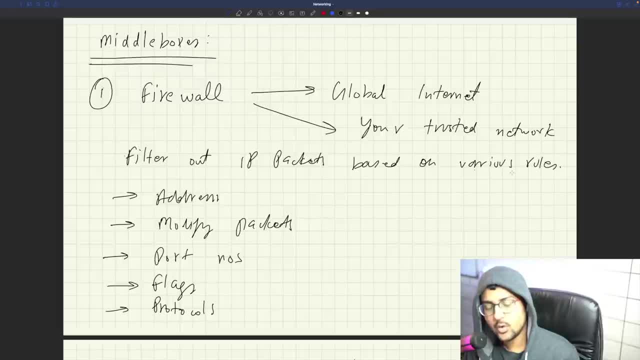 about firewall okay so let's see what a firewall is okay so so far we have learned about like two types of devices one is like the end systems or computers and another one another one is what the routers but there's one more type of device that comes in between which are known as middle boxes so middle boxes are like uh you know um they they also uh work with like you know your brackets that interact with the network layer and then they also interact with the network layer that are being coming so you can allow some packets and reject some packets and modify these packets so on and so forth all right so some of these they operate over like in the network layer but they also exist in the transport layer so one of these middle box that we look into is a firewall so middle box is something there's just like or middle like devices apart from your computer and the routers that also work with packets so for example using a firewall there are like two types of firewalls right so so there's one that is connected to like the global internet and one that is connected to your own network right so what firewall does is it provides like filters so you are uh you are get given like some filters like okay all the ip packets that are coming to my network uh they can be filtered out based on let's say the address okay so if you have someone who who an ip address 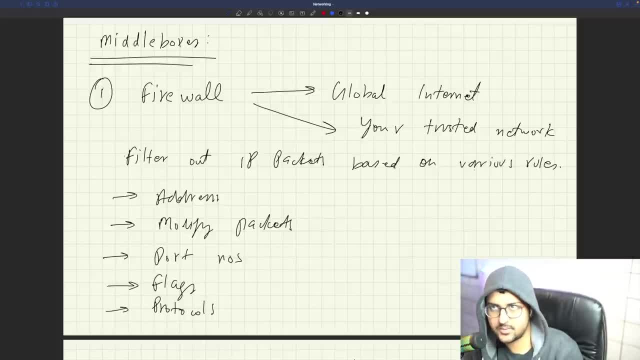 is coming from a specific address you want to block that so you can block that you can modify the packets of example some ip address coming to your internet so you can block it you can also do is coming it's coming it's going to location destination a you want to change it to destination b you can change its header or something like that you can uh you know set some rules on like 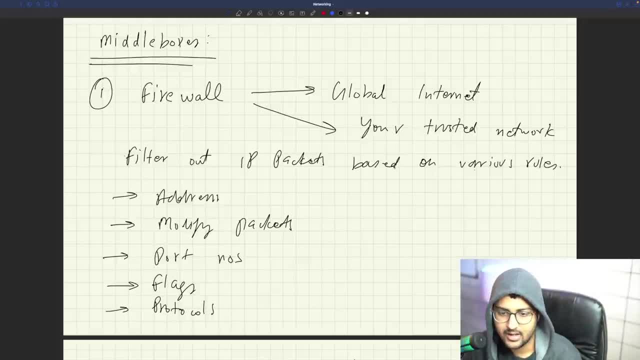 the port numbers like okay on this port numbers we're not allowed to have uh you can set flags so for example in the new connection we saw that a sin flag is required right um so you can be like okay block all the sin flags so that no one can make a new connection and like simply like port numbers and protocols so on and so forth right so there are like two types of firewalls there's 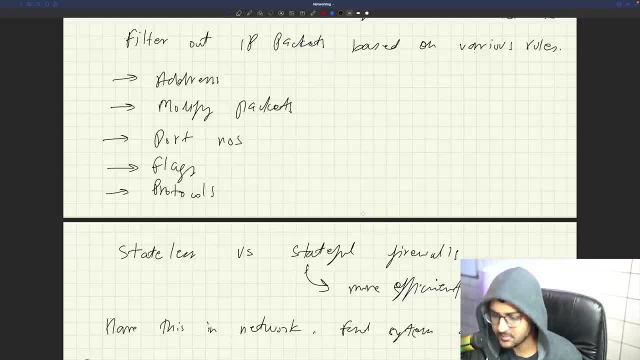 a stateless firewall and there's a stateful uh firewall so the stateless firewall will obviously do not maintain a state um and a stateful firewall will uh you know see the packet and maintain its state means it's stored it stores it in its cache memory so all the other that will come uh you know for it it will basically be like okay we have received some sort of a similar packet we can allow this one or deny this one or whatever so since it's using cache memory and something like that it's a little bit more efficient so where is this in the network it's basically uh in the um you know um 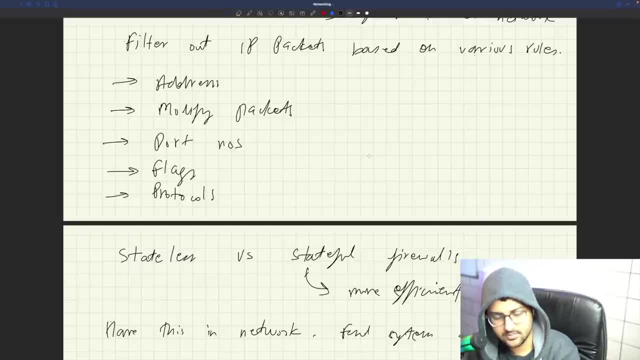 there's like two types of it so one is like the the one that is hosted uh you know by the host and end systems and one that is in the network so it's in the network layer as well and it's in the transport layer as well okay so the second middle box that we're looking at 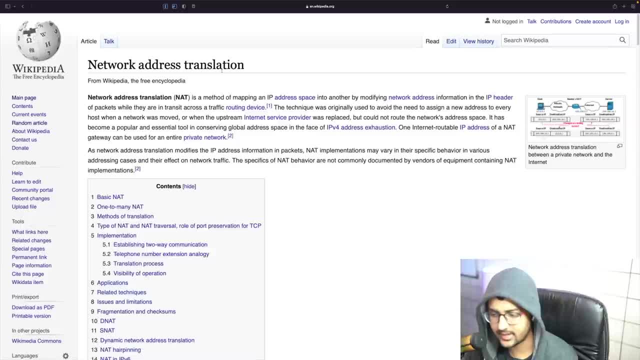 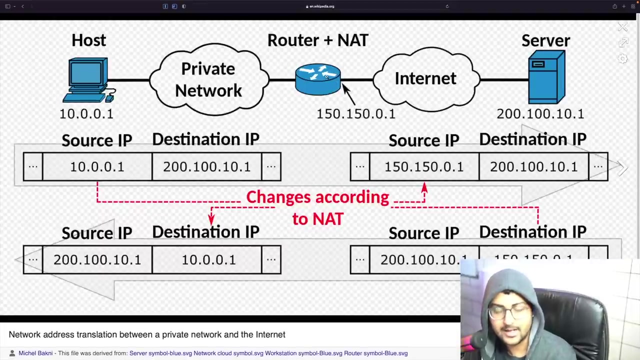 is called a network address translator okay network address translation which is known as nat so what is not so basically not is a method of mapping an ip address space into another by modifying the network address ip information in the header of the packet okay so the idea is something like this that you have your own ip addresses over here right and you have a not over here network address translation so it will modify the addresses so to the outside world the address of the packet is what is called a network address and this is the same thing so we're of the devices will look like 150.150.0.1 that is connected to the internet okay and now since the 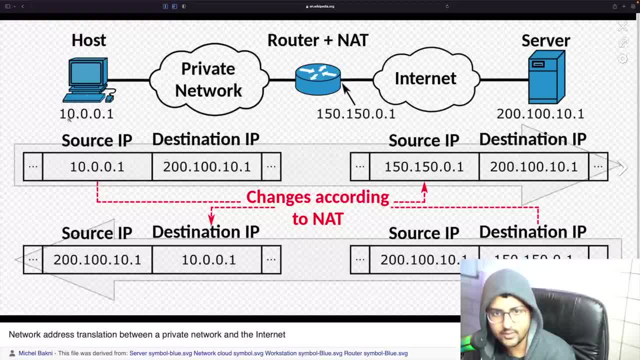 ids are coming from this network initially the host id was 10.0.0.1 but nat actually modified it for the internet now the id is coming from 150.150.0.1 so now all the ids in your network can be worked as a private ip this is the basically what nat is okay sound good so why did this happen so basically uh you know um to slow down the consumption of ip addresses you can 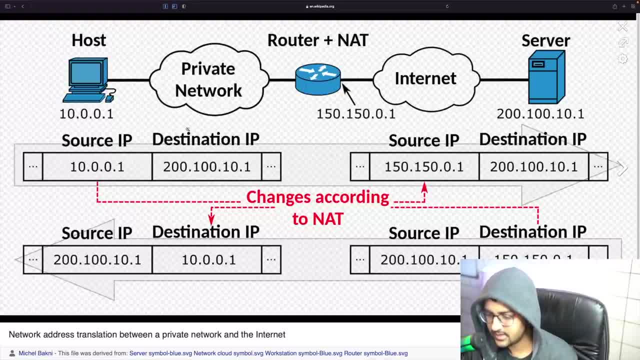 only have like two ish part 32 so that's basically one of the reasons okay so some enterprise uh you know networks also use this and you can learn more about how you can send a message over a nut okay so that's basically about it all right 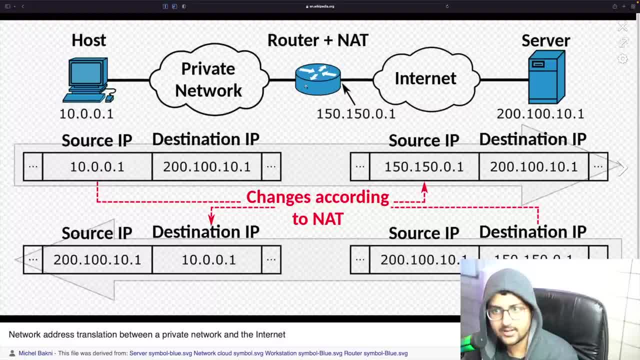 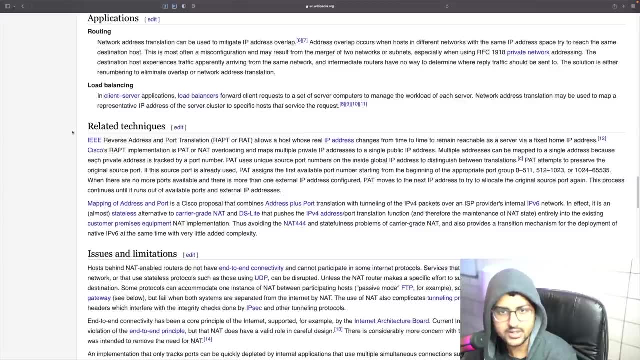 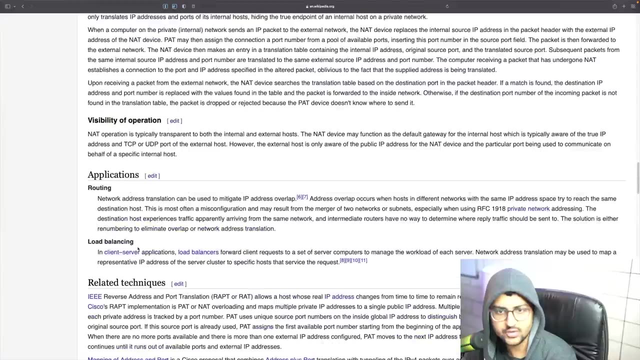 whenever you're getting some packets or something like this nat will have like uh like its own like you know uh memory or something where it's gonna save it and then it's gonna pass it over over the internet you can learn more about it like there's a lot of types of uh nuts as you can see uh you know like applications for example so it's used in routing in load balancing right um and uh also some issues and limitations you can also learn about like how it works the implementation so like a two-way communication 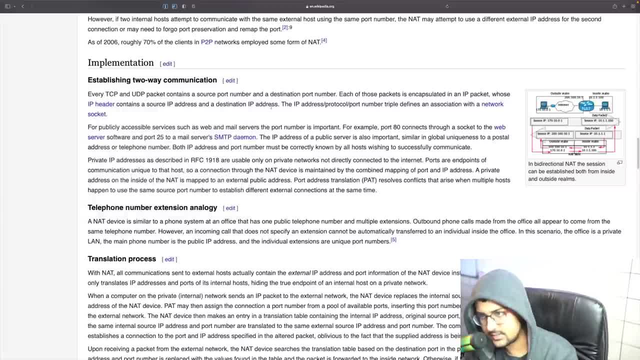 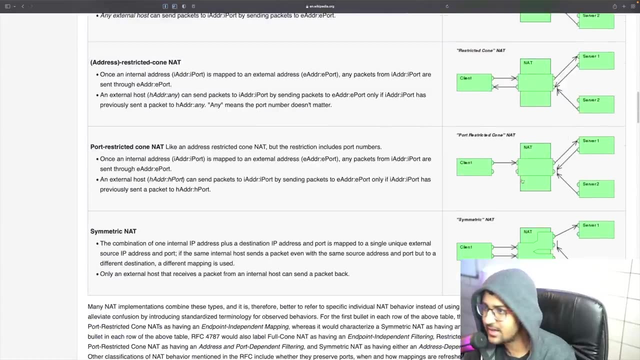 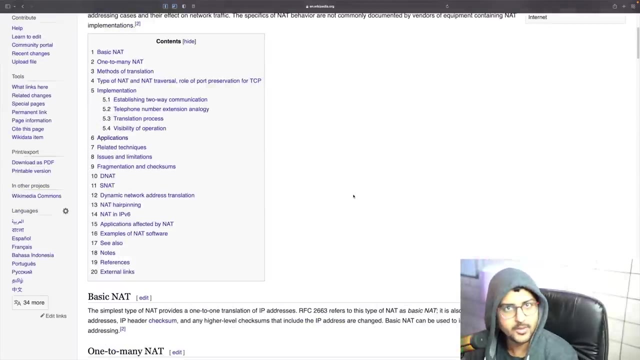 and ip header contains the ip source and destination ip address there's something we already know and uh you know so many things like you can do so you can have private ip addresses and everything like that okay and translation process and visible visibility of operation everything you can types of nuts you can see on the screen right over here and methods of translation and all these other things so it's a pretty big topic and definitely you know out of uh out of our scope but uh a good information like 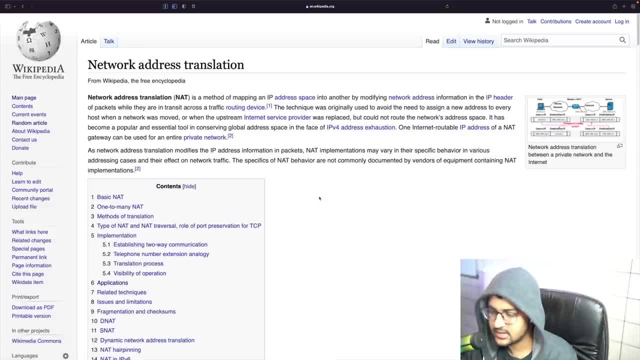 website, thouI send write and bring in a packet and a link will be given in the description 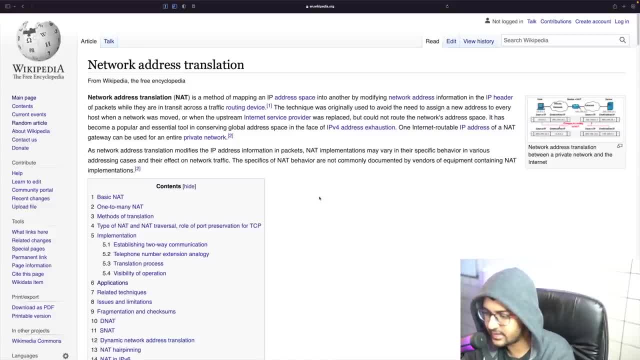 so basically that reminds you about theceu- jokes and what you can do as a discord server 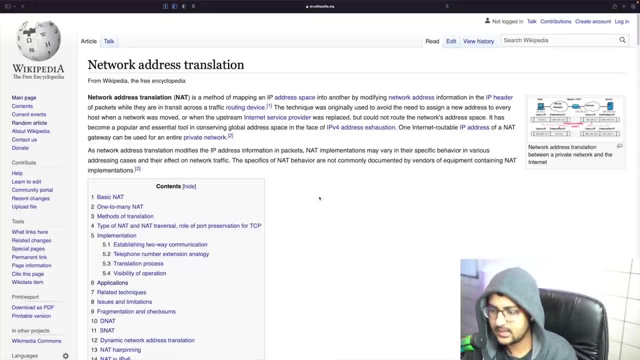 and also how sharing works to the eskimo so data untrans Sergio goes across перев hoş that her words back catalog and we had some 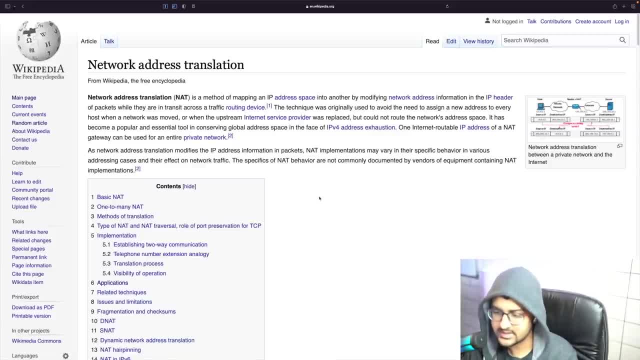 you know disks you know tools of the sco flor a ease of doing a lot of different things is basically so important too important to give it's the same thing like uh you know the the source address of the packet that you'll be having uh that that is replaced by the public address 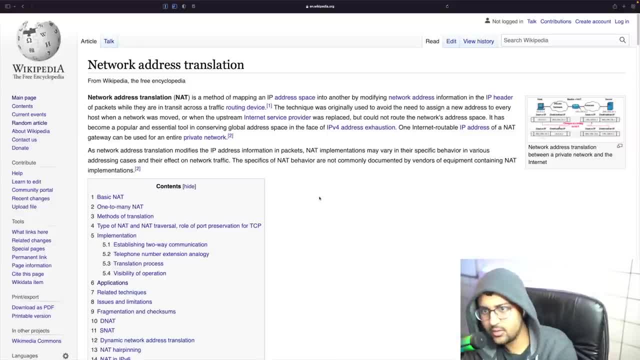 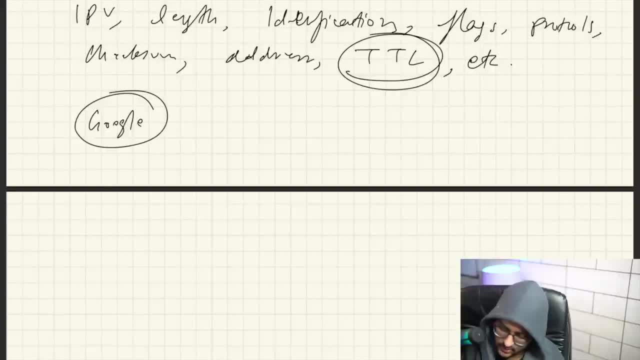 gotten it from the public internet and then it is forwarded in your own internal network so that's about NAT and that's another type of middle box so this was about like the network layer and then 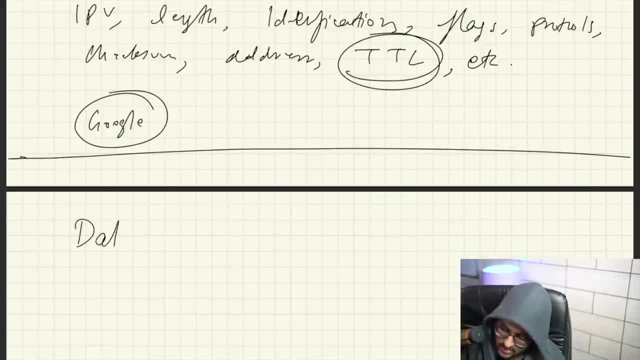 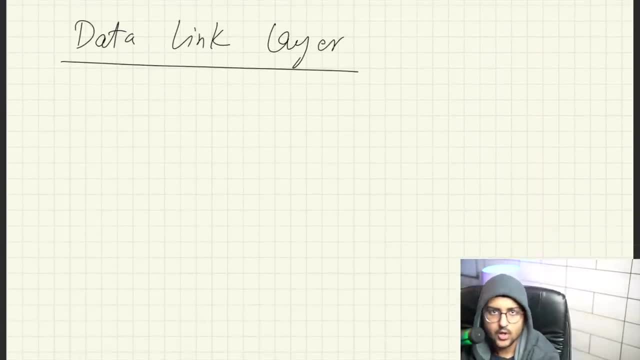 now the second last layer so let's talk about data link layer of TCP okay so let's talk about data link layer and what it does so the data packets that we received from the network layer the data link layer is responsible to send these packets over a 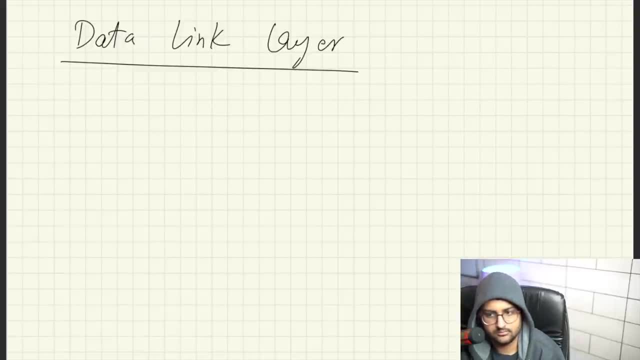 over a physical link okay sound good cool so it will just transport like your data between like connected devices for example so for example you have your own router I mentioned this previously you have your router okay your router has some 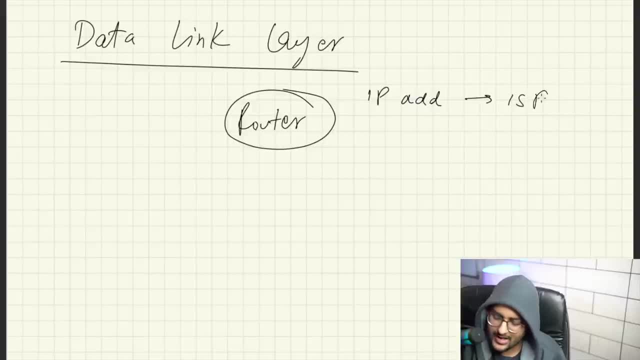 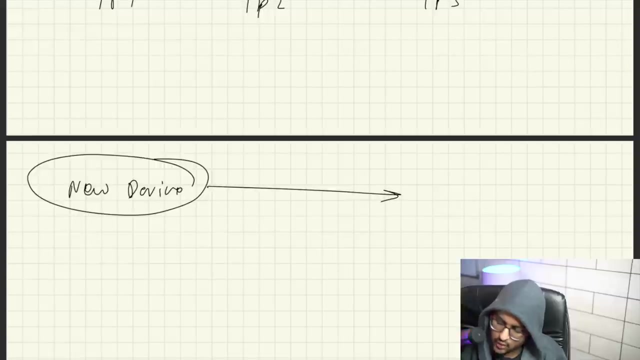 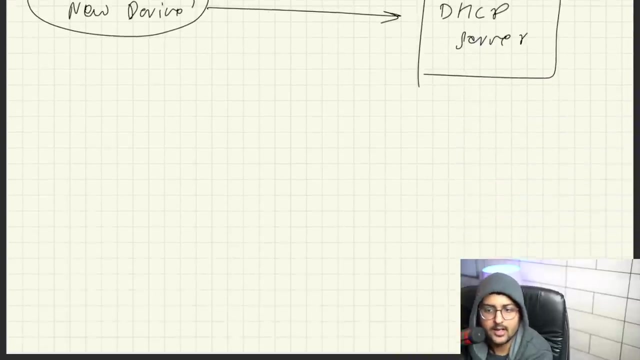 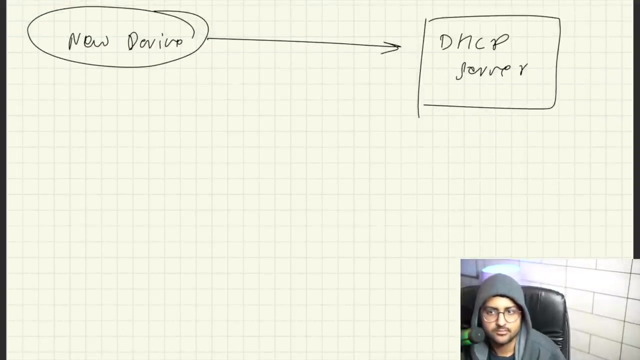 IP address that is provided by your ISP some devices are connected to that router these devices have their own IP address says so there's going to be a subnet available over here and new IP addresses are going to be allocated to this how does this happen I have mentioned this previously DHCP okay it's known as dynamic host configuration protocol okay so dynamic you can google it yourself dynamic host configuration protocol so whenever a new device is added to your router or whatever it will connect your new device basically your new device is going to connect to the DHCP server okay he's going to be like hey I need some IP address can you please allocate me some of the some of the IP addresses okay so this is going to be like this okay and every DHCP server will have some pool of IP addresses pool of IP addresses ABCD IP addresses so it's going to assign some IP address to your new device okay okay so since 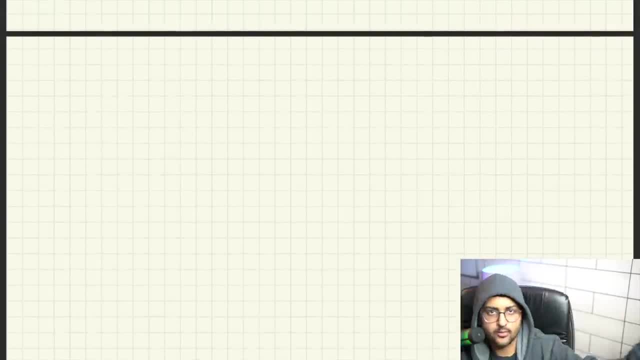 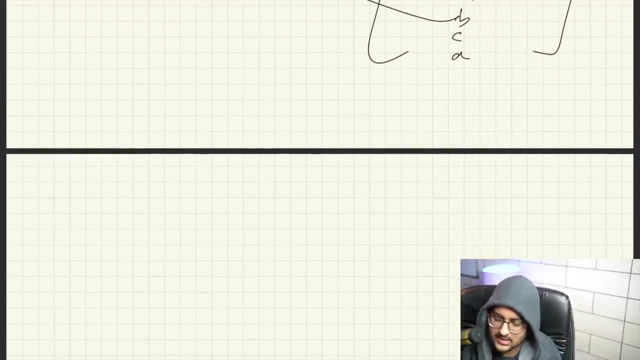 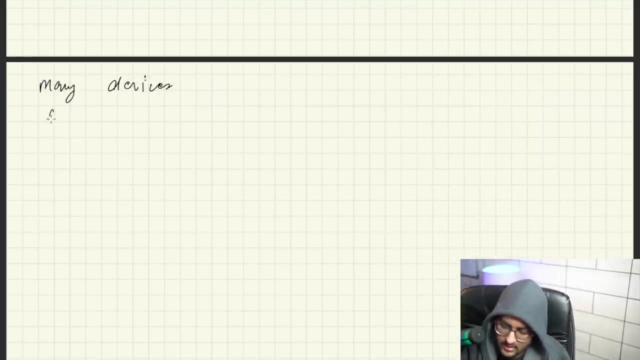 we're talking about the data link layer we are now not like talking about network like in the networking how it was now we're talking about the actual physical presence like how data will be refrigerated everytime we have any spark connected in the network right this might not be the case like this is like if you could connect a huge existing network you're saying it's played from like somebody 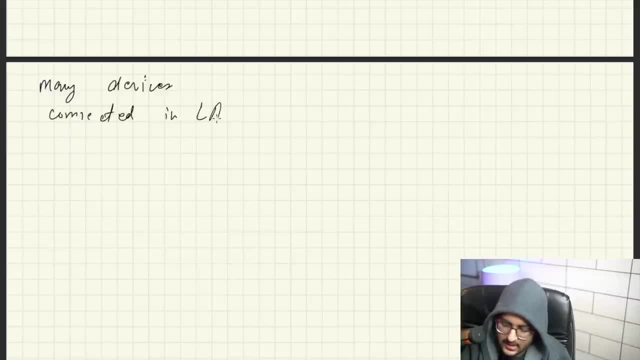 away from the network and you assume the network has a share just toşle hard that's why it is didnt connect okay 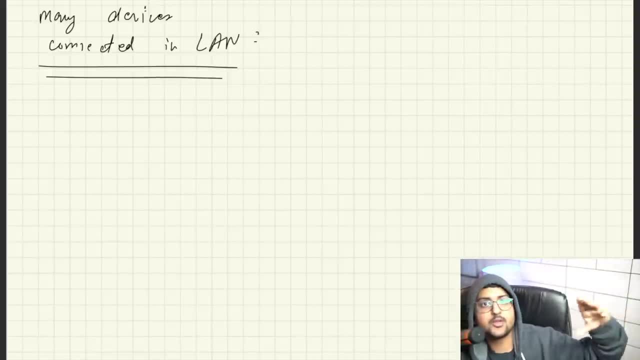 when you connect to your network yes you can split URL into where you can plug redes PCs two computers are being found out together or whatever using the ip addresses and subnets of 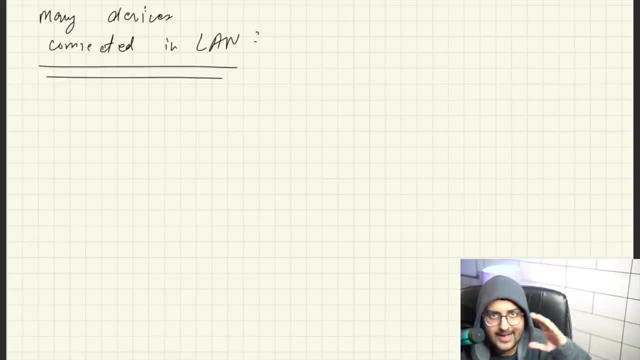 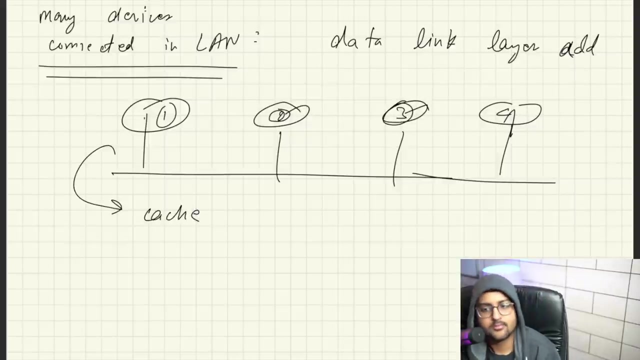 the ip uh internet service providers or whatever but at the data link layer they communicate with each other using the data link layer address okay something known as the data link layer address so every device that will have like you know an ip address they will also have the data link layer address so all the you know if you're sending from one place to another they may know their own data link address like of the destination also so basically what happens is how it uh you know happens you can manually allocate data link address data link layer address to devices but it also happens sometimes like automatically okay so for example devices are connected to one LAN let's say device number one two three and four so device number one two three and four let's say device number one needs to send something to device number four okay so device number one will check in its own cache hey do i have the um you know the data link layer of device number four it's gonna be like no you don't when it does not have it then it's going to uh ask in 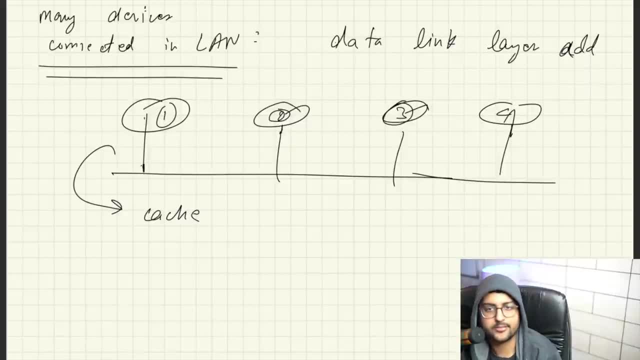 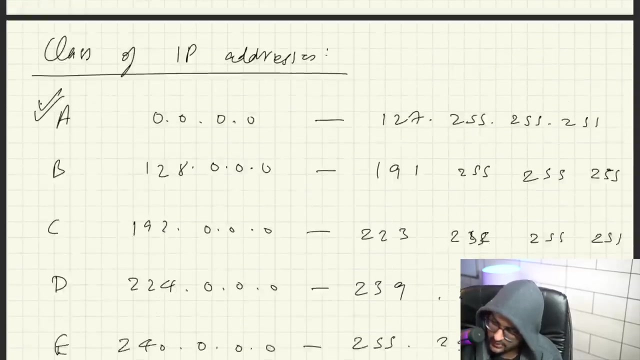 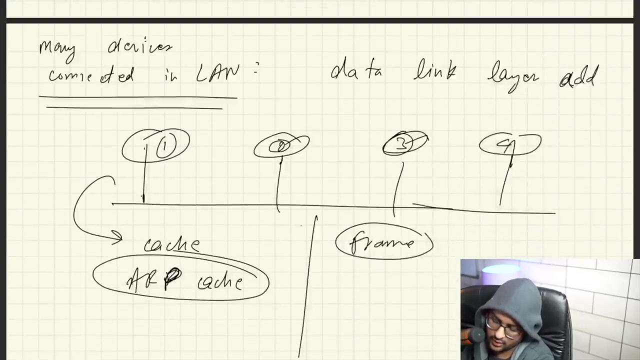 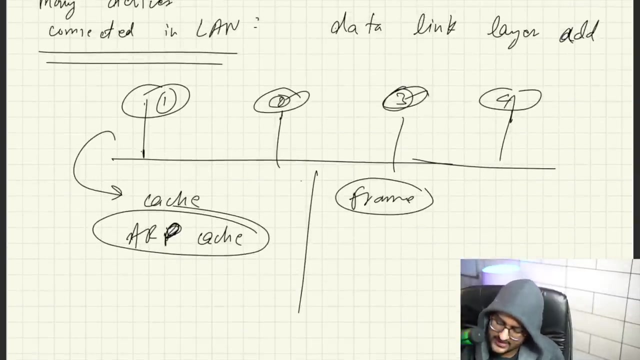 the in the all the like the devices that are connected over here okay this is known as arp catch arp cache okay this is known as arp cache so all the devices i repeat all the devices that will be connected in this will receive a message from this device what will be the message message will be a packet okay or a frame since we are in data link layer so data link layer transfers in frames let's see we wrote it down over here somewhere data link layer frames okay so what does the frame contain another good question frame basically contains what the data link layer of from where the data is coming of the sender so data link uh layer address of sender and ip address of destination then it's going to be like hey is the ip address of the destination can you send me the data link layer of the destination it's going to be like yeah sure how about that that's it and that's and this is known as address resolution protocol 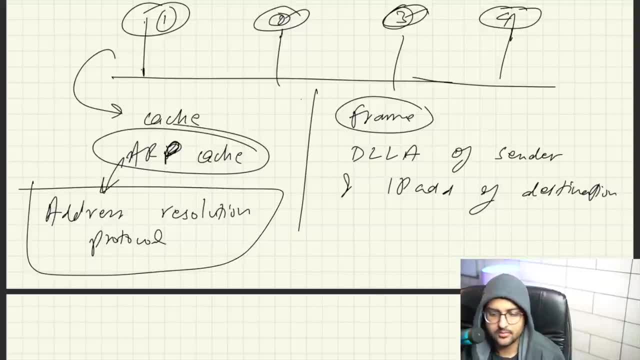 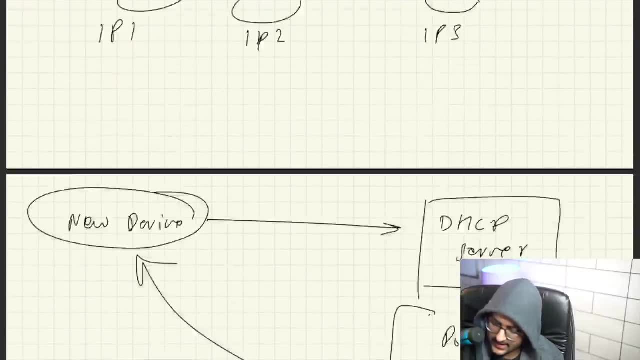 okay this is what is known as address resolution protocol cool all right okay and it is these data link layer addresses that we are talking about the data link layer when we're talking about the data link layer addresses 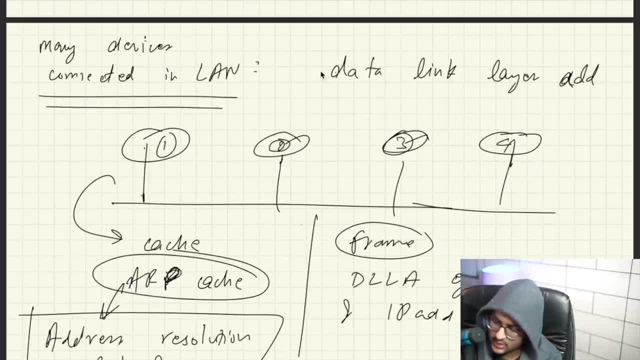 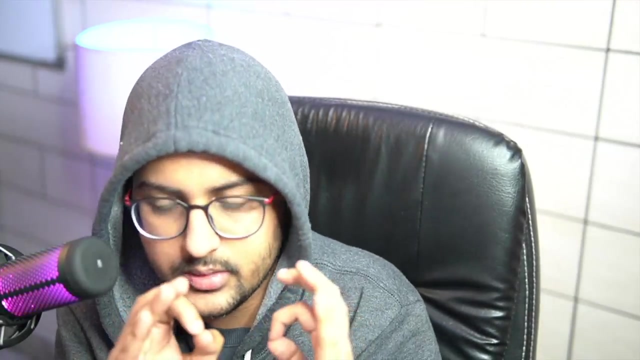 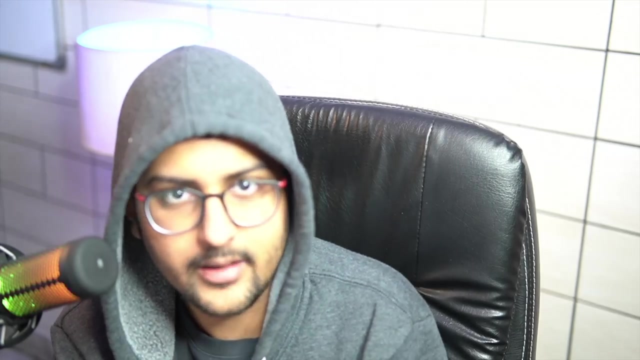 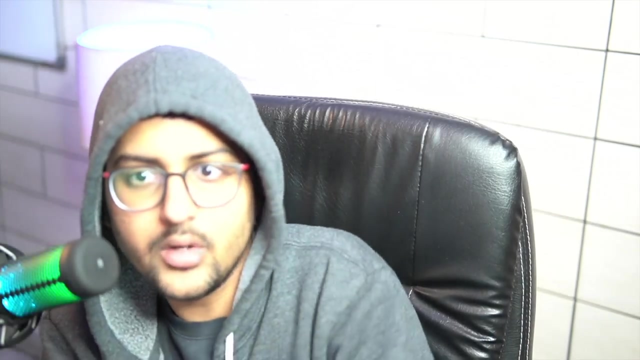 okay the data link layer addresses this thing is known as mac address of your devices when we're talking about eternets and stuff this is also known as your mac addresses it identifies the device so mac address is not of your device it's actually of the component so your wi-fi may have a different mac address okay your bluetooth may have a different mac address right so this is basically about mac addresses so it sends all the mac addresses like okay which one do i want to go to it will go to that one so as you can see data link layer works very closely with the physical layer okay it takes a lot of you know like if you if you talk about physical layer how that works that will take a lot of time because that in that then we'll talk about electronics okay and hardware and stuff this is more about the computer networking part that we're talking about okay so if you're into electrical and hardware stuff then definitely research more about it okay so mac address like when you make a request and when the data comes back to your router the it the router it will basically attach the correct private ip address to the data packets ensuring that they got to the computer and device the router will do this because all those private ip address that i talked about they actually correspond to the correct mac address only okay so this thing that i talked about the data link 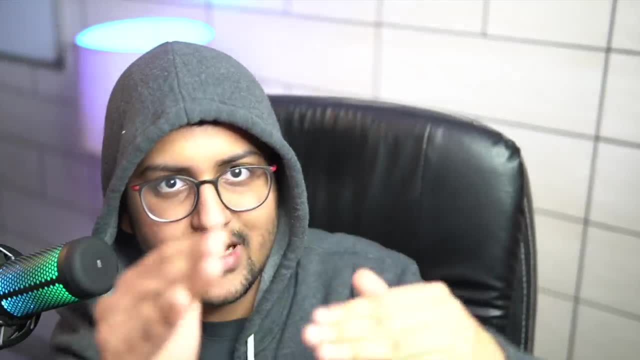 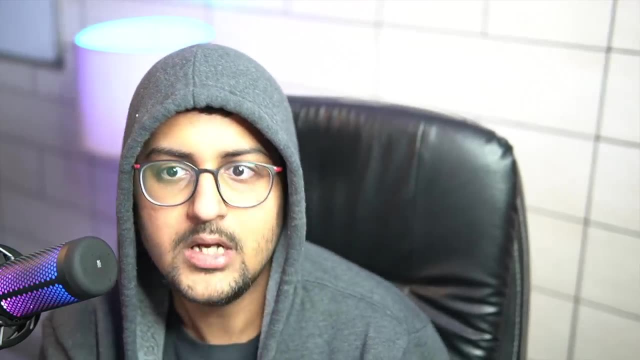 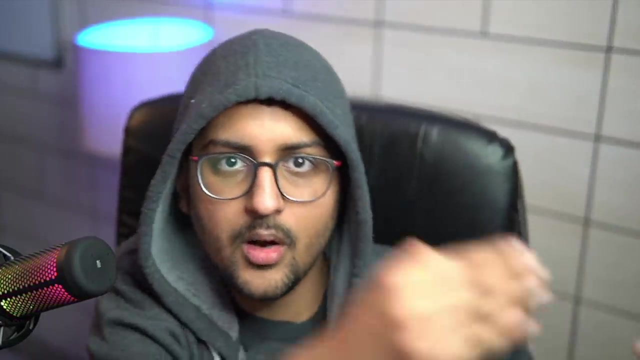 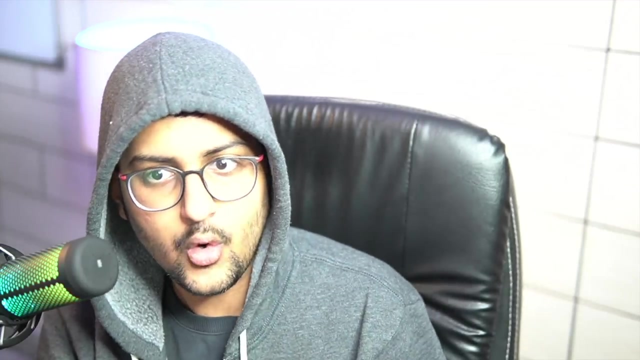 layer address those are the mac addresses okay so the router will assign like ip addresses and mac addresses to it and that way it will make sure like it reaches the correct particular device okay so since like the public and the private ip address will you know remain the same but the mac address will keep on changing as data will travel from one device to another so mac address like a 12 digit alphanumeric string it's called as media access control okay and it's a unique identity for a particular network interface it's used by all ieee 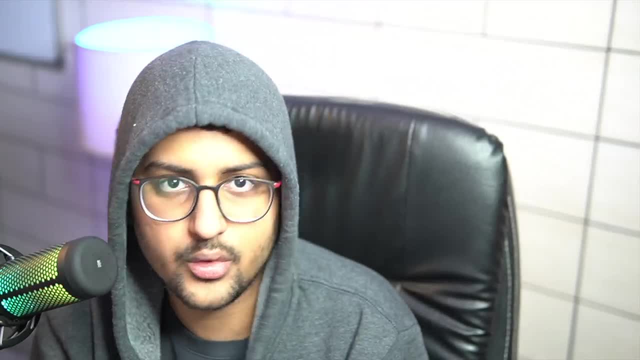 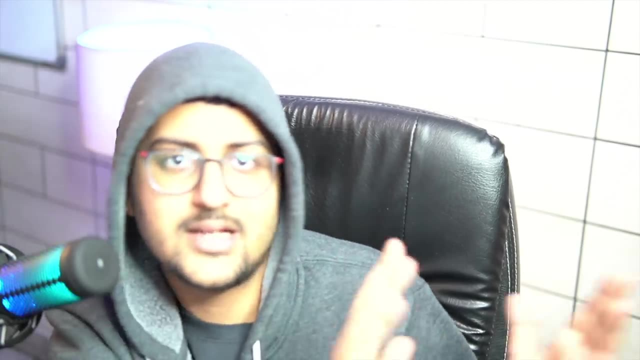 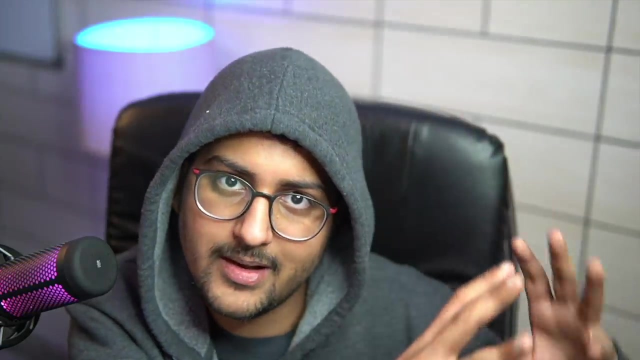 network technologies like ethernet wi-fi bluetooth and so on and so forth okay good so you can also block some of the devices like okay this mac address device is blocked or this a device is you know allowed or whatever you can do that using mac addresses as well i hope you are now able to understand how data travels from like the network layer to the data link layer and the data 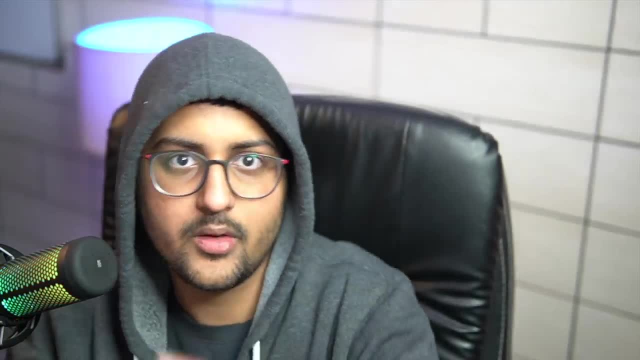 link layer is the one that works with mac addresses okay it works at your router level and with the physical devices okay so it converts these into like zeros and ones of the network so that is why this is color reaction connected so it works with any of these devices okay so it's great to know that mac addresses are around internet but yeah dark boards are good and i really hope you learned much about internet as well and i hope you learned things that I learned a lot from this tutorial and of course� 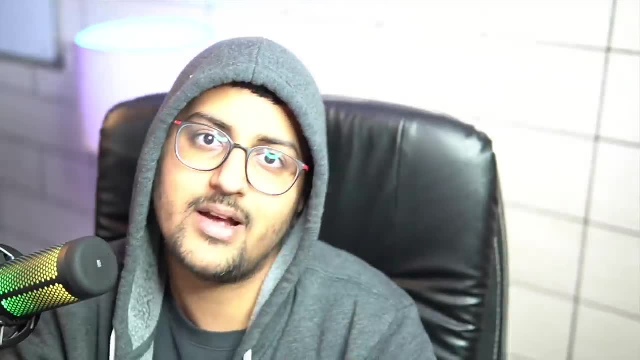 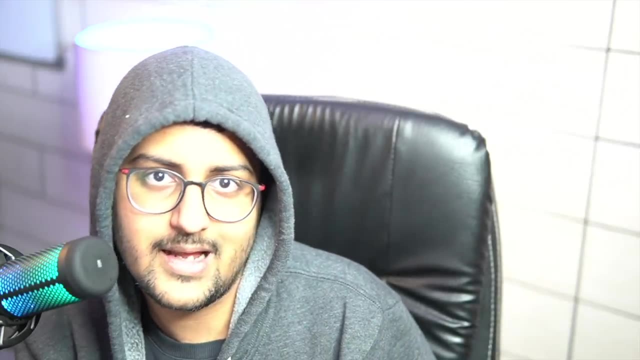 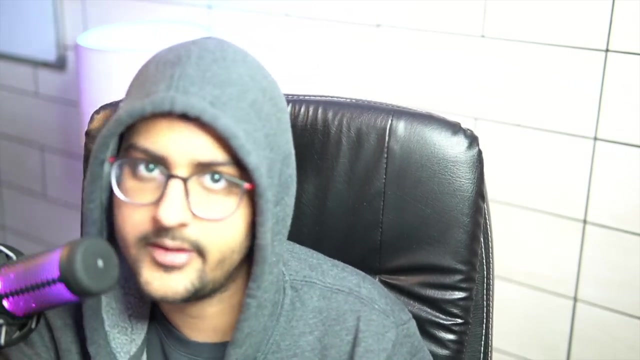 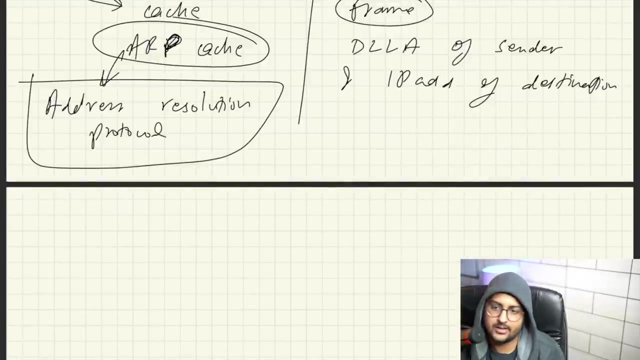 bits and transfers is into your physical devices using all the protocols everything we just mentioned okay address resolution protocol and everything so we talked about protocols in like all the layers we have talked about all the protocols in every layer and where every layer works everything is covered remember like the command we did if config you can use that command to check your mac address also okay so that's basically about it and uh yeah that's the data 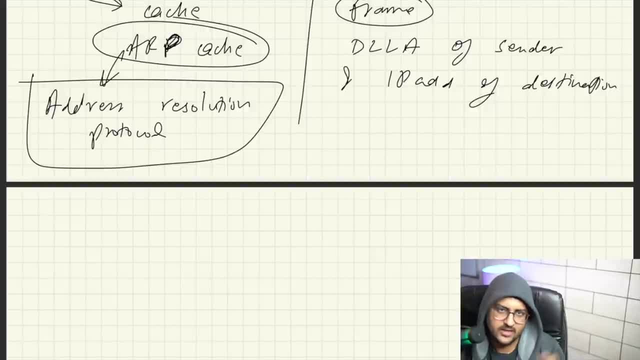 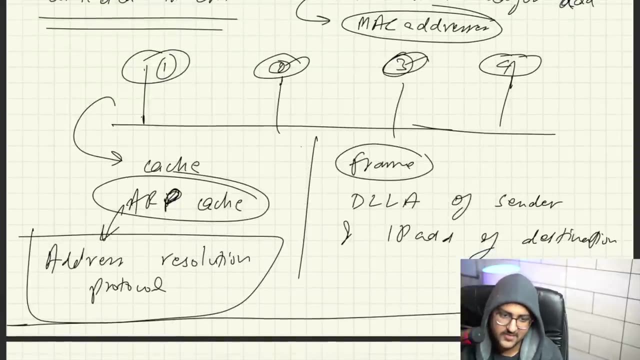 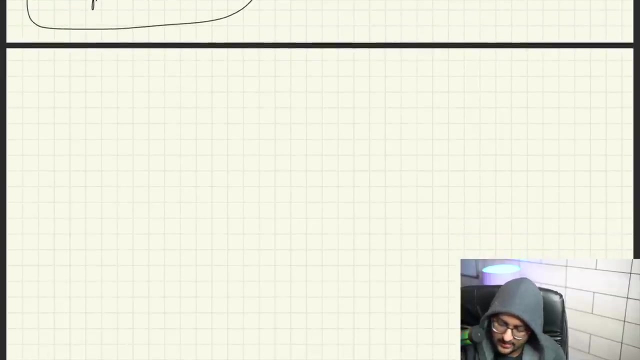 link layer and that's address resolution protocol and then comes like the physical layer so actually data gets converted into electrical signals and then gets sent to your devices or whatever okay so i was in short about how you know not in short we covered a lot of things how the the internet works uh if you want to more if you look at more at like the uh data link layer part you can check out how it does like the uh for example uh there's this thing called like framing okay the framing uh like working with the frames how those get converted and everything it also does error detection okay just mentioning some few things you can check in in brief like that was it and 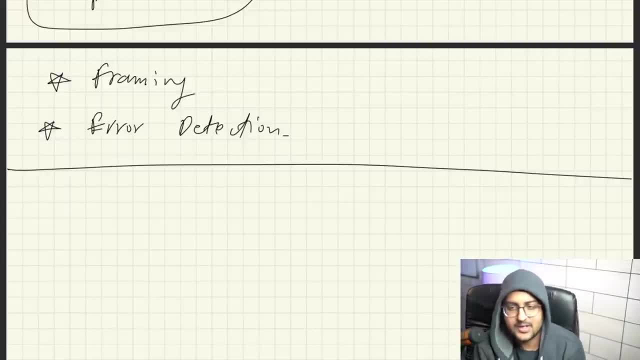 that's how the you know internet works and uh i'm super excited and if you just a few things we are doing complete devops bootcamp so uh like in depth i taught you all these things i'll teach you that as well so first of all make sure you like share subscribe right now and comment right now and 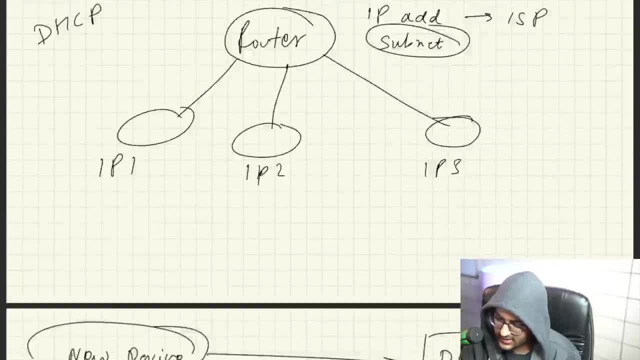 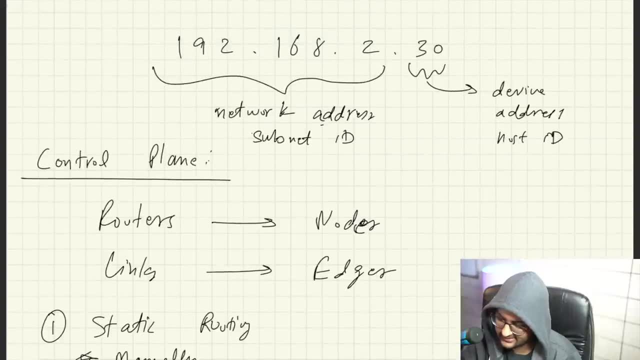 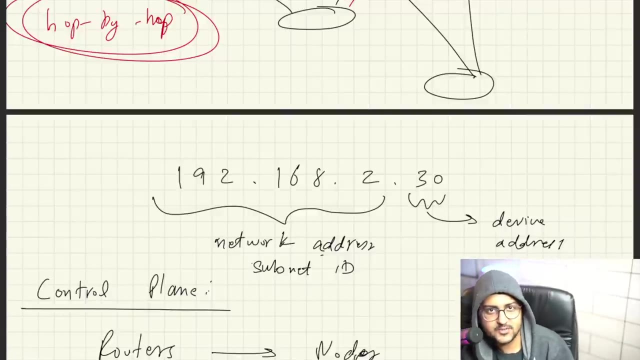 you can take a photo of this and uh then you can like maybe yeah you can take a photo and then you can uh like um you know add it on socials you can use the hashtag devops with kunal the twitter bot will retweet so it's a our learning in public initiated that initiative that we always support